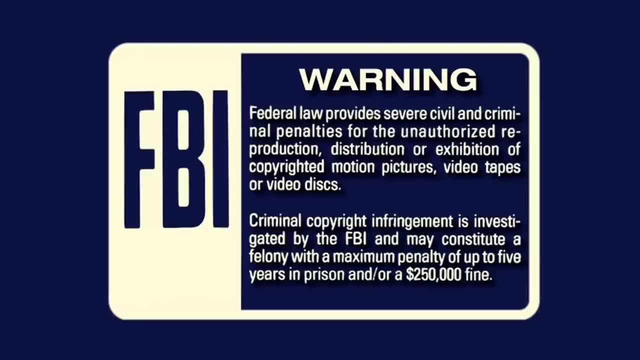 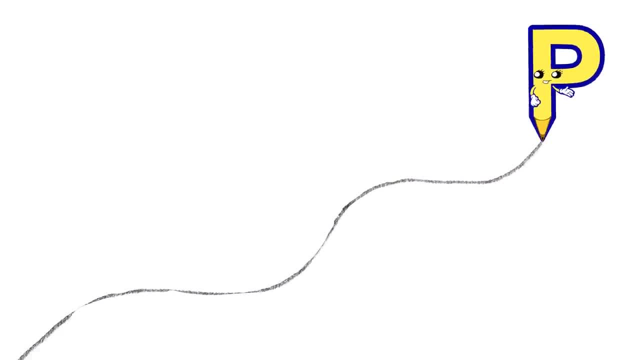 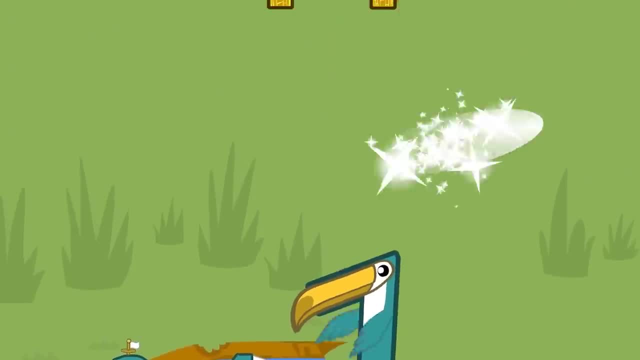 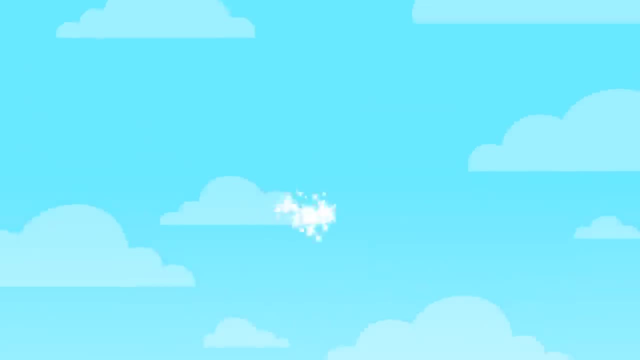 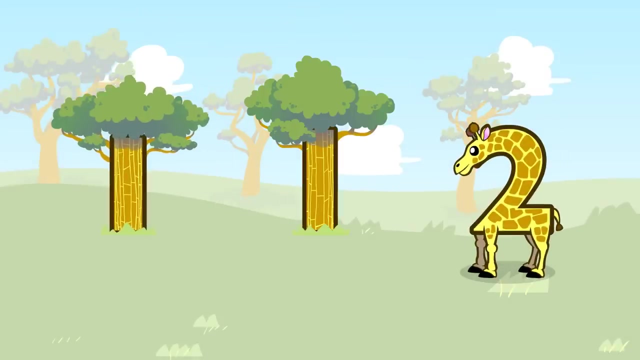 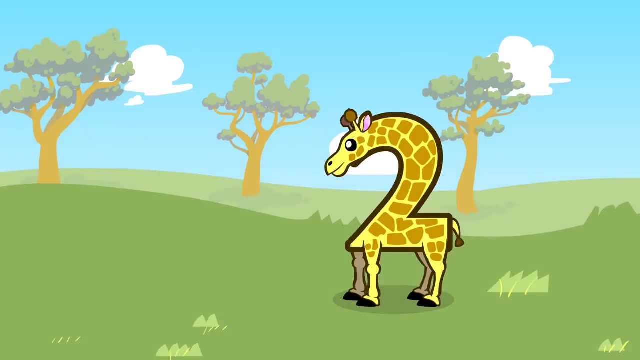 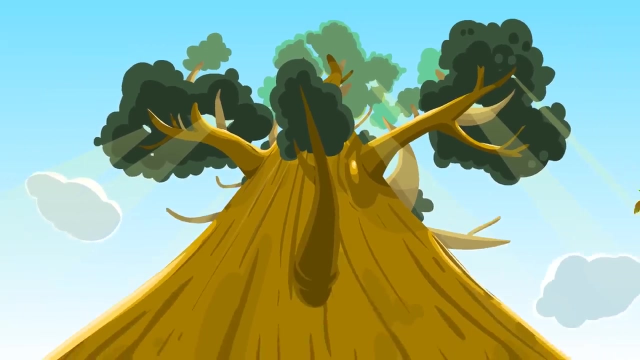 Preschool Prep Company Presents: Meet the Math Facts. Yay, 1 plus 1 equals 1 plus 1 equals 2!. 1 plus 1 equals 2!. 1 plus 1 equals 2! 2!. 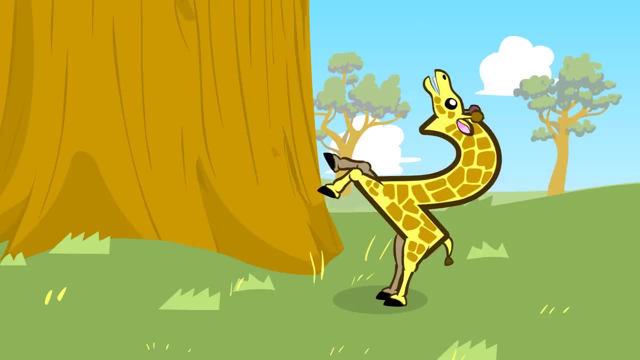 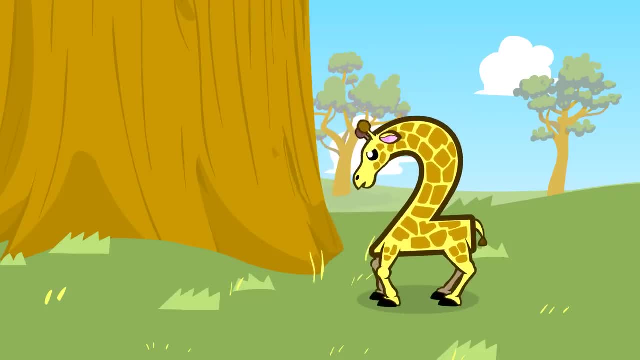 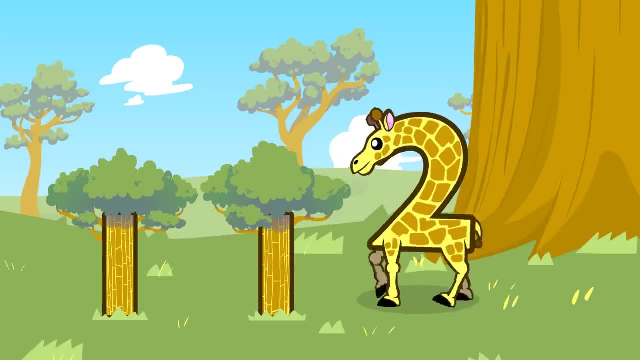 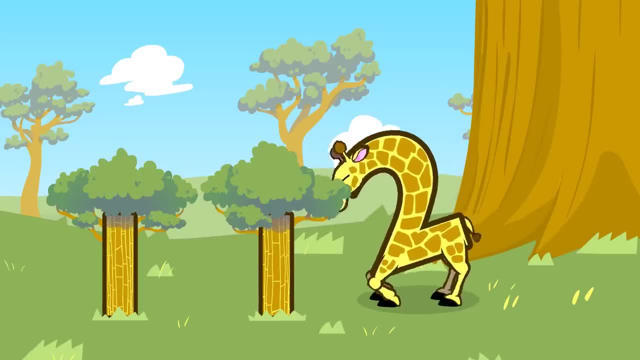 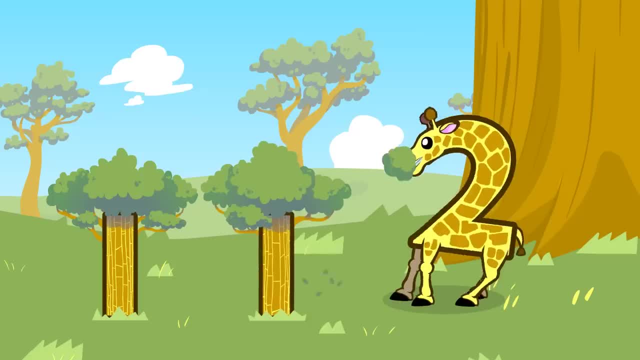 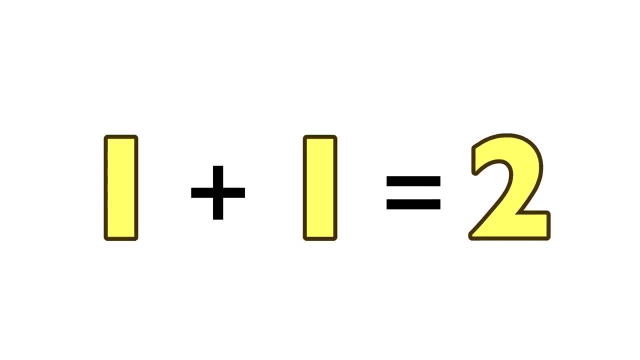 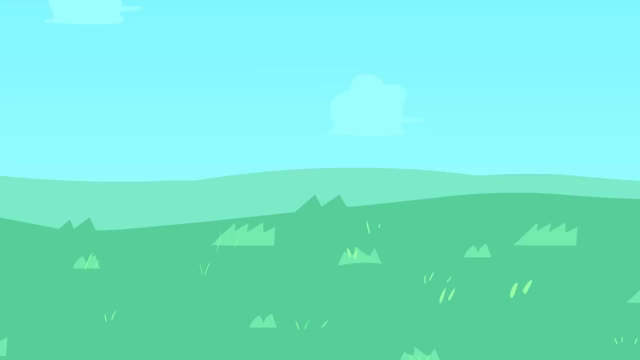 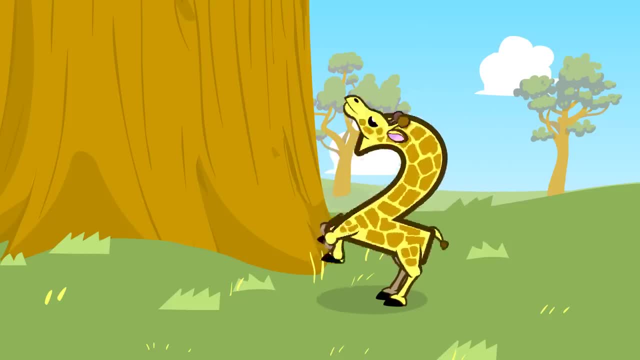 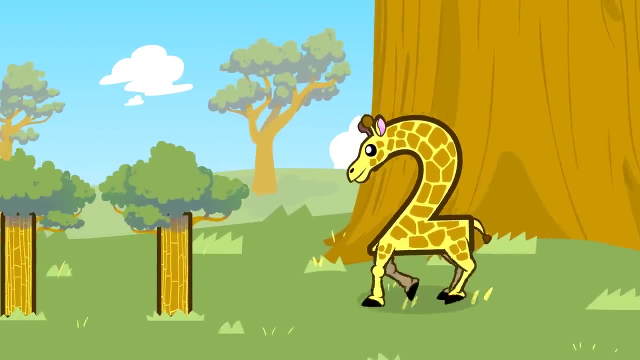 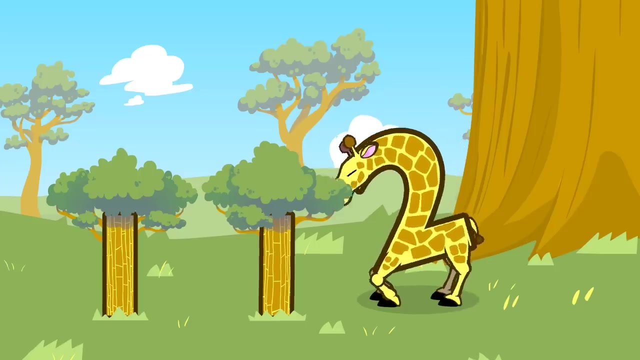 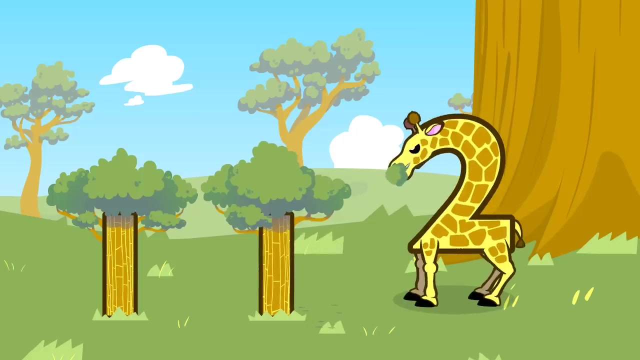 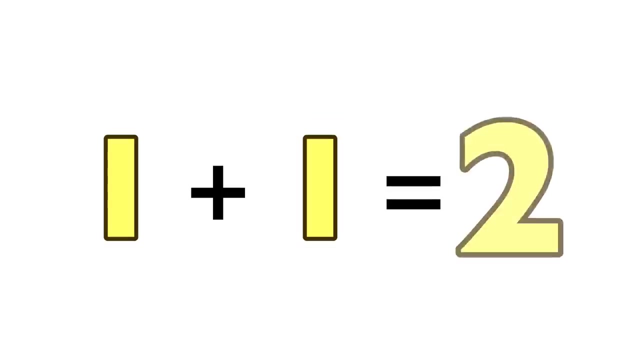 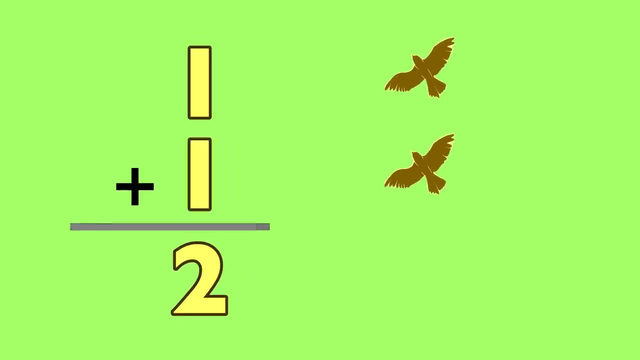 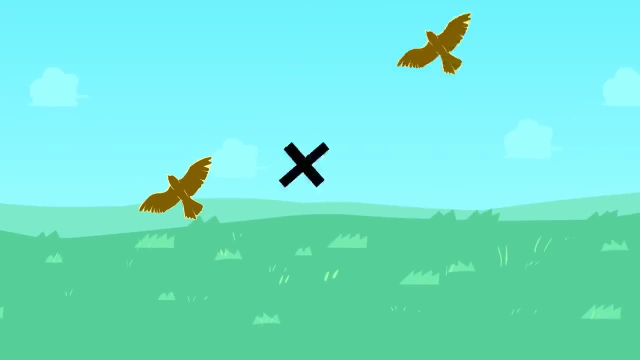 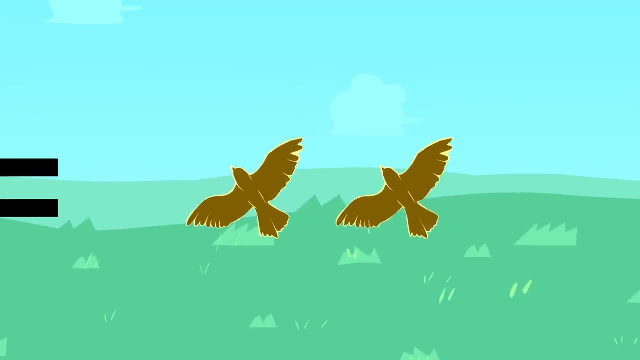 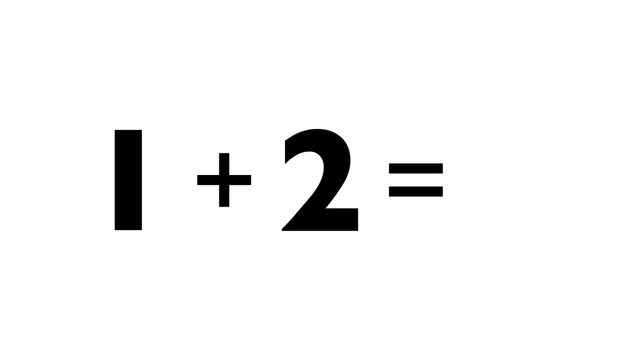 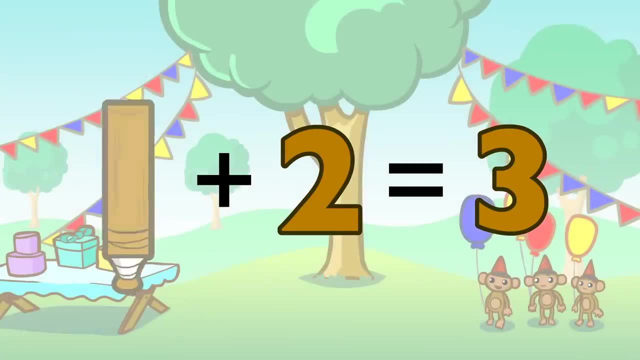 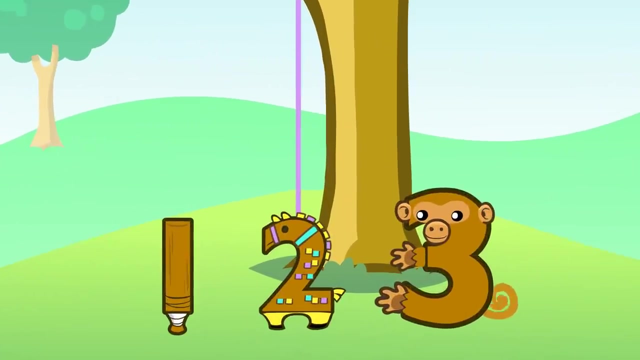 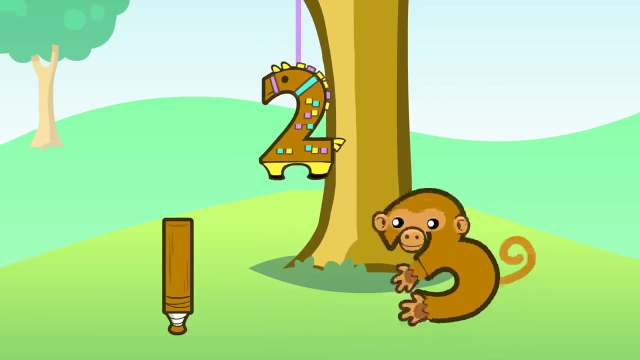 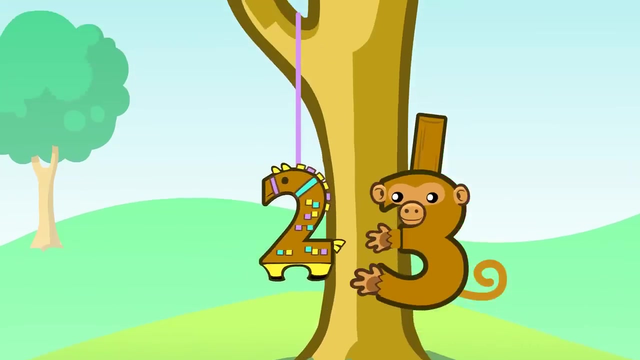 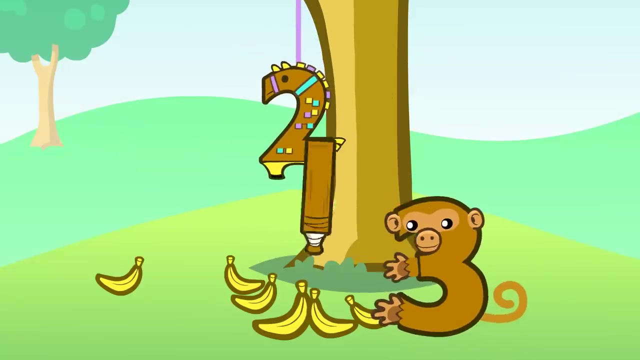 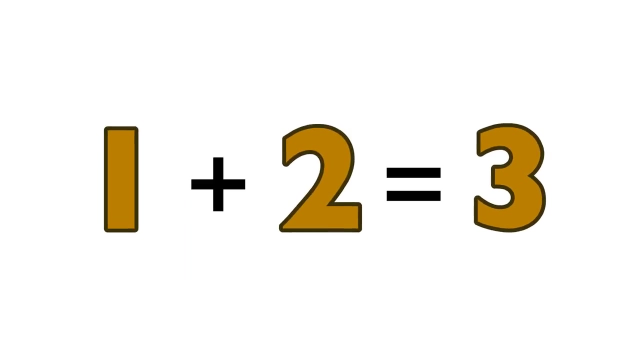 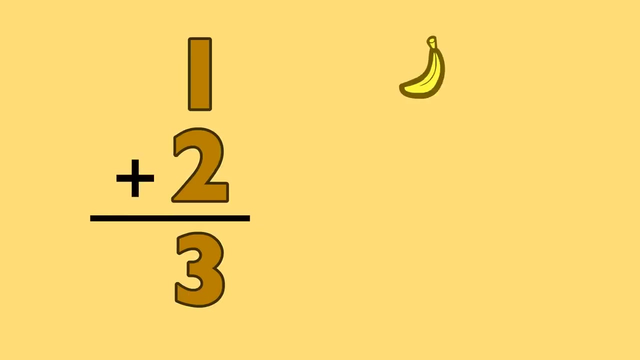 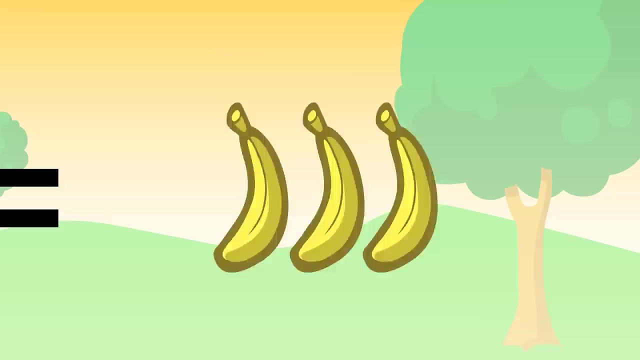 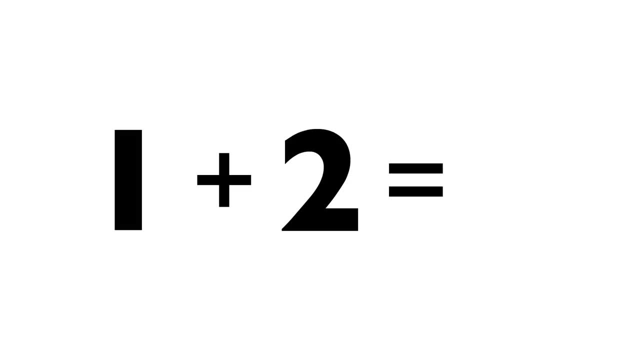 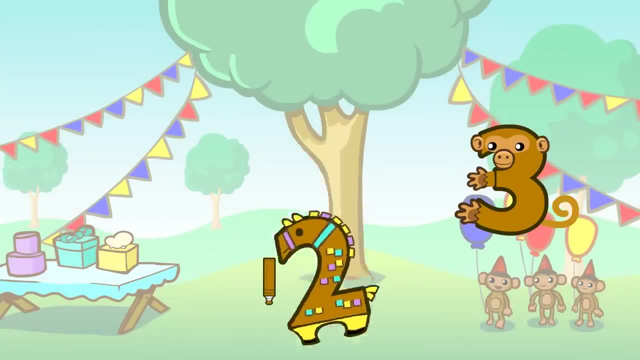 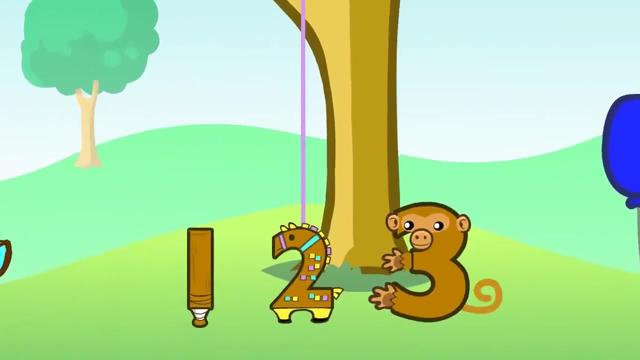 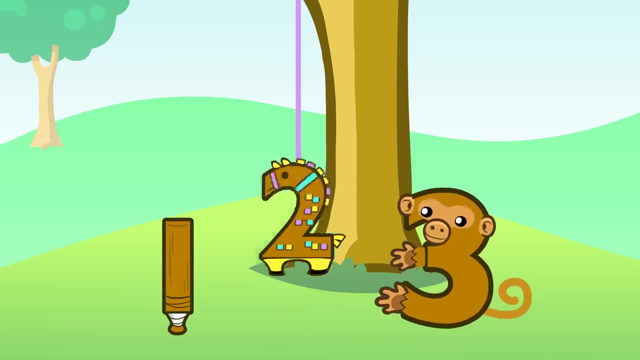 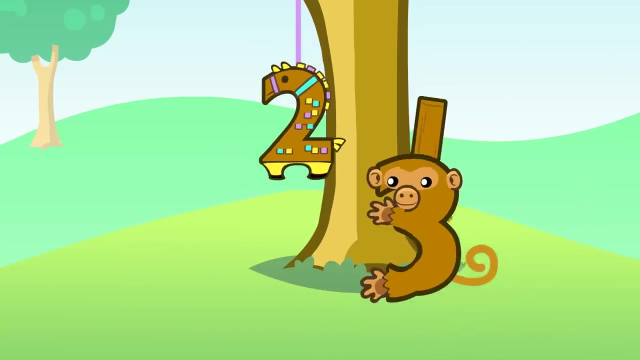 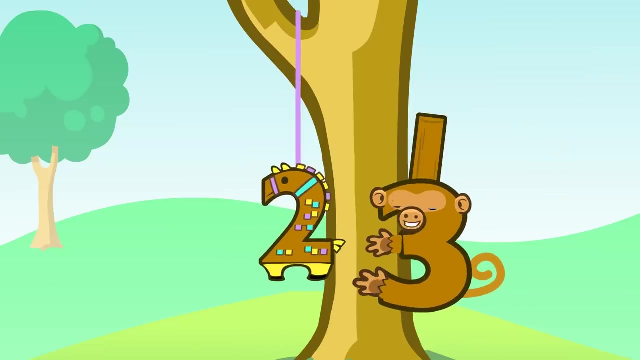 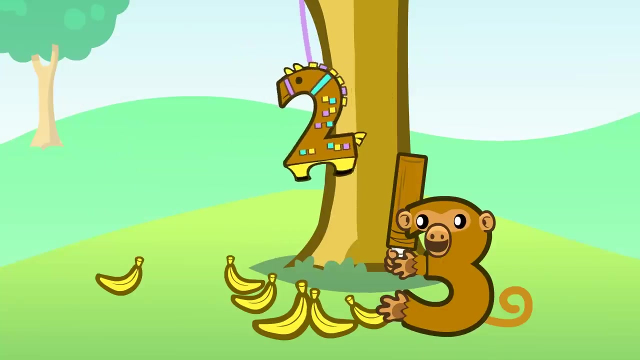 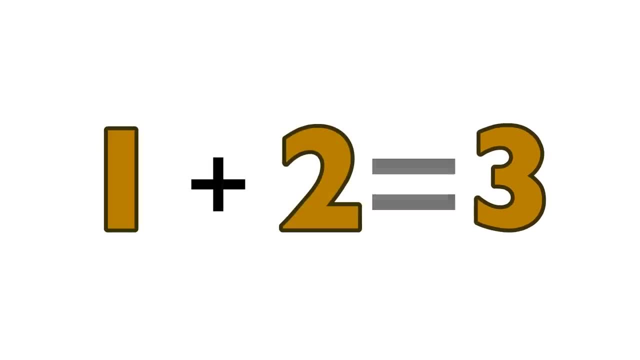 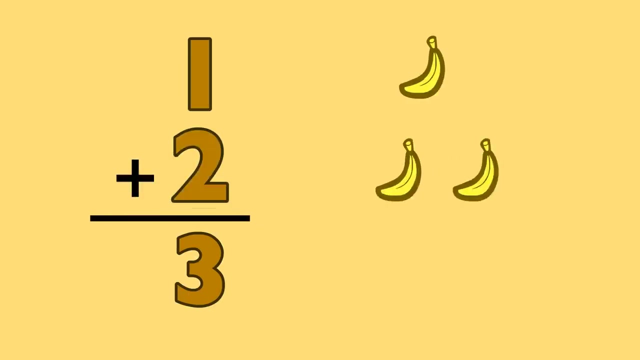 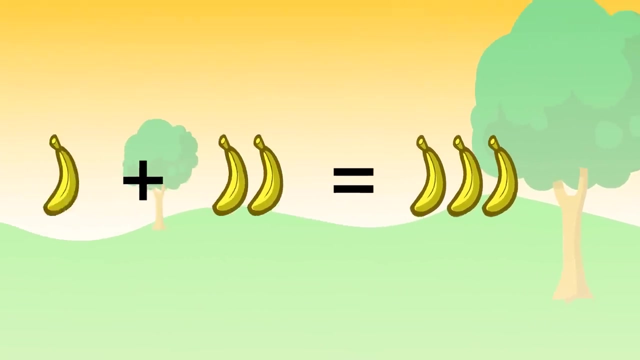 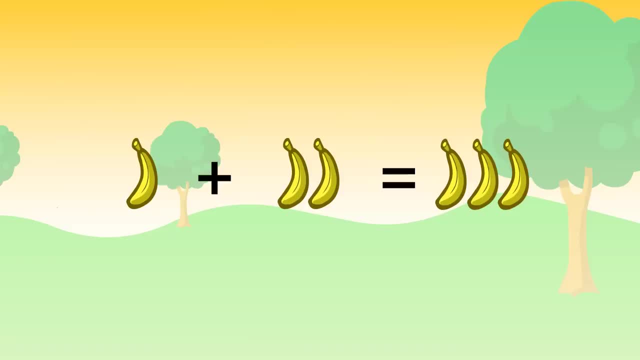 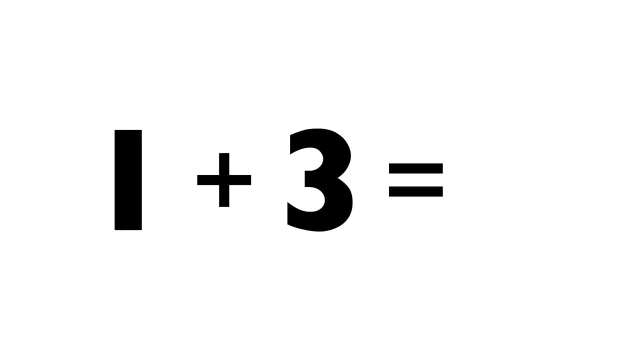 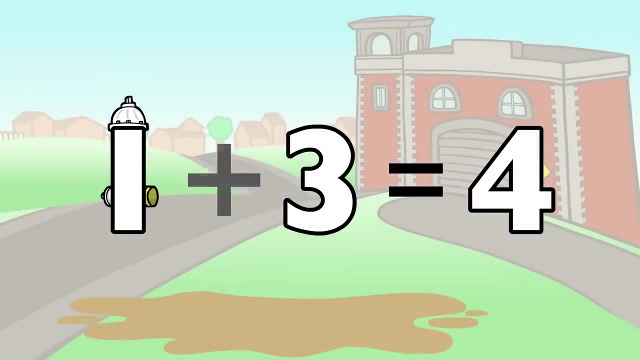 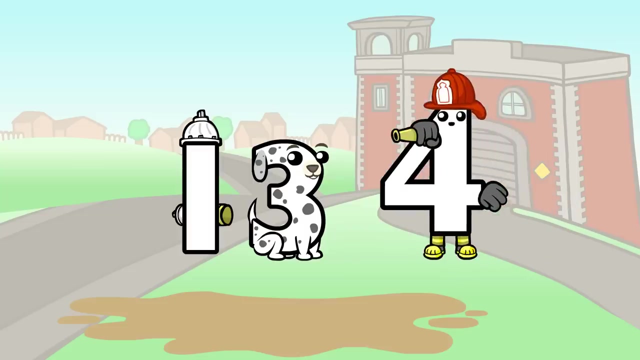 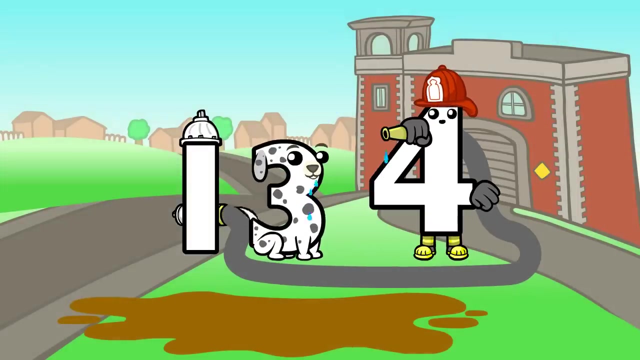 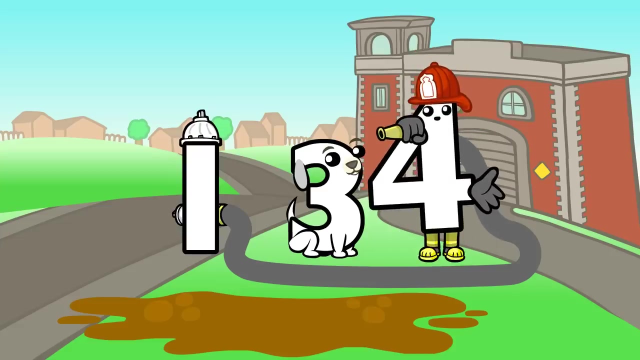 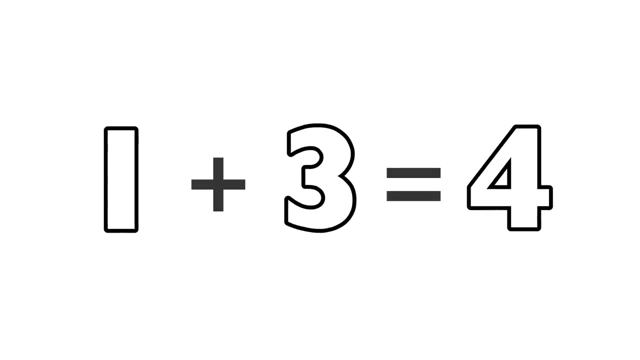 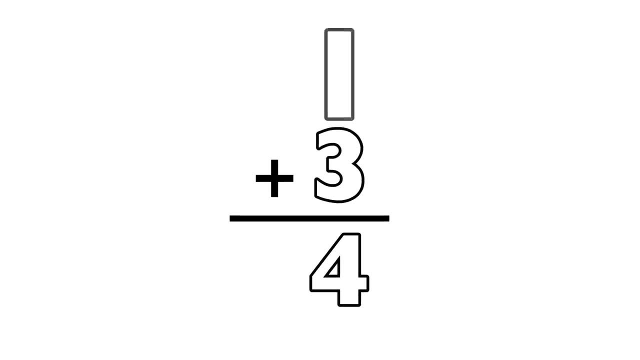 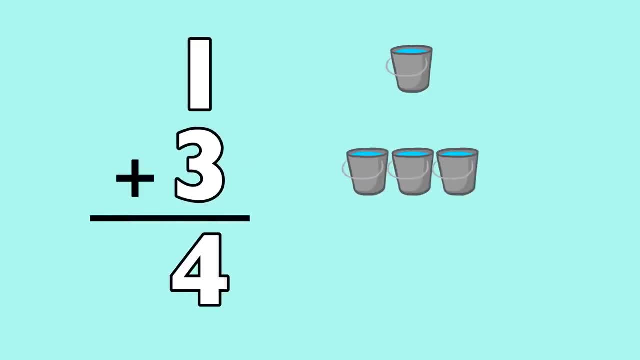 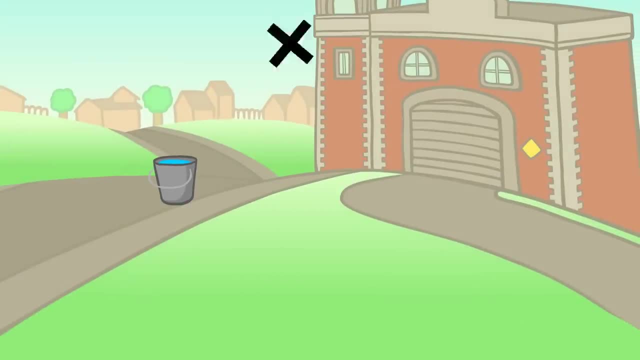 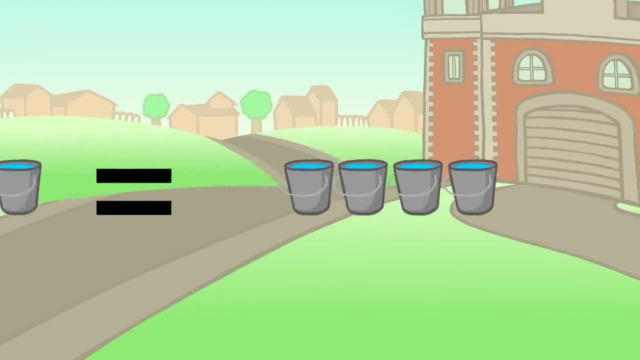 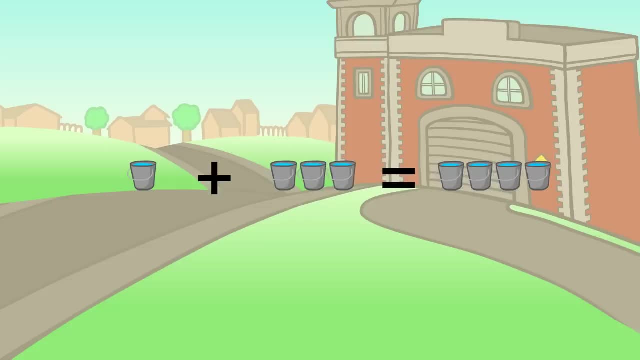 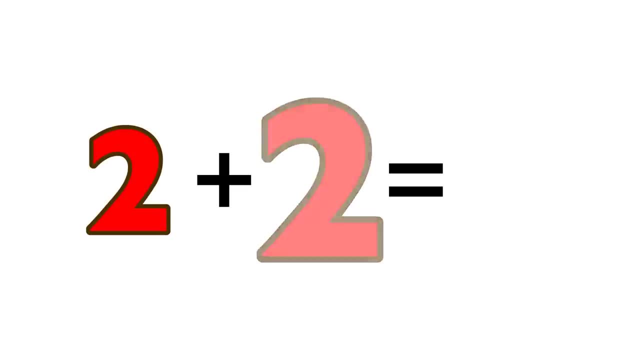 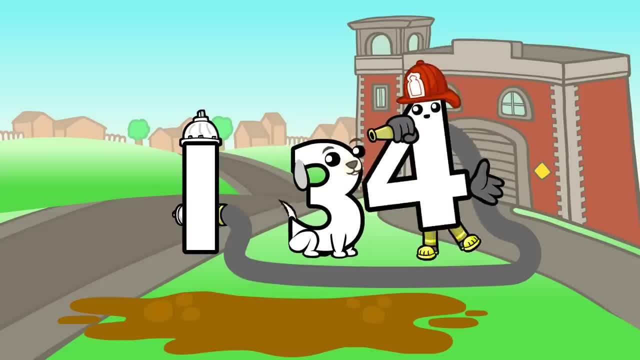 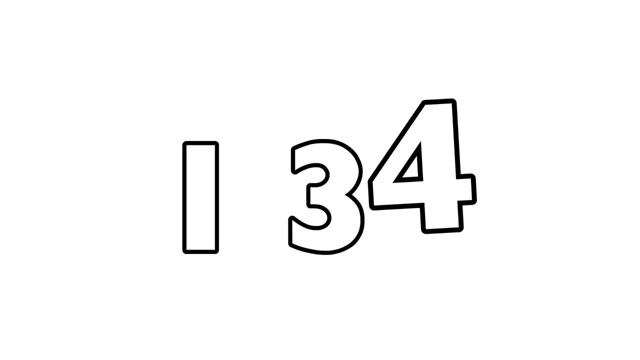 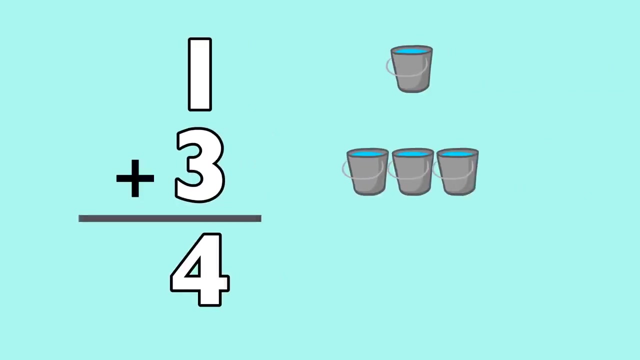 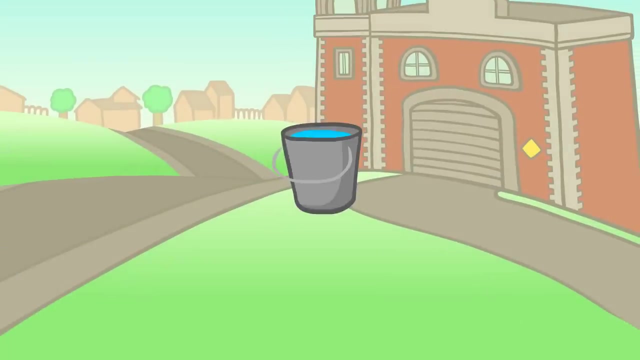 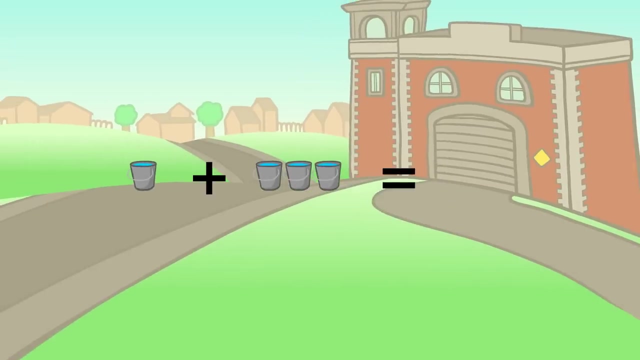 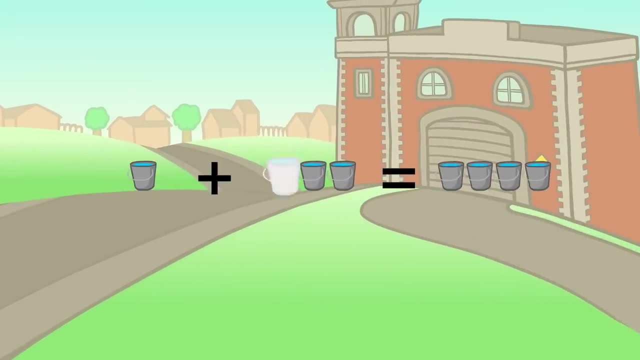 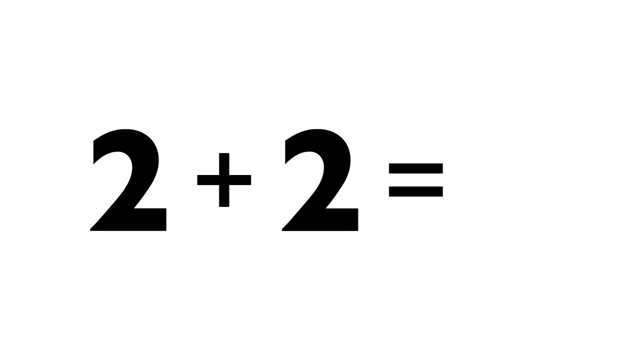 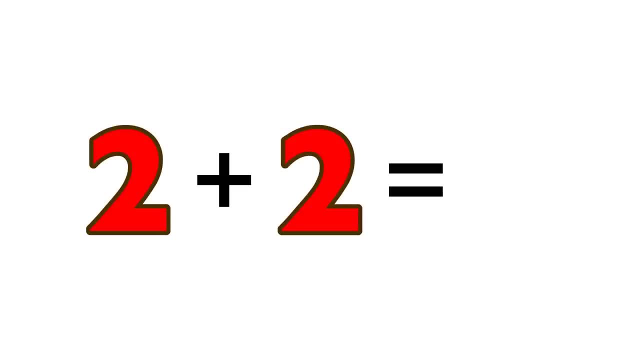 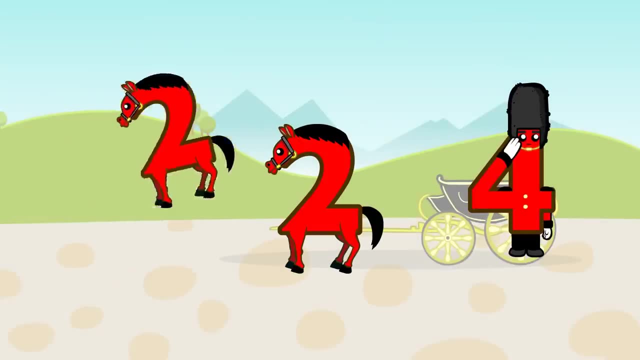 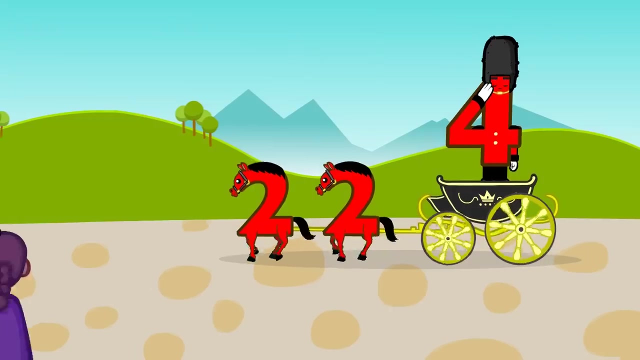 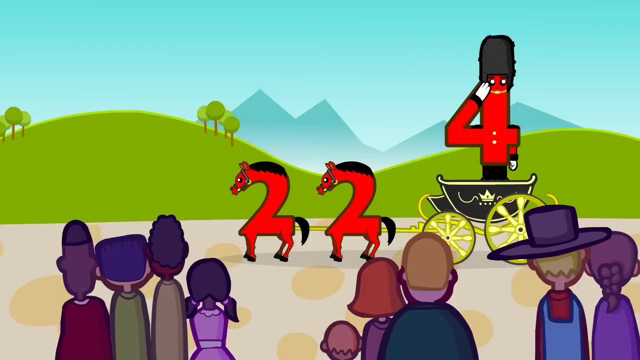 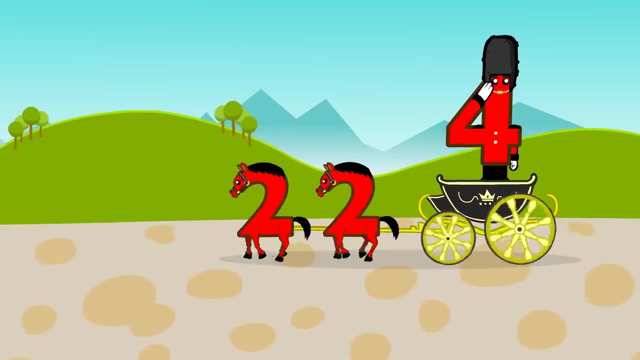 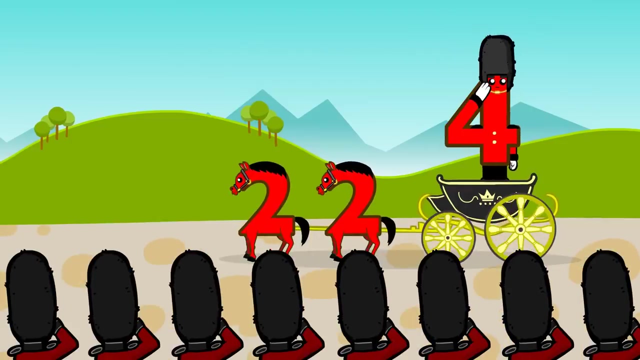 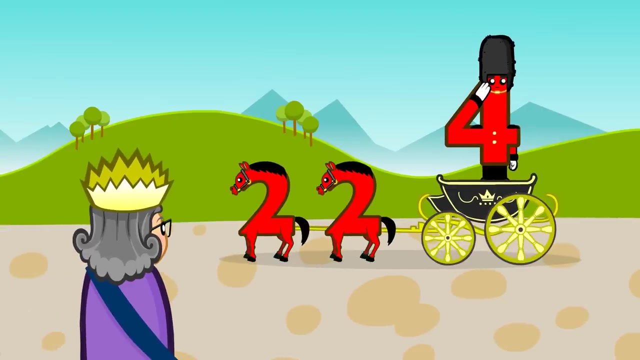 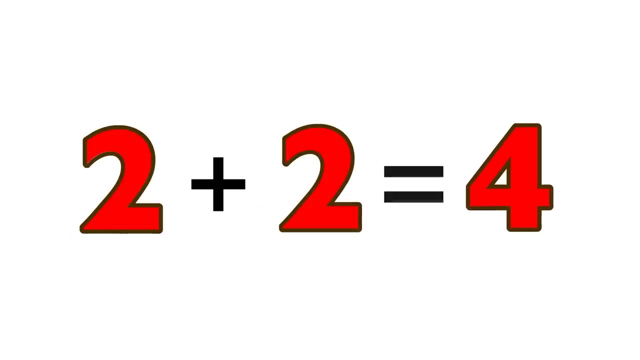 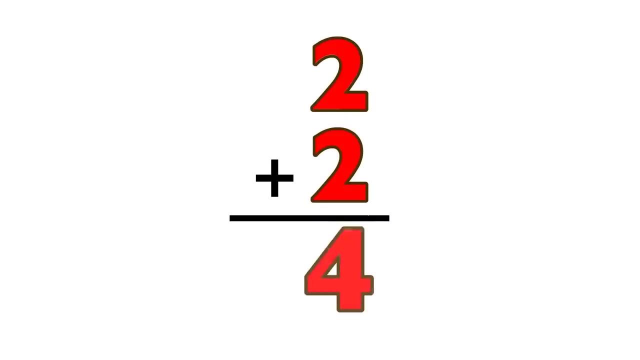 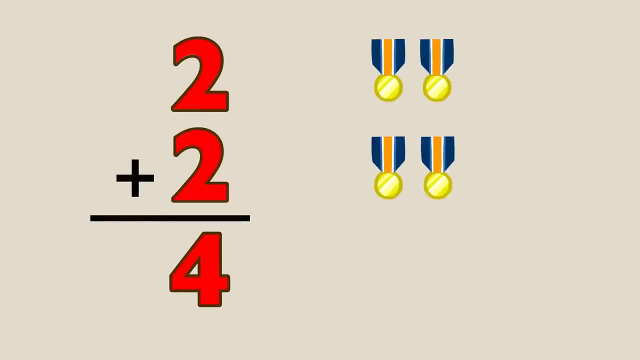 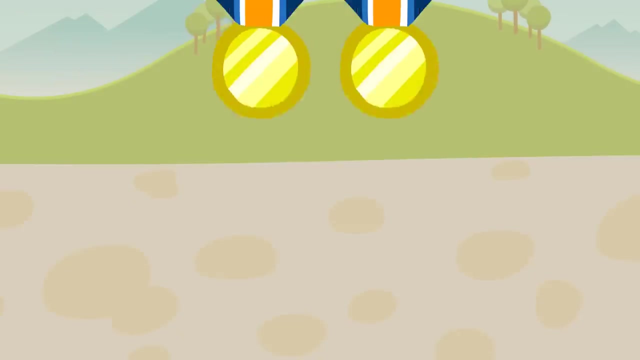 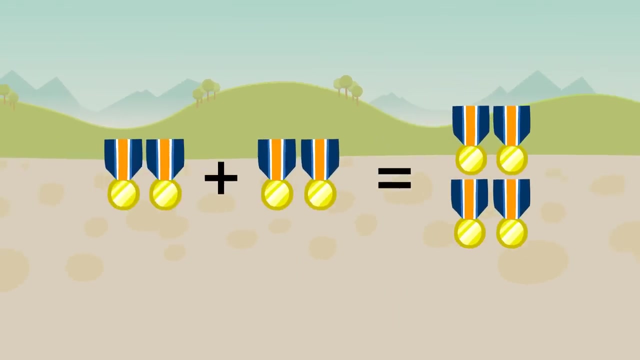 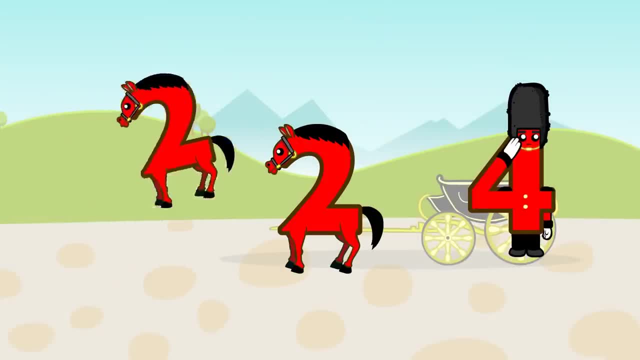 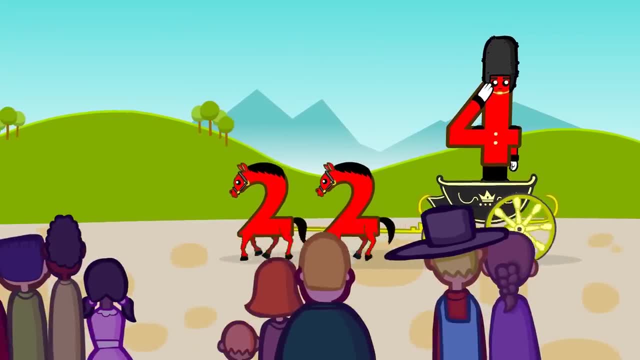 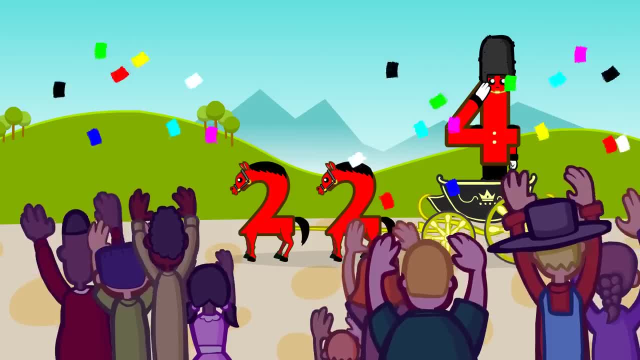 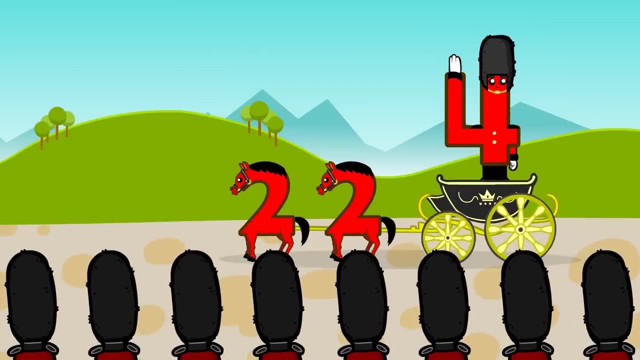 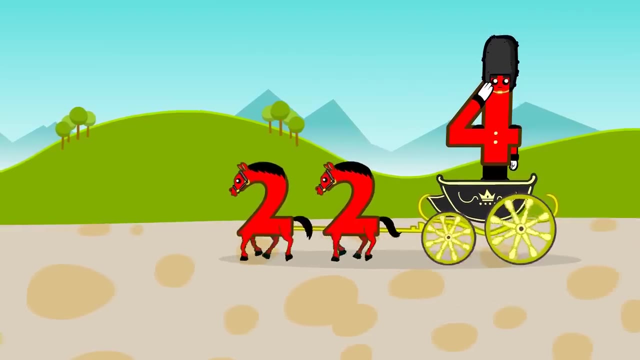 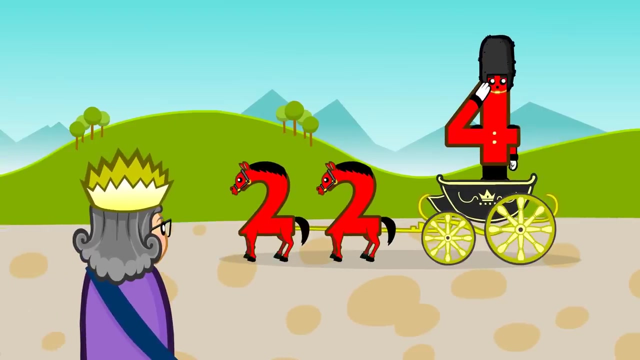 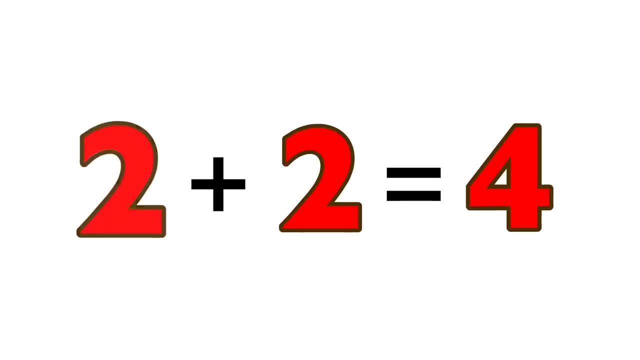 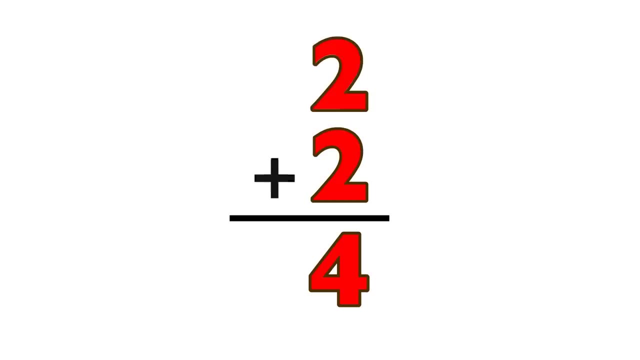 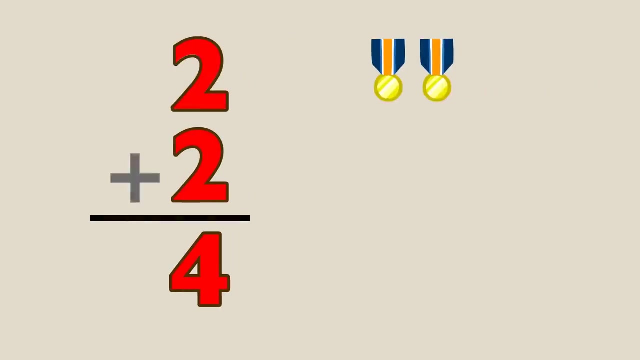 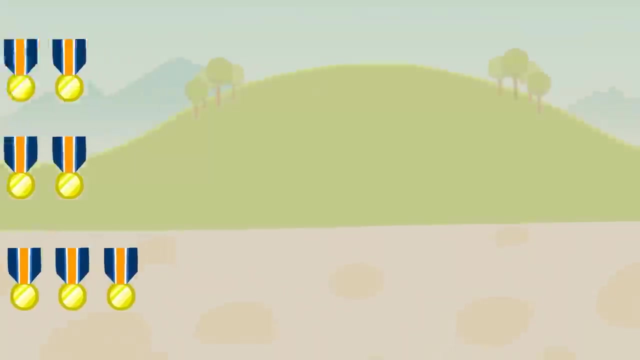 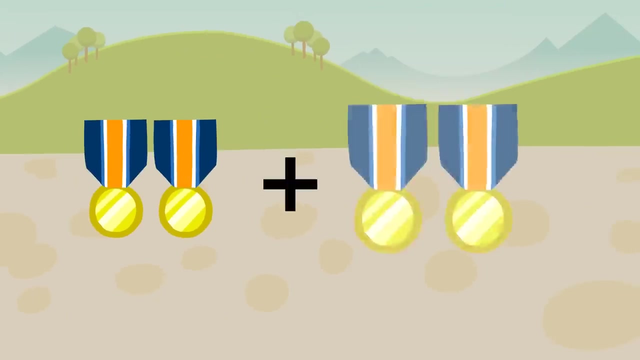 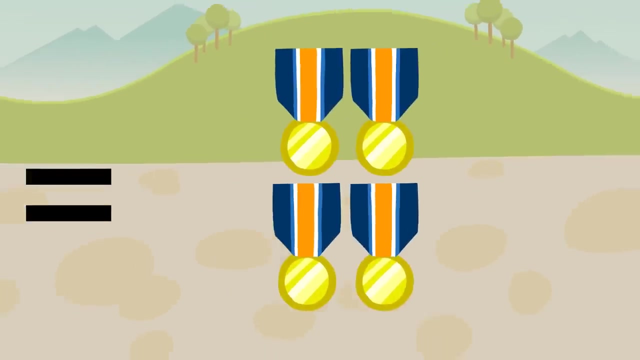 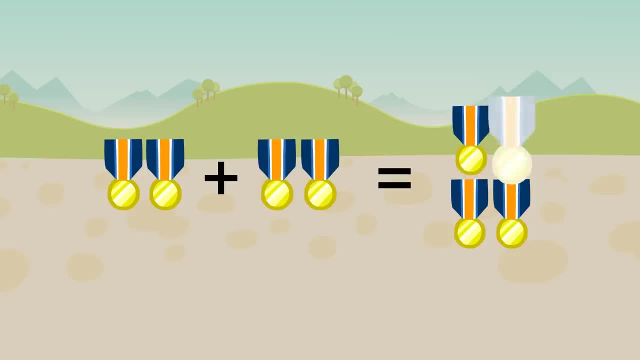 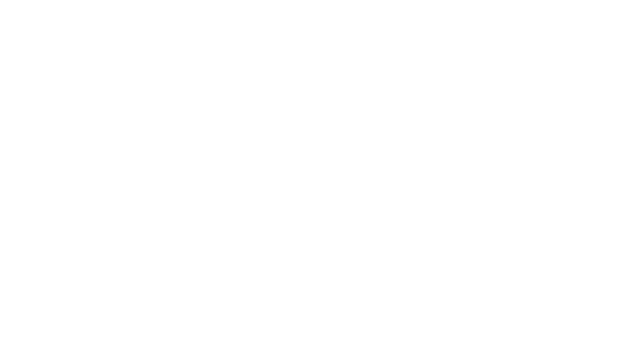 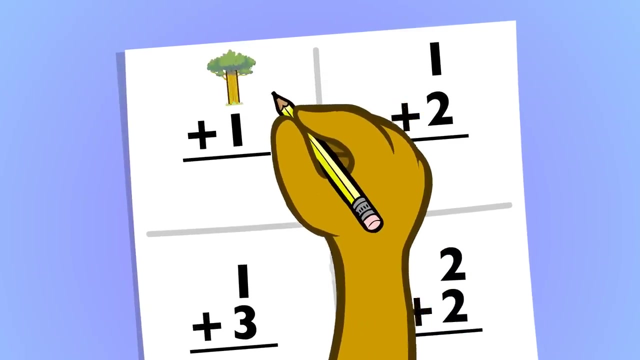 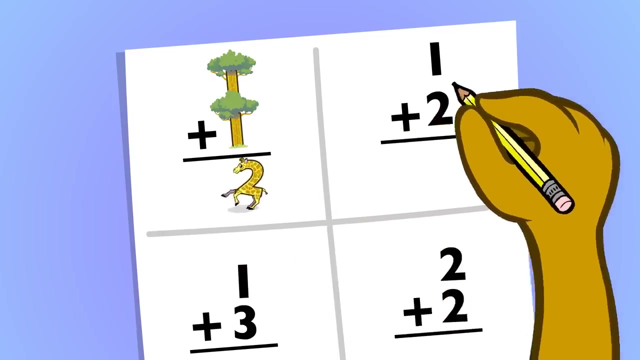 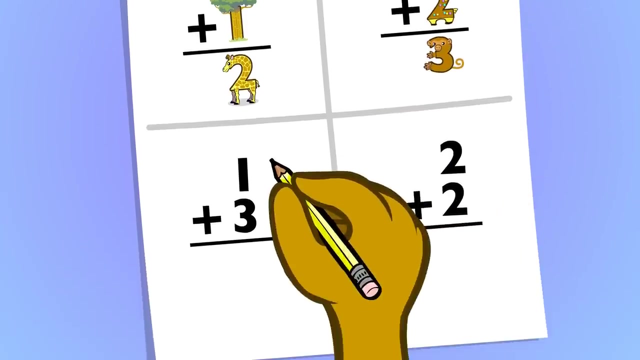 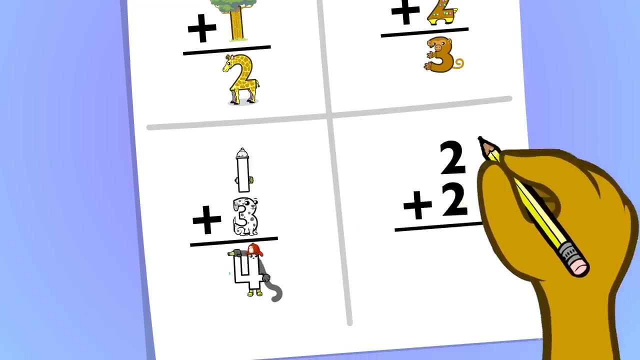 1, 2, 3, 4 equals 1,2,3 ,4. 1, 1 Plus one equals two. One plus two equals three. One plus three equals four. Two plus two equals. 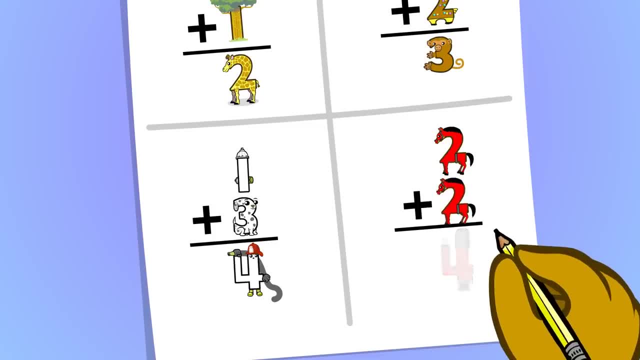 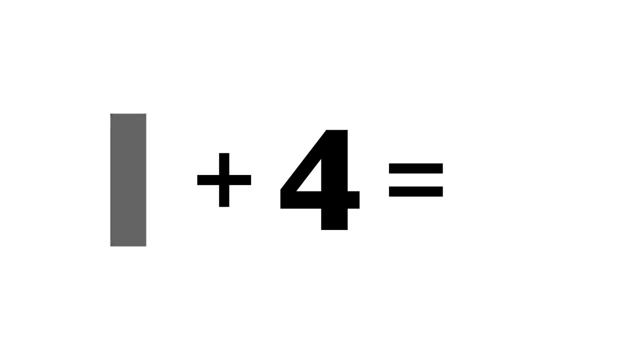 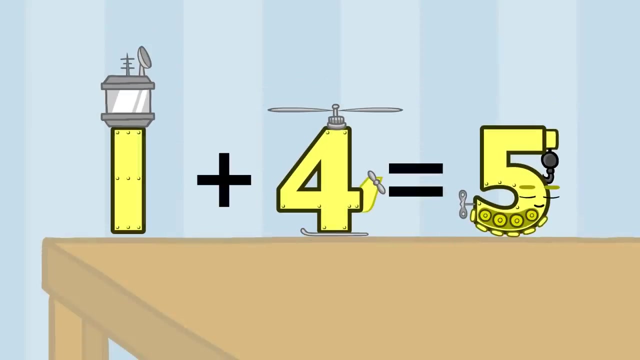 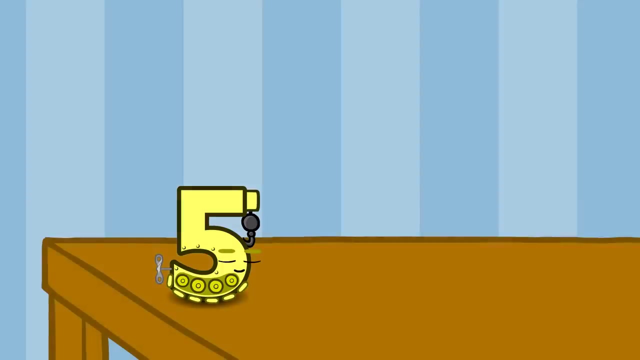 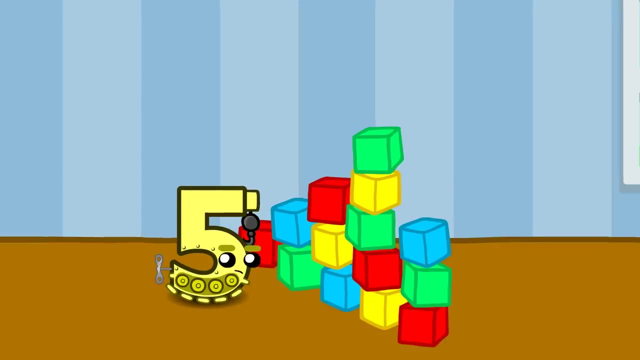 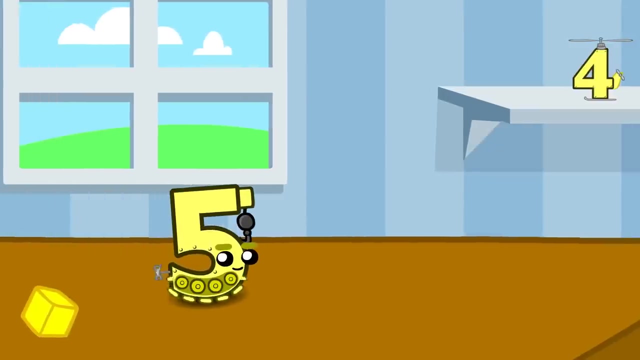 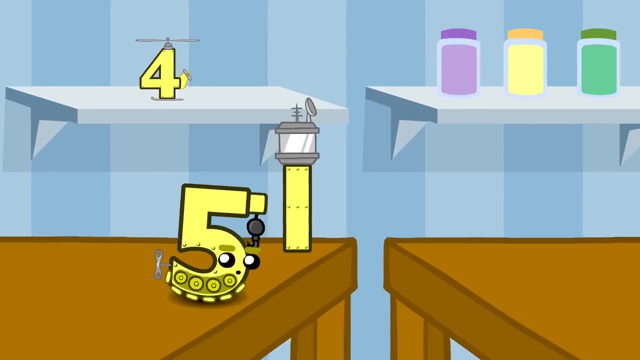 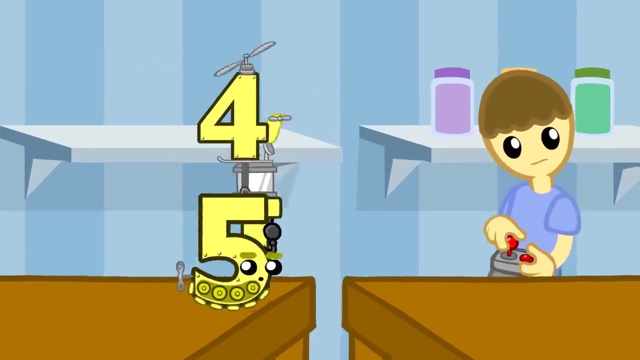 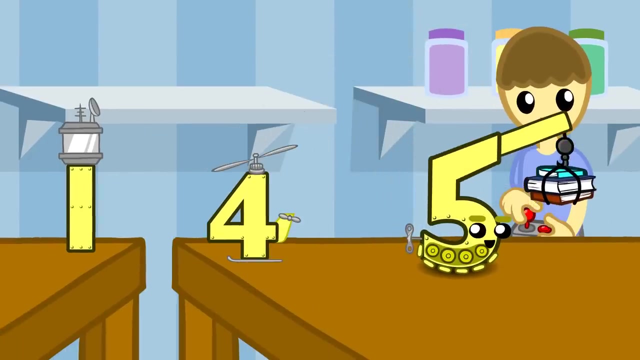 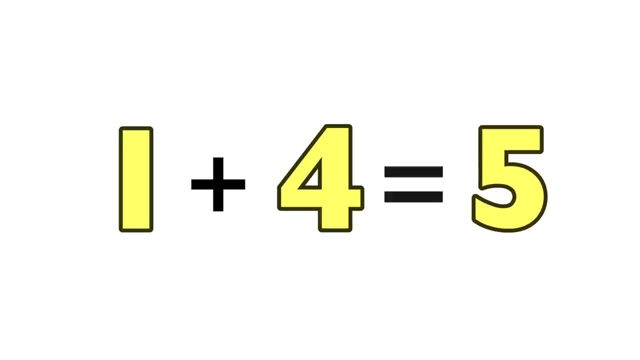 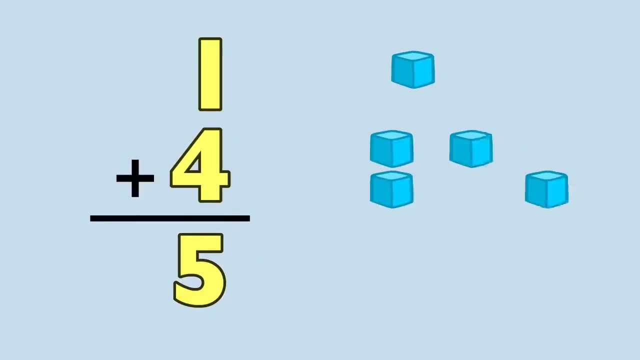 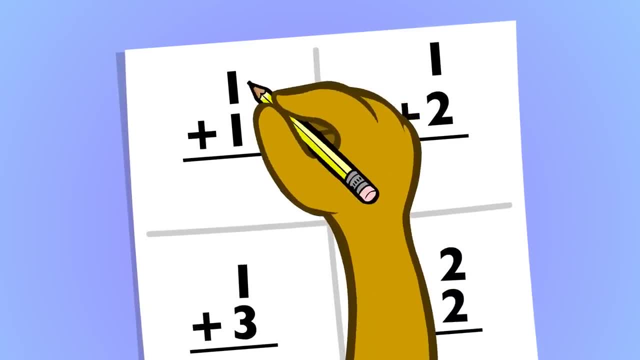 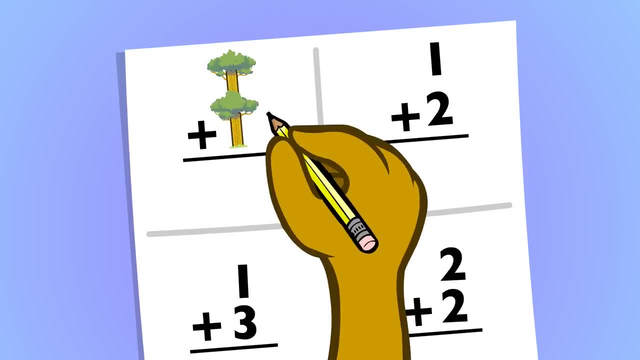 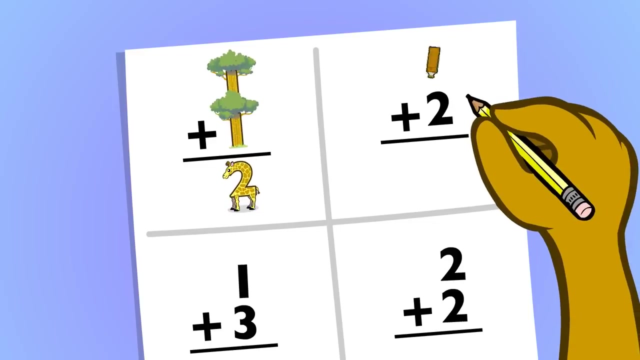 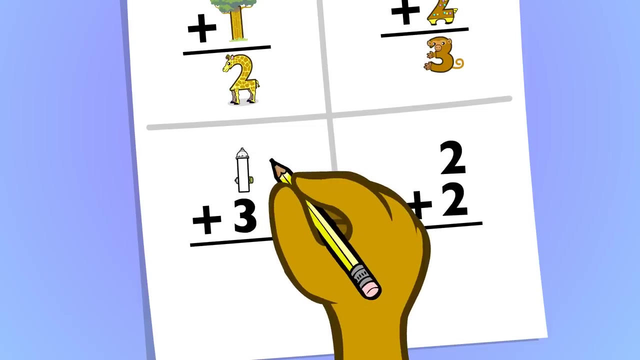 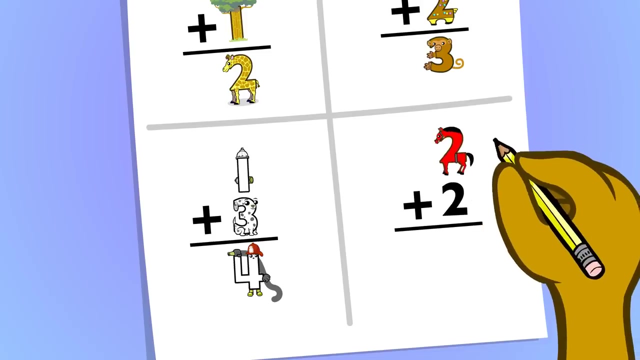 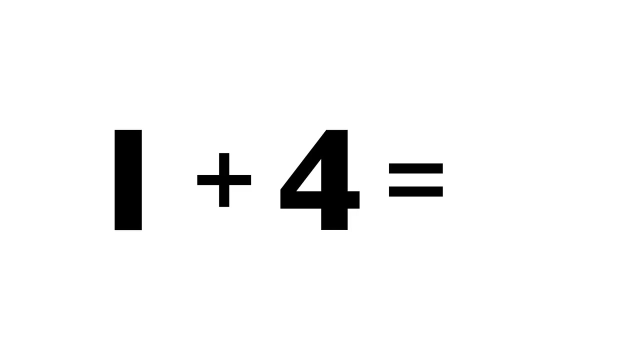 1 plus 1 equals. 2.. 1 plus 2 equals 4.. 3.. 1 plus 3 equals. 4.. 2 plus 2 equals 4.. 4.. 1 plus 4 equals. 1 plus 4 equals 5.. 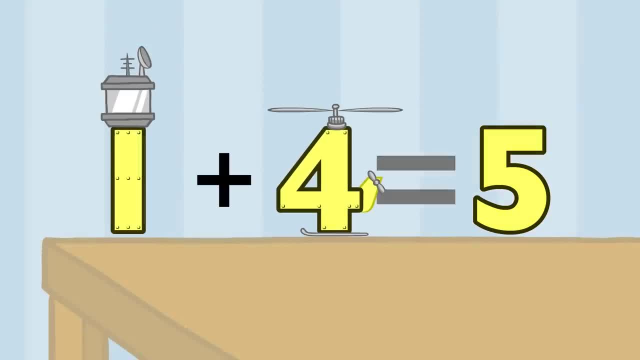 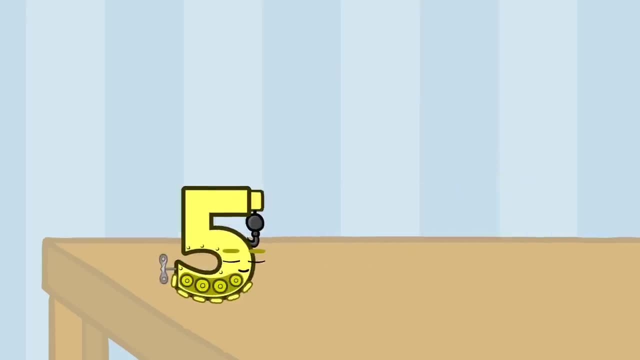 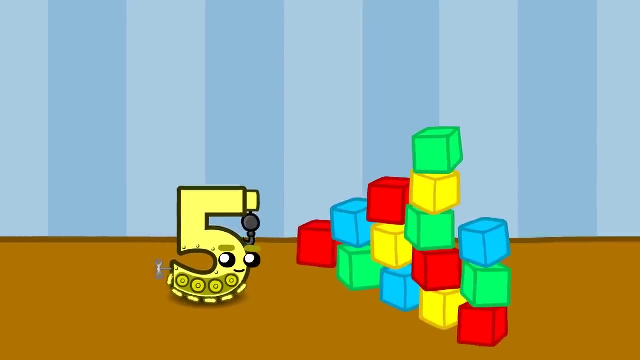 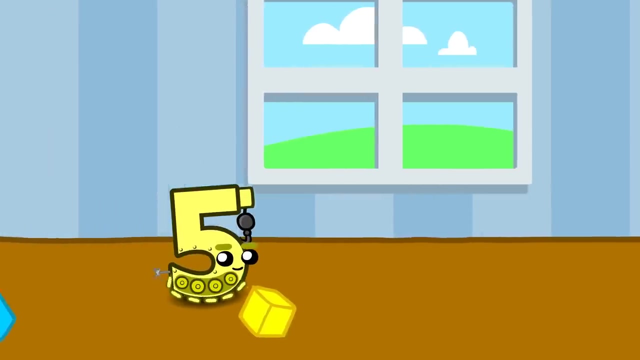 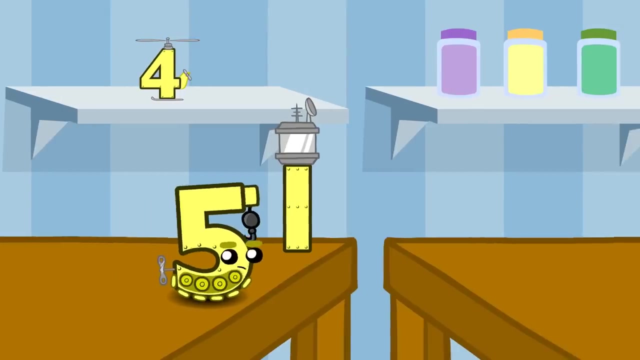 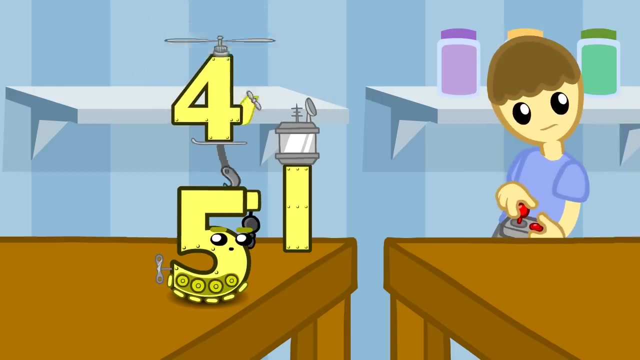 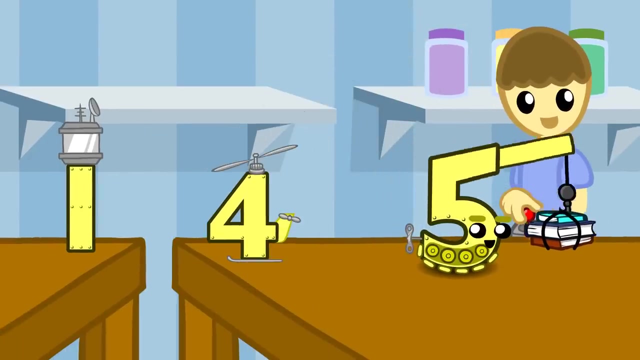 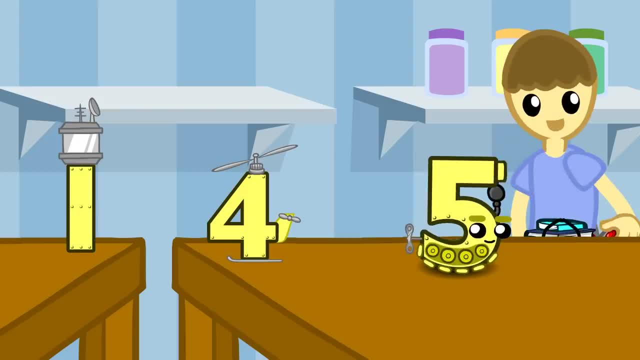 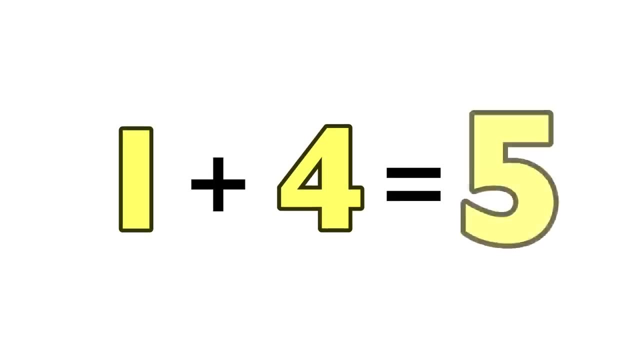 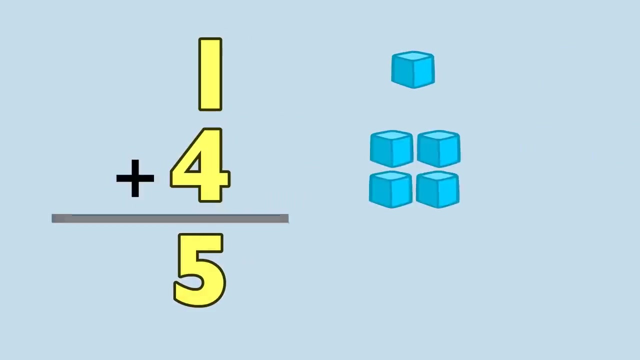 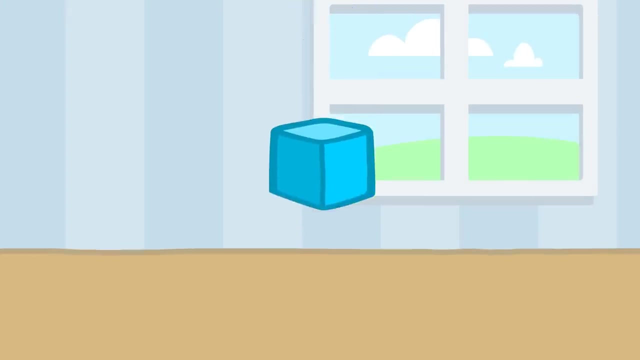 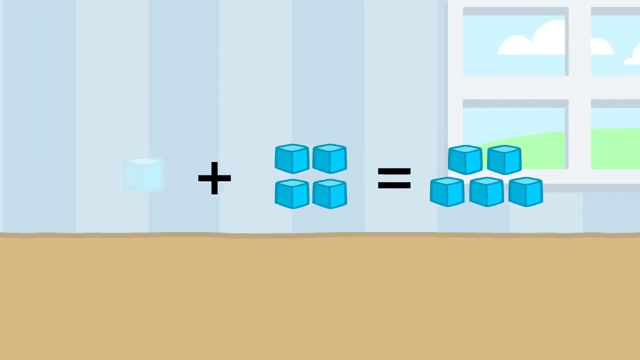 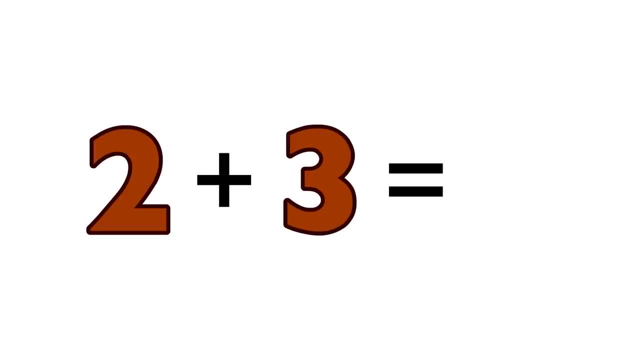 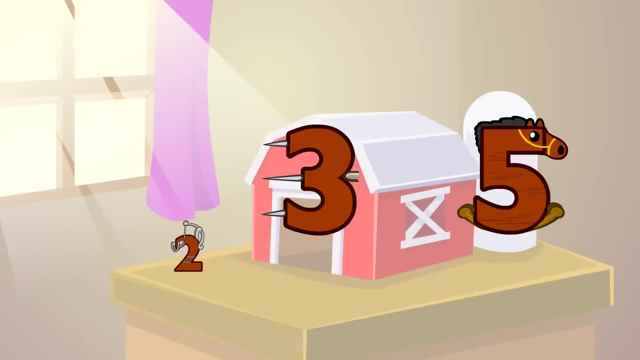 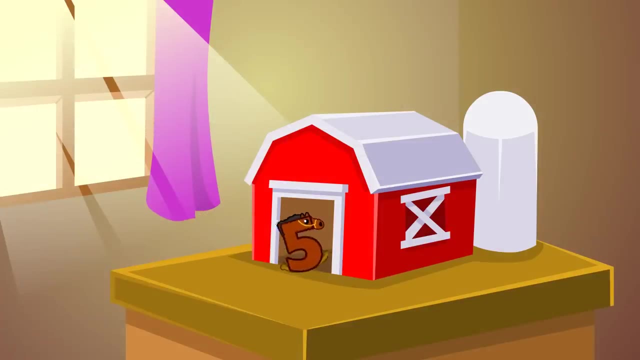 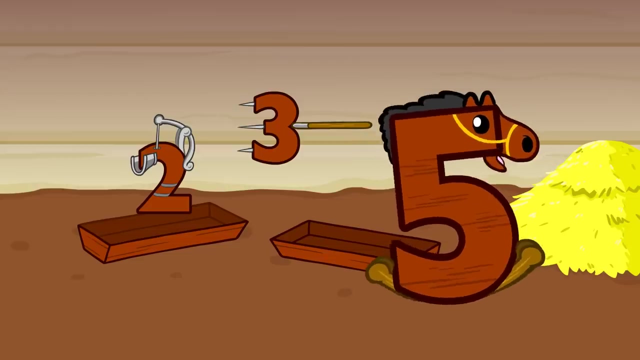 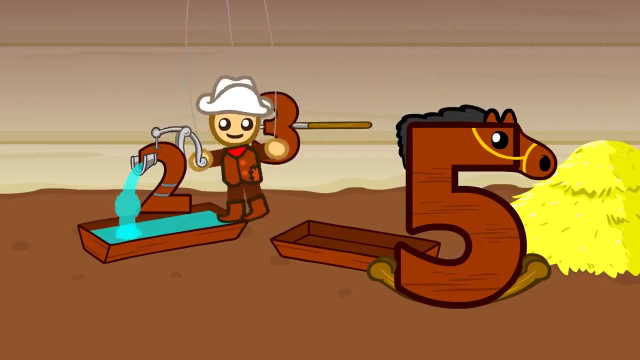 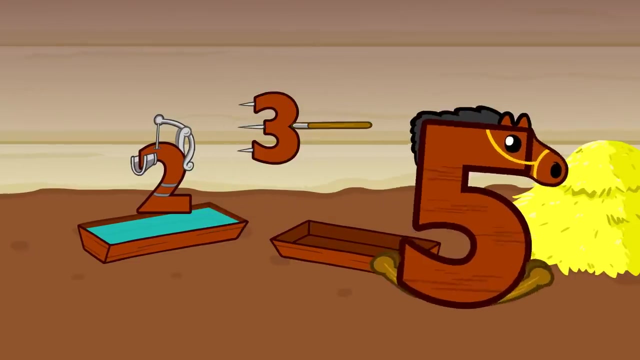 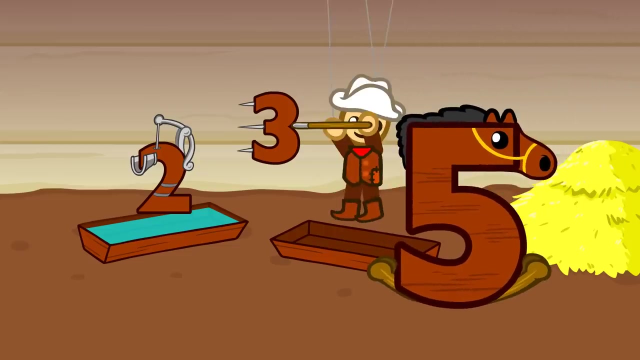 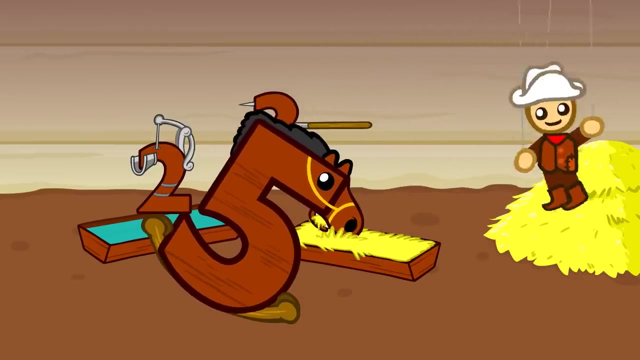 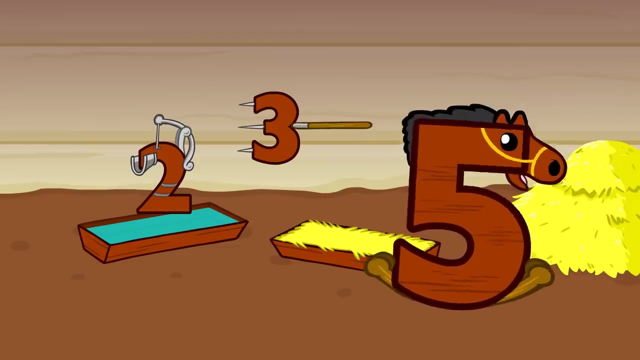 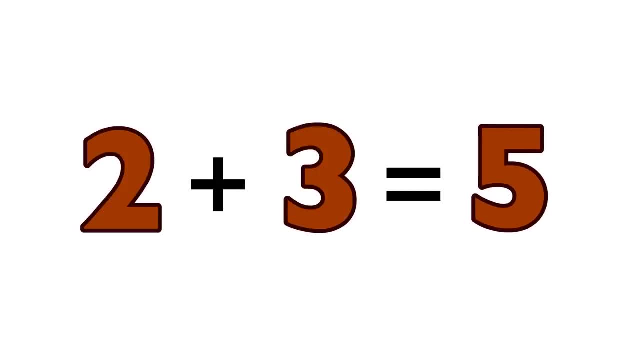 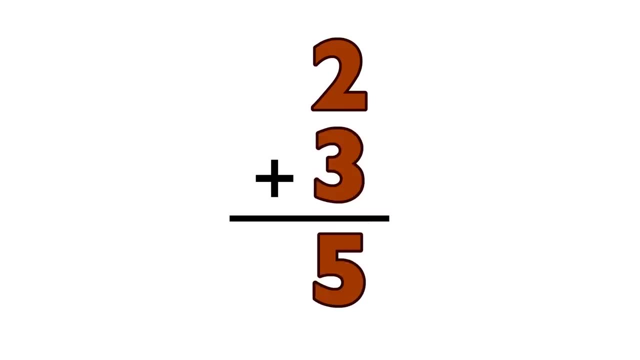 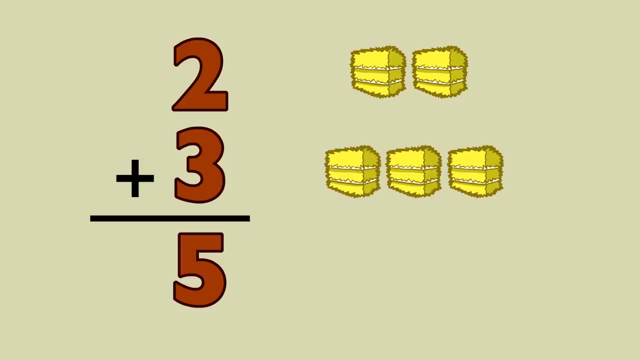 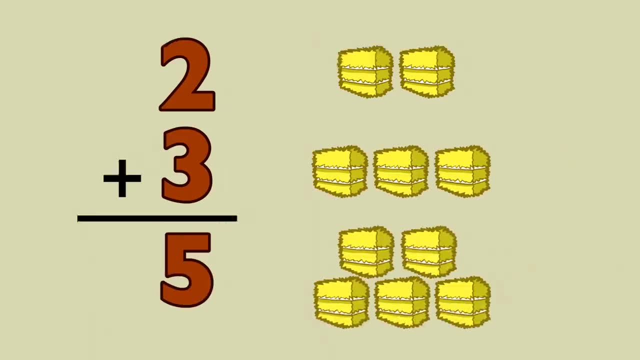 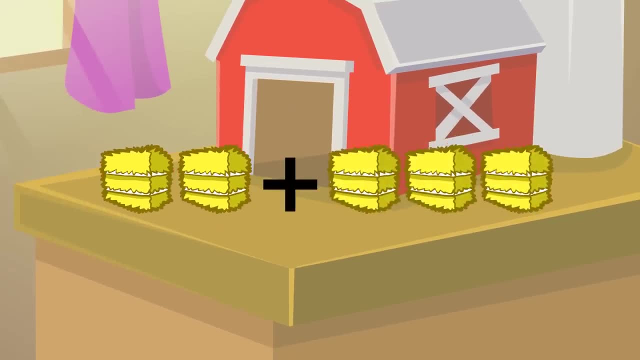 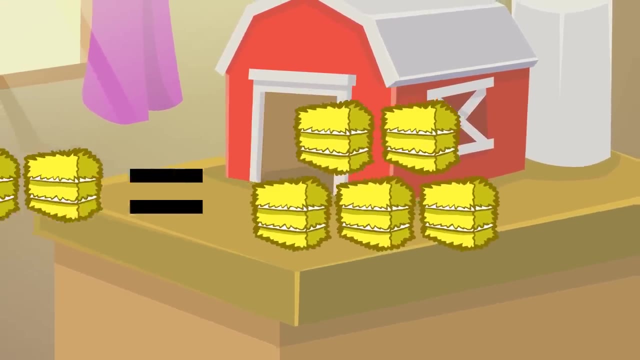 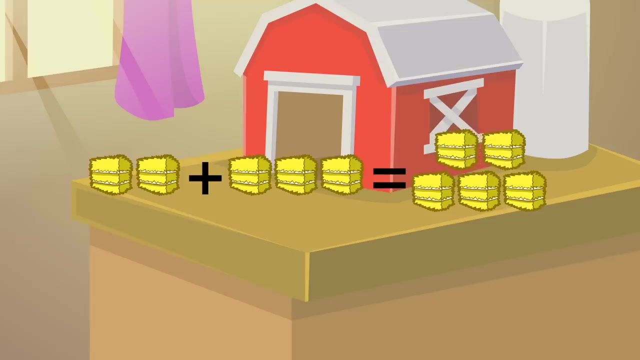 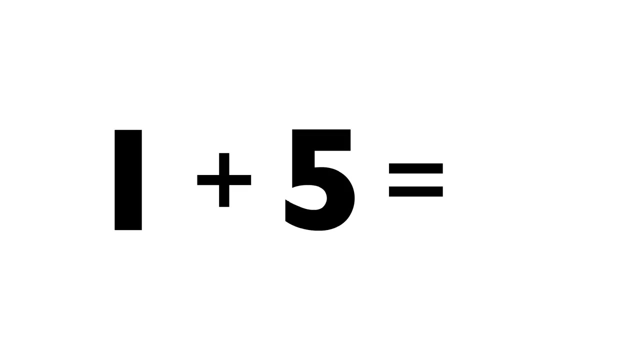 Two plus three equals five. 2 plus 3 equals 5.. 1, 2, 3, 4, 5 equals 1, 2, 3, 4, 5.. 1 plus 5 equals, 1 plus 5 equals 6.. 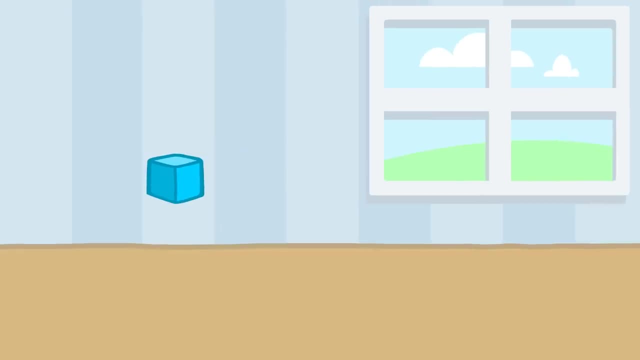 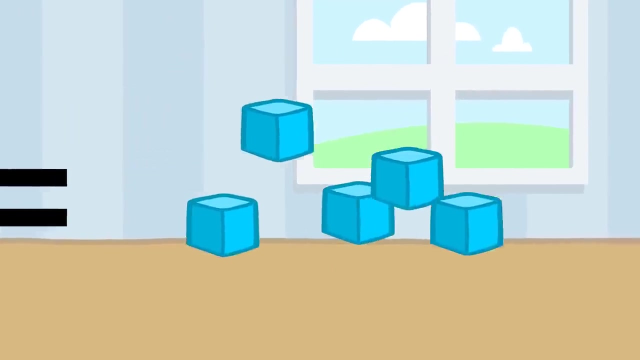 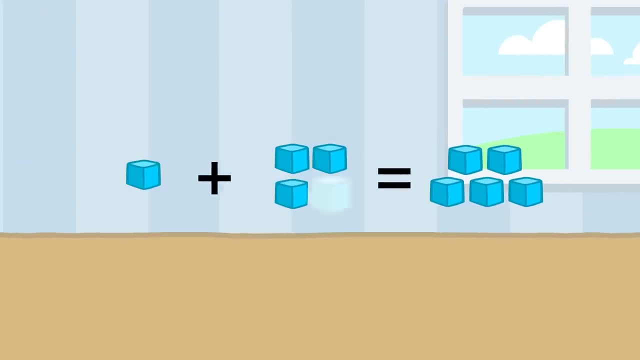 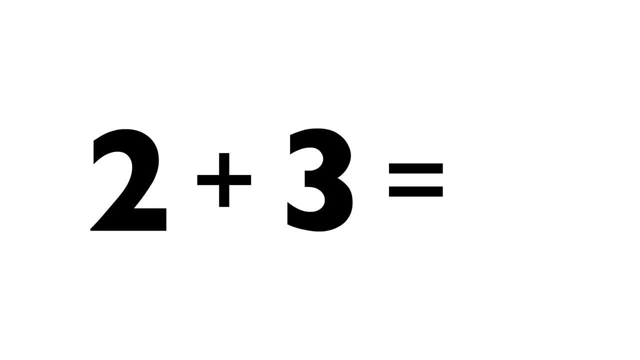 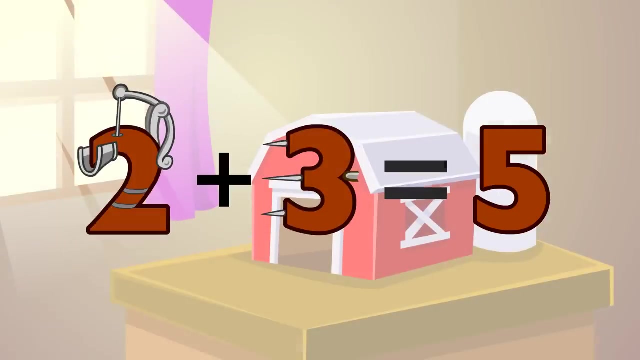 plus four equals five. One plus four equals five plus four equals five. one, two, three, four, five equals one, two, three, four. five two plus three equals. two plus three equals five. two plus three equals. 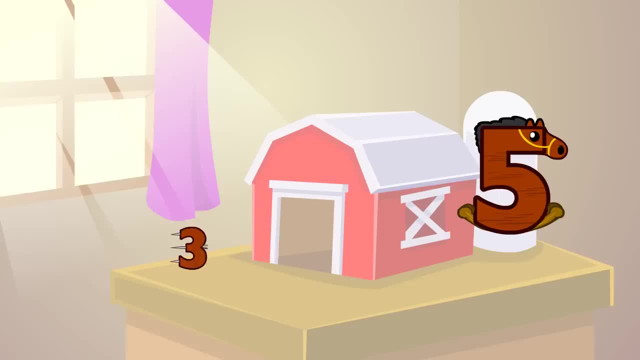 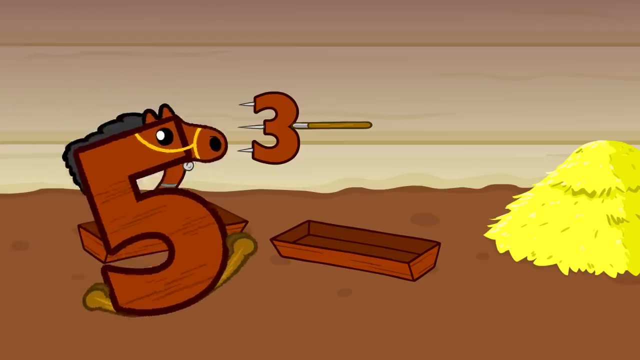 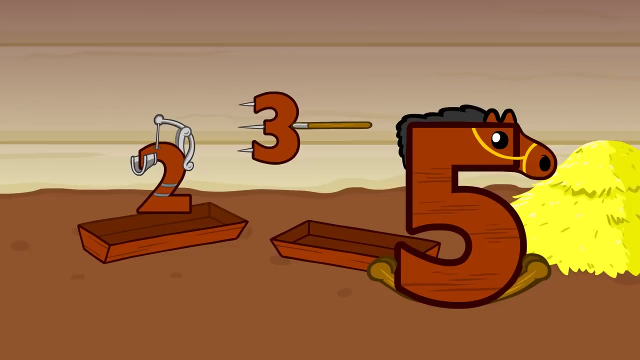 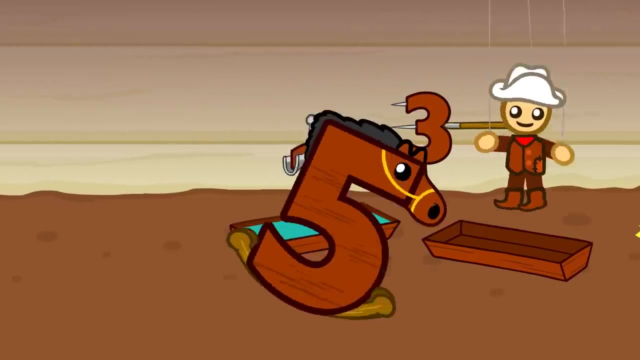 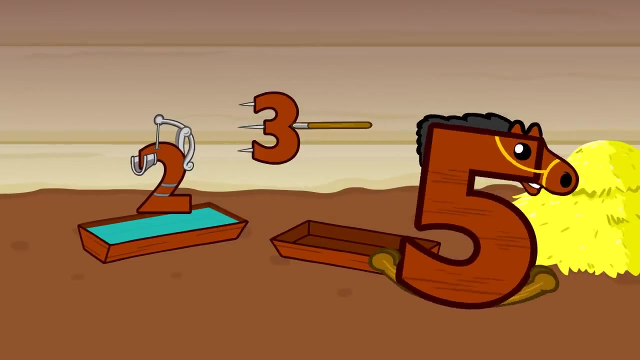 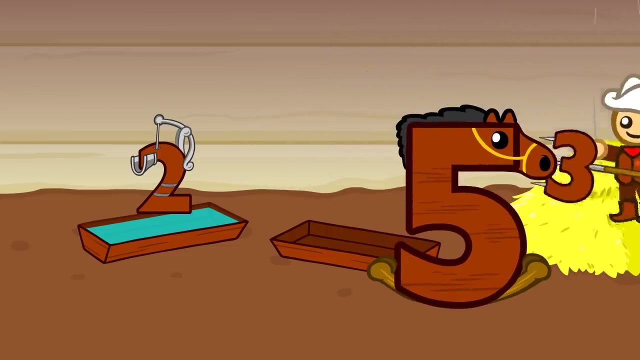 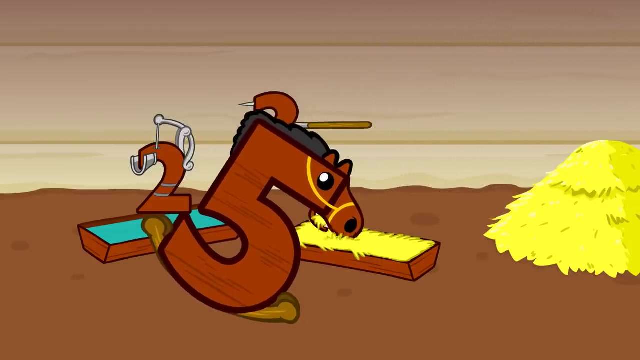 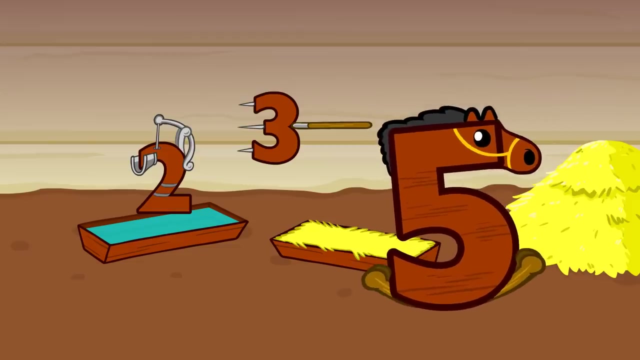 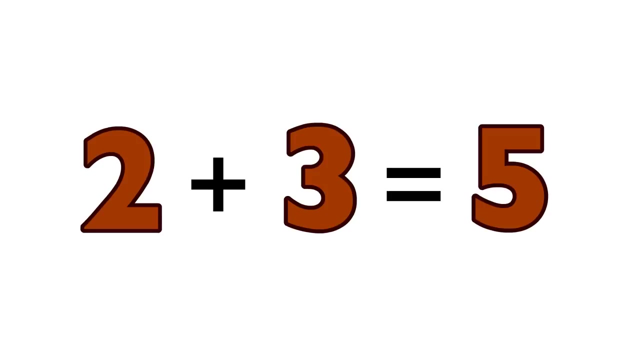 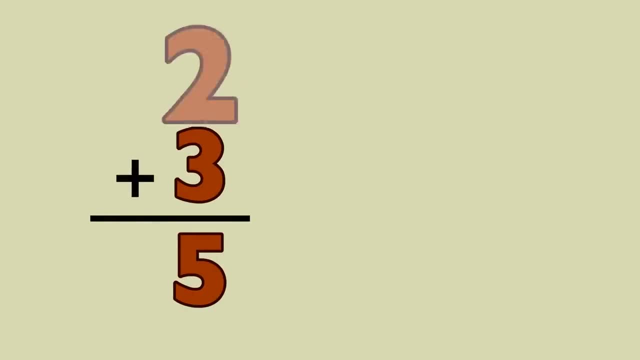 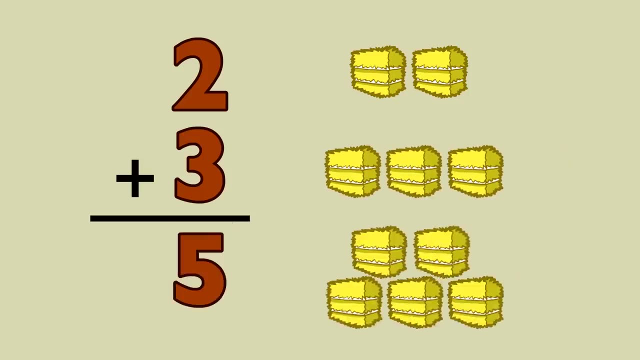 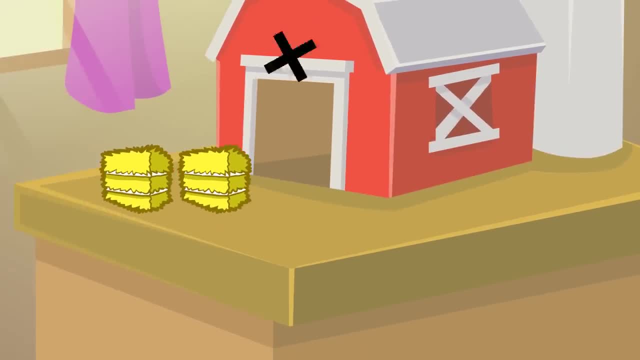 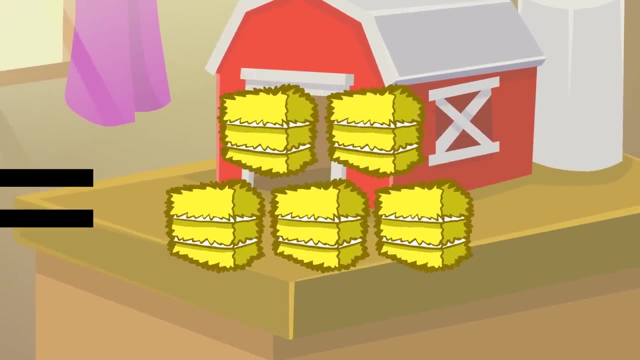 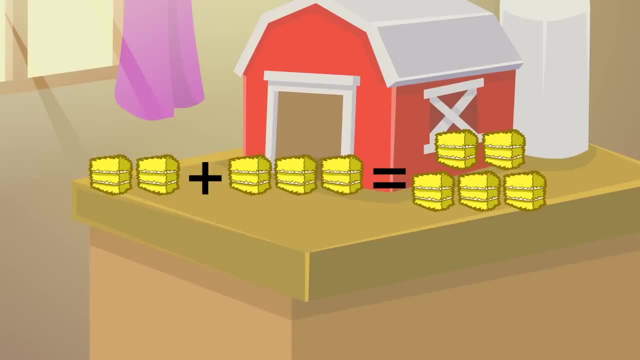 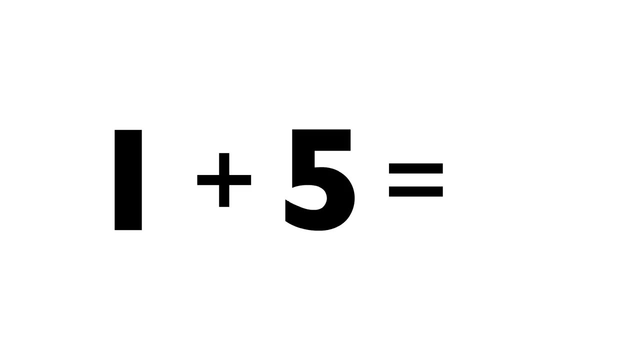 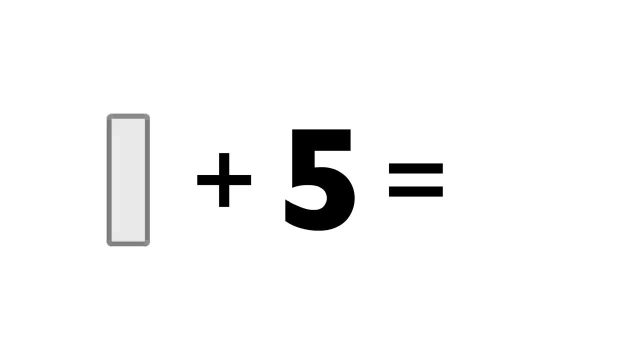 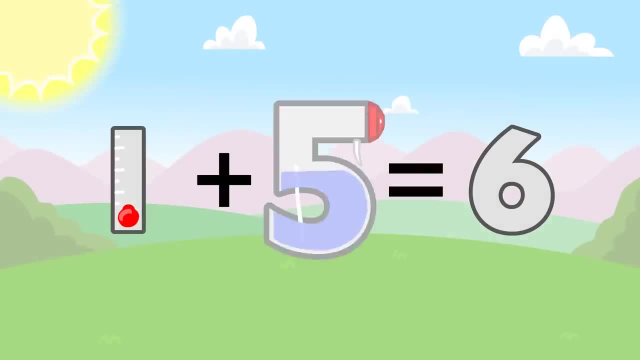 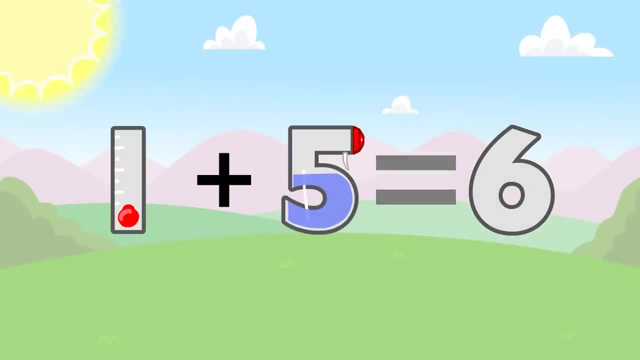 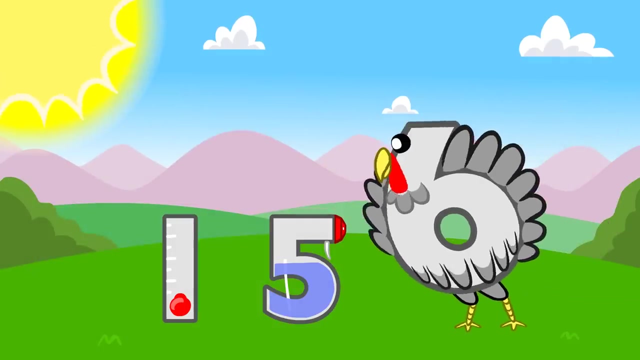 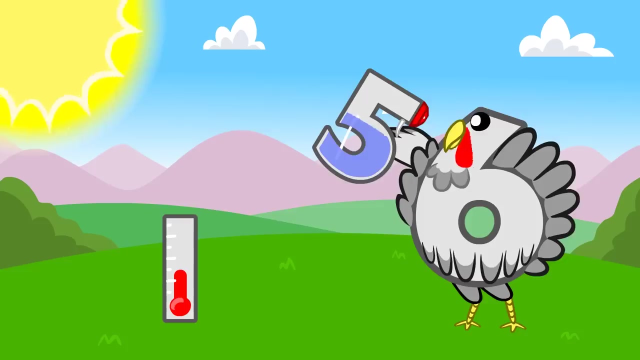 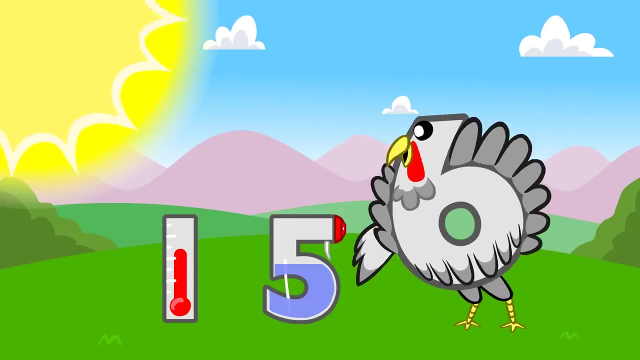 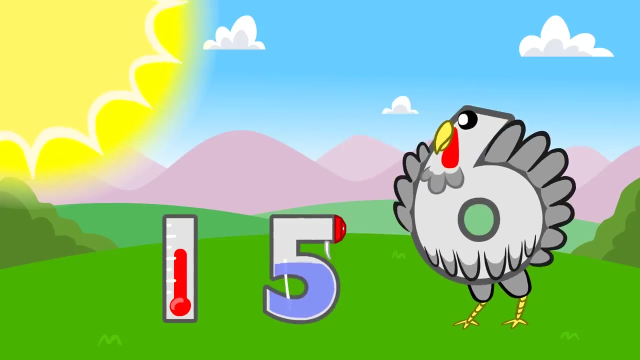 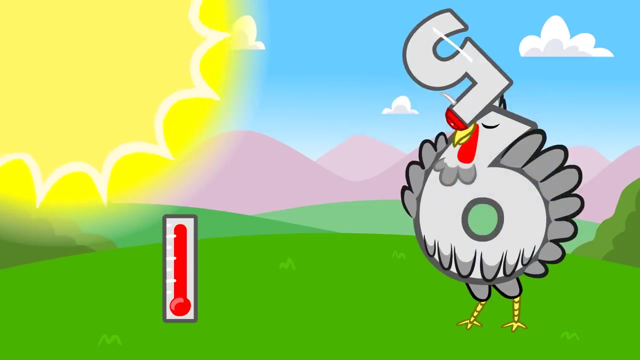 1 plus 5 equals 6.. 1 plus 5 equals 6.. 1 plus 5 equals 6.. 1,, 2,, 3, 4, 5 equals 1,, 2,, 3,, 4, 5.. 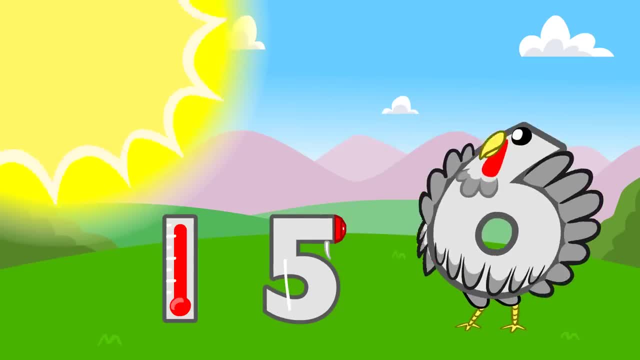 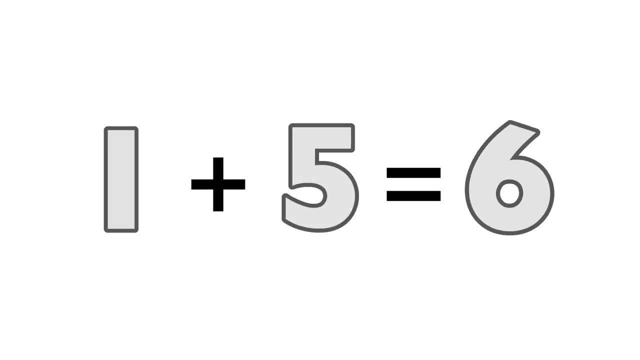 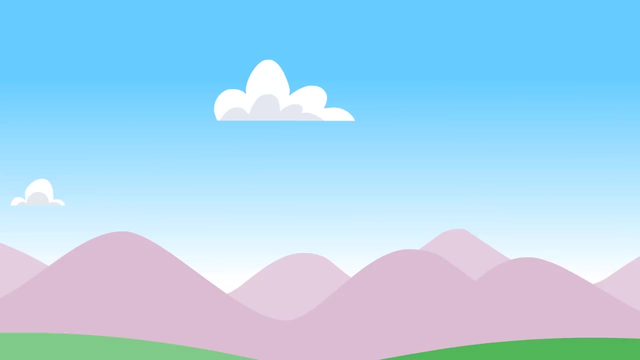 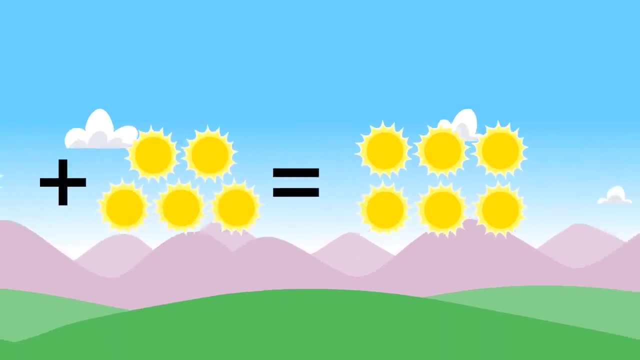 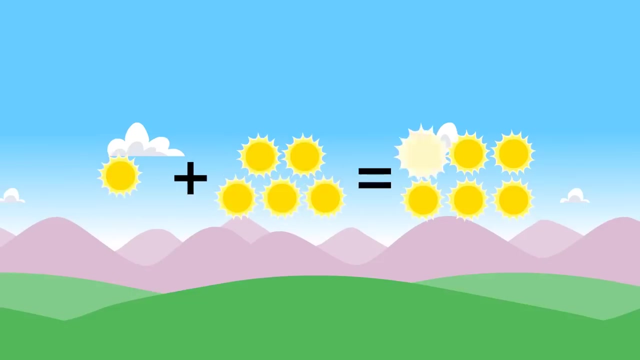 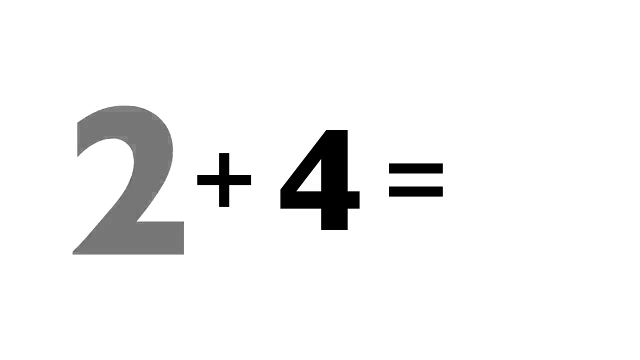 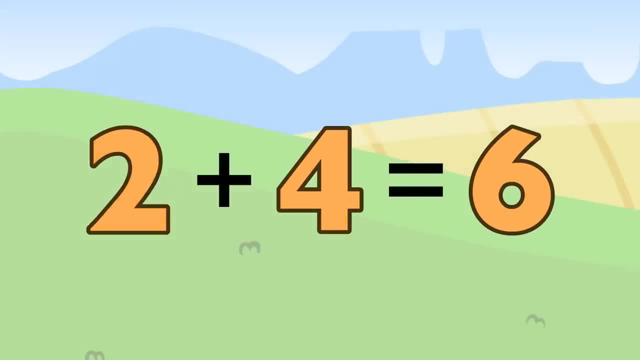 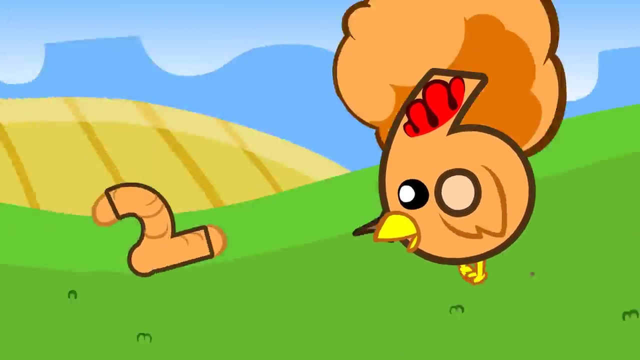 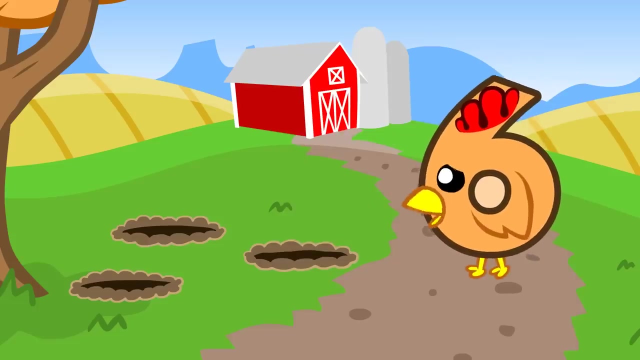 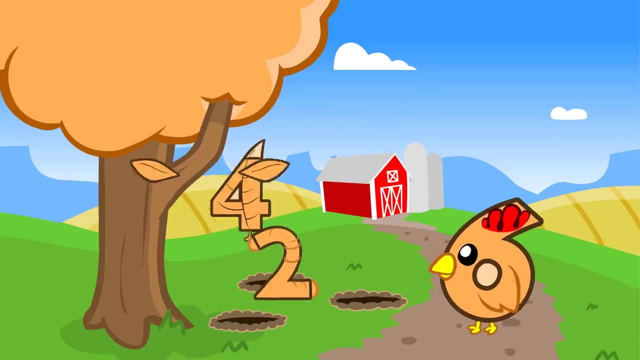 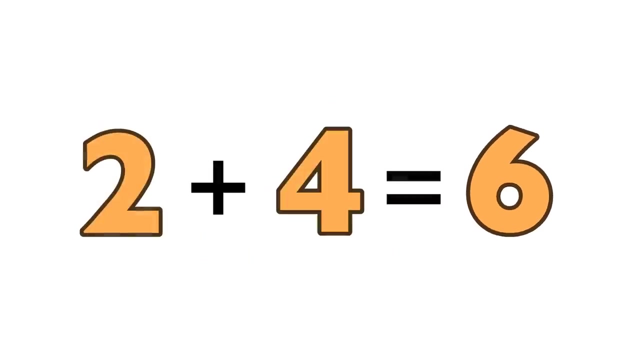 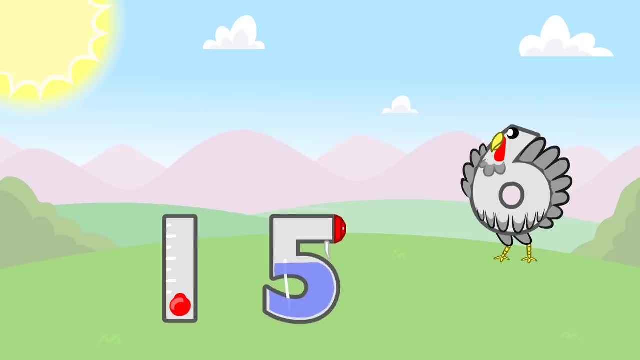 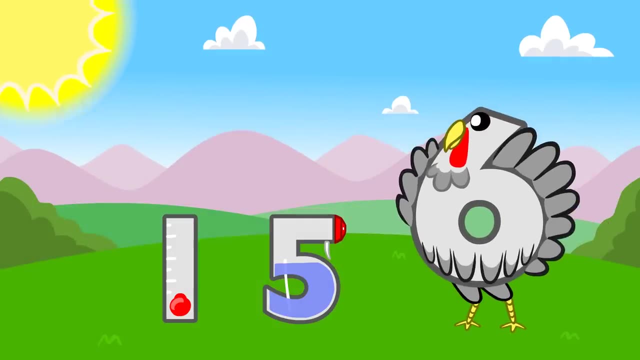 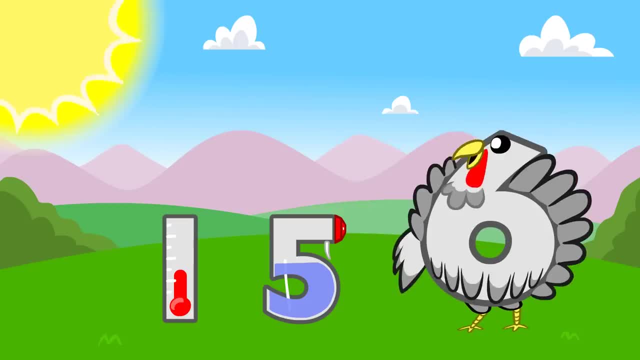 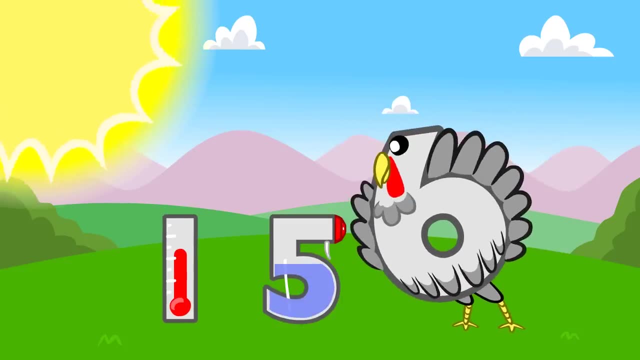 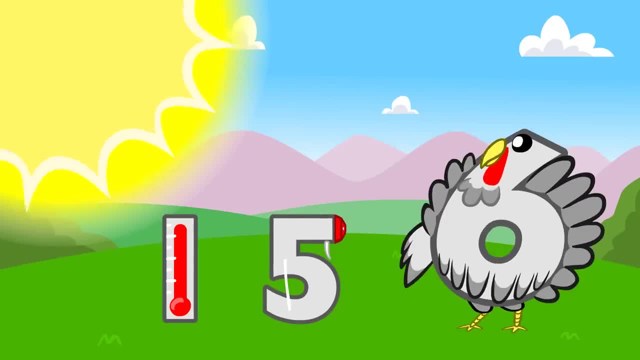 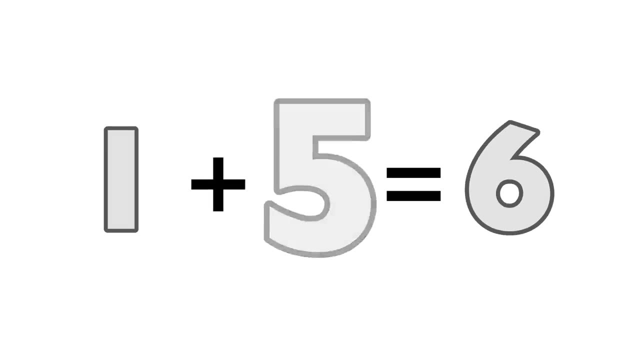 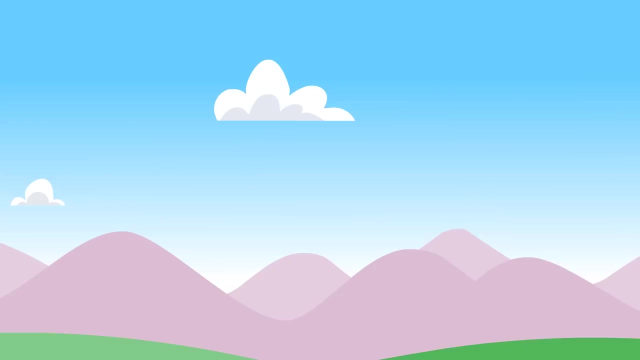 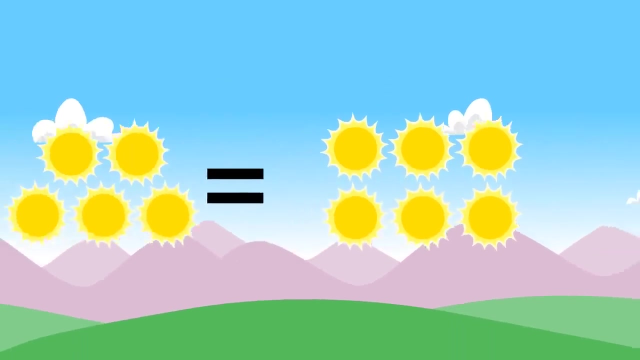 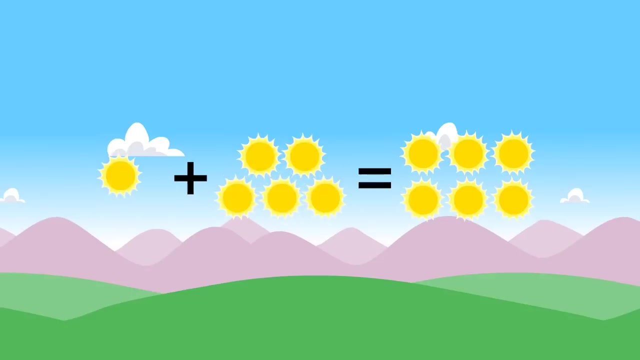 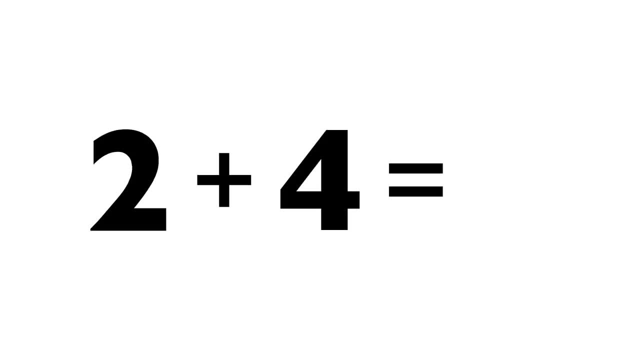 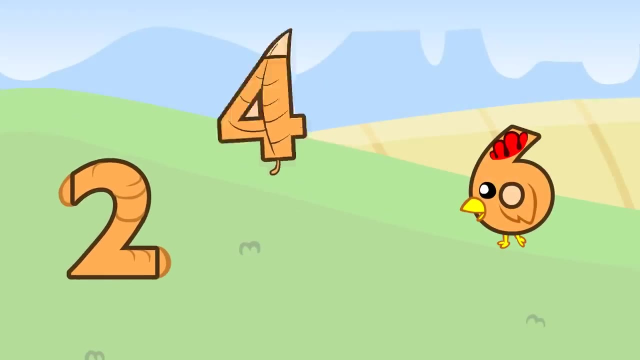 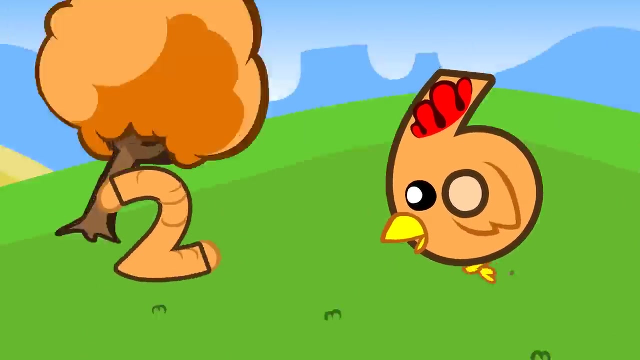 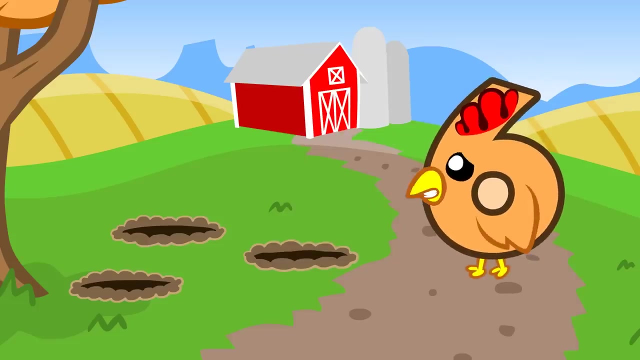 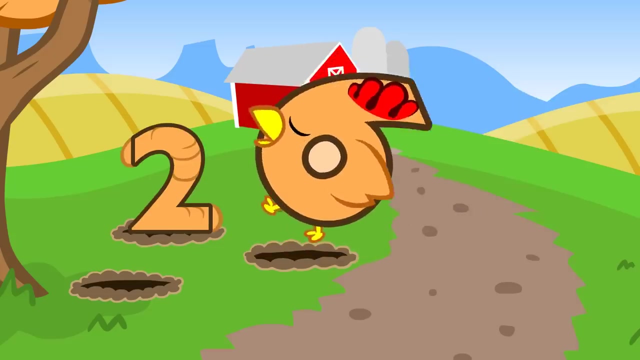 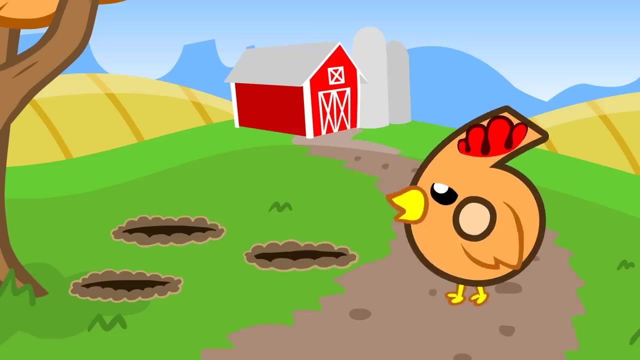 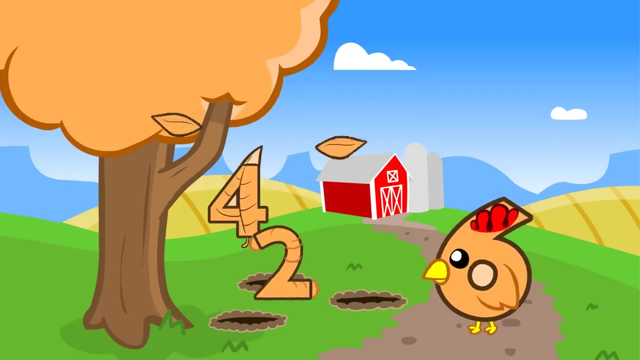 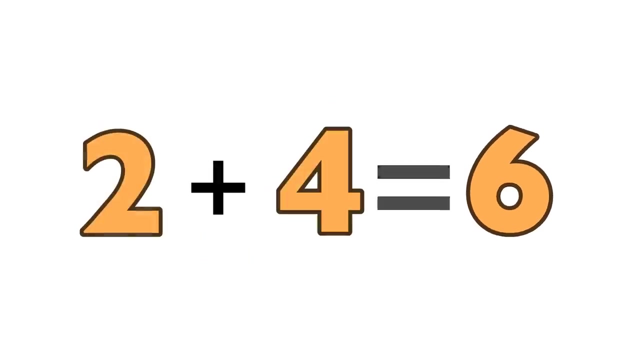 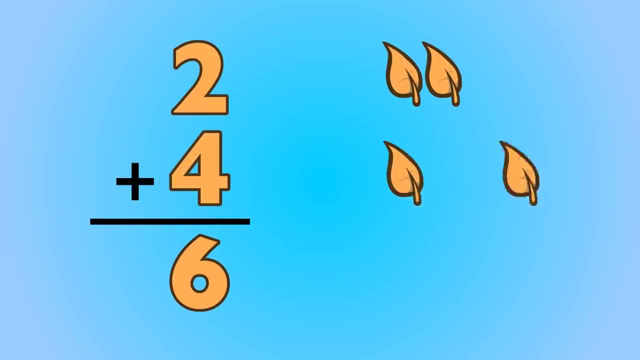 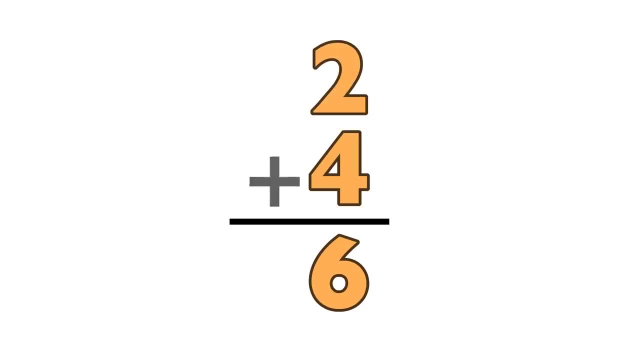 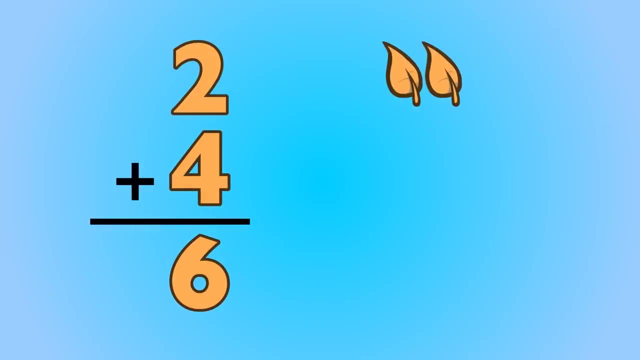 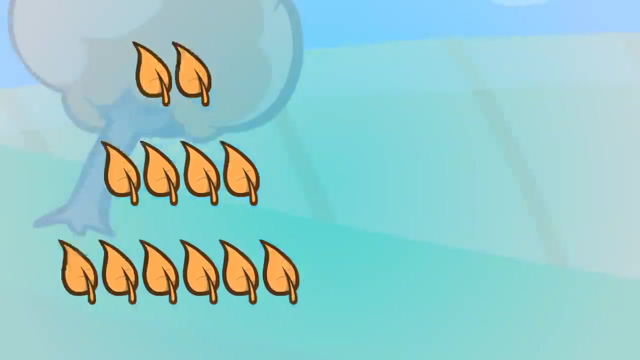 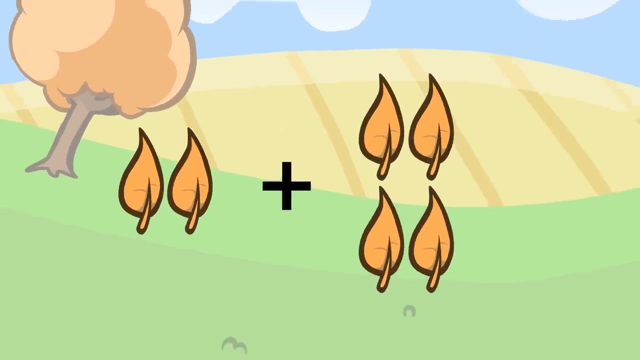 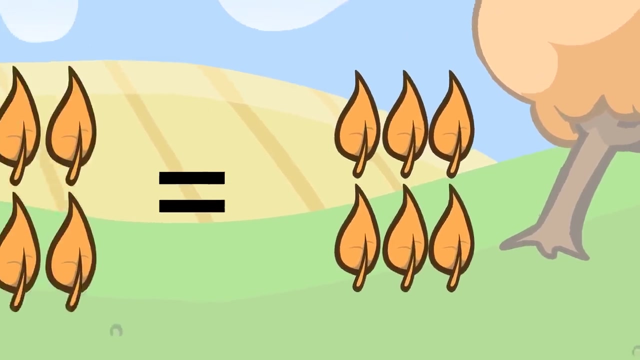 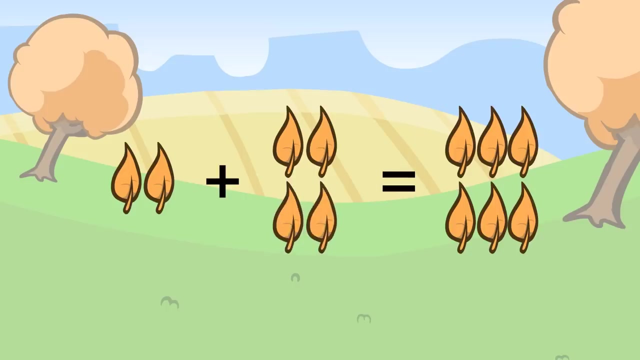 2 plus 4 equals 6.. 2 plus 4 equals 6.. 2 plus 4 equals 6.. 1,, 2,, 3,, 4, 5, 6 equals 1,, 2,, 3,, 4,, 5, 6.. 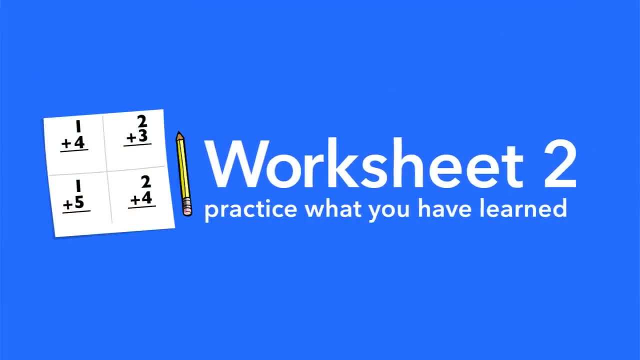 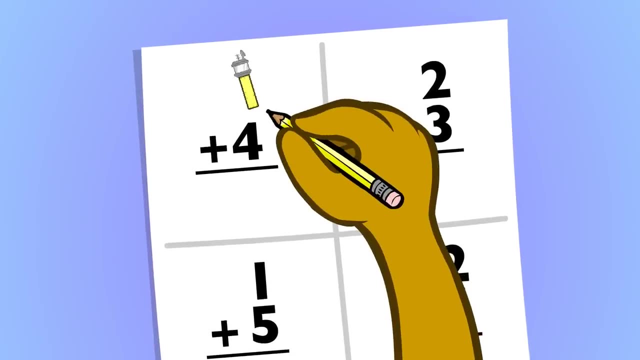 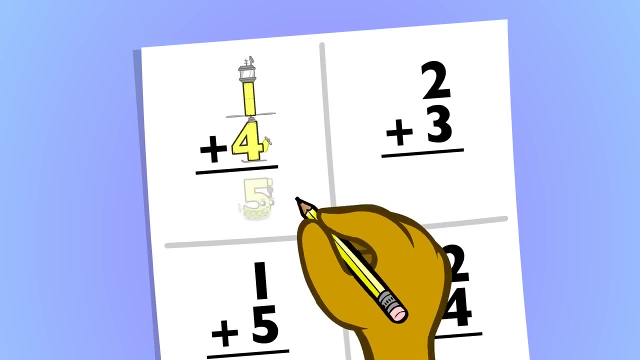 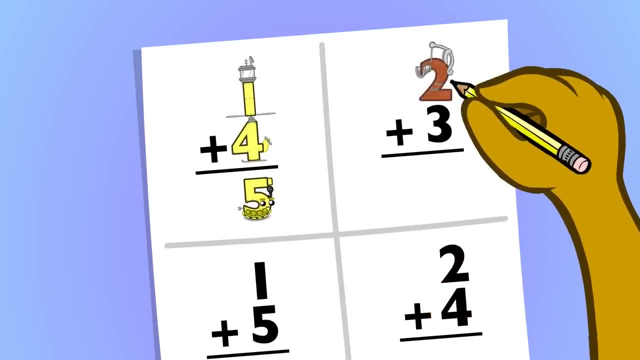 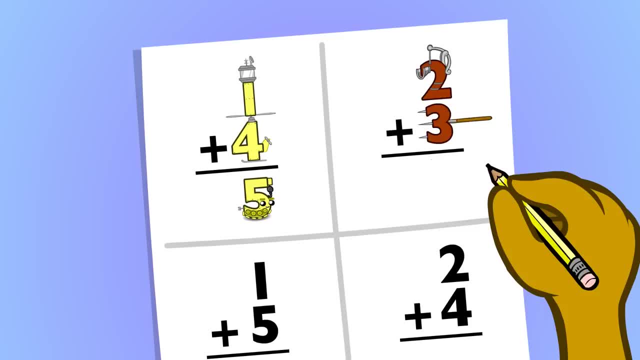 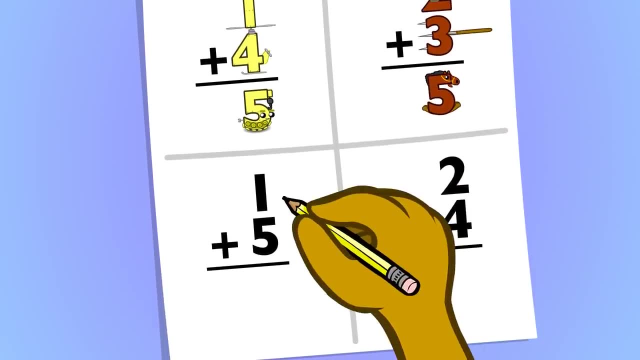 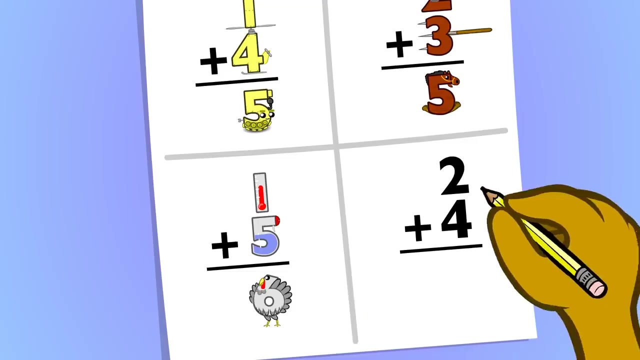 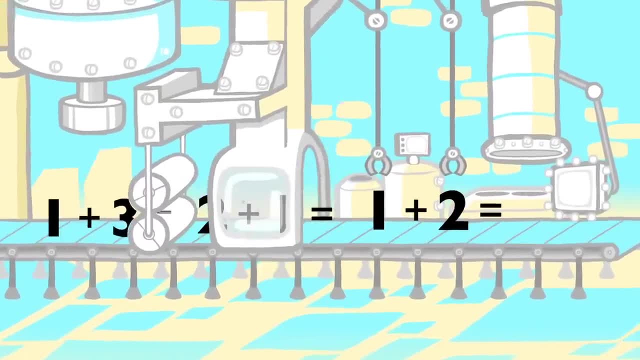 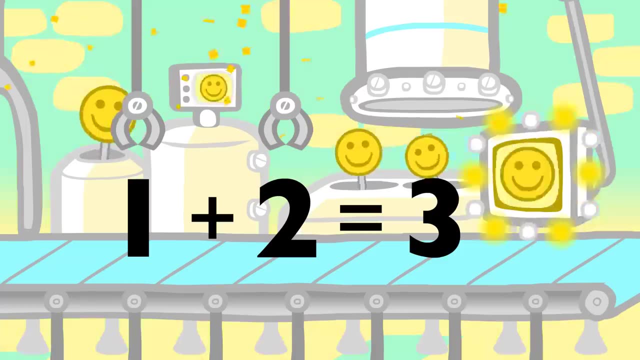 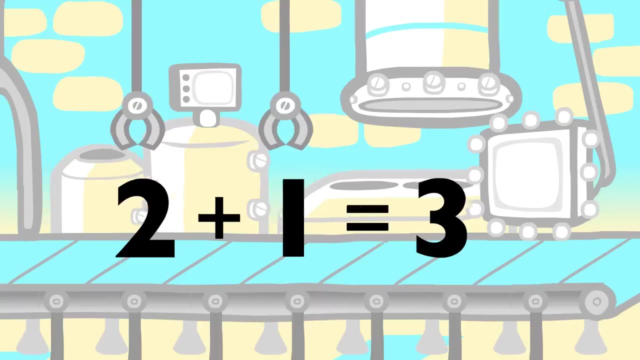 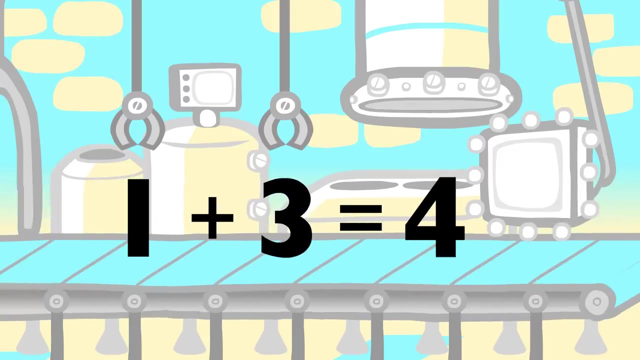 1 plus 2 equals 3.. And 2 plus 1 equals 3.. 1 plus 3 equals 4.. And 3 plus 3 equals 4.. 1 equals 4.. 1 plus 4 equals 5.. 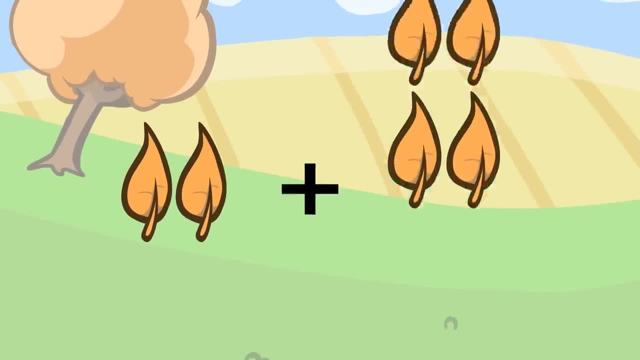 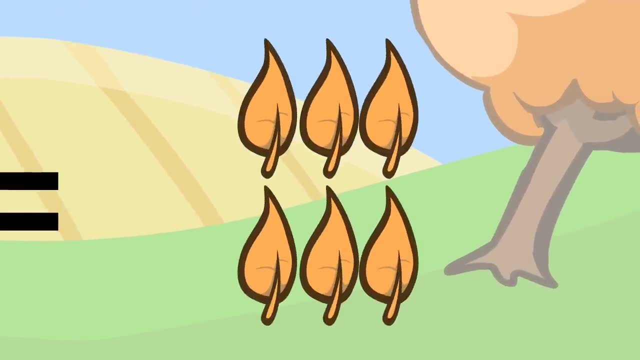 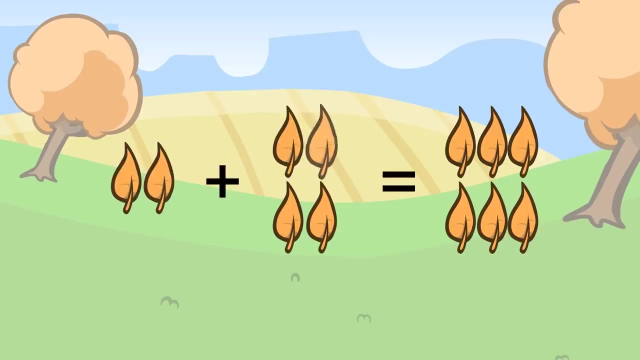 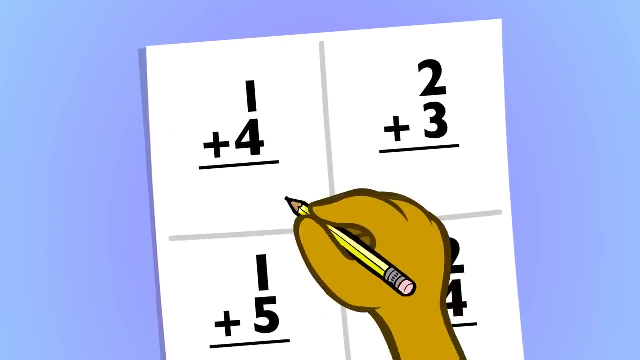 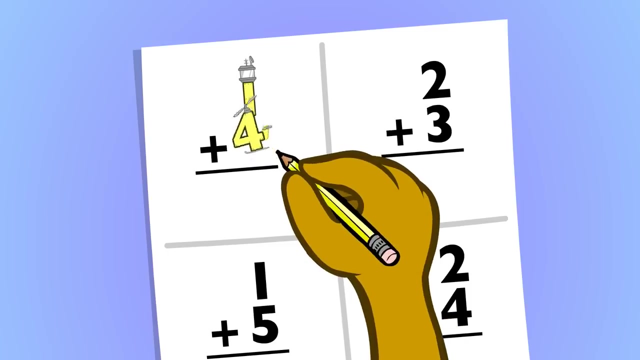 Two plus four equals six. Two plus four equals six. Two plus four equals six. One, two, three, four, five. six equals one, two, three, four, five, six. One plus four equals six, Plus four equals five. 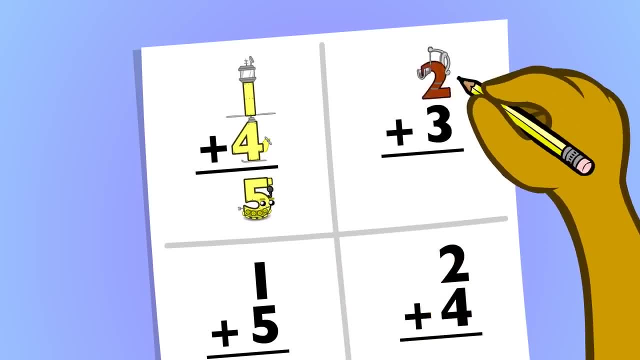 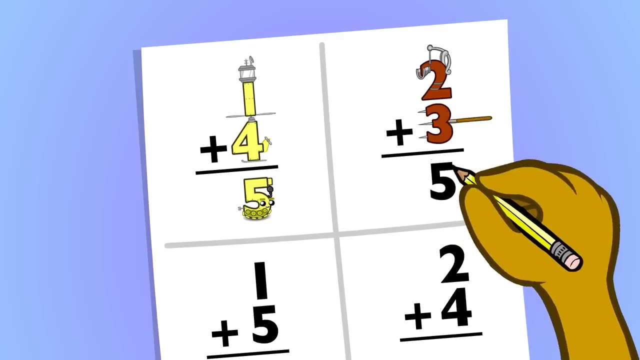 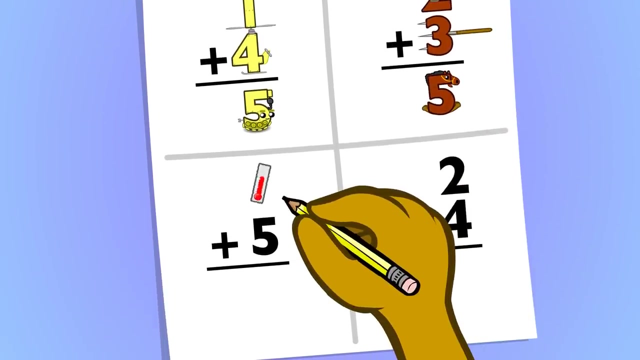 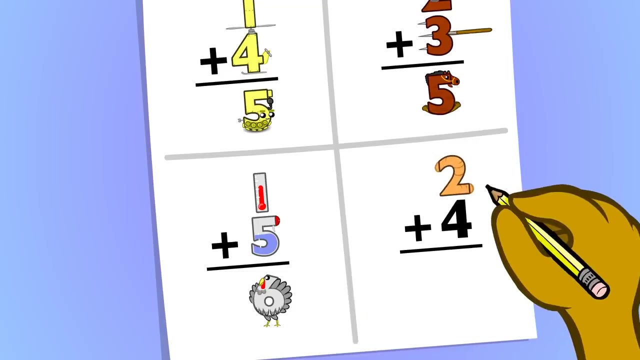 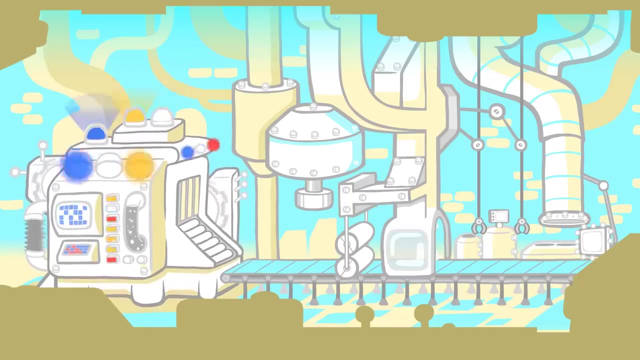 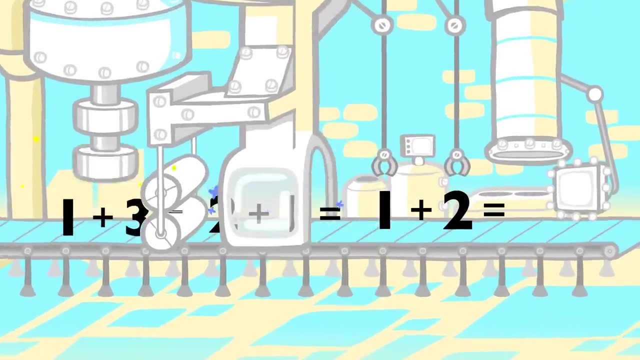 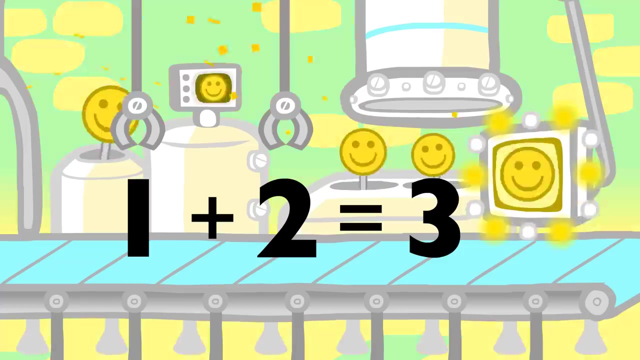 Two plus three equals six. 5. 1 plus 5 equals 6. 2 plus 4 equals 6. 1 plus 2 equals 3, and 2 plus 1 equals 3. 1 plus 3 equals 4 and 3. 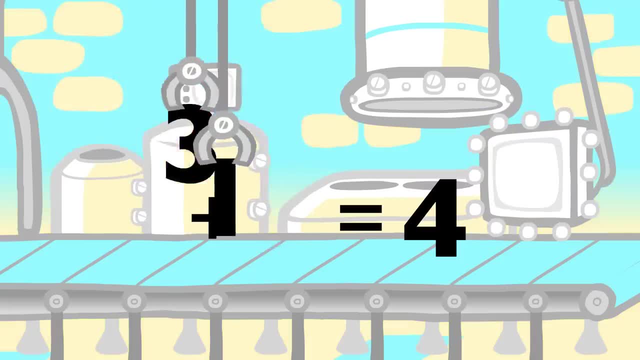 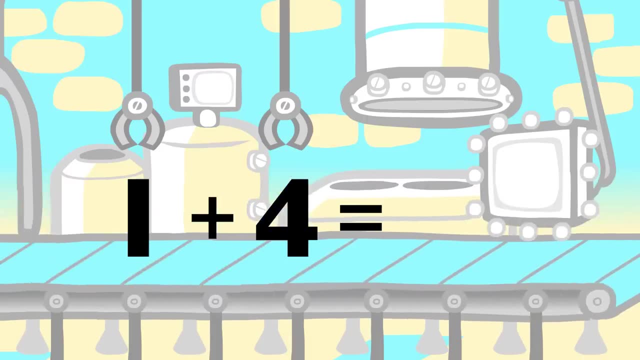 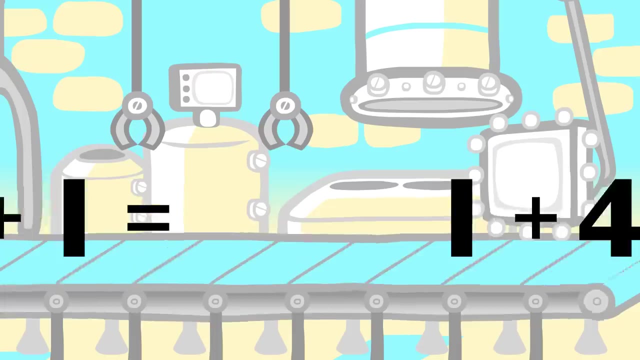 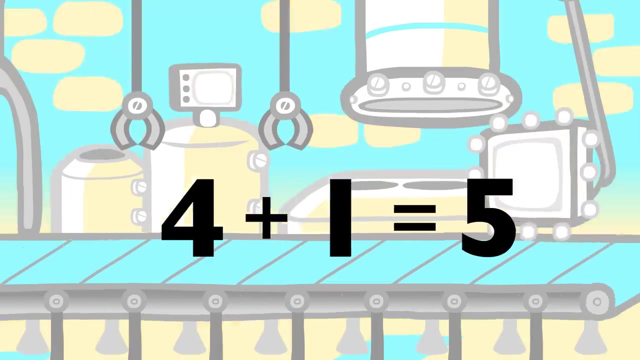 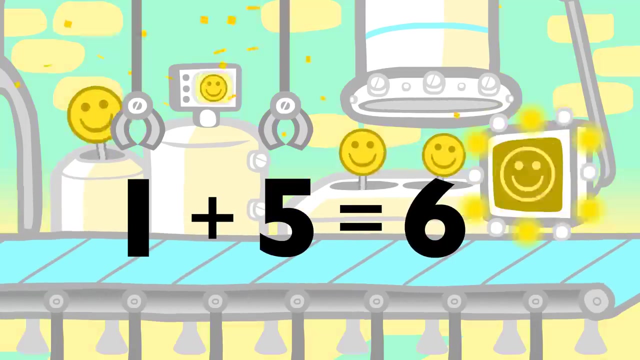 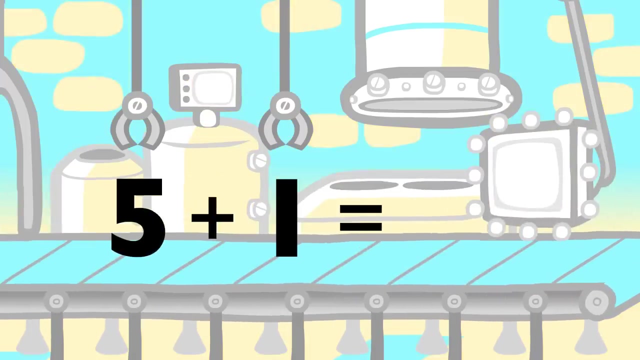 plus 1 equals 4, and 3 plus 1 equals 4, 1 plus 4 equals 5, and 4 plus 1 equals 5, 1 plus 5 equals 6, and 5 plus 1 equals 6 and 5. 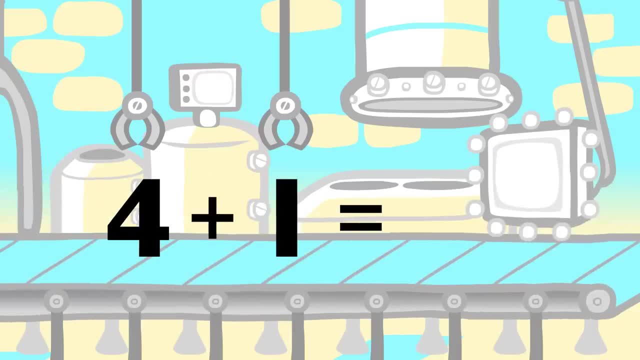 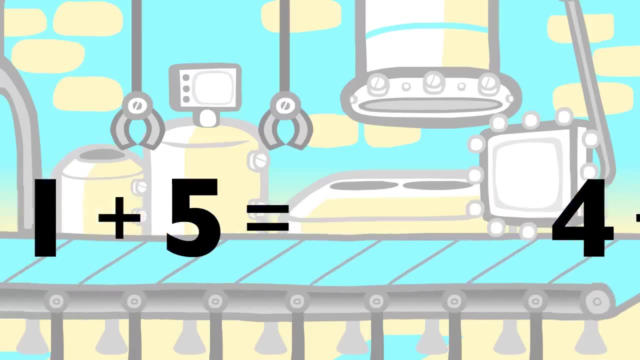 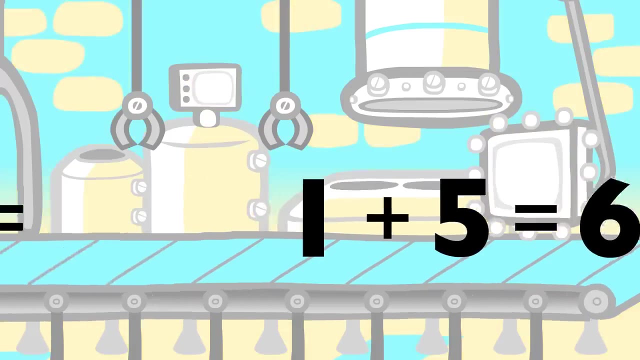 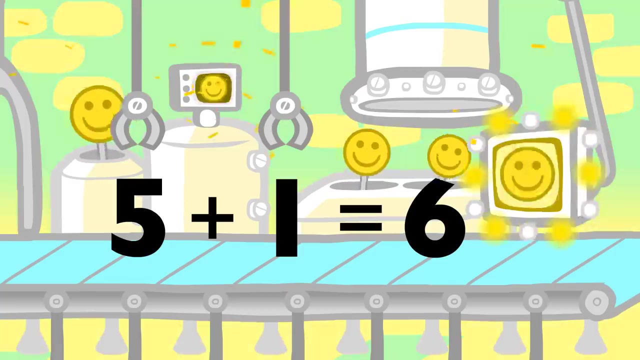 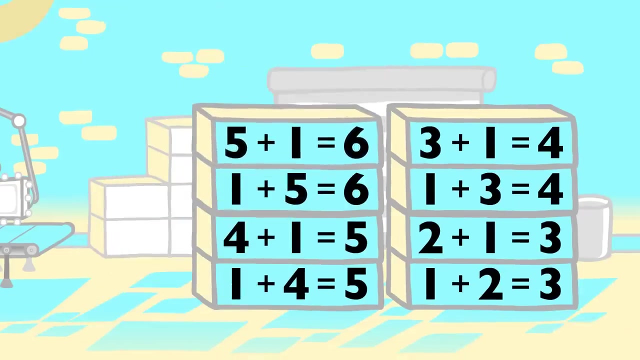 And 4 plus 1 equals 5.. 1 plus 5 equals 6. And 5. Plus 1 equals 6. And 5. And 6. And 7. And 8. And 9. And 10.. 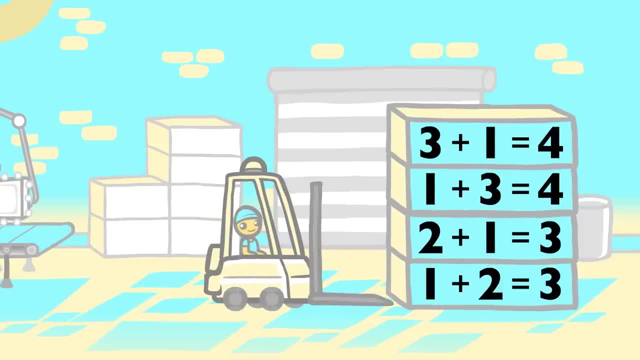 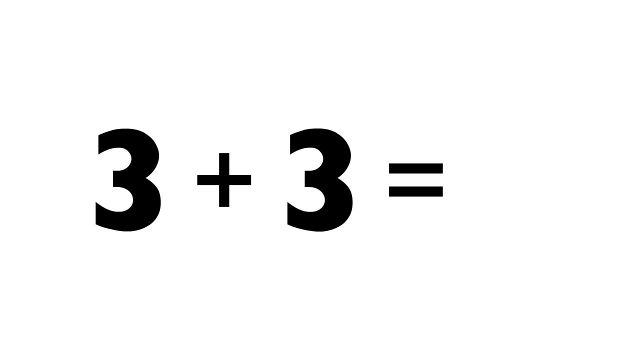 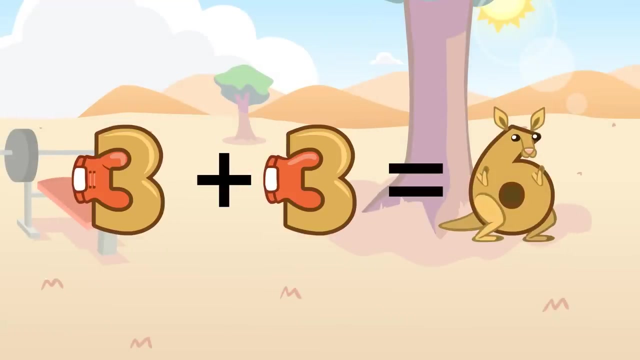 And 11. And 12. And 13. And 14. And 15. And 16. And 17. And 18. And 19. And 20. And 21. And 21. And 22.. And 23. And 24. And 25. And 26. And 27. And 28. And 29. And 30. And 31. And 32. And 32. And 33. And 34.. 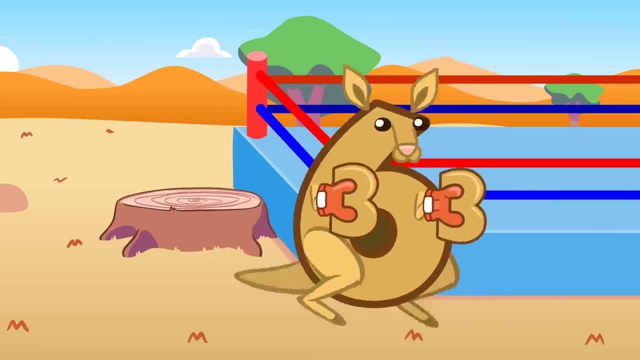 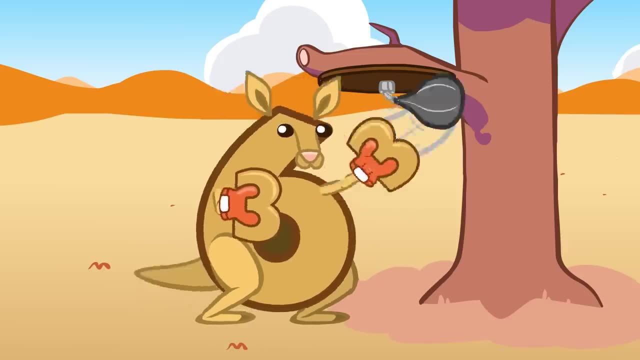 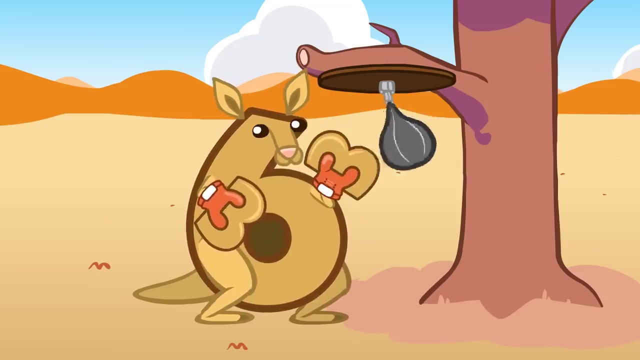 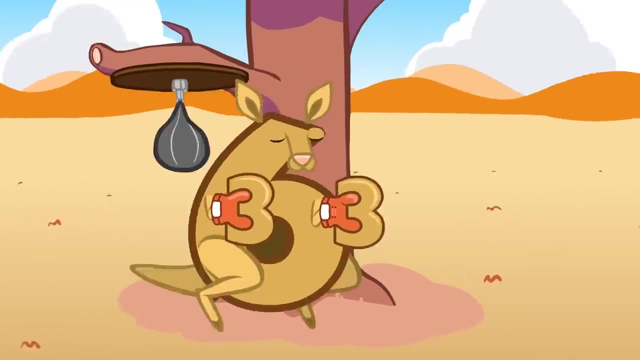 And 34. And 35. And 36. And 37. And 38. And 39. And 40. And 41. And 42. And 42. And 43. And 42. And 43.. 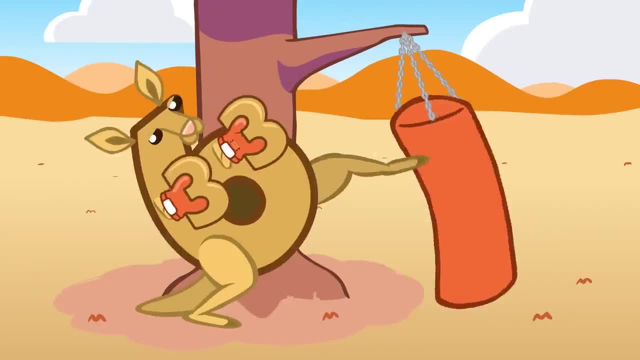 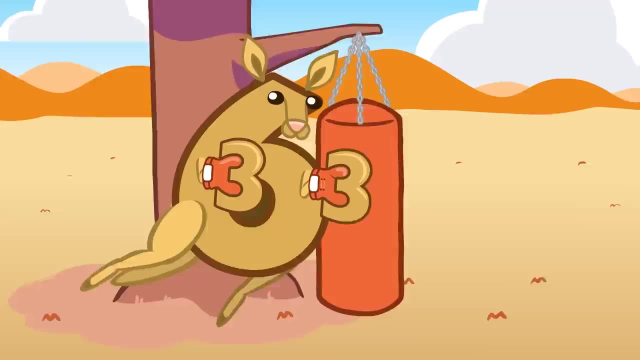 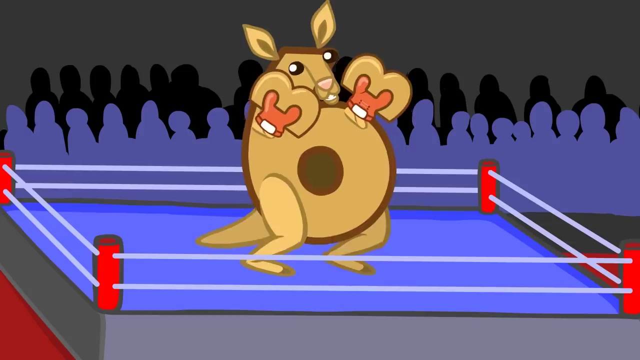 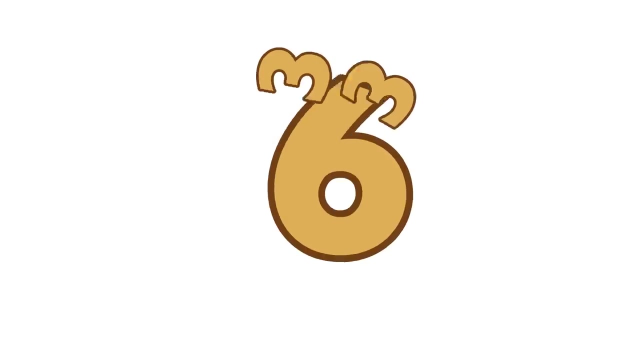 And 44. And 44. And 45. And 46. And 47. And 48. And 49. And 50. And 51. And 52. And 53. And 54. And 55.. 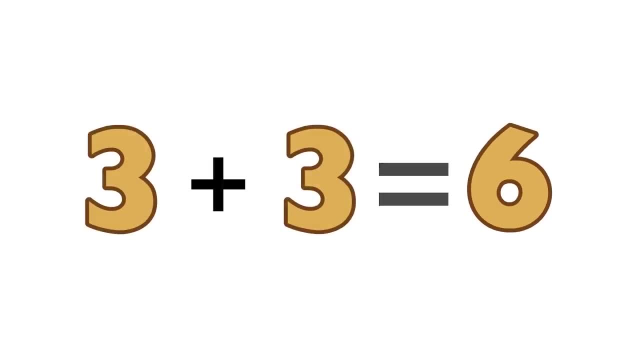 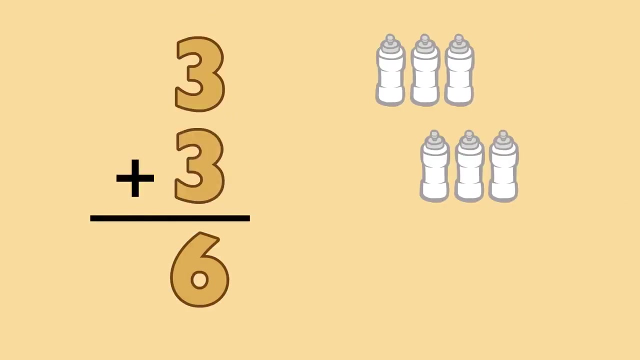 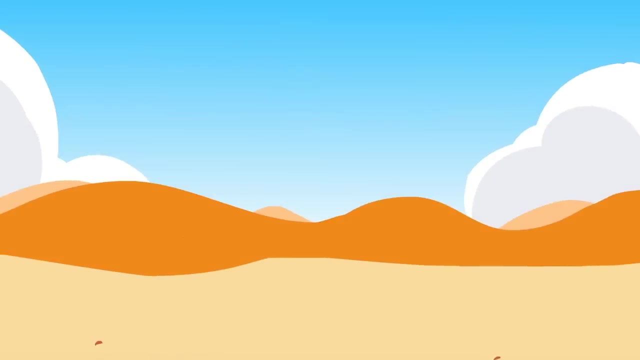 And 56. And 57. And 58. And 59. And 60. And 61. And 62. And 62. And 63. And 63. And 64. And 65. And 66.. 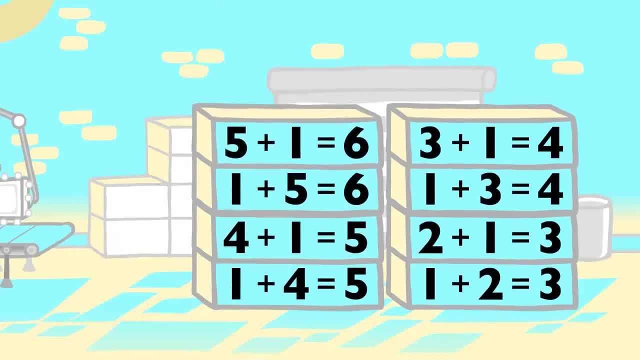 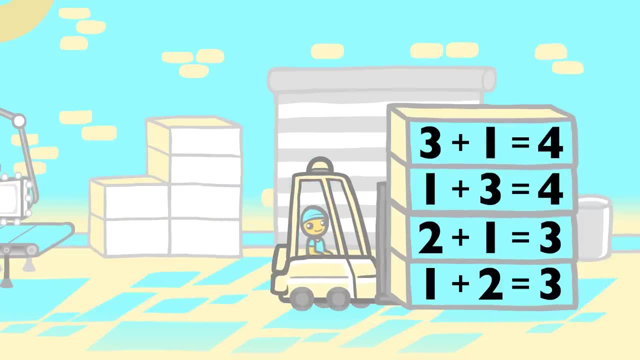 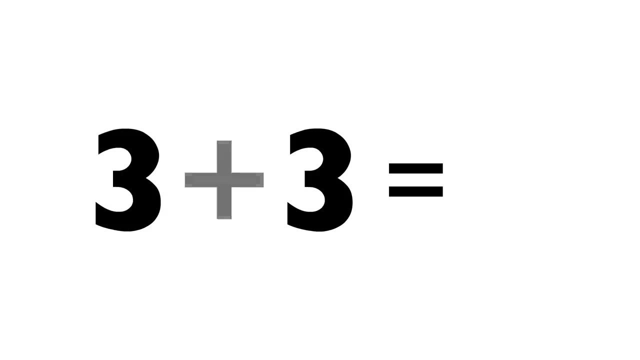 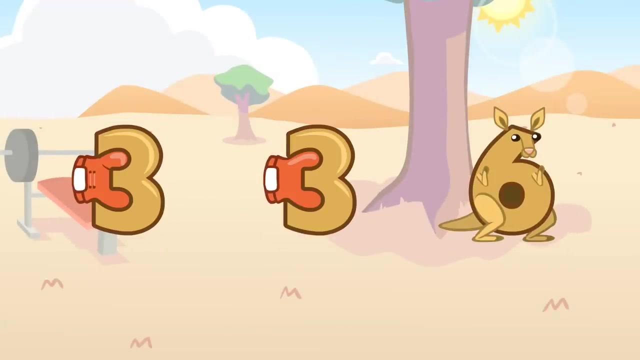 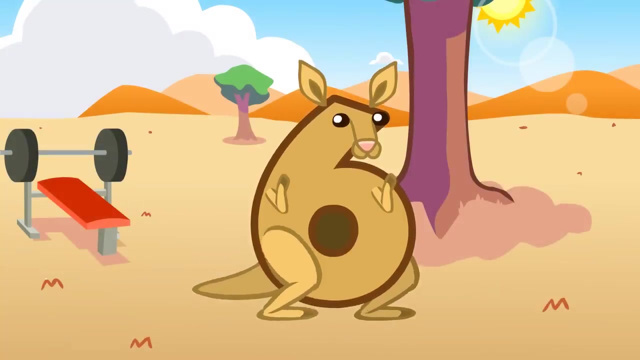 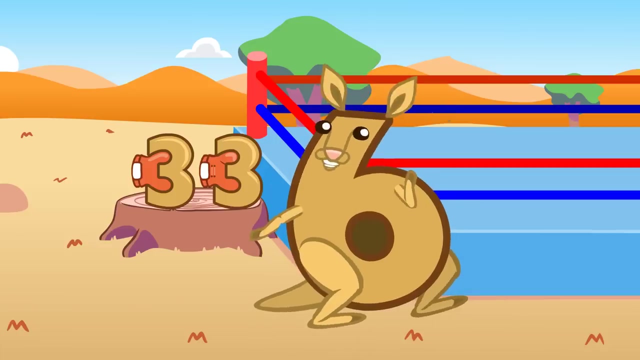 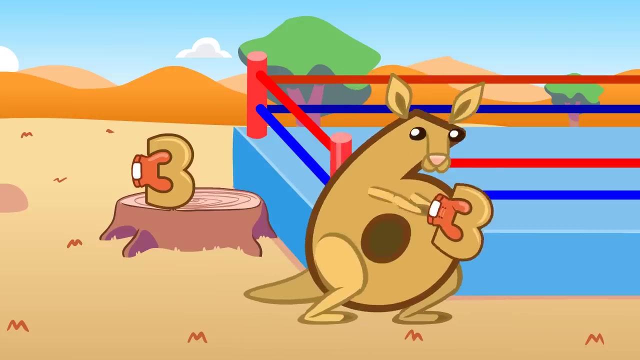 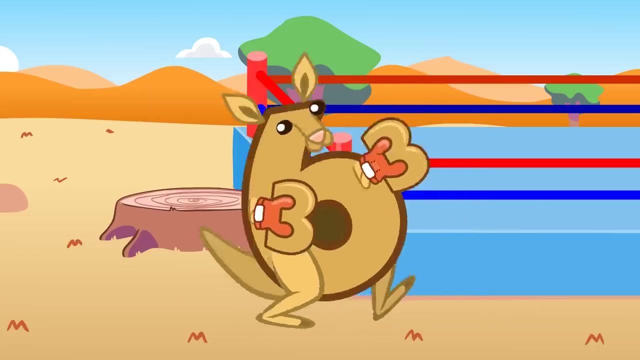 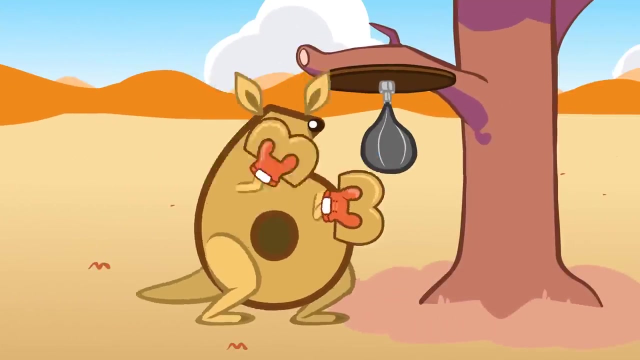 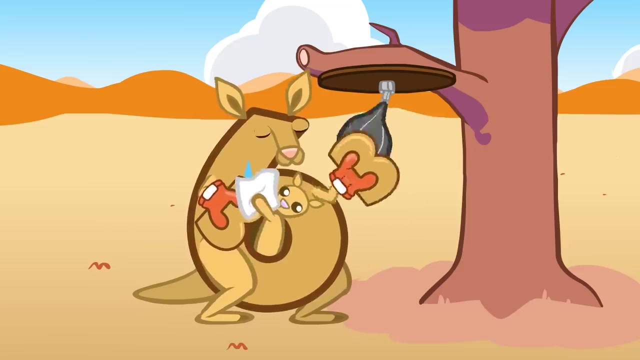 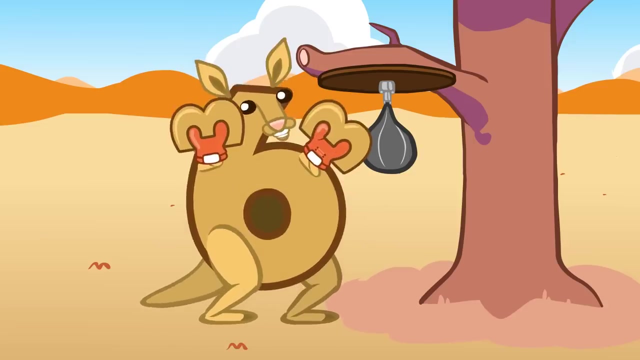 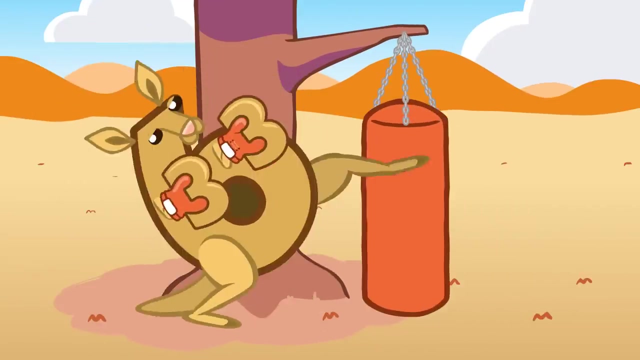 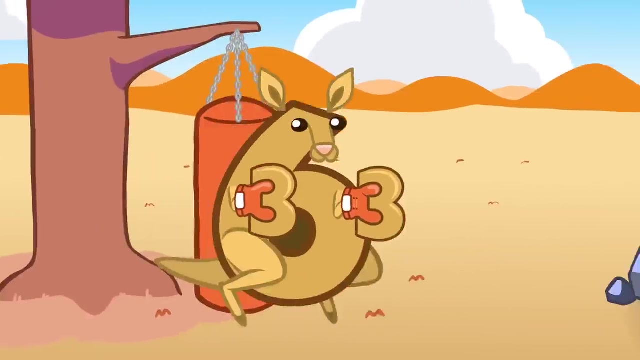 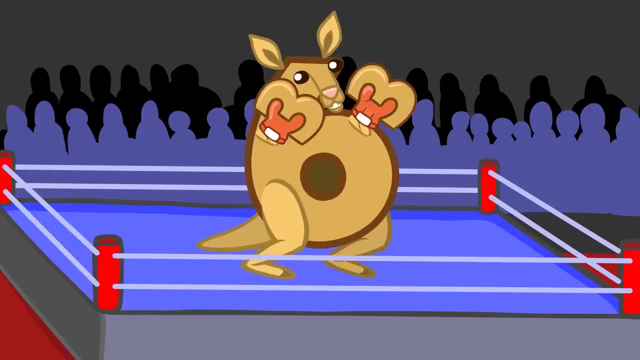 equals 5 plus 3, and 4 plus 5 equals 3 and 5 and 6. or 1 and 3 equals 1: 3. Six, three plus three equals six. Three plus three equals six. Oh, Three plus three equals six. You, Three plus three equals six. 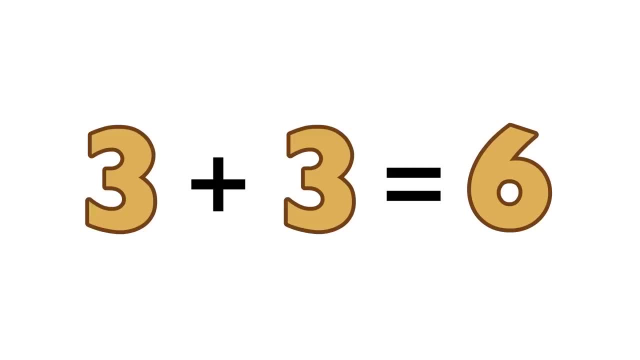 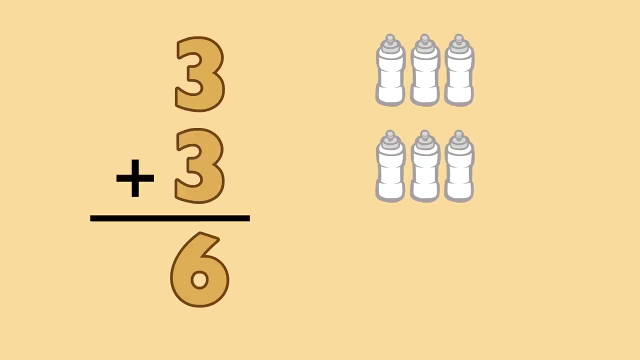 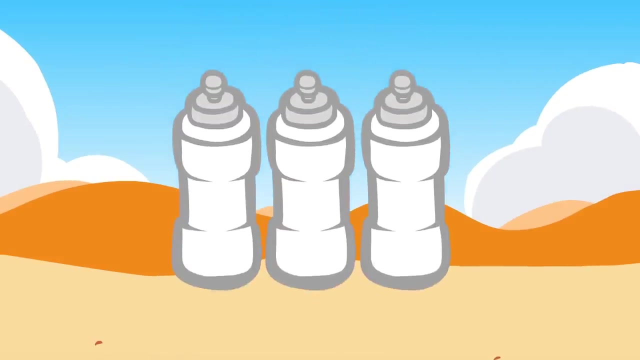 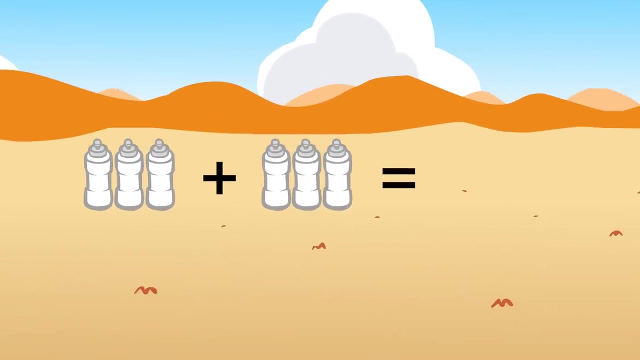 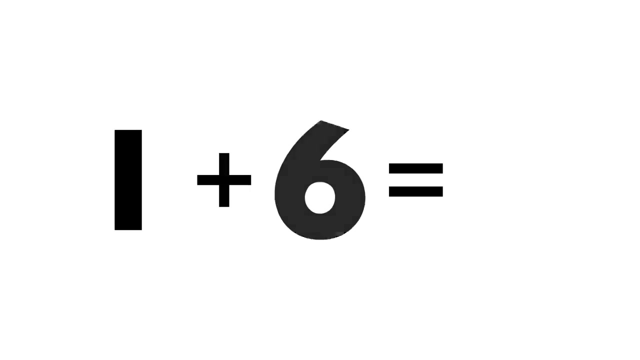 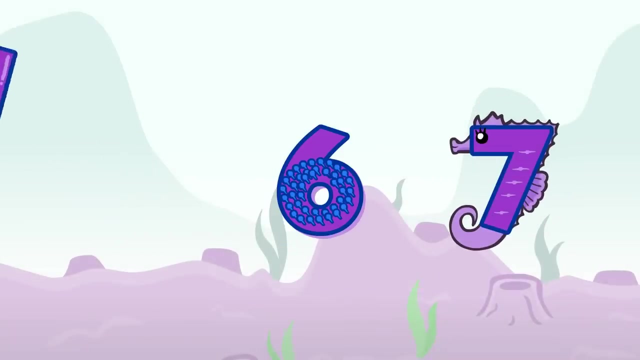 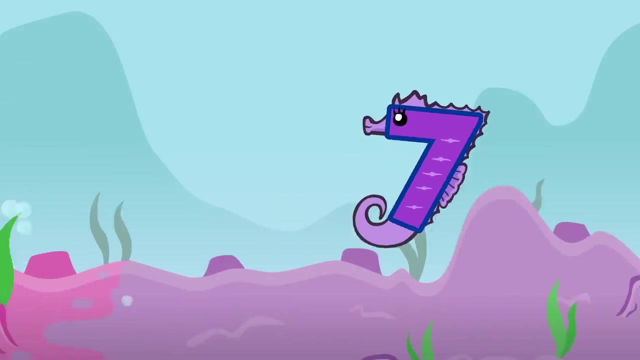 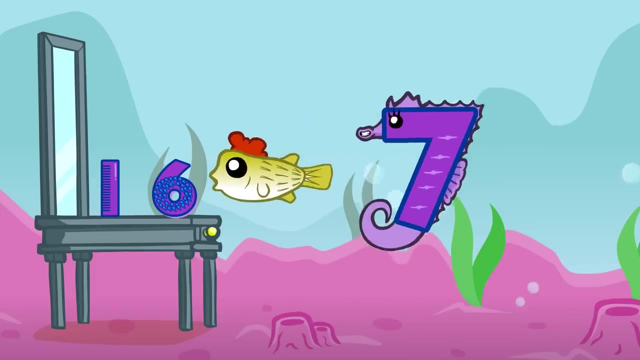 Three plus three equals six. You, Three plus three equals six. Three plus three equals six. Three plus three equals Six. One, two, three, four, five, six equals one, two, three, four, five, six. One plus six equals One plus six equals seven. one plus six equals seven. One plus six equals seven. 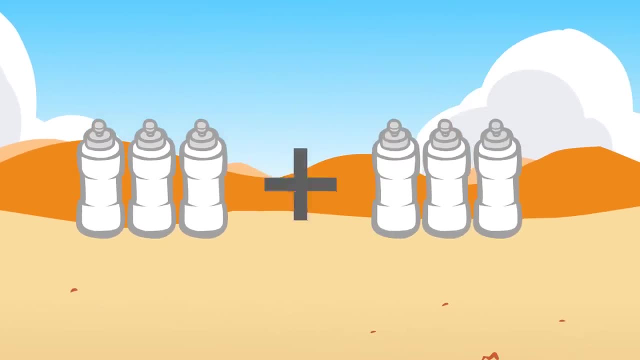 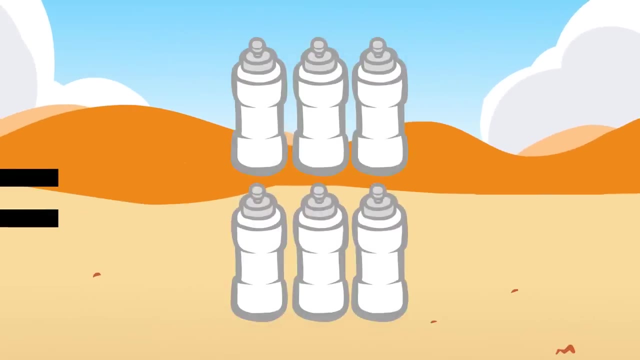 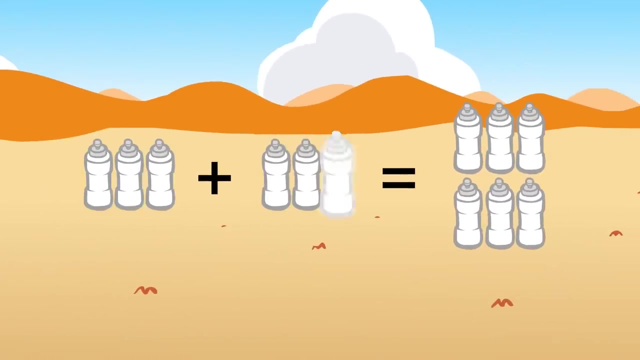 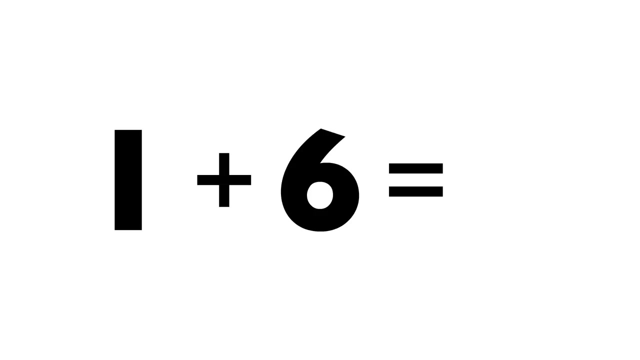 And 67. Plus 3 equals 6.. One, two, three, four, five, six equals 1,, 2,, 3,, 4,, 5, 6.. One plus 6 equals 1 plus 6 equals 7.. 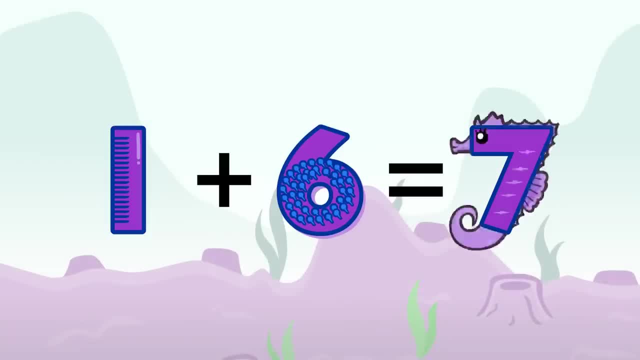 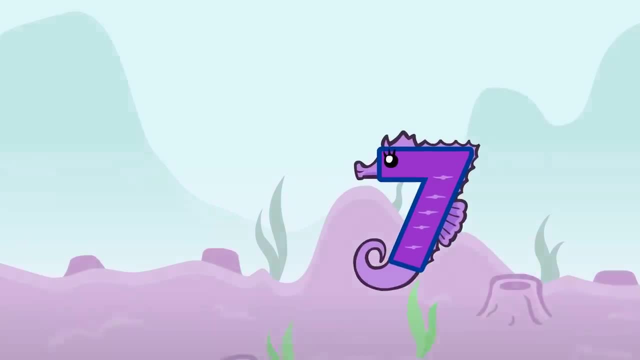 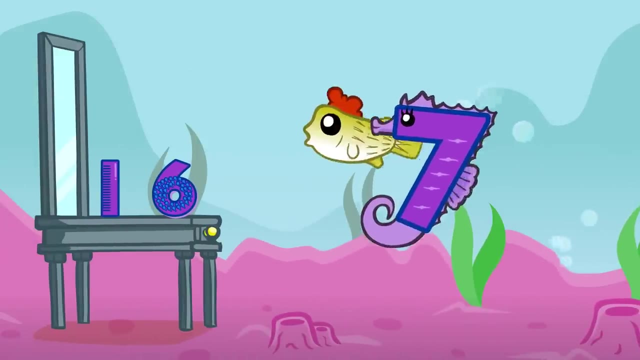 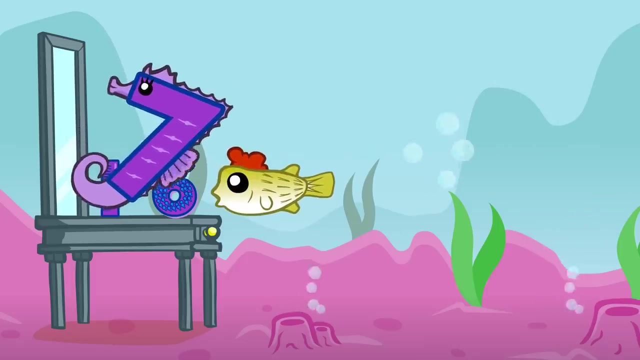 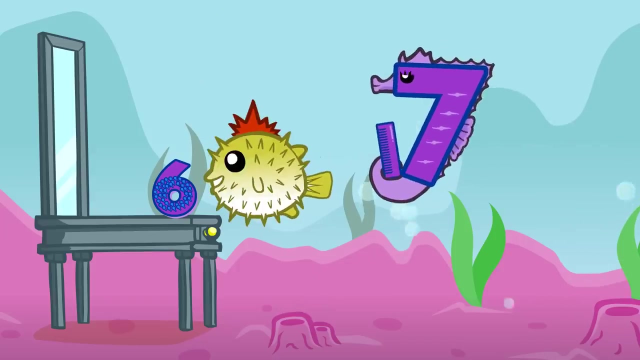 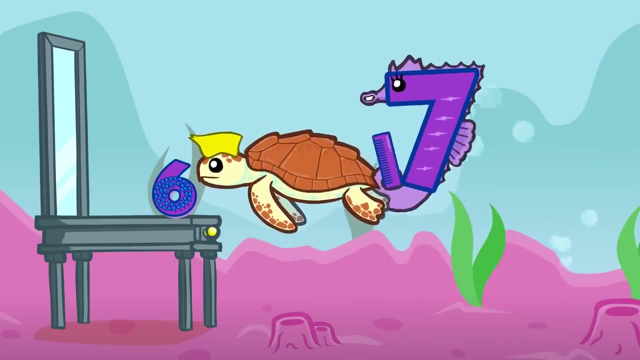 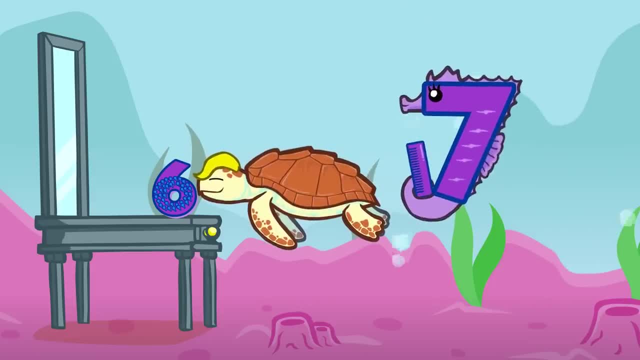 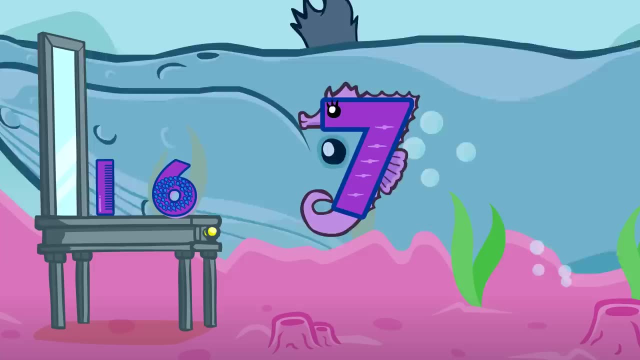 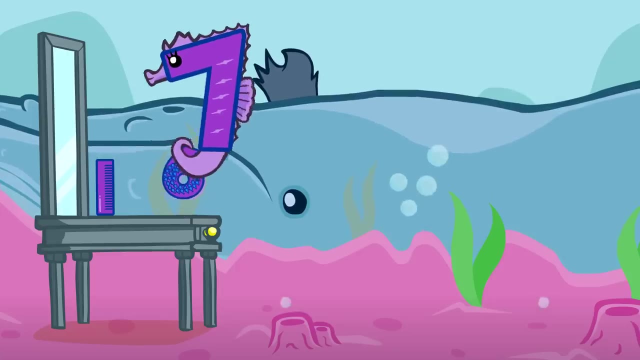 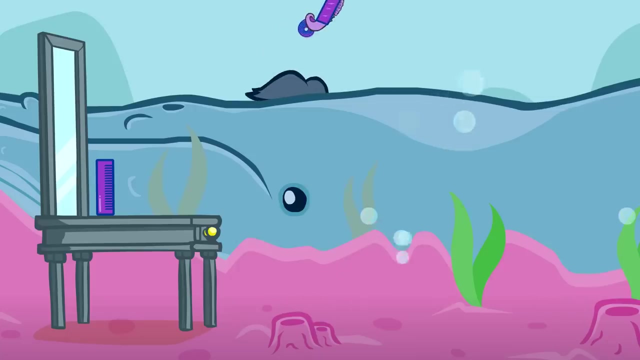 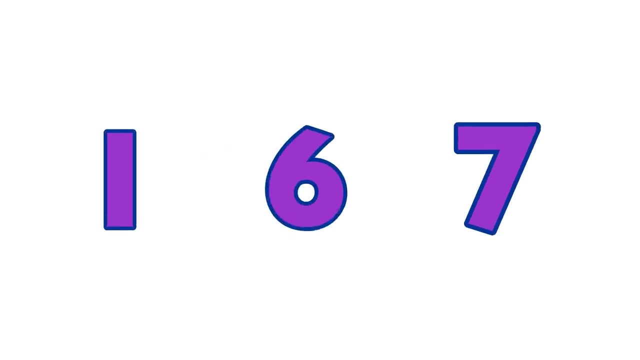 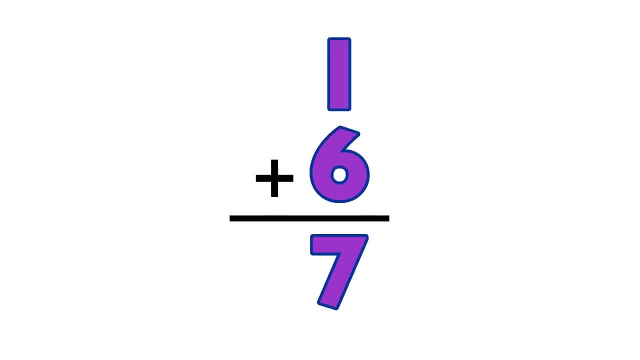 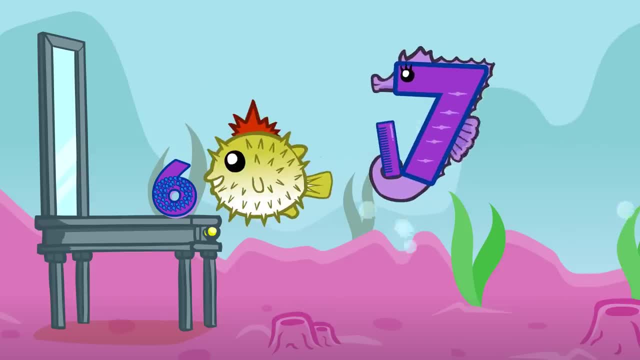 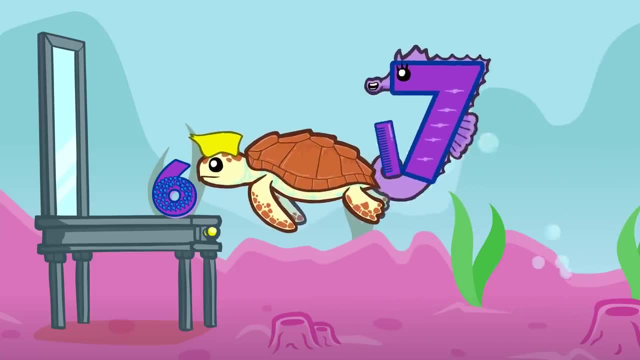 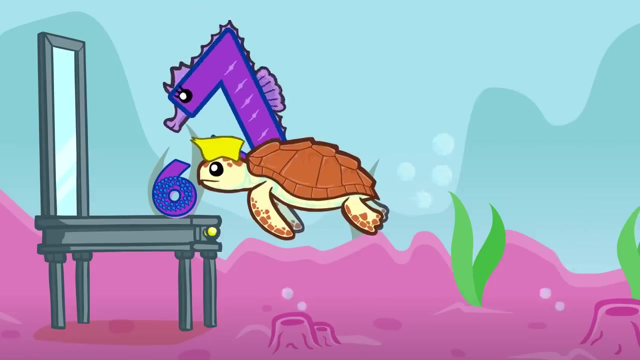 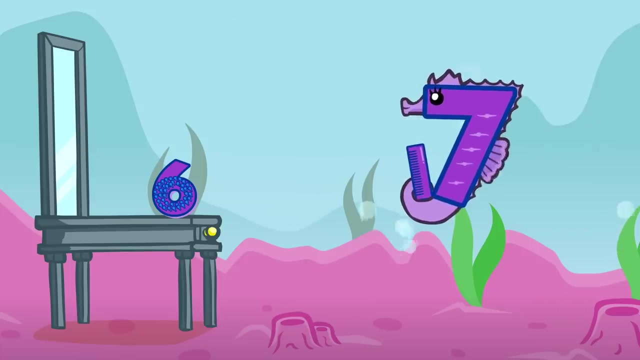 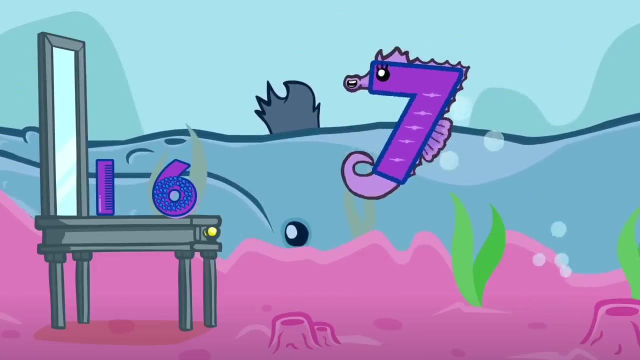 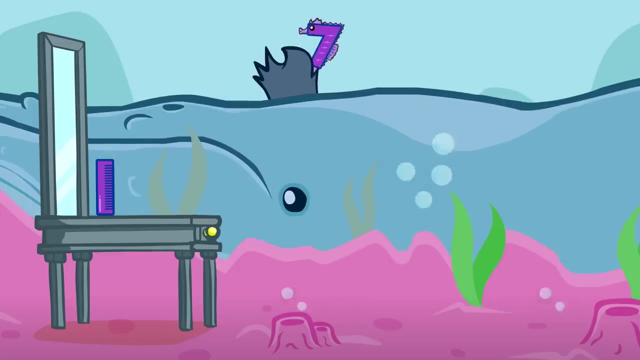 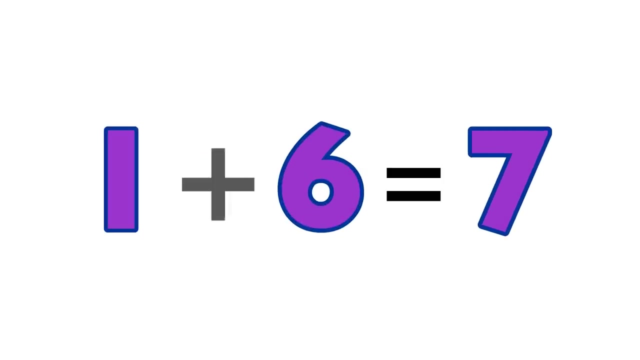 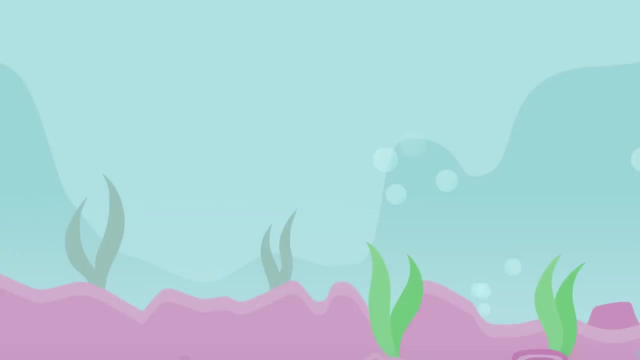 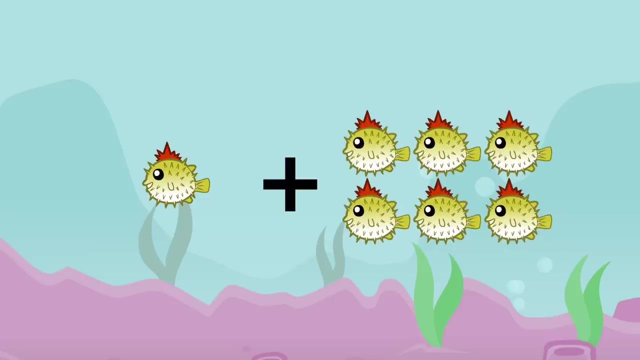 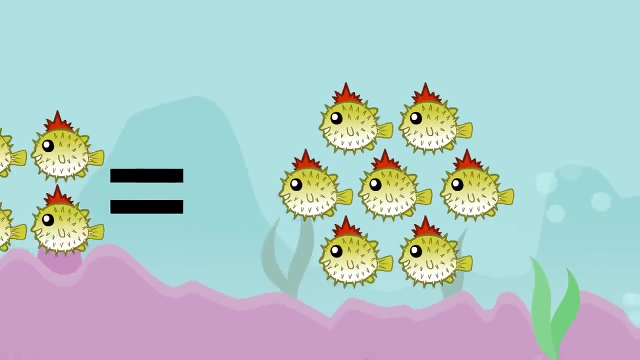 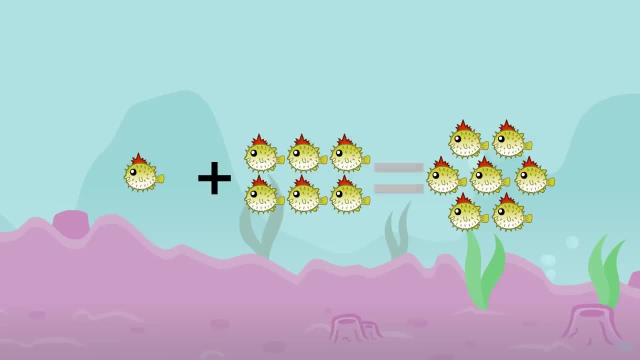 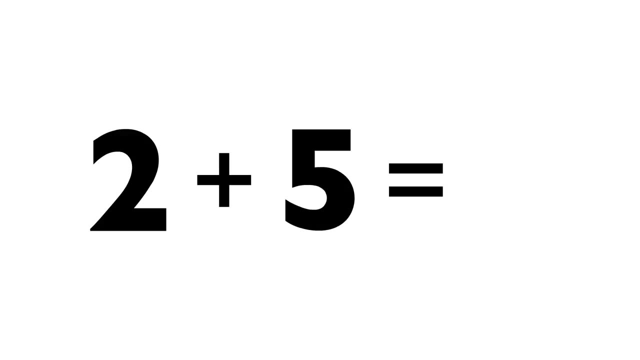 3,, 4,, 5, 6, 7 equals 1,, 2,, 3,, 4,, 5, 6, 7.. 2 plus 5 equals 2 plus 5 equals 7.. 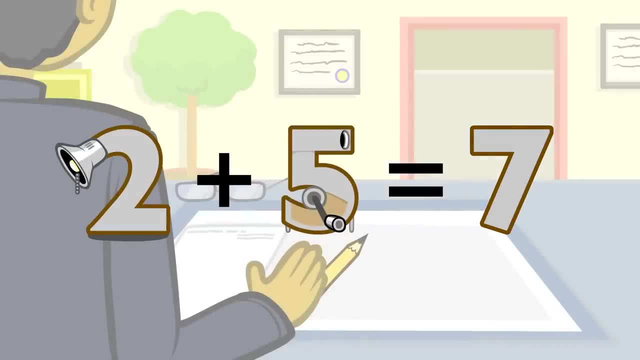 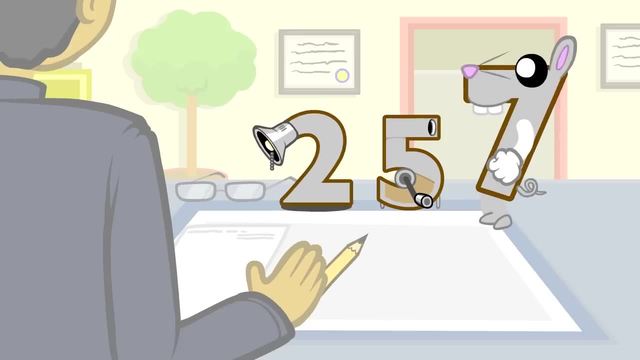 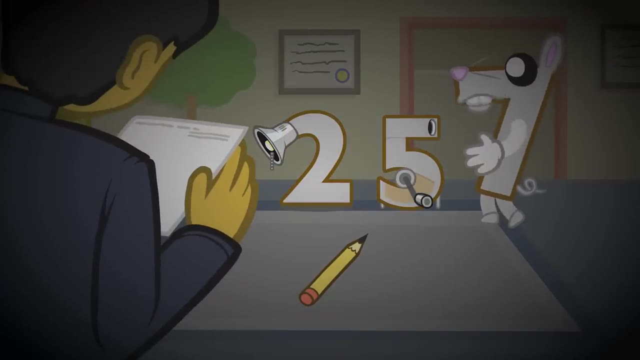 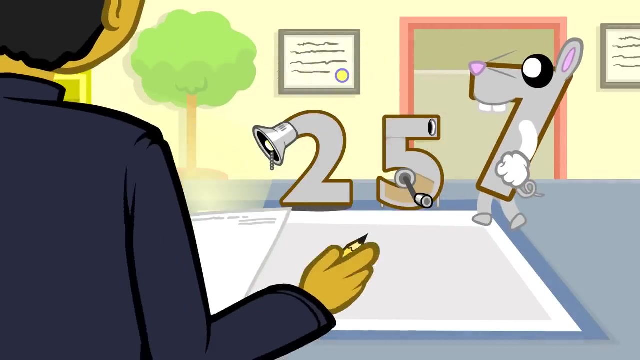 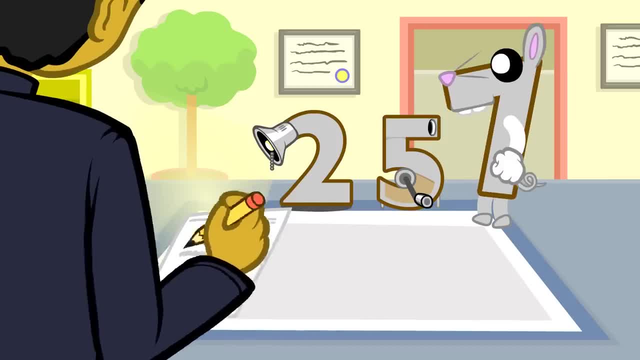 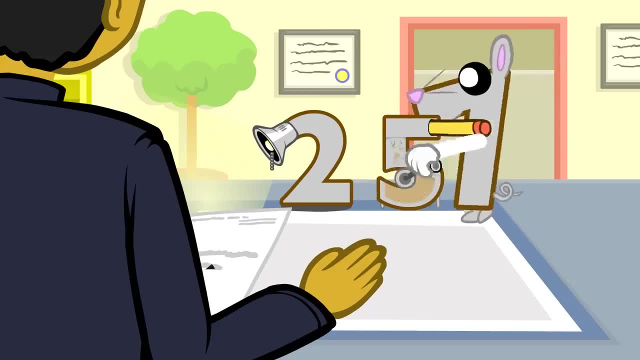 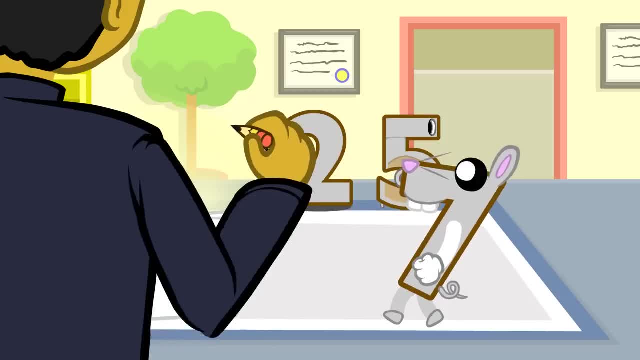 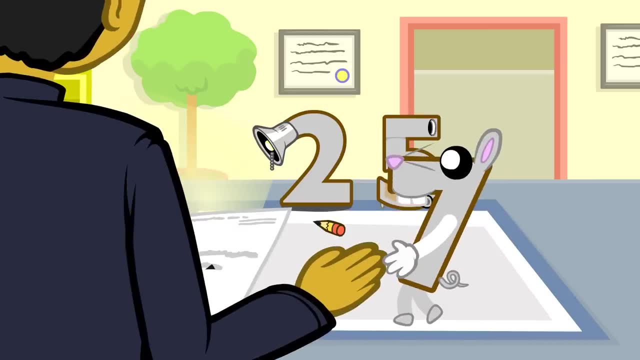 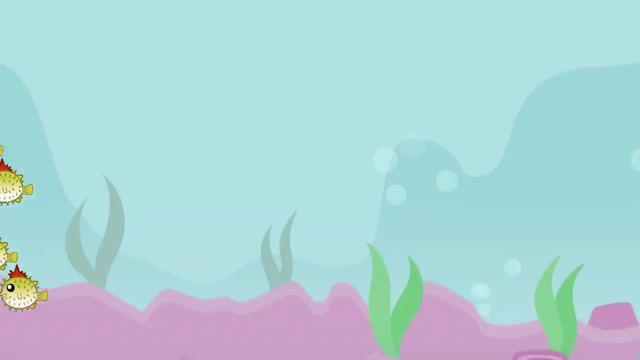 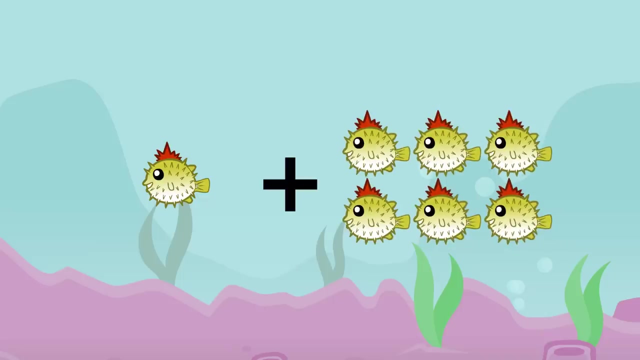 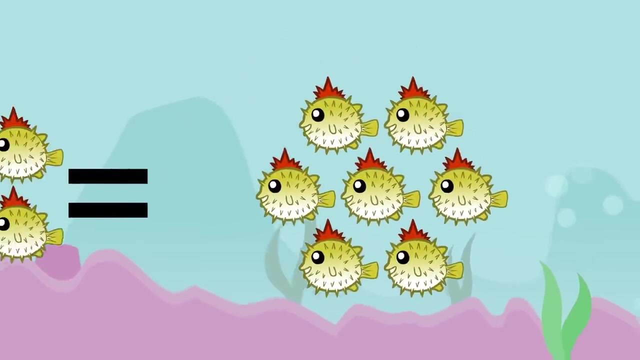 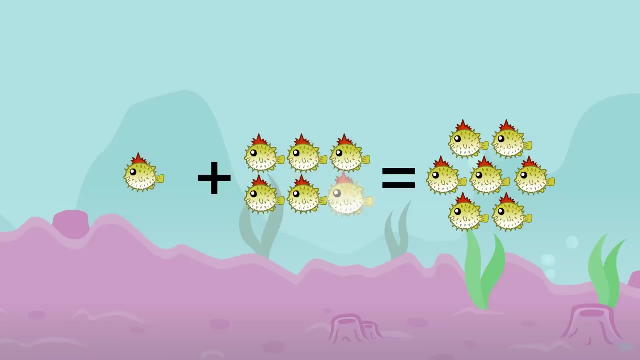 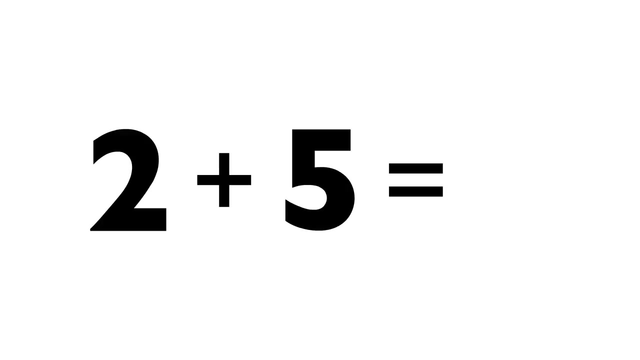 1 plus 6 equals 7.. 1,, 2,, 3,, 4,, 5, 6, 7 equals 1, 2,, 3,, 4,, 5,, 6, 2 plus 5 equals. 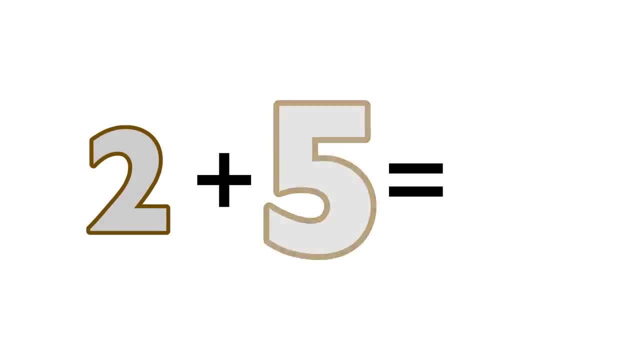 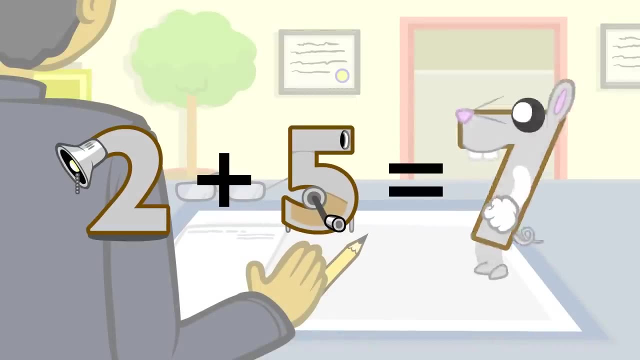 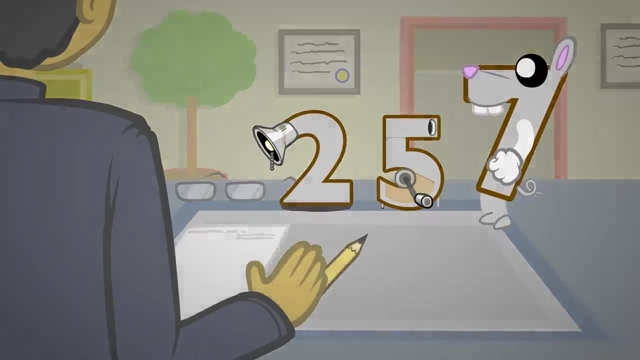 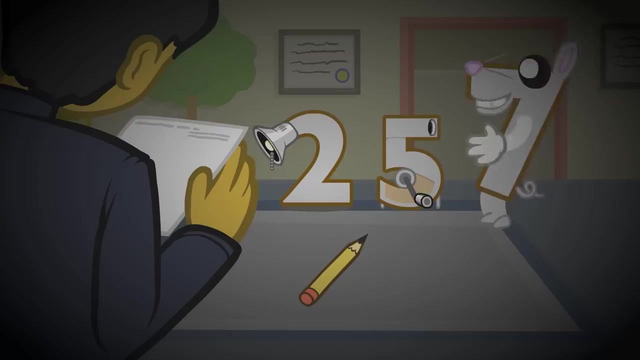 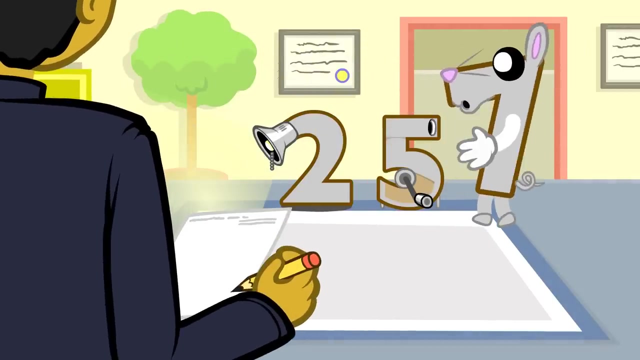 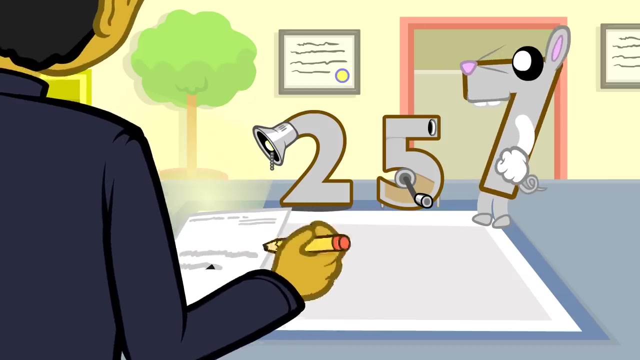 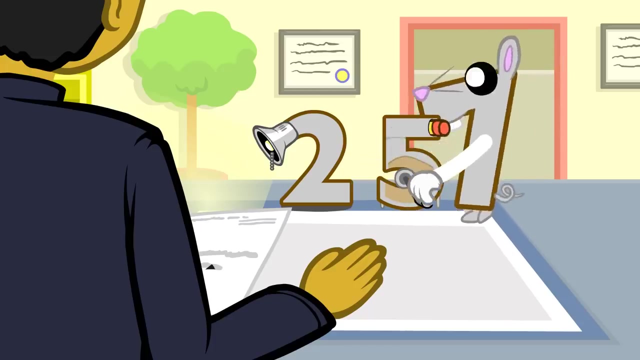 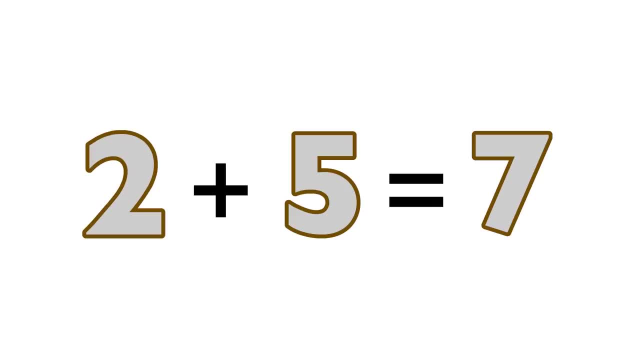 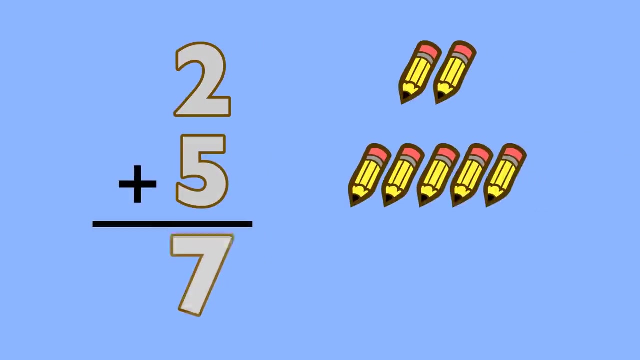 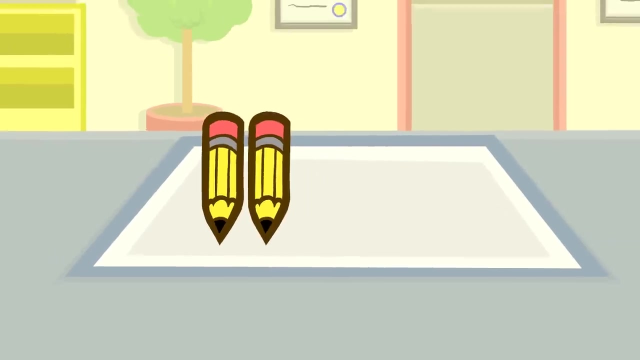 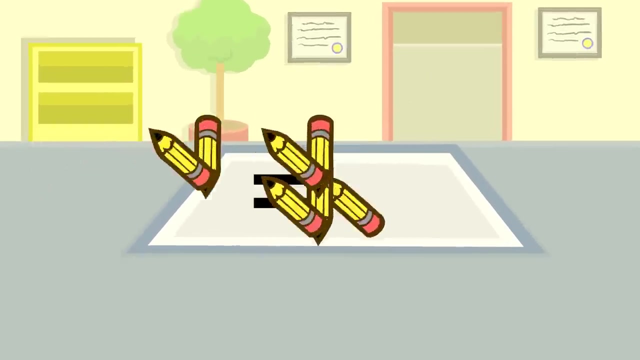 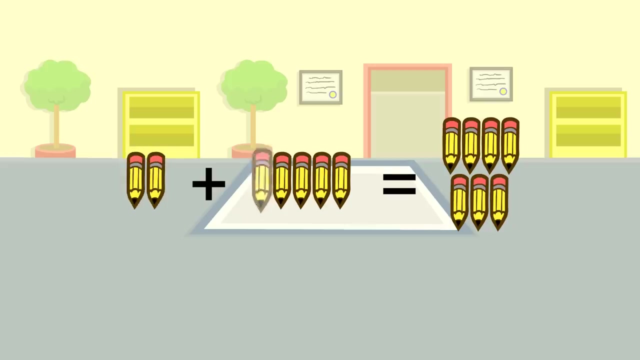 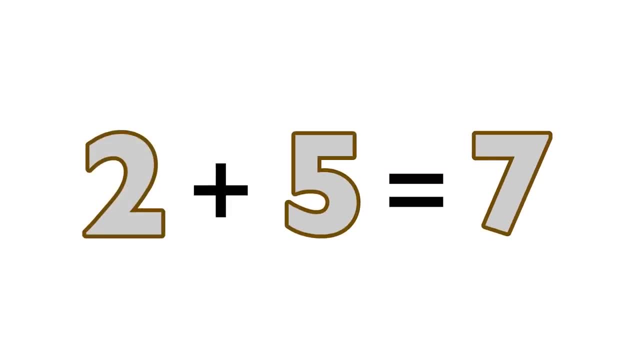 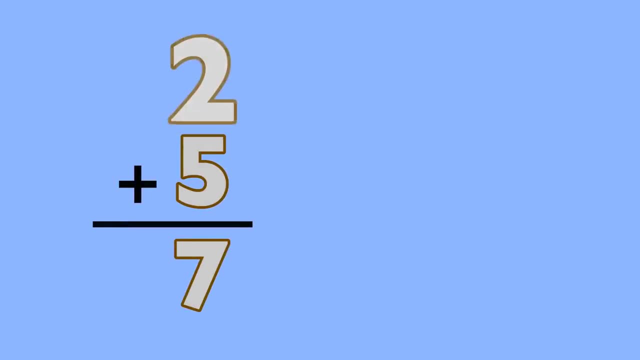 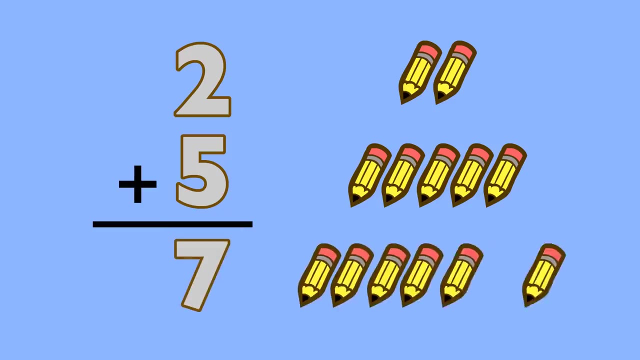 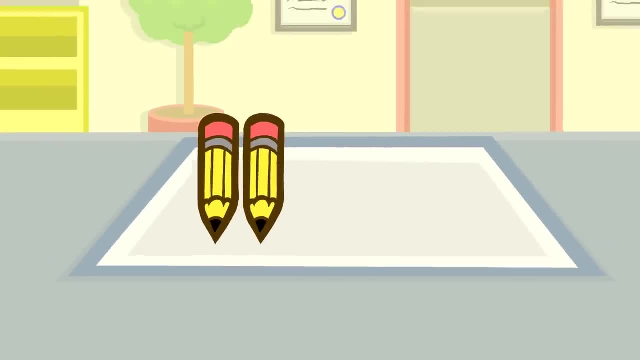 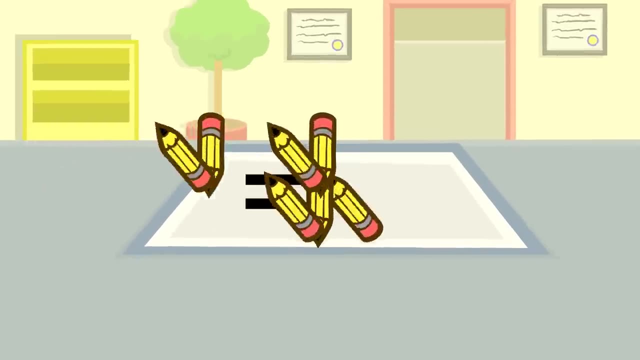 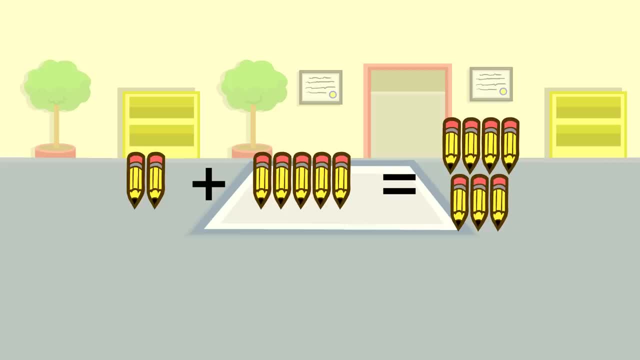 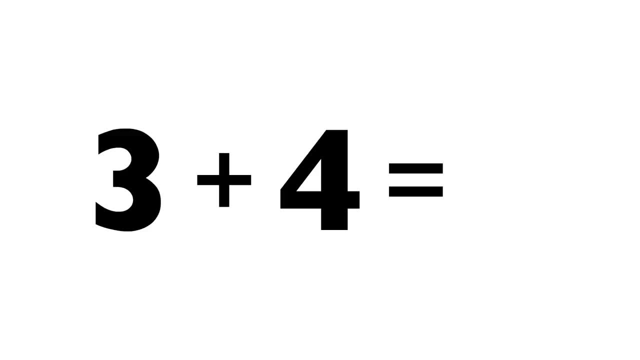 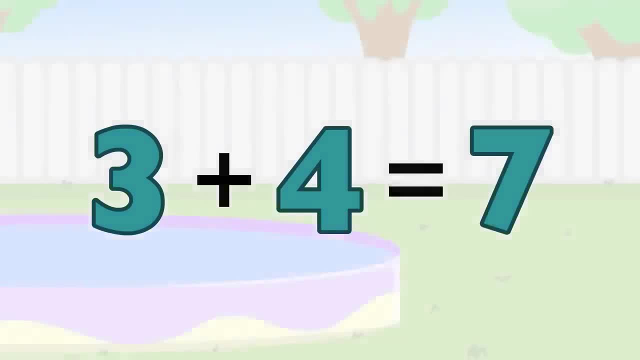 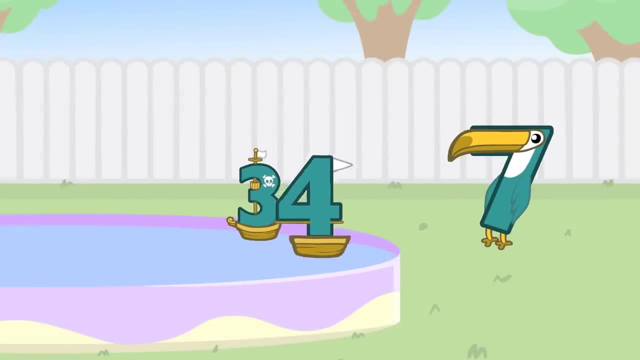 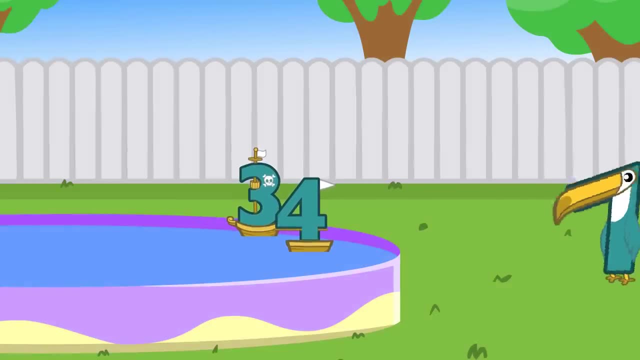 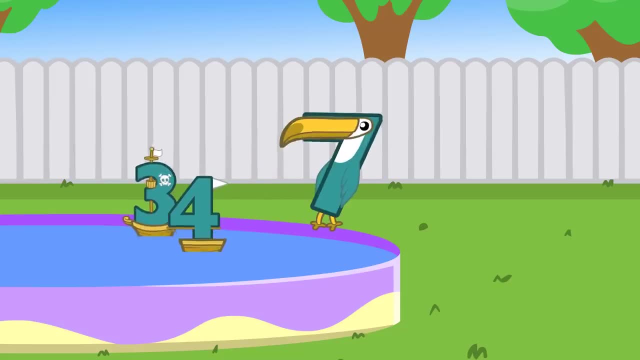 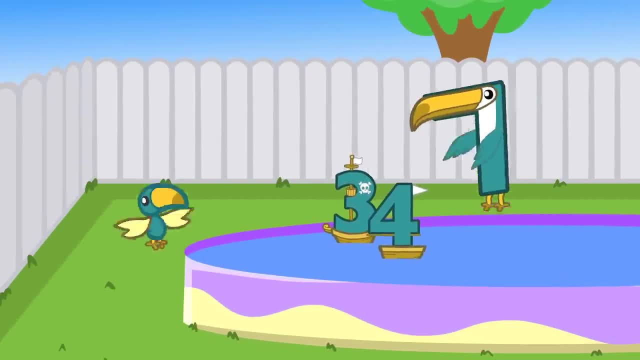 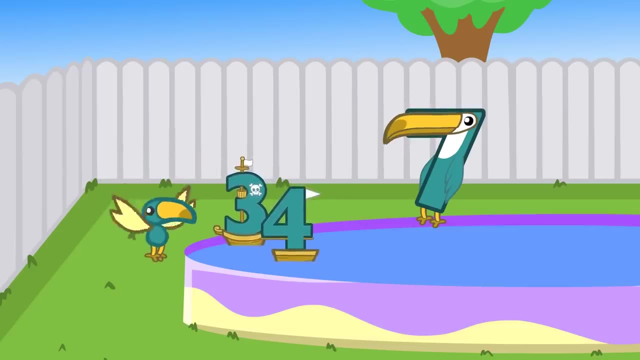 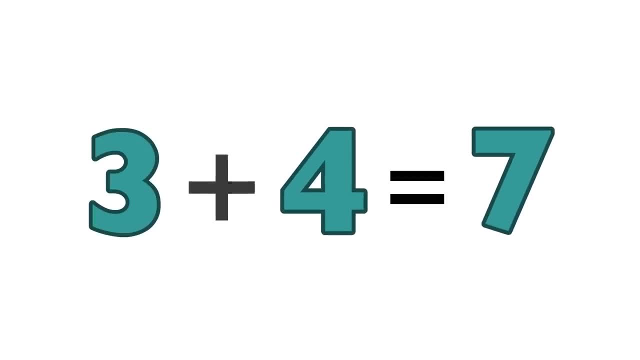 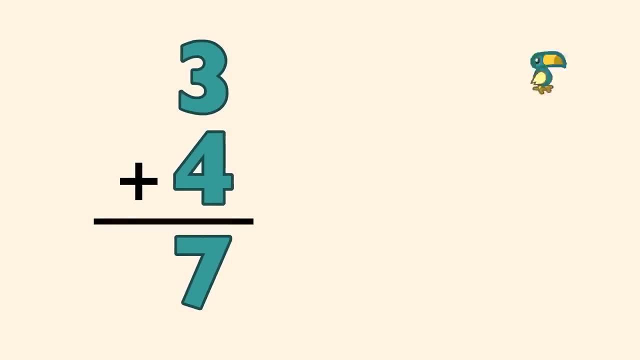 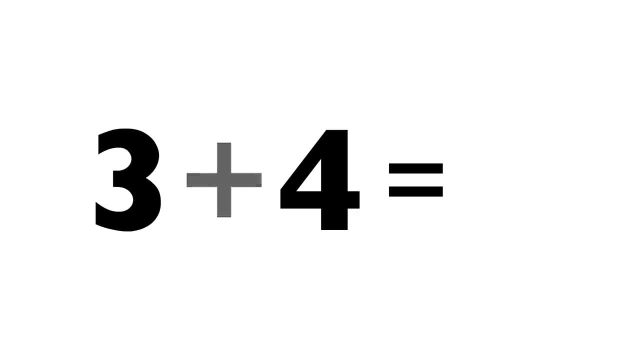 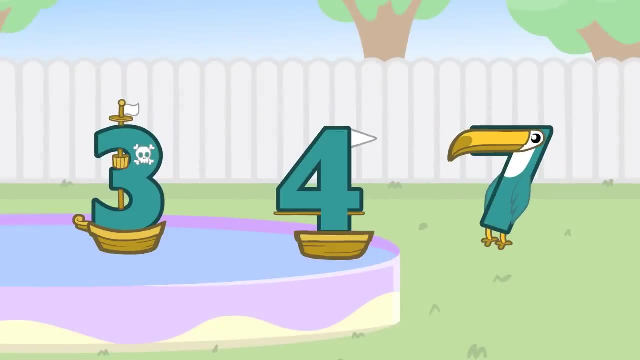 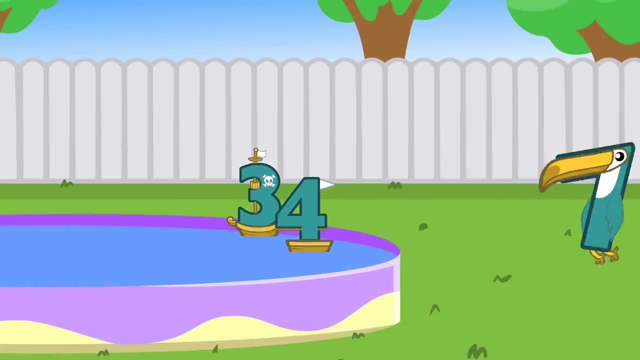 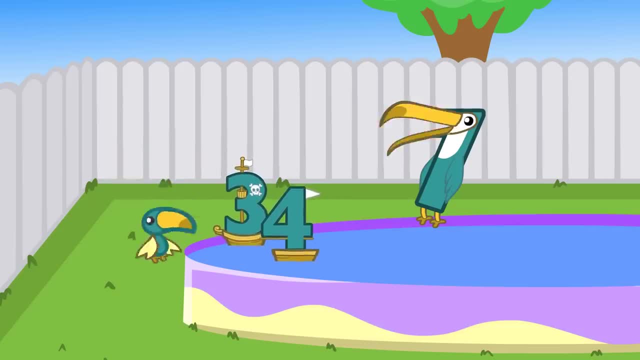 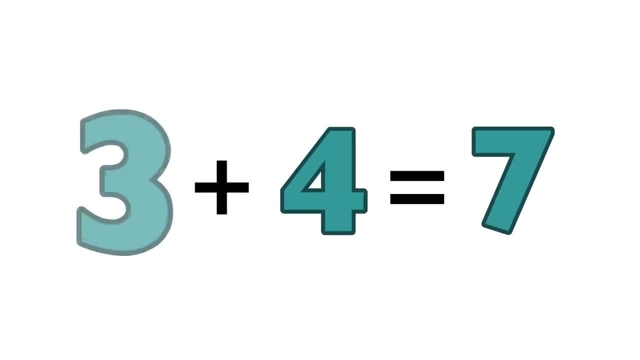 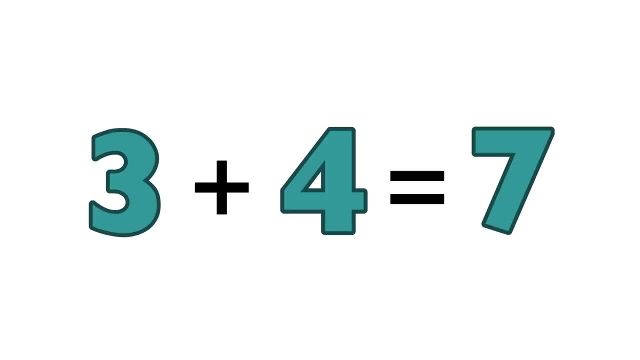 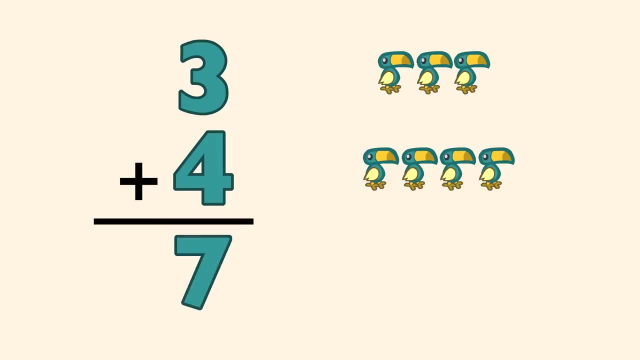 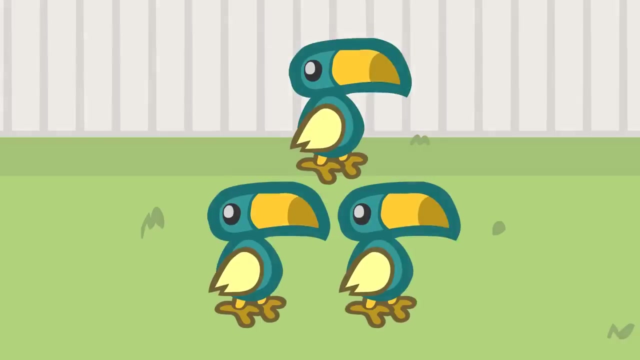 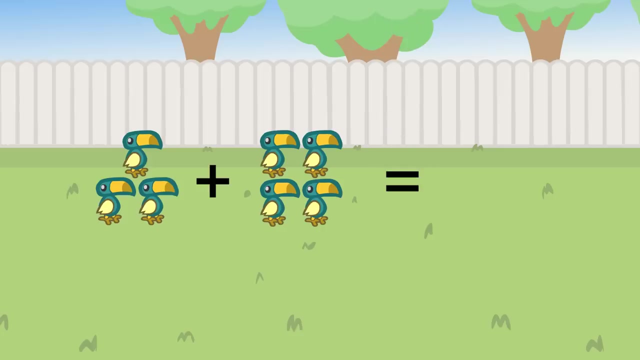 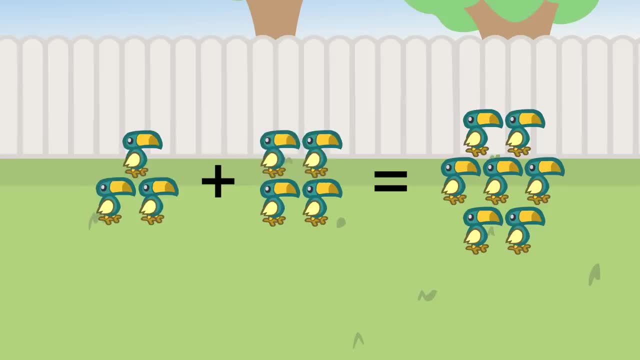 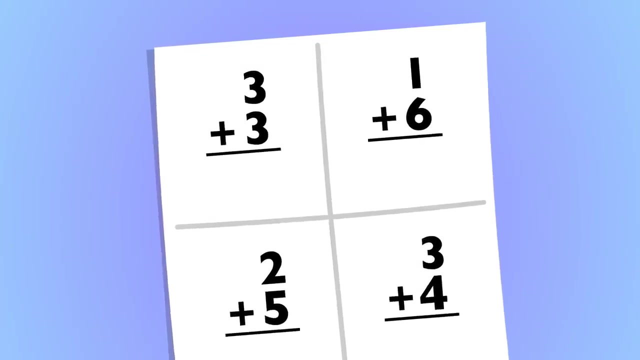 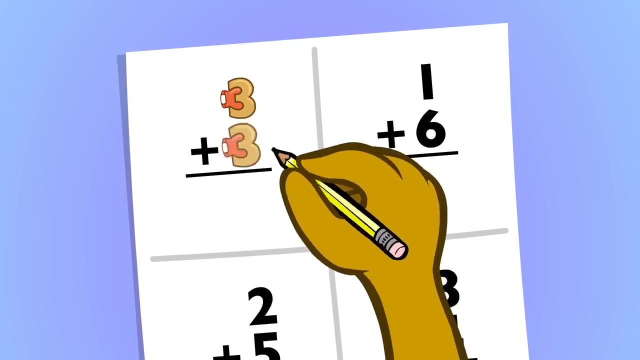 1,, 2,, 3,, 4,, 5,, 6, 7 equals 1,, 2,, 3,, 4,, 5, 6. 7. 3 plus 3 equals 6.. 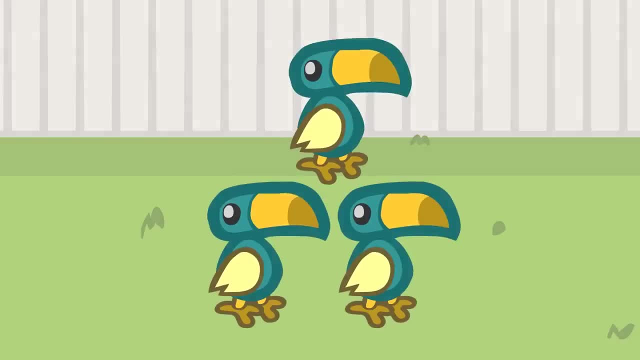 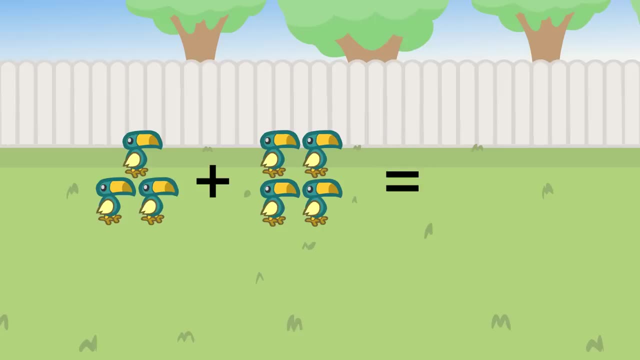 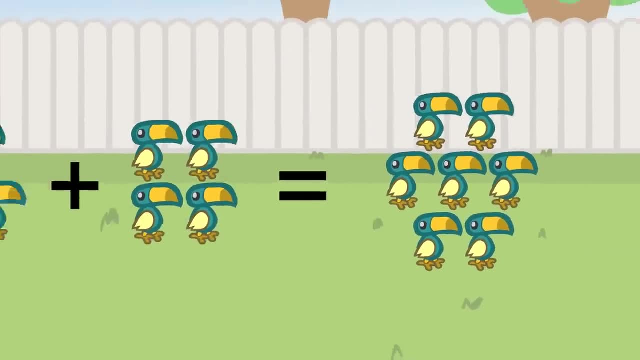 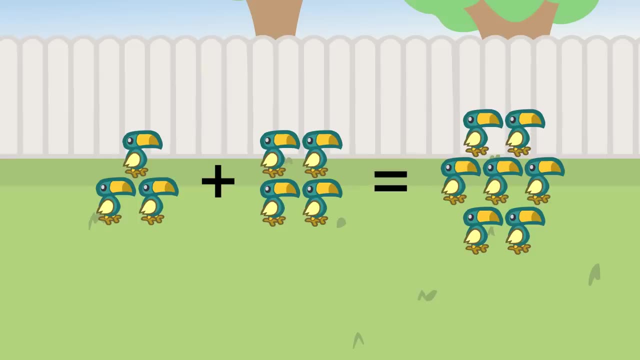 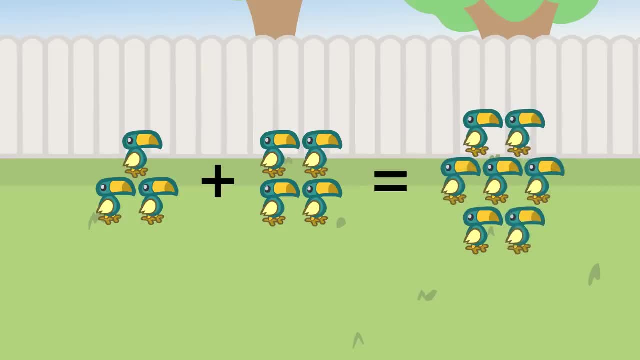 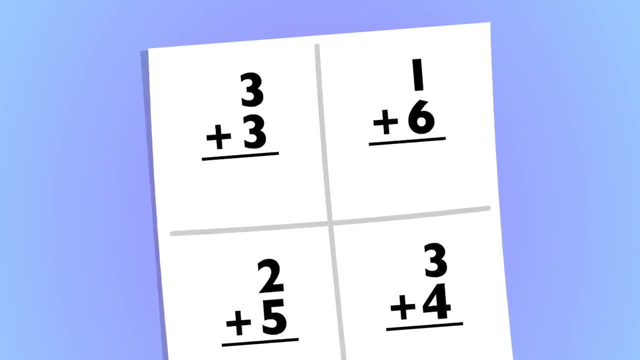 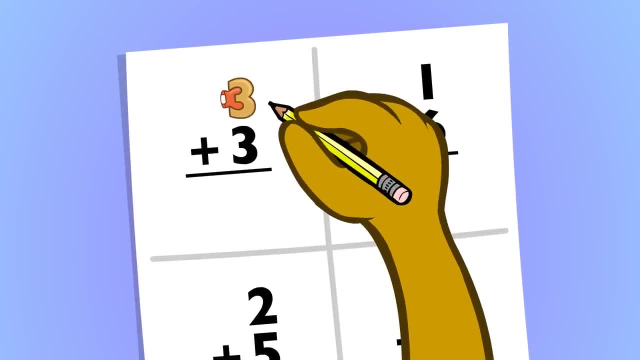 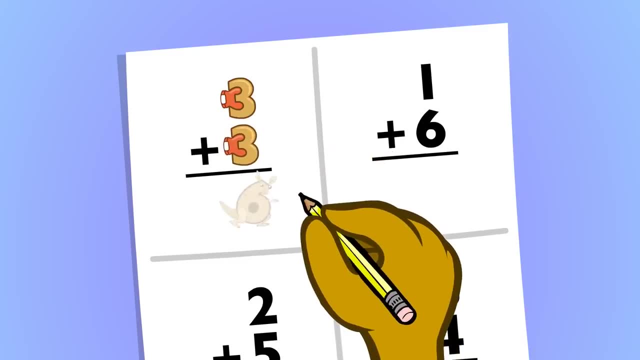 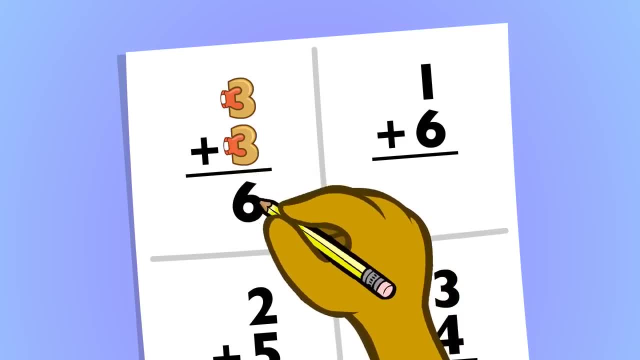 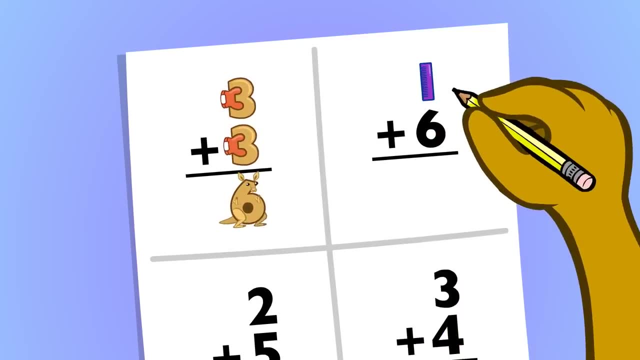 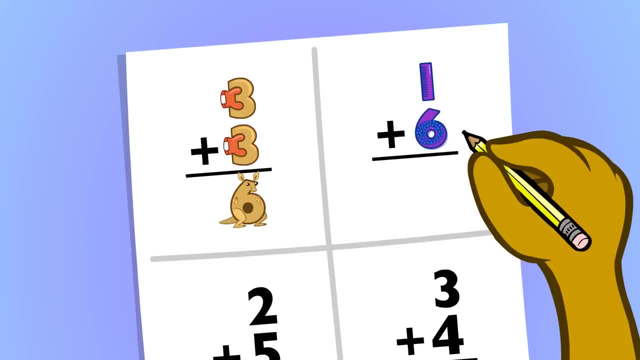 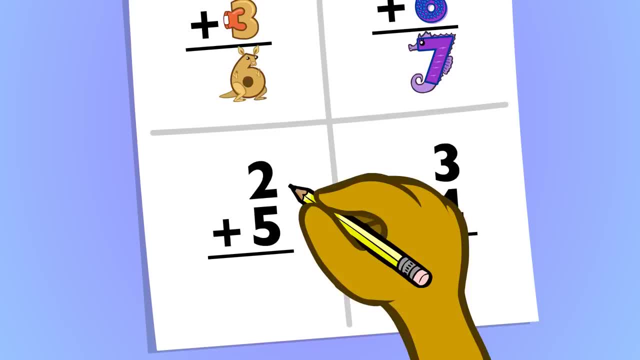 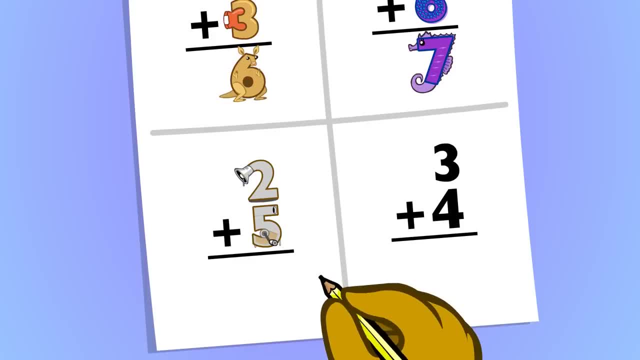 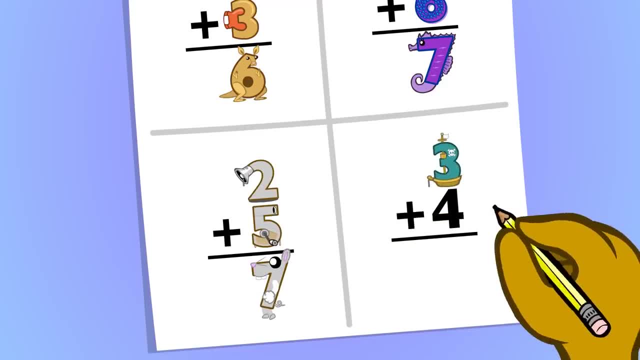 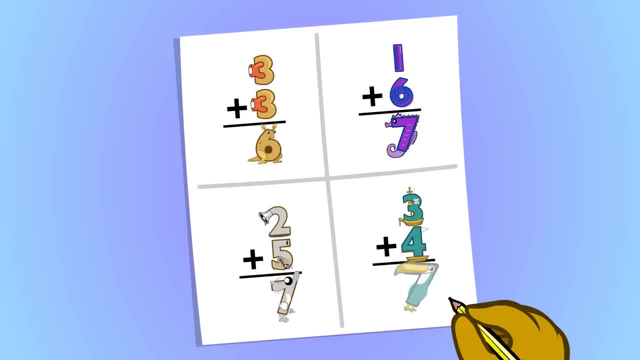 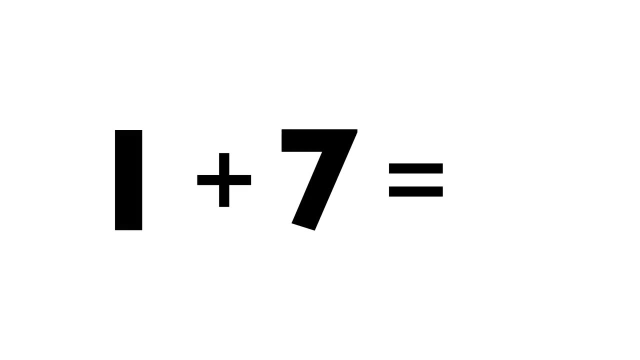 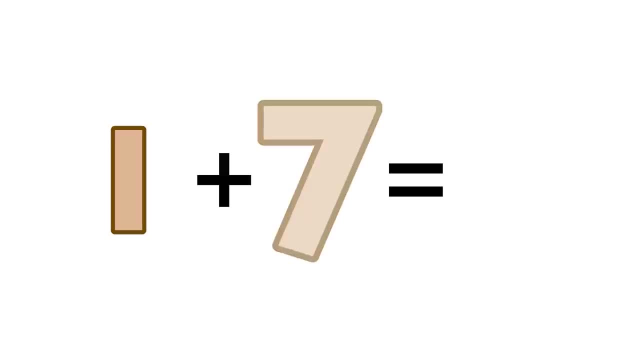 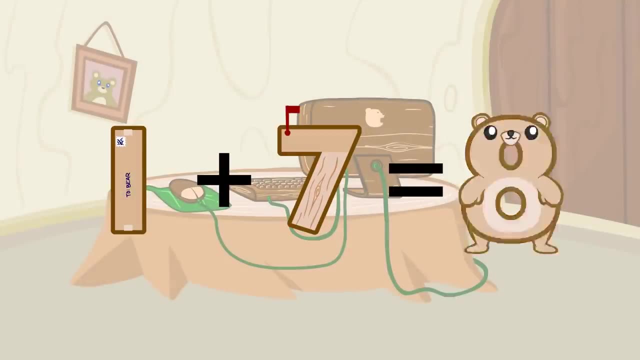 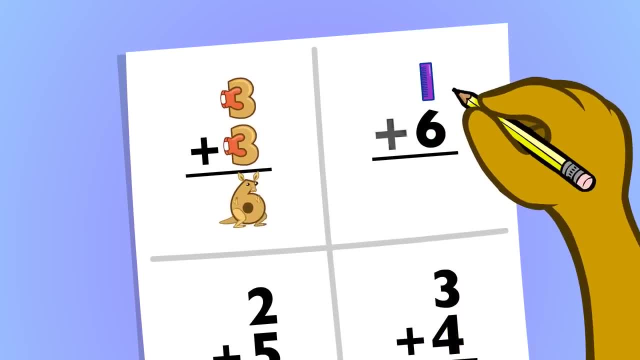 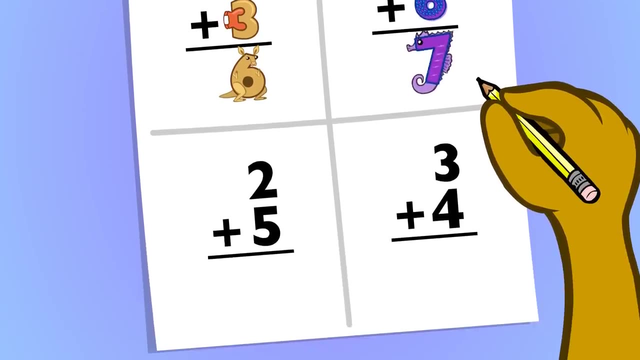 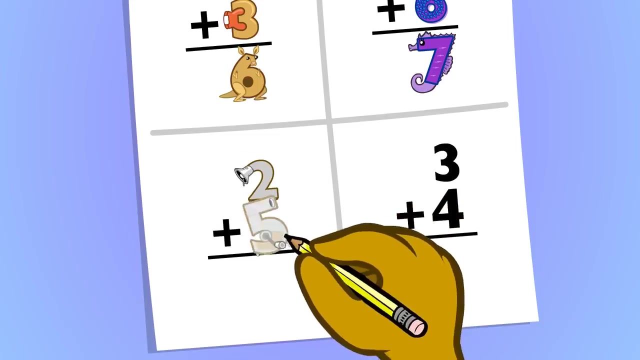 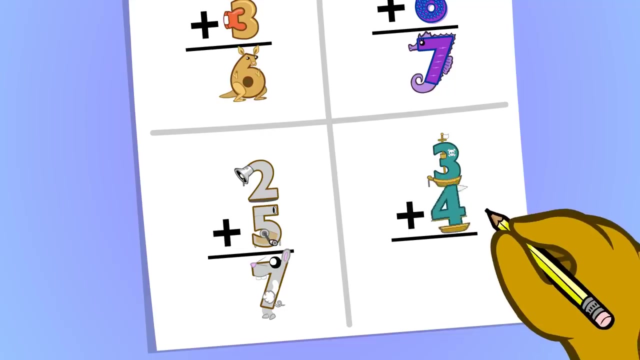 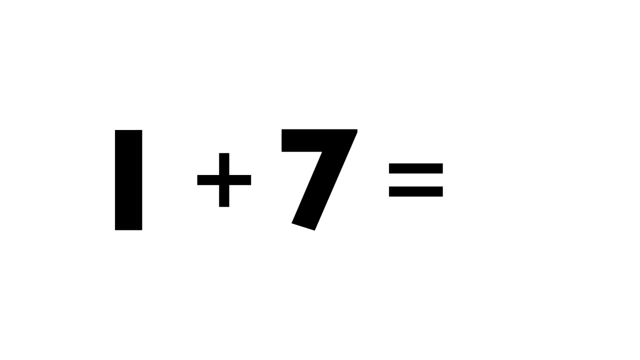 6. 1 plus 6 equals. 7.. 2 plus 5 equals 2. 4 equals. 7.. 3 plus 4 equals 7.. 3 plus 4 equals 7. 7.. One plus seven equals. 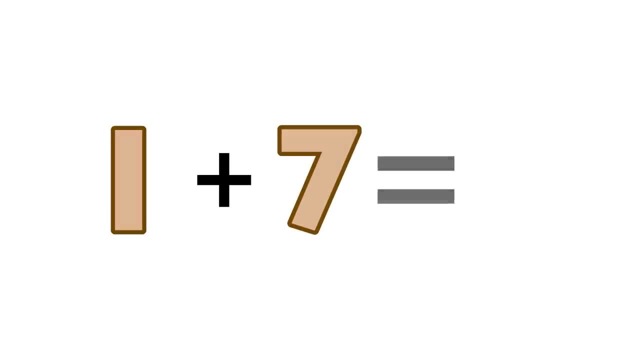 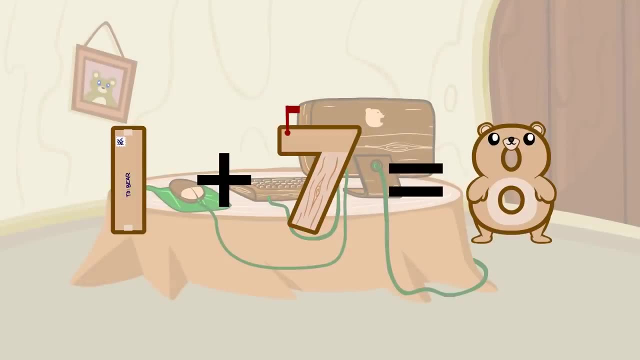 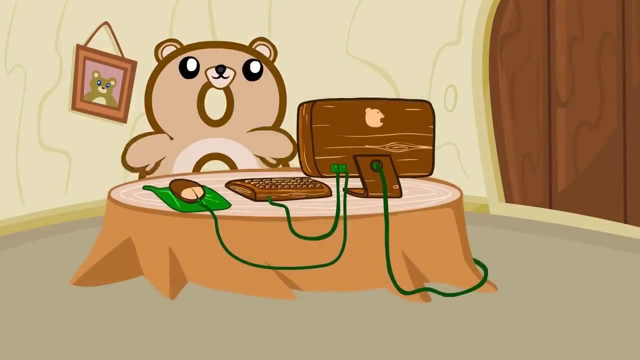 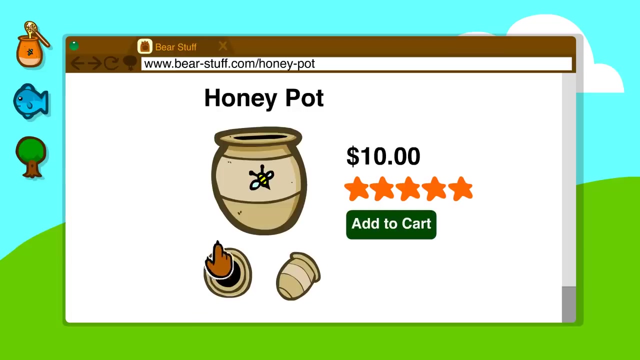 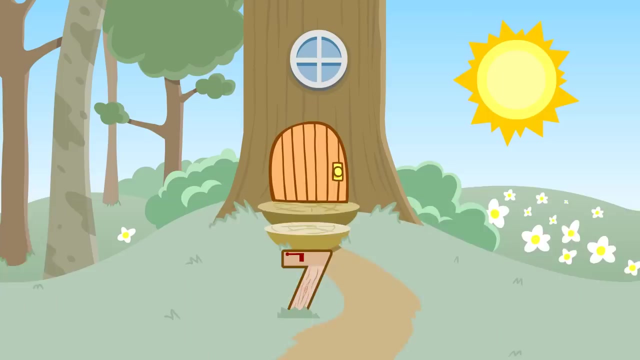 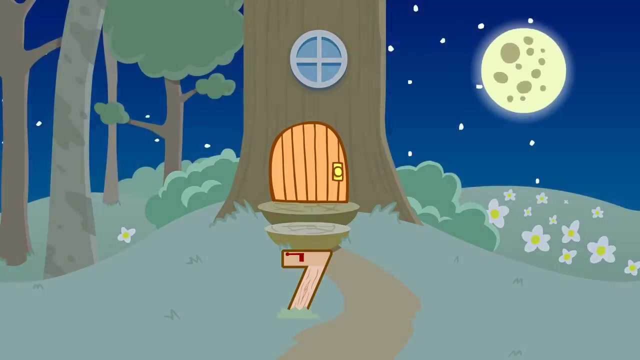 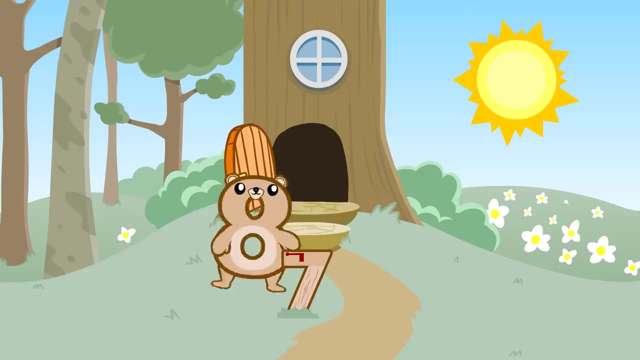 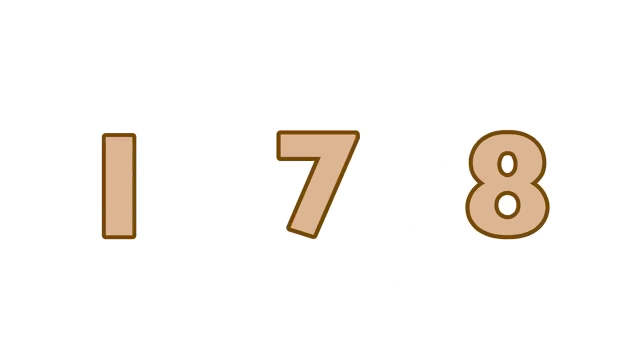 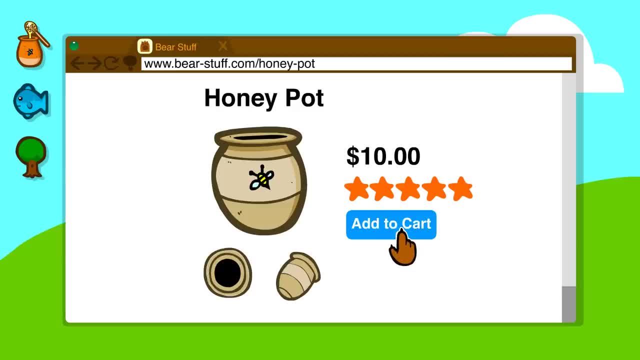 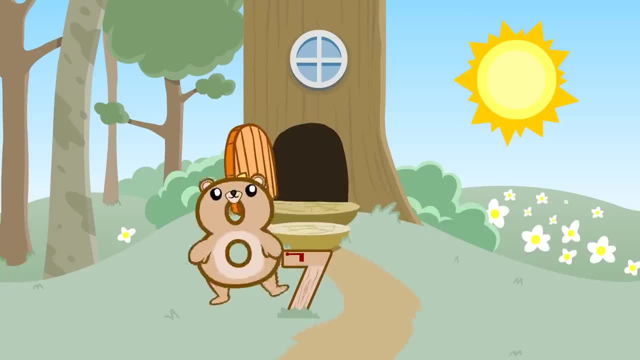 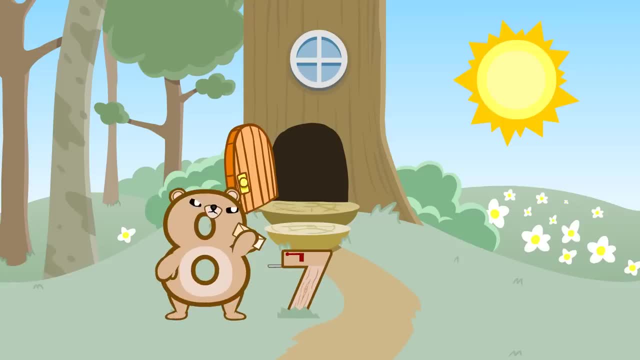 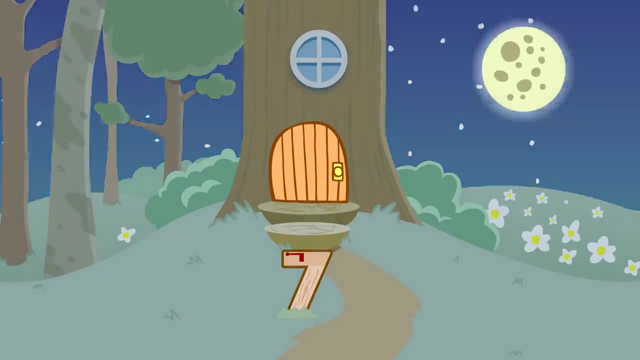 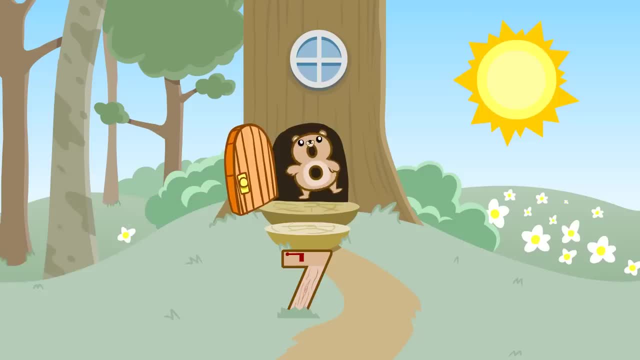 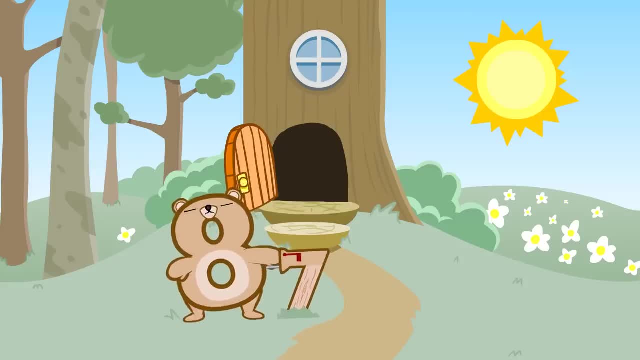 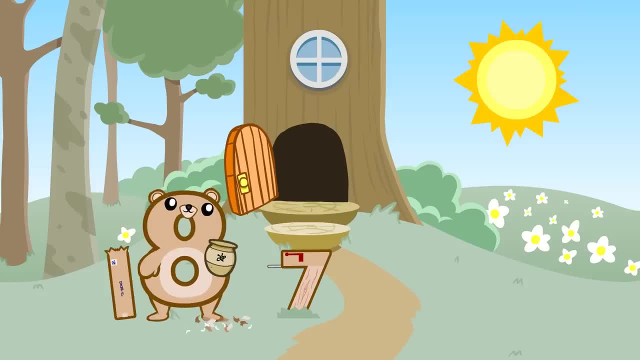 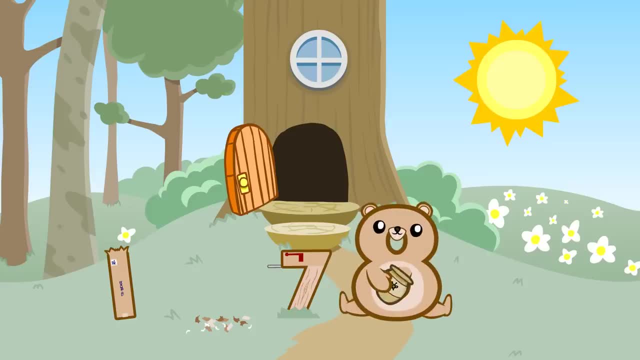 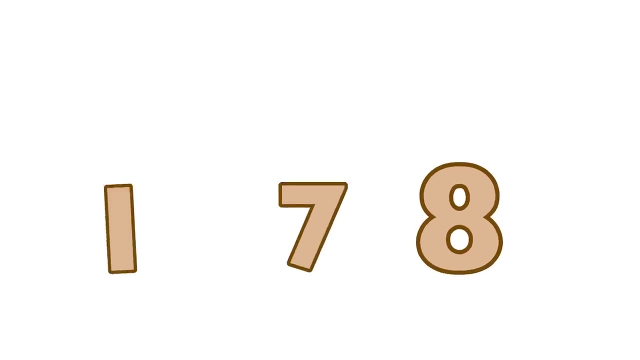 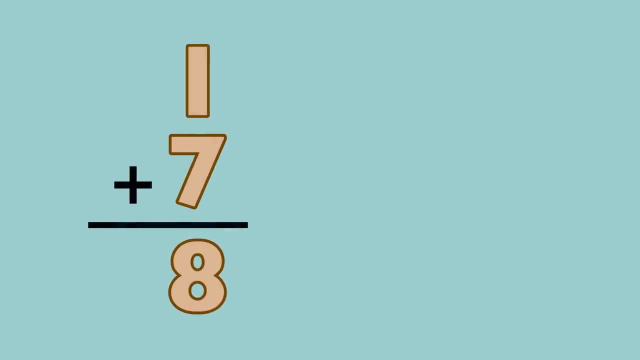 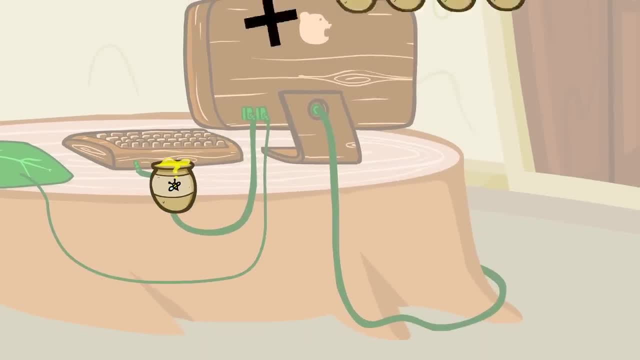 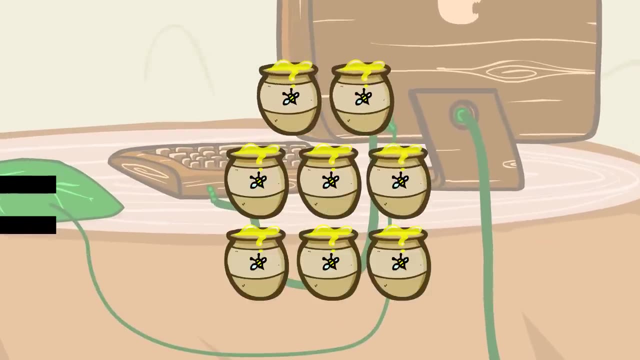 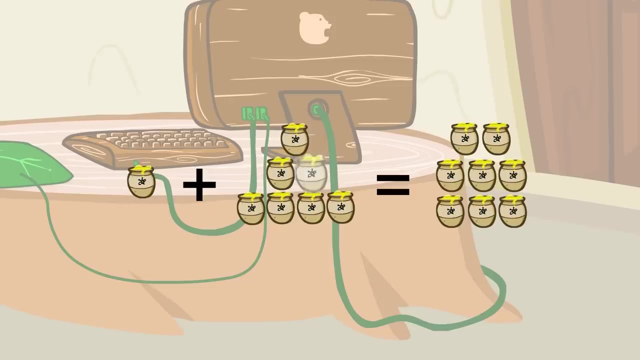 1 plus 7 equals 8.. 1, 2, 3.. 1,, 2,, 3,, 4,, 5,, 6,, 7, 8 equals 1,, 2,, 3,, 4,, 5,, 6,, 7, 8.. 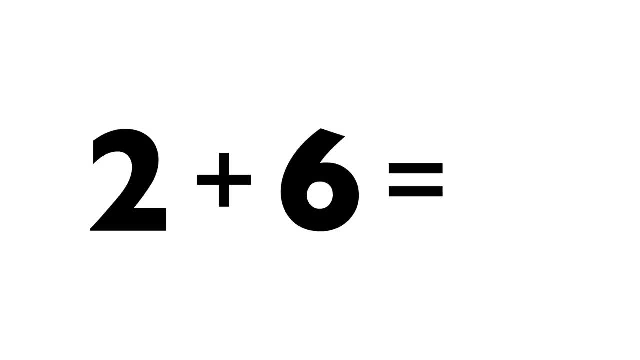 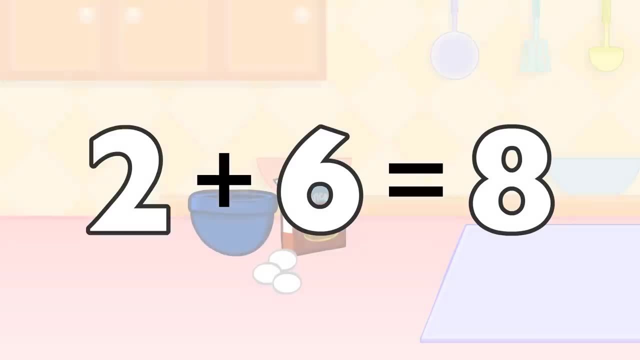 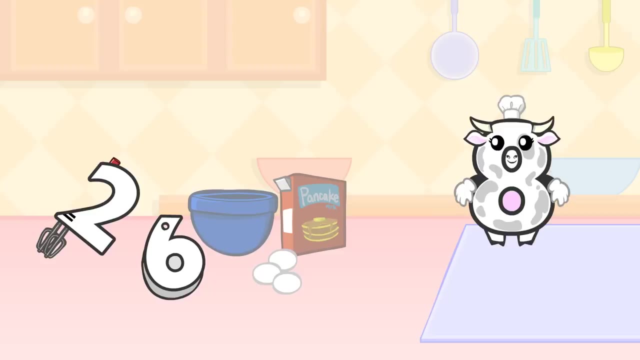 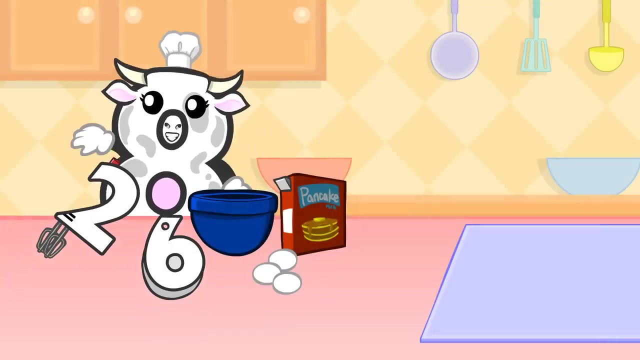 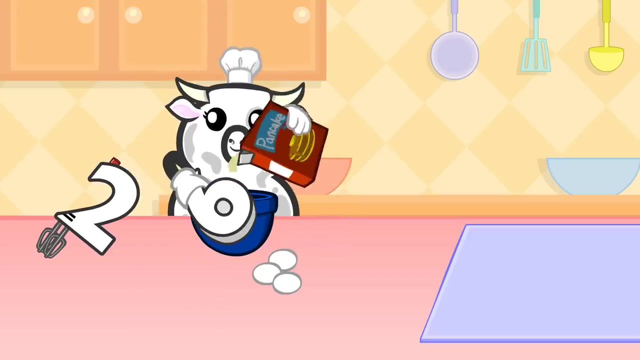 2 plus 6 equals. 2 plus 6 equals 8!. 2 plus 6 equals 8.. 2 plus 6 equals 8.. 8!, 8!, 8!, 8!, 8!, 8!. 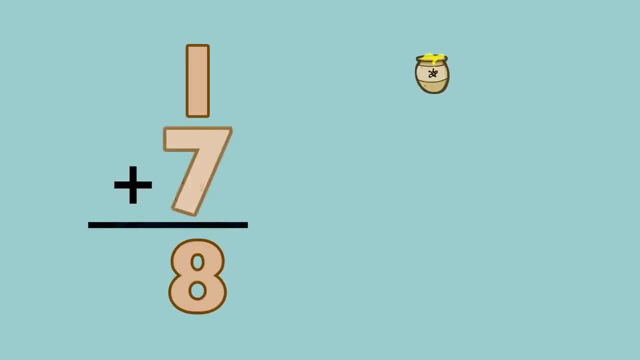 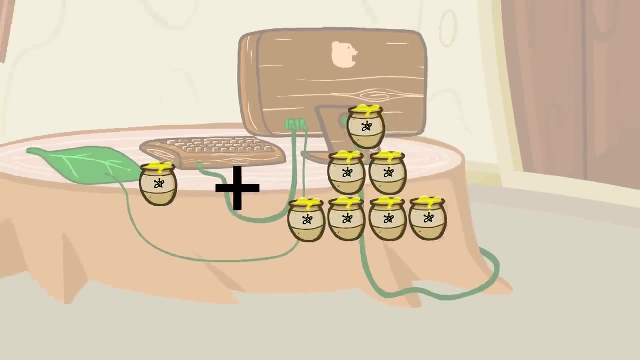 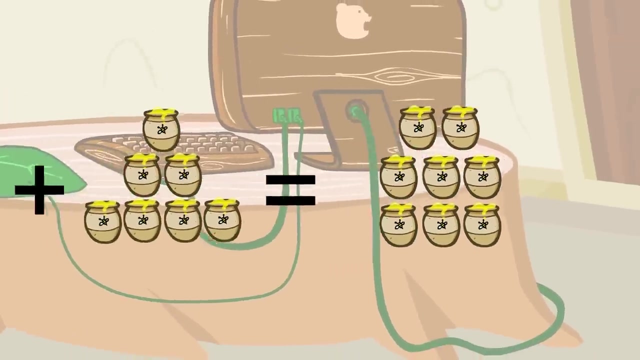 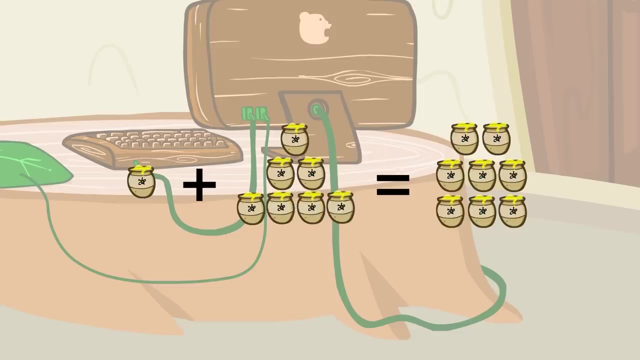 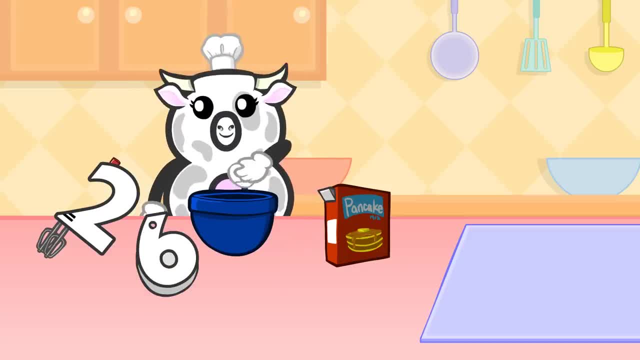 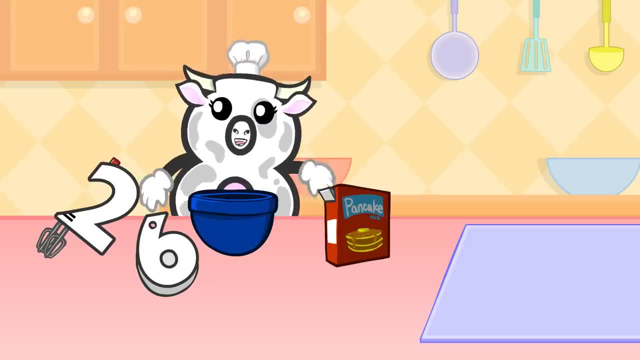 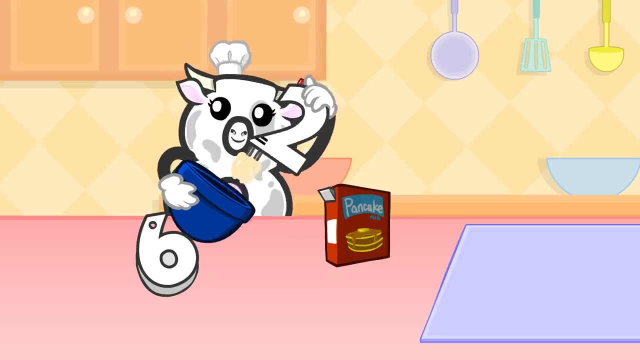 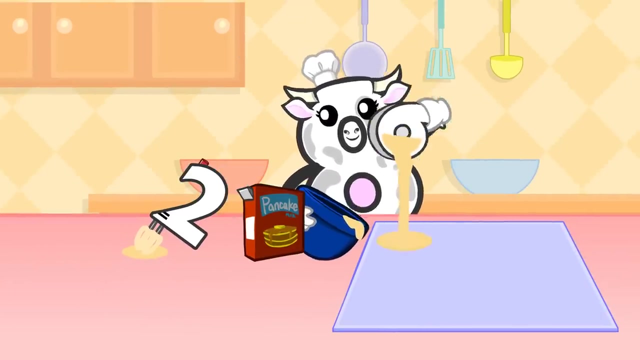 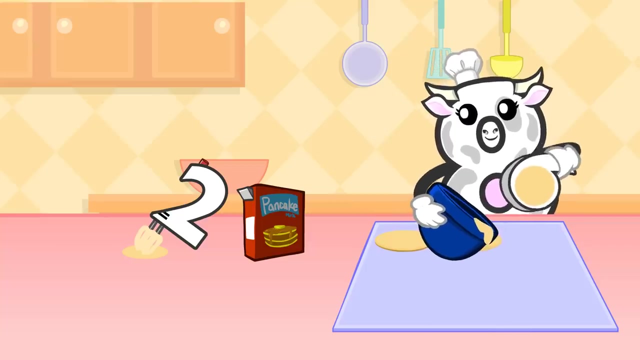 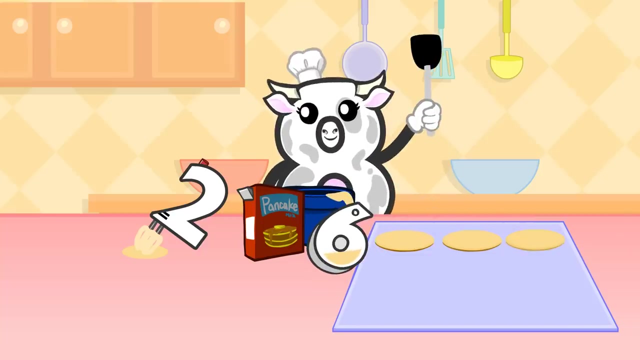 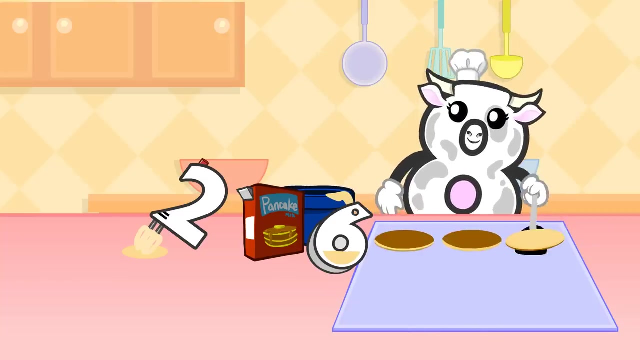 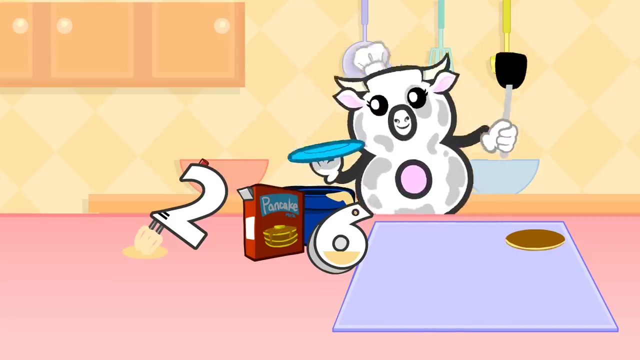 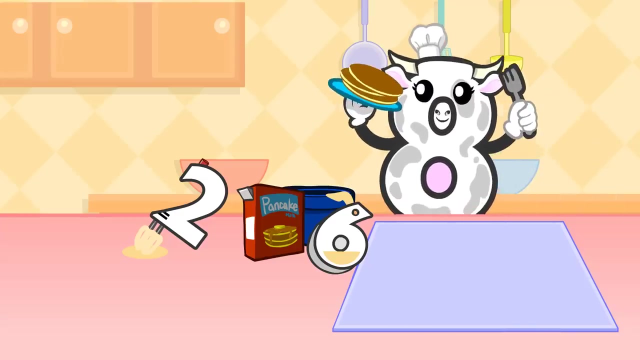 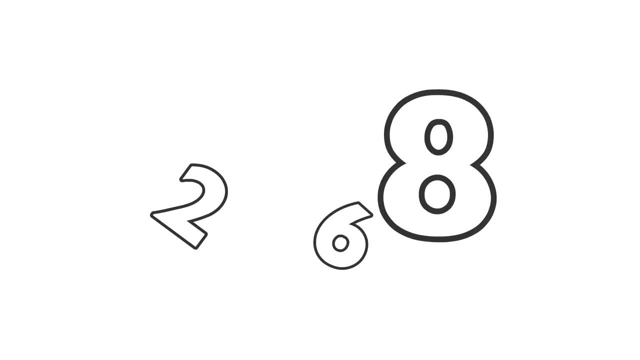 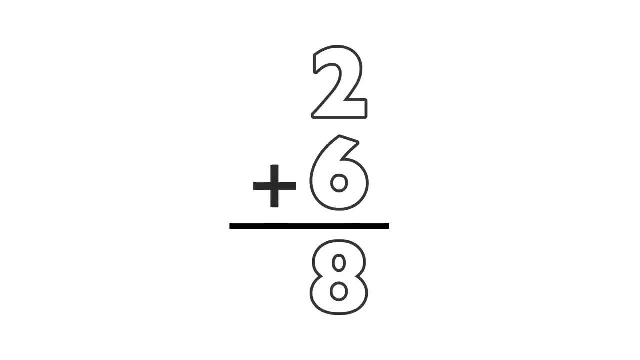 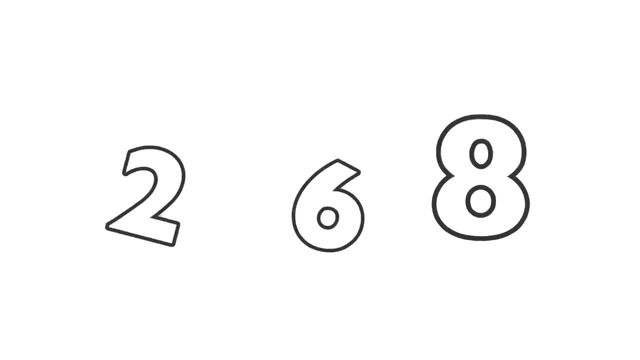 18! One Stop. What happened? 2 plus 6 equals 8!. C62! 2 plus 6 equals 8.. 2 plus 6 equals 8.. 2 plus 6 equals 8.. 1, 2, 3, 4, 5, 6, 7, 8 equals 1, 2,, 3,, 4, 5, 6, 7, 8.. 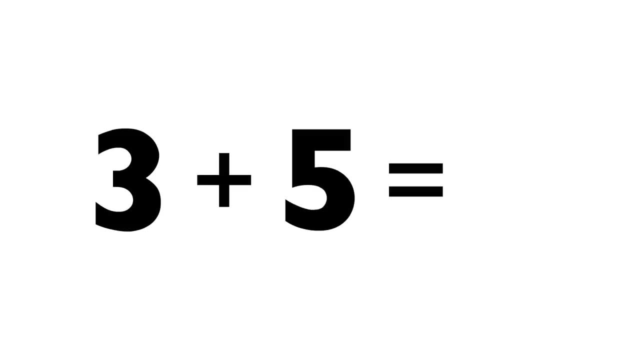 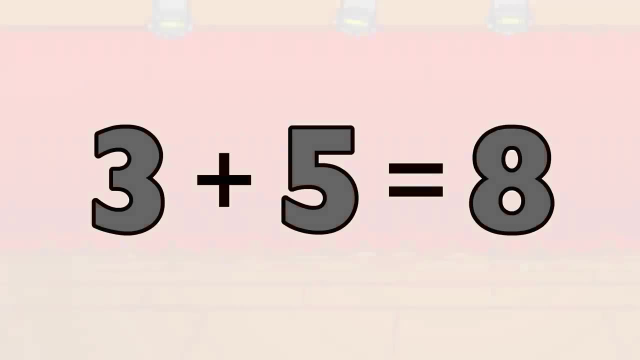 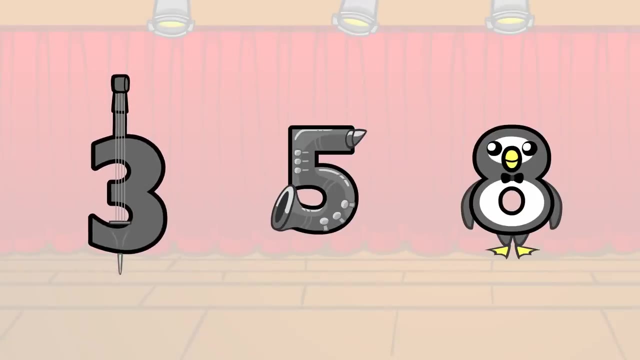 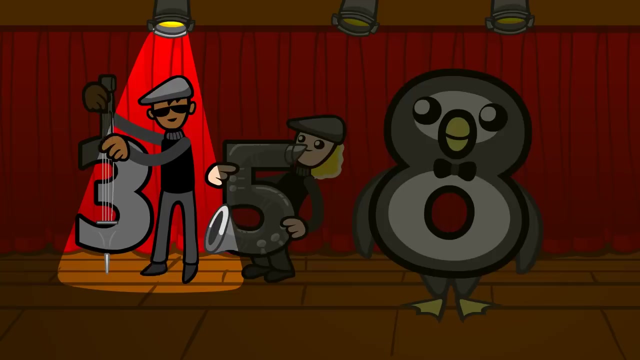 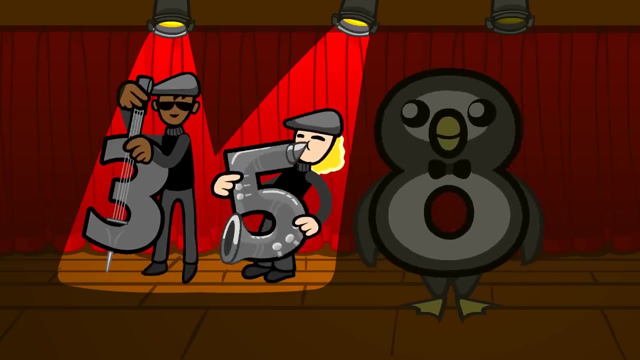 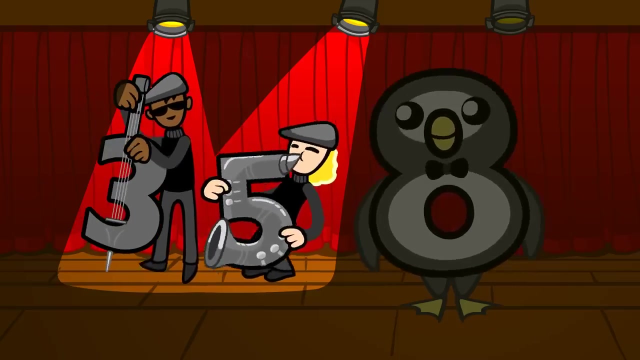 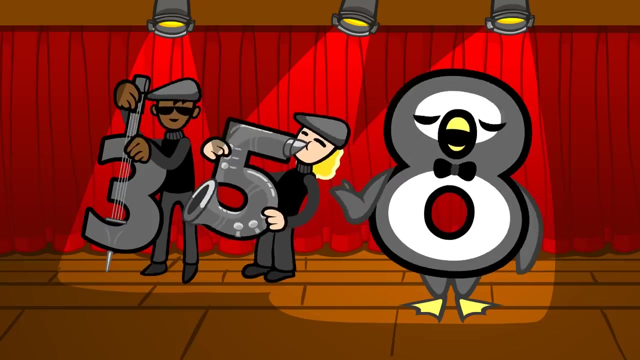 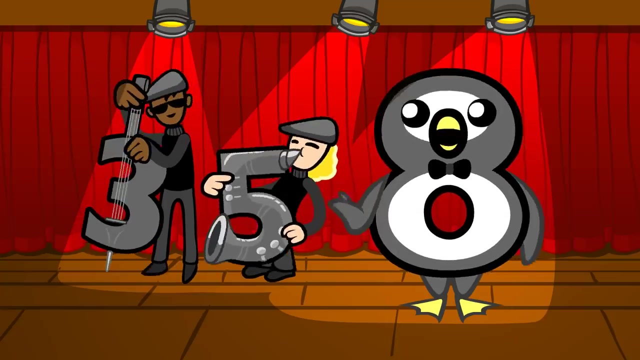 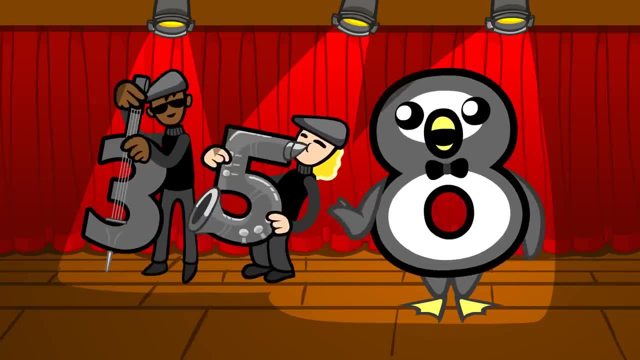 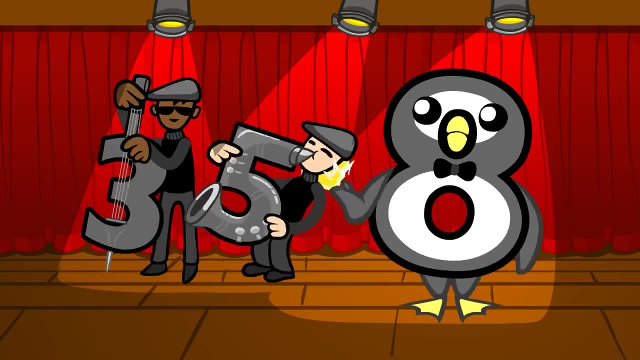 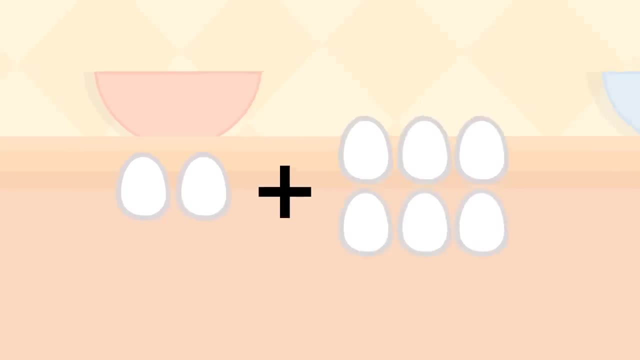 2 plus 6 equals 8.. 2 plus 6 equals 8.. Plus six equals eight. One, two, three, four, five, six, seven. eight equals one, two, three, four, five, six, seven, eight. 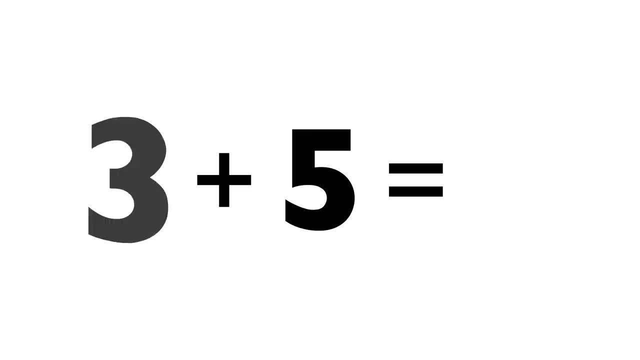 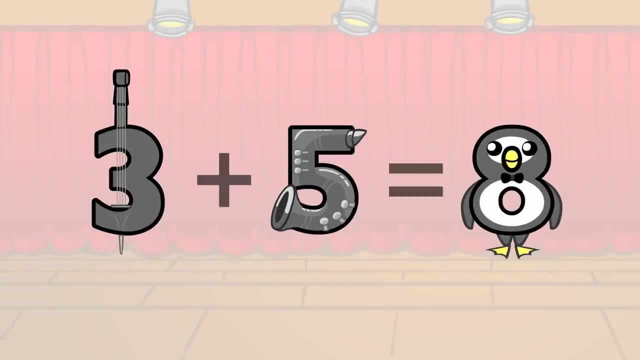 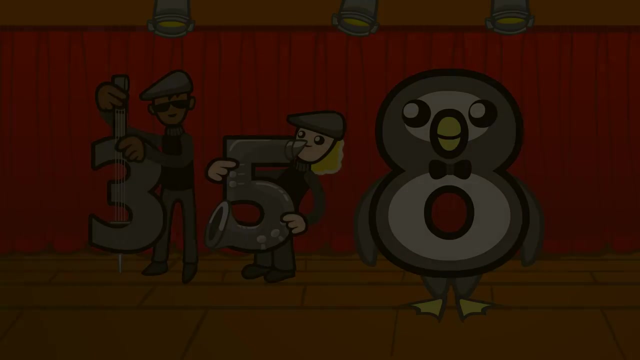 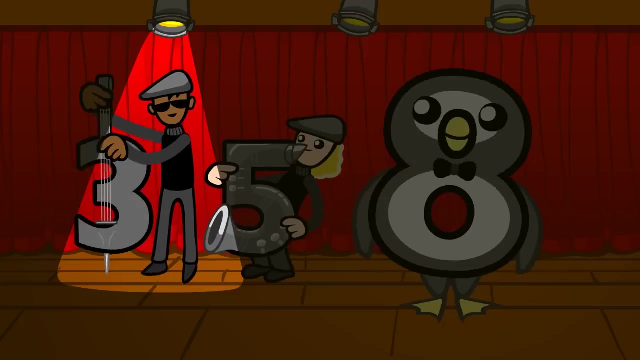 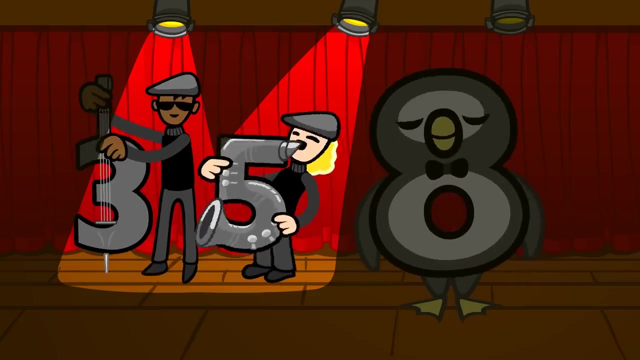 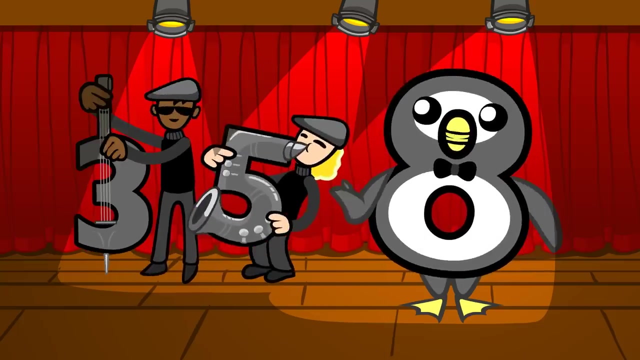 Three plus five equals eight. Three plus five equals eight. One, two, three, four, five, six, seven. eight equals one, two, three, four, five, six, seven, eight, Ba da ba da ba. three plus five equals eight, eight, eight. 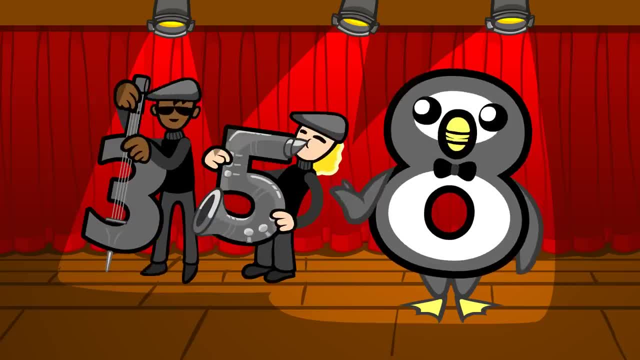 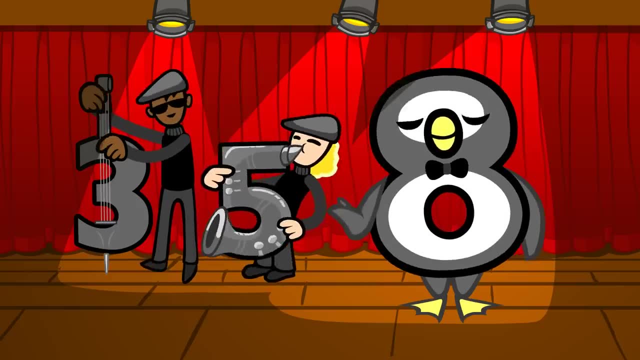 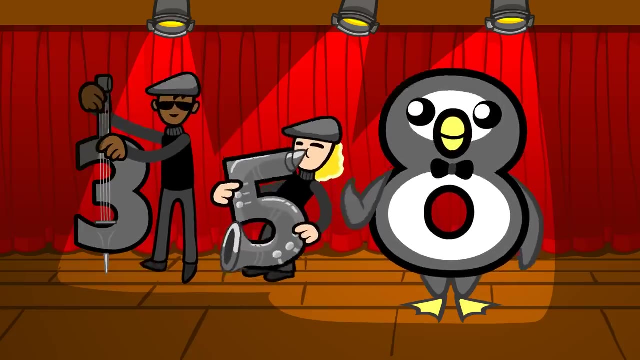 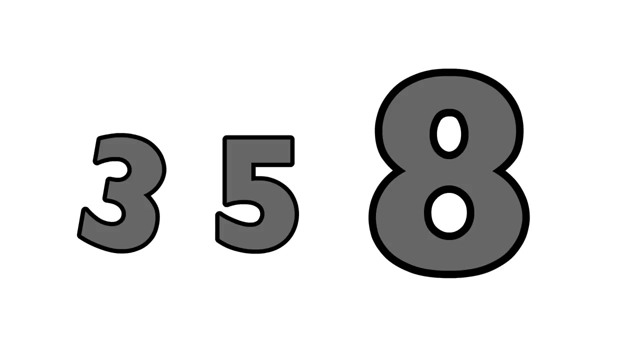 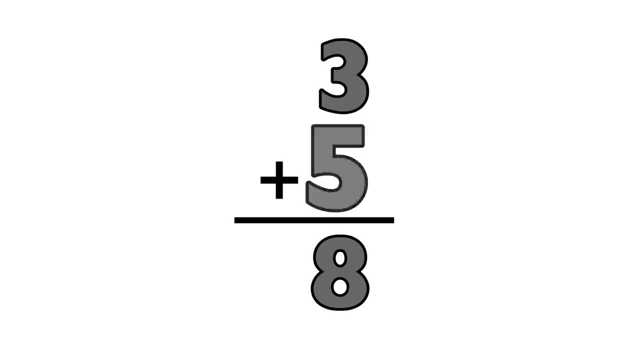 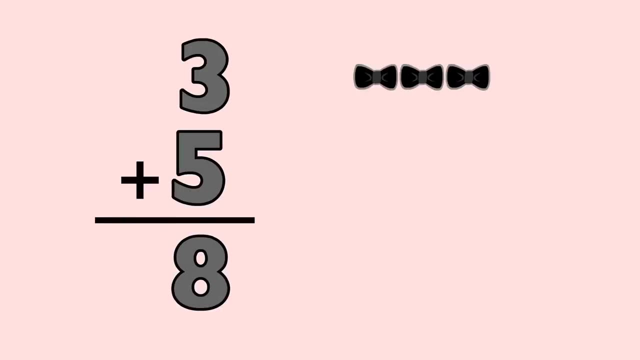 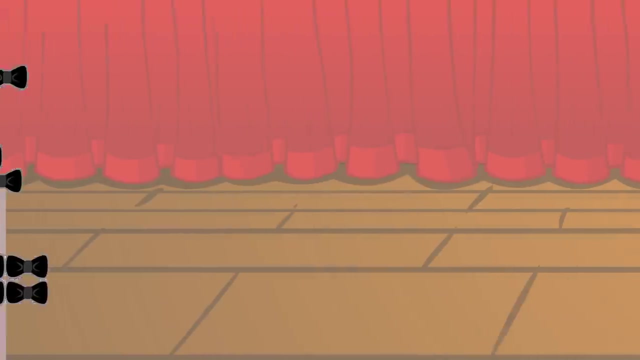 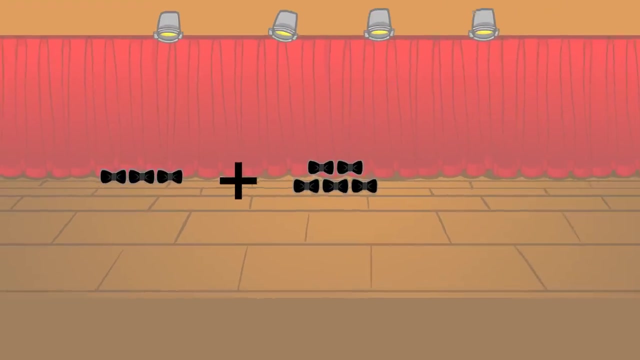 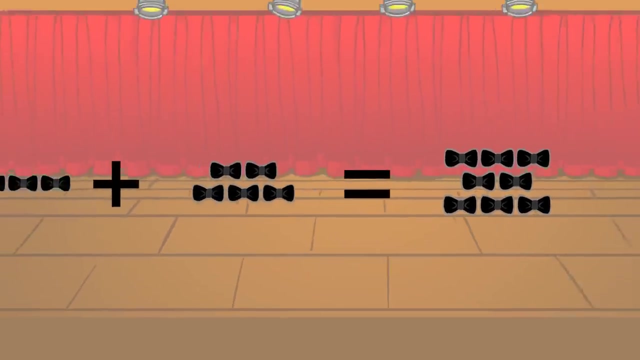 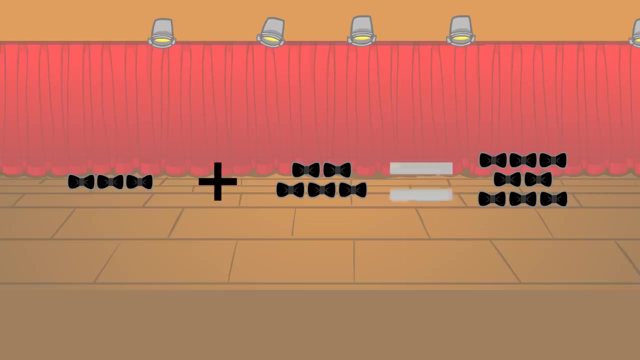 3 plus 5 equals 8.. 3 plus 5 equals 8.. 3 plus 5 equals 8.. 1,, 2,, 3,, 4,, 5,, 6,, 7,, 8 equals. 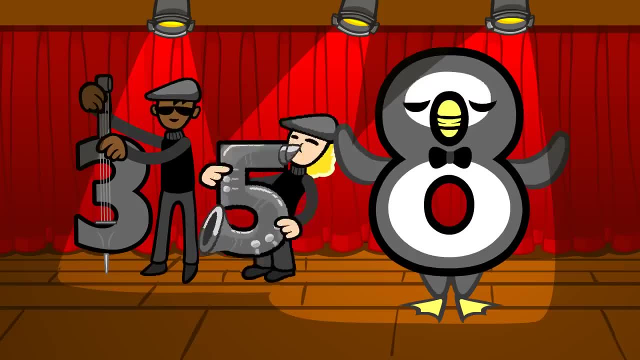 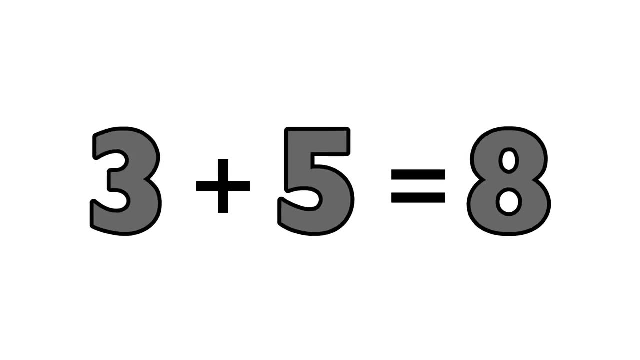 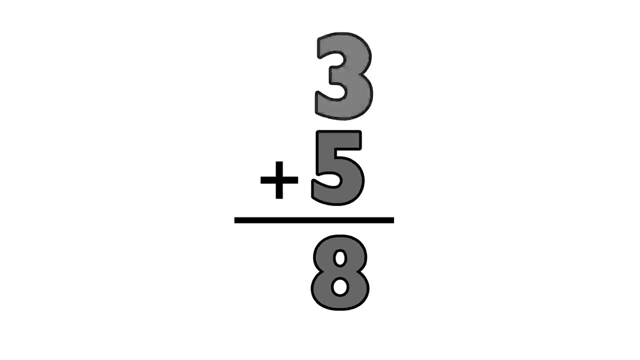 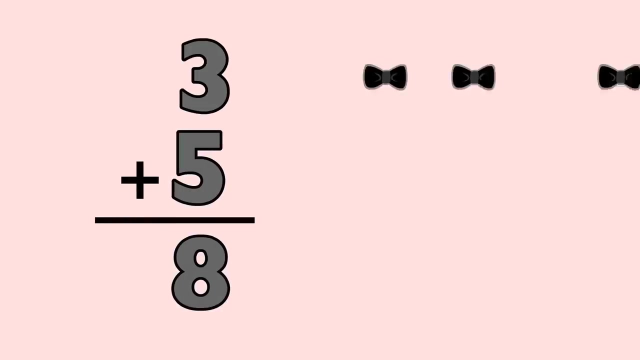 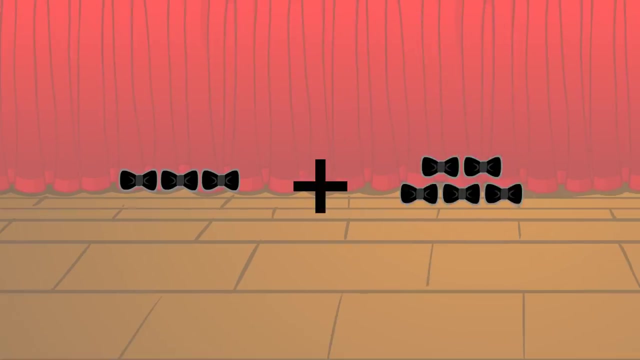 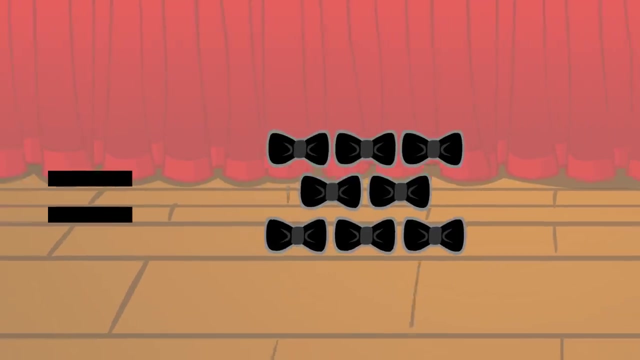 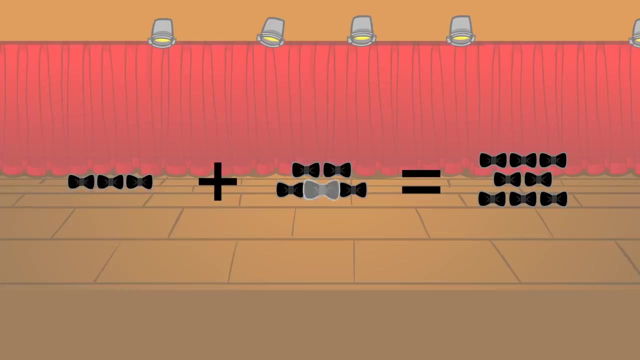 3 plus 5 equals 8. 3 plus 5 equals 8. 3 plus 5 equals 8. Three plus five equals eight. Three plus five equals eight. One, two, three, four, five, six, seven, eight equals. 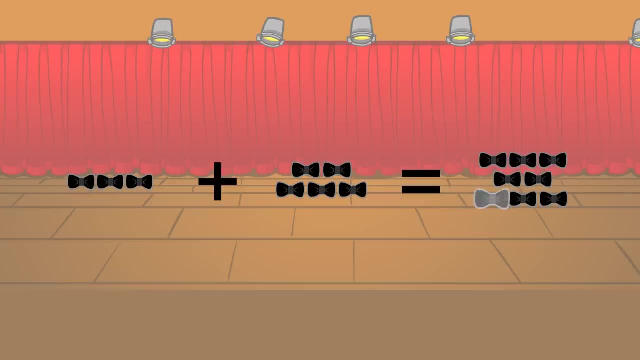 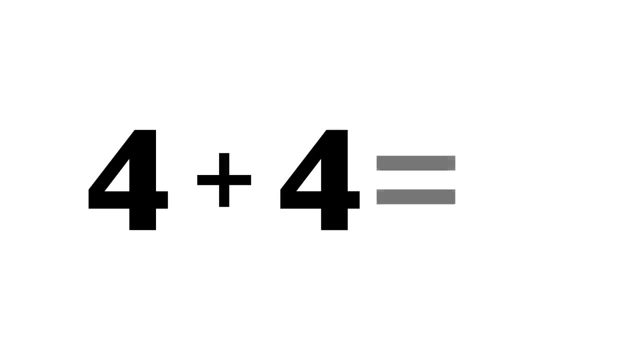 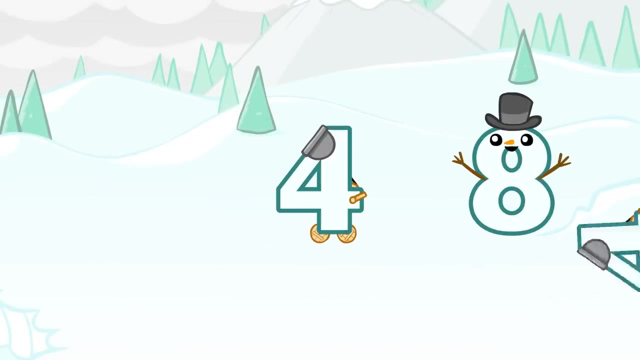 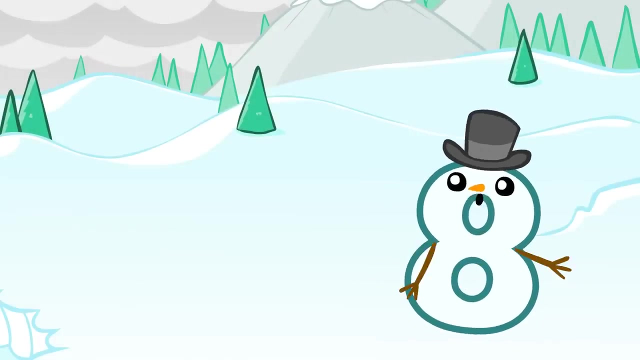 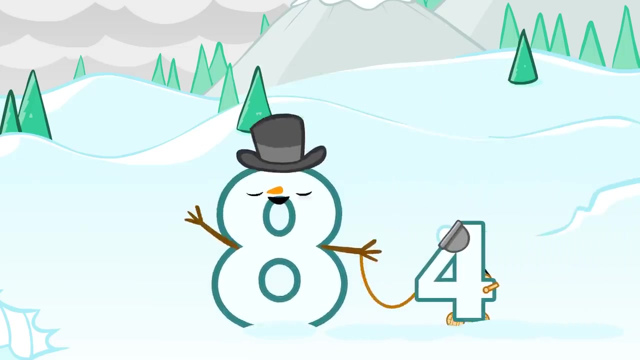 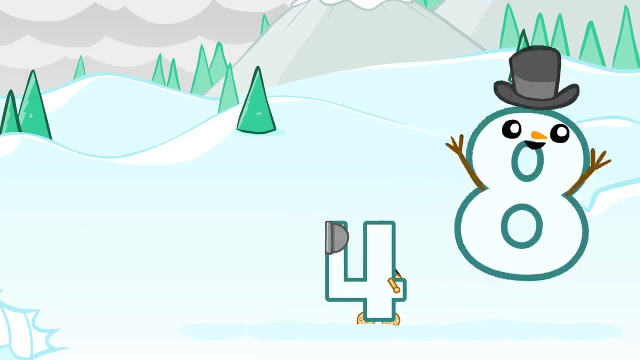 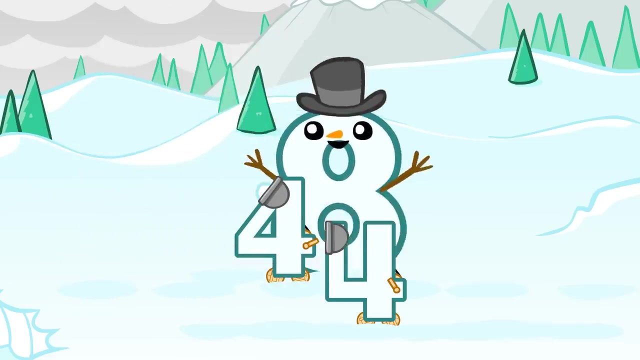 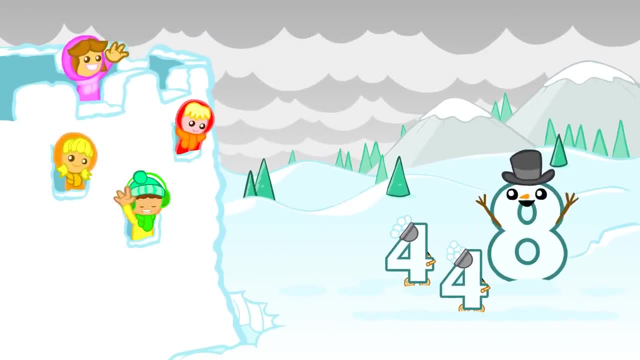 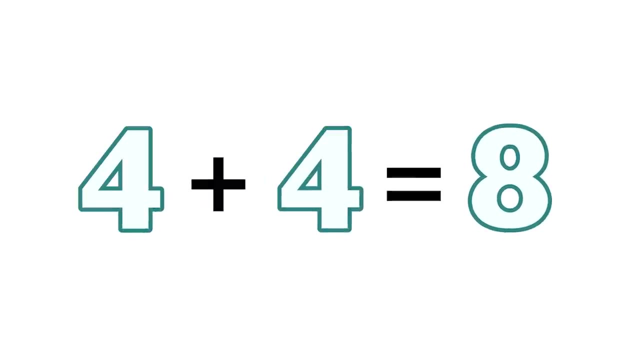 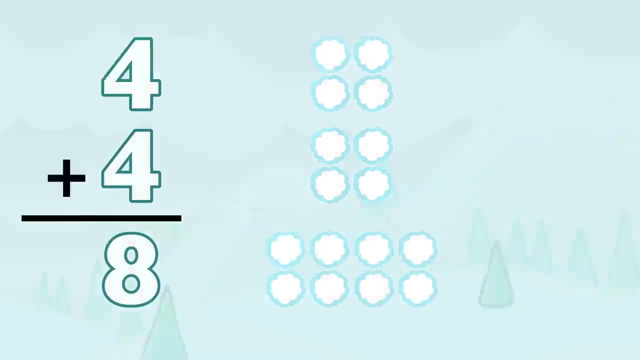 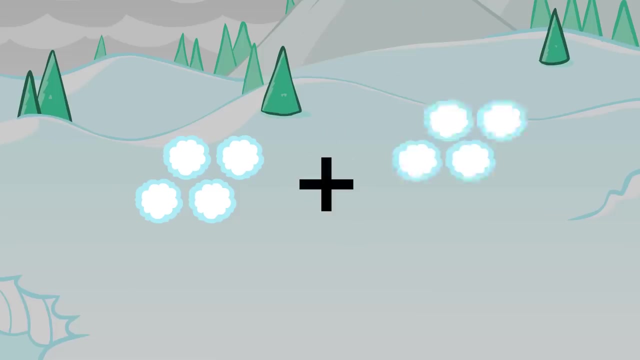 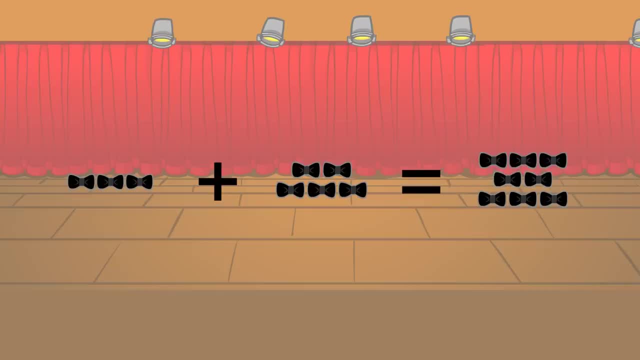 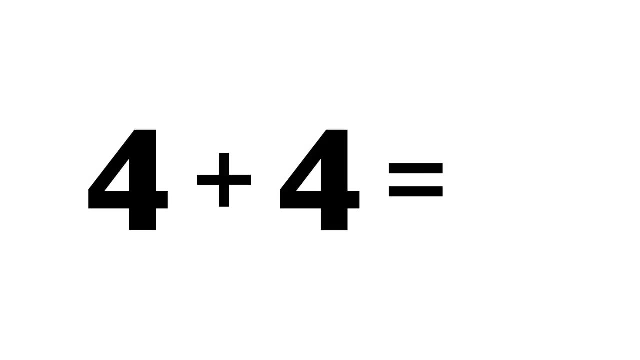 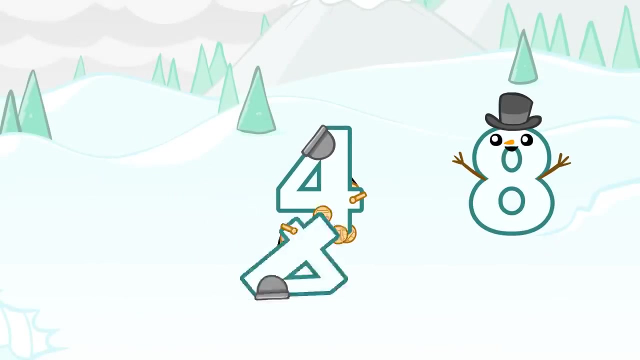 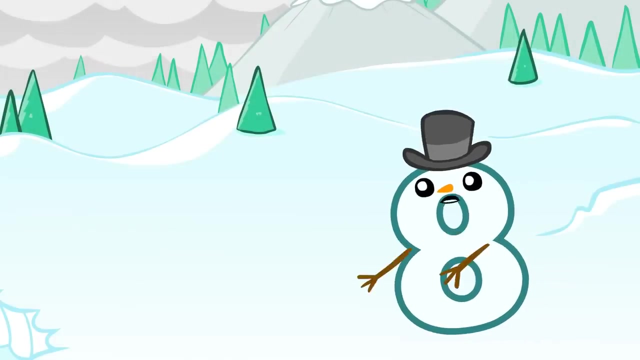 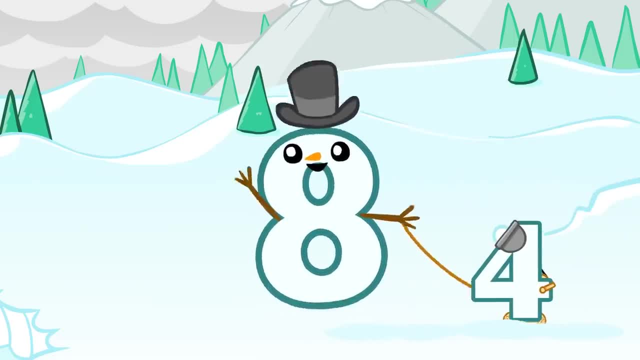 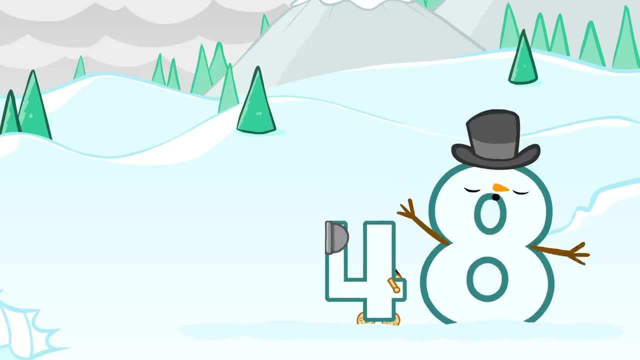 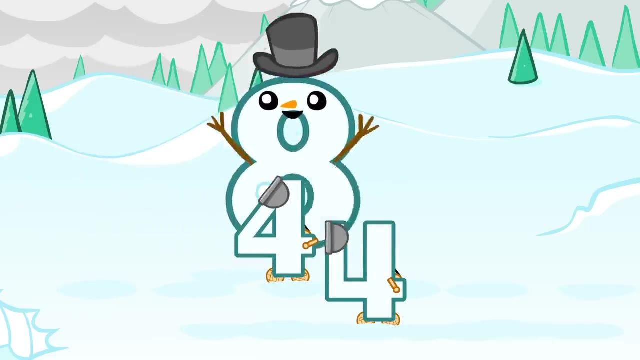 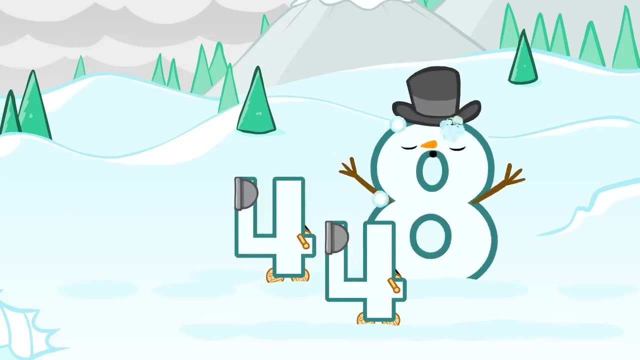 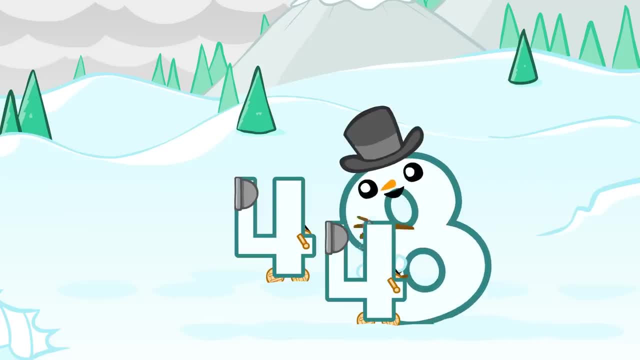 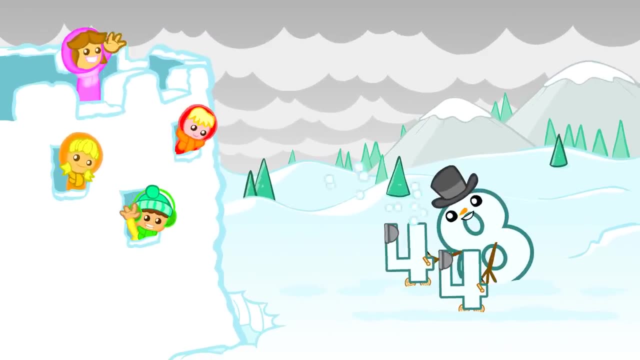 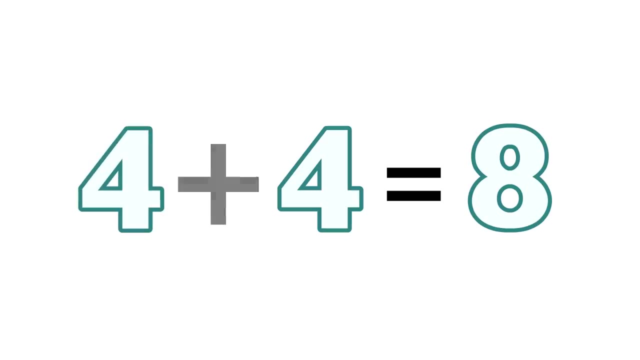 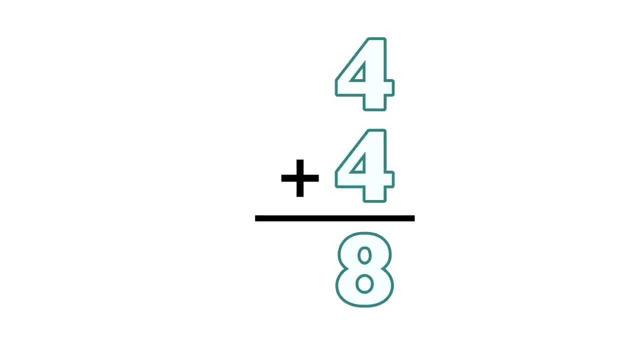 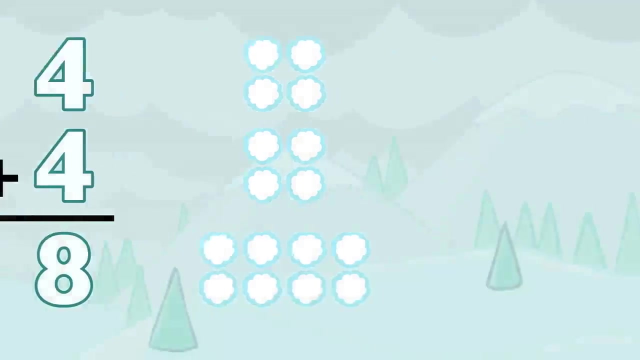 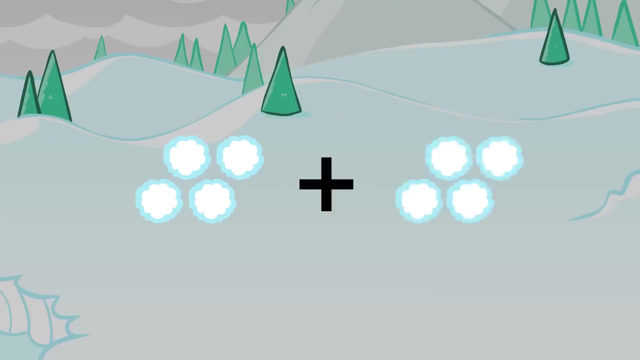 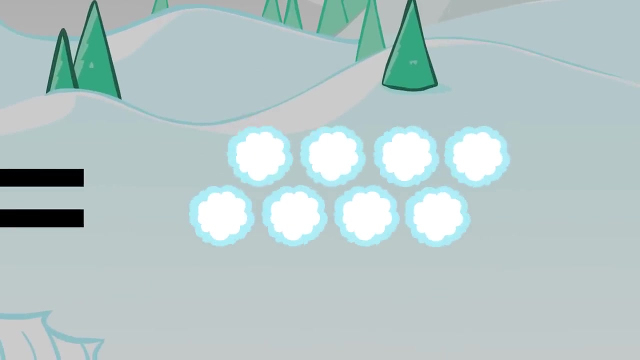 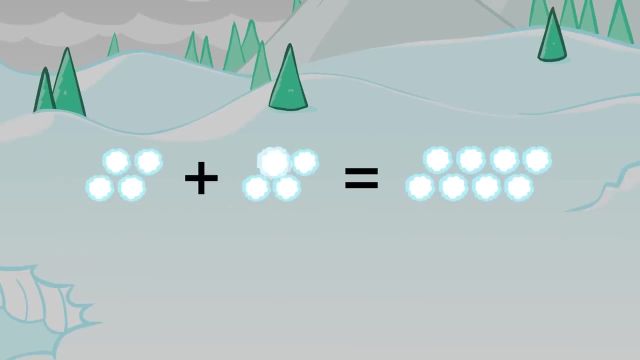 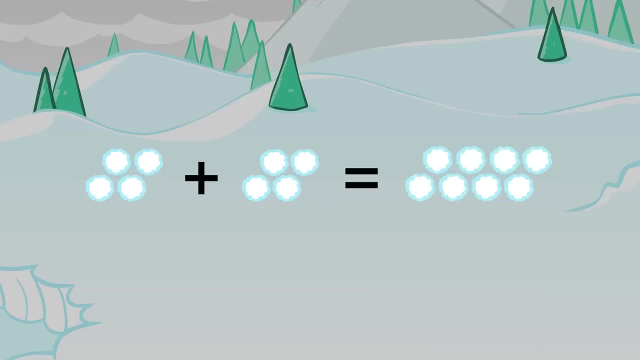 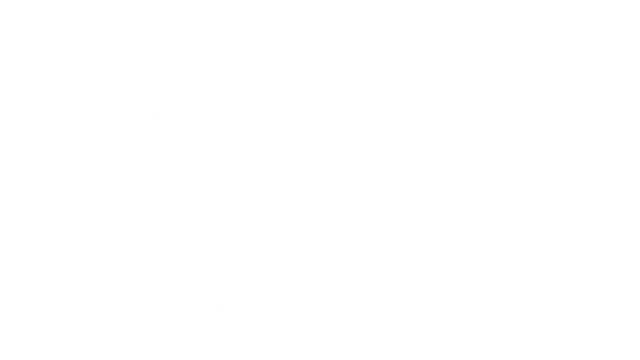 equals 1,, 2,, 3,, 4,, 5,, 6,, 7,, 8: 1,, 2,, 3,, 4,, 5,, 6,, 7,, 8, 1 plus 7. 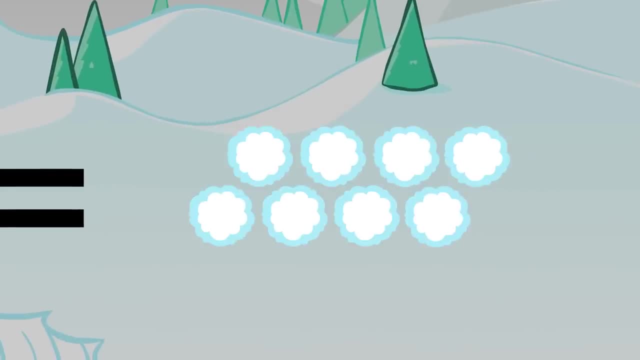 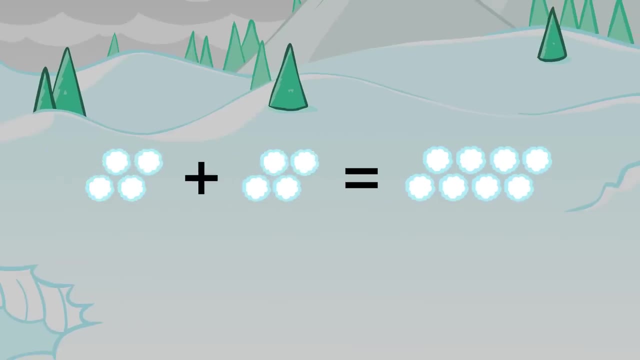 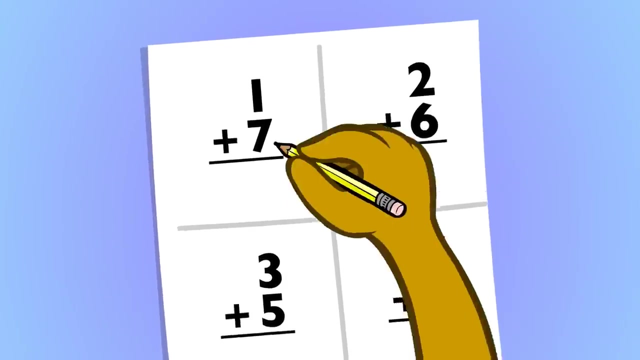 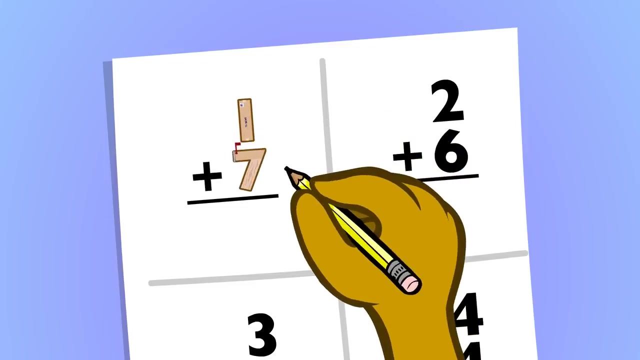 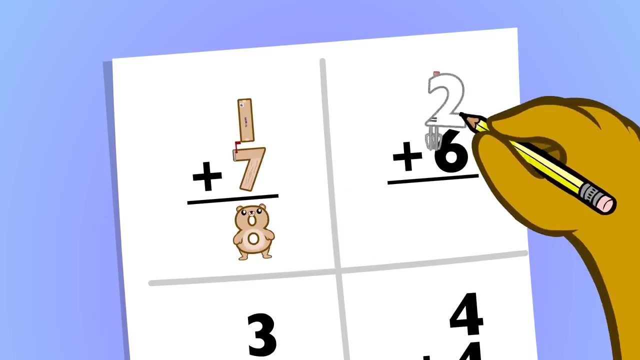 Four plus four equals eight. One, two, three, four, five, six, seven, eight equals One, two, three, four, five, six, seven, eight. Four plus four equals eight. 7 equals 2 plus 6 equals. 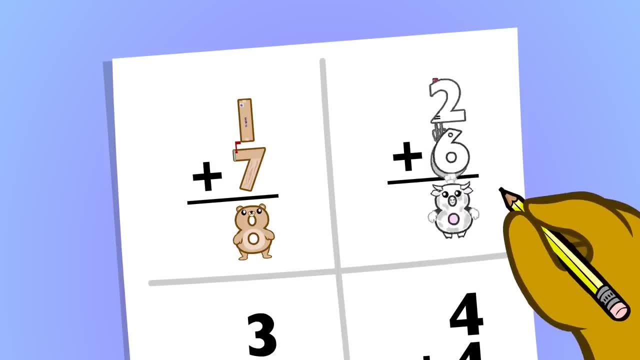 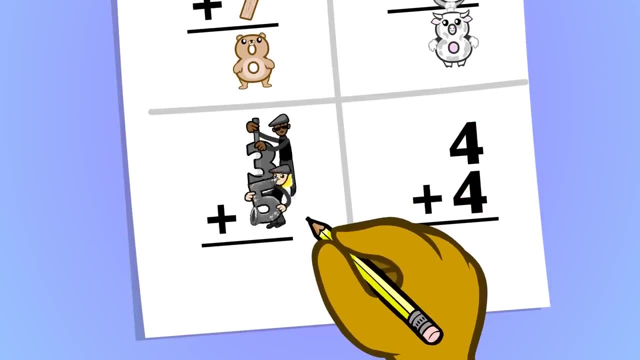 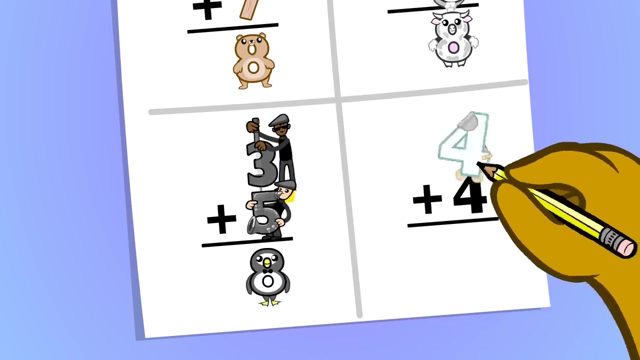 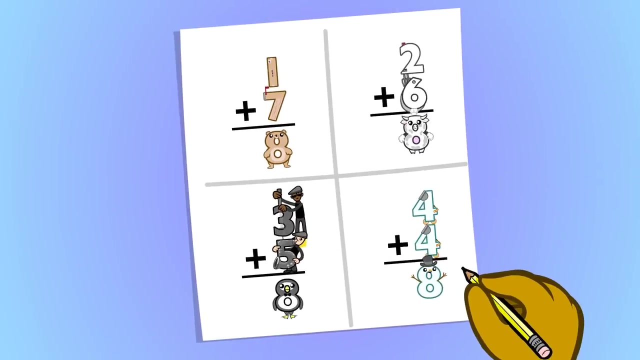 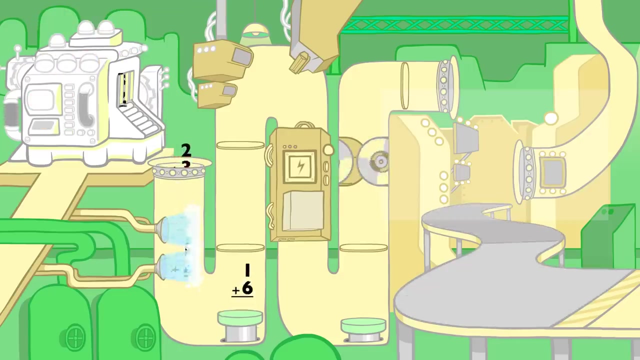 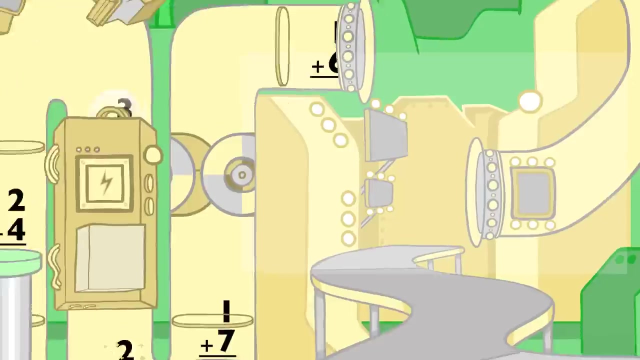 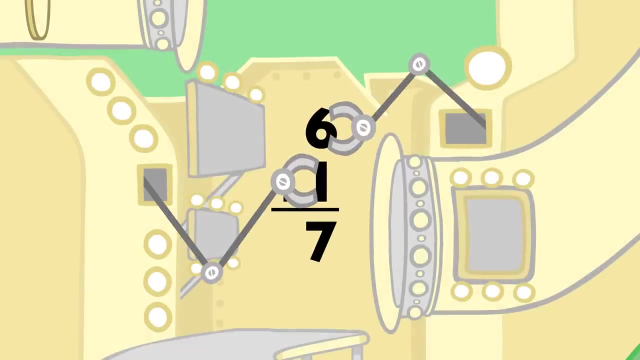 8, 3 plus 5 equals 8. 4 plus 4 equals, 4 plus 4 equals 8. 1 plus 6 equals 7, and 6 plus 1 equals 7, 1 plus 7 equals 8, and 7 plus 1 equals 8. 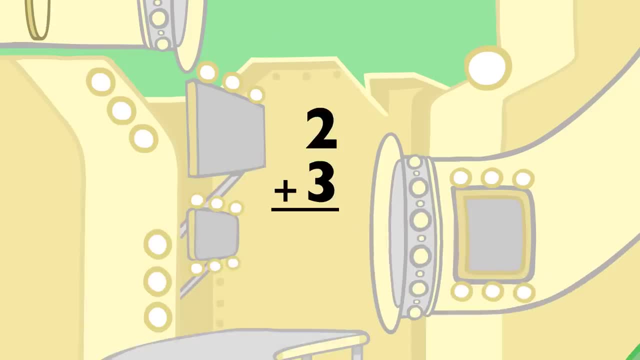 2 plus 3 equals 5. 3 plus 2 equals 5. 2 plus 4 equals 6. 4 plus 2 equals 6. 2 plus 5 equals 7. 5 plus 2 equals 7. 2 plus 6 equals 8. 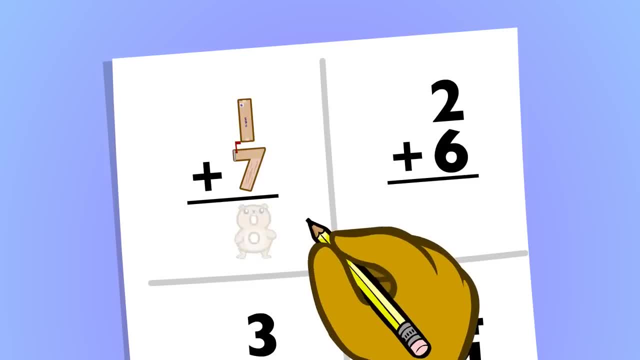 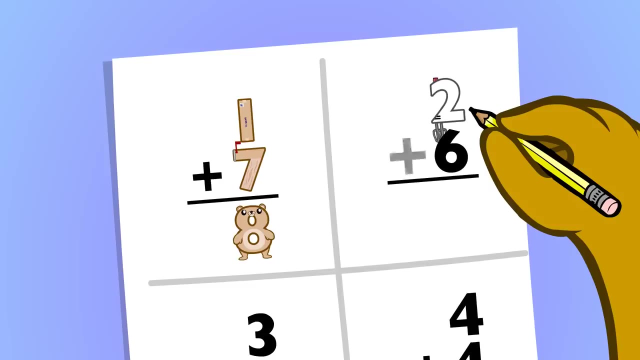 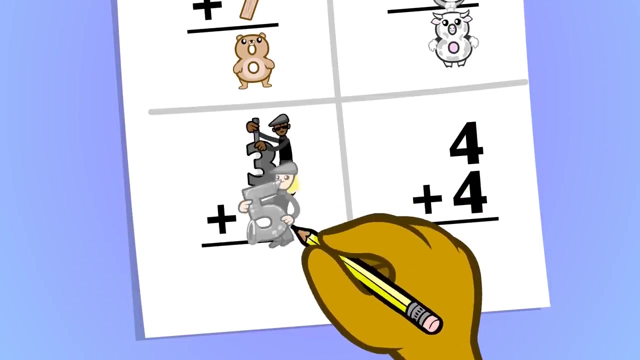 equals 8: 1,, 2,, 3,, 4,, 5,, 6, 7, 8. equals 1: 1, 2,, 3,, 4,, 5,, 6,, 7, 8. 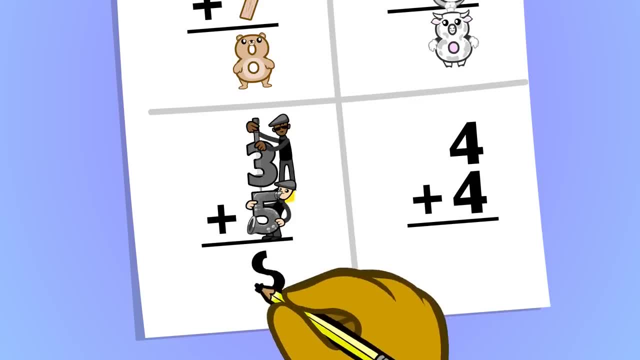 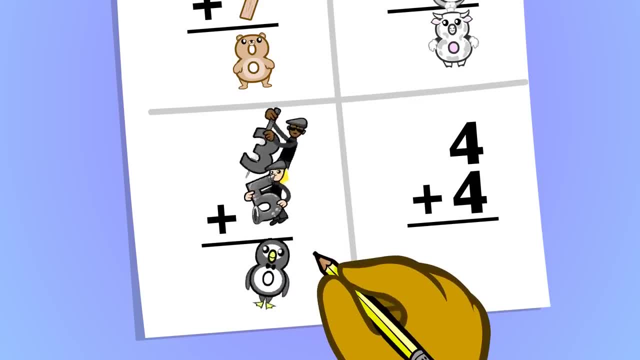 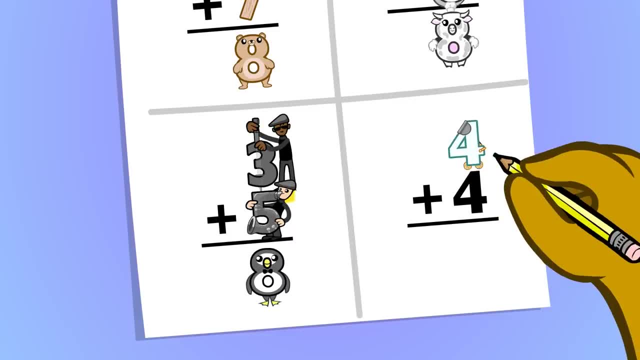 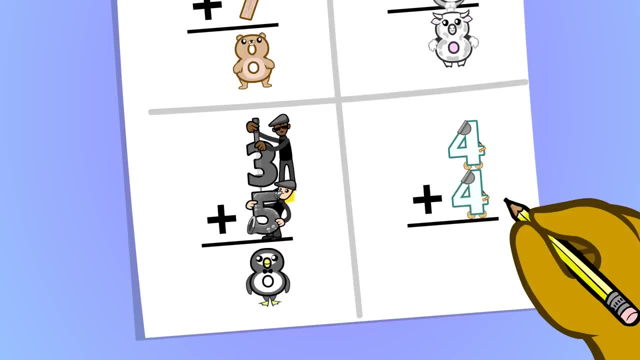 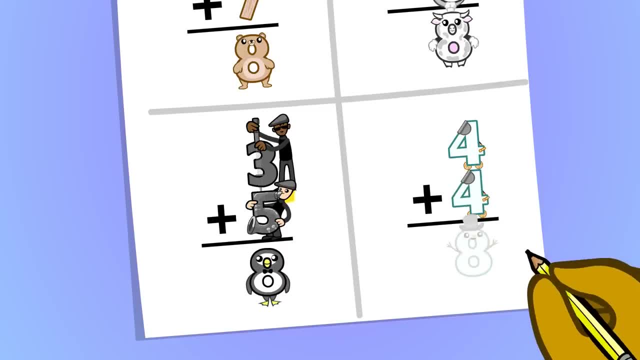 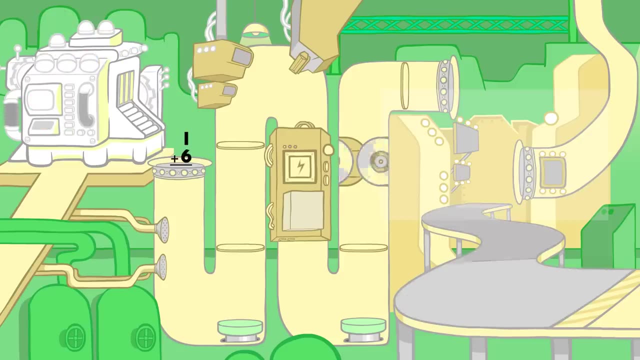 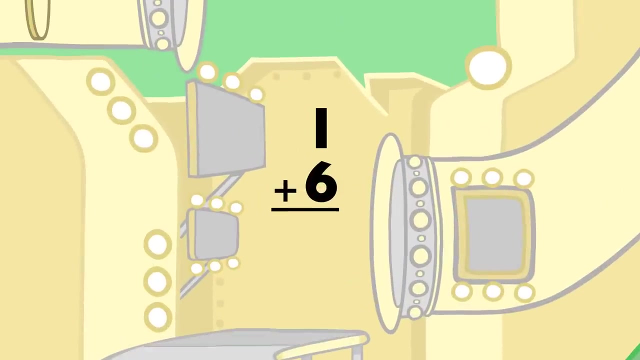 equals 1, 1,, 2,, 3,, 4,, 5,, 6, 7, 8 equals 1. 1 plus 6 equals 7.. And 6 plus 1 equals 7.. 1 plus 7 equals 8.. 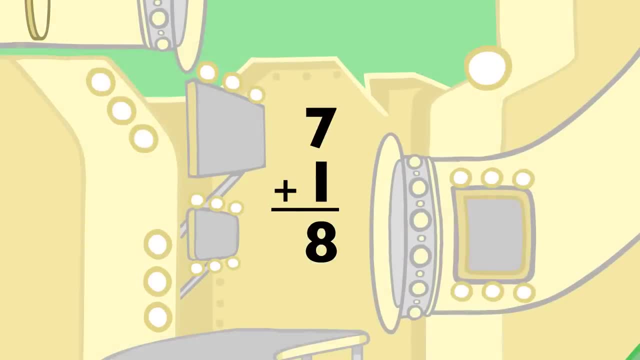 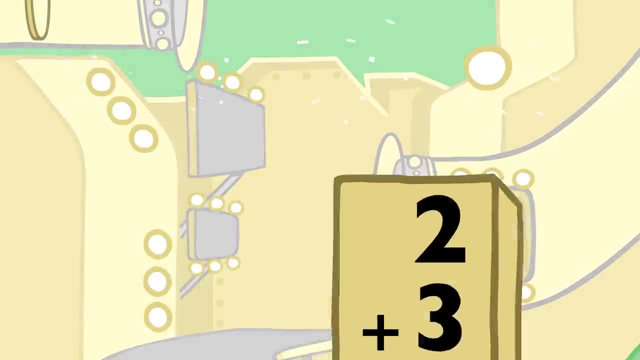 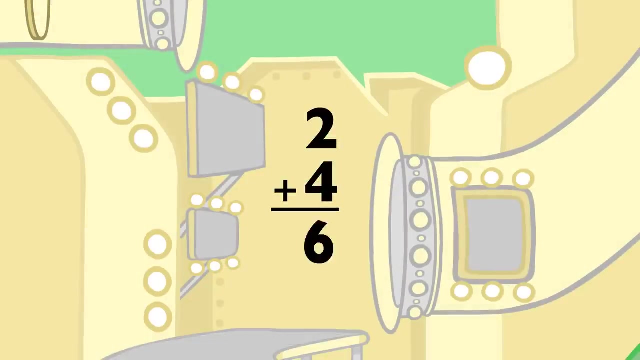 And 7 plus 1 equals 8.. 2 plus 3 equals 5.. 3 plus 2 equals 5.. 2 plus 4.. 4 plus 2 equals 6.. 2 plus 5 equals 7.. 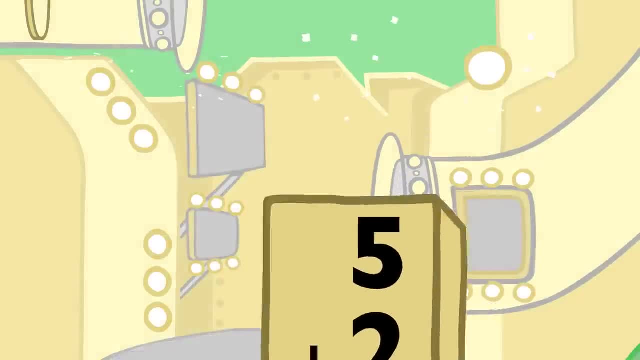 5 plus 2 equals 7.. 2 plus 6 equals 8.. 6 plus 2 equals 8.. 3 plus 4 equals 7.. 4 plus 3 equals 8. 7.. 8 plus 1 equals 7.. 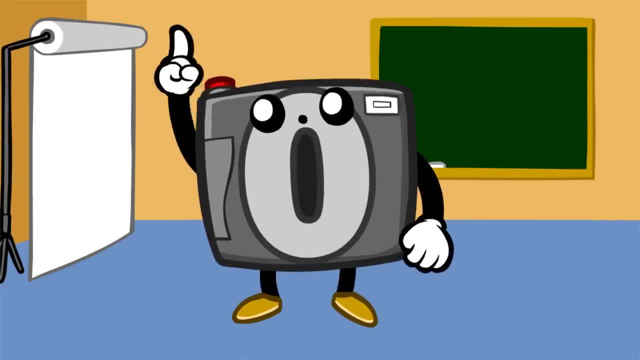 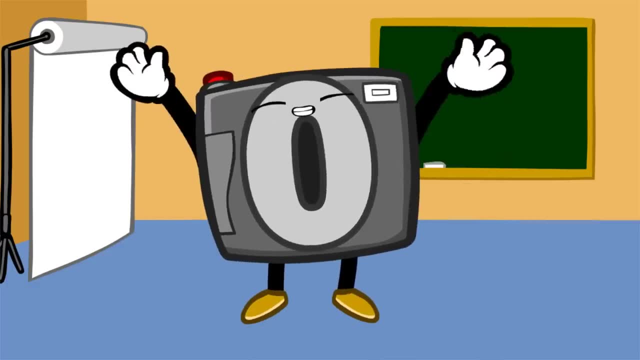 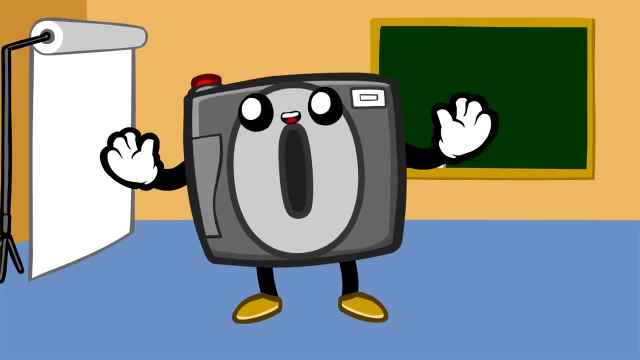 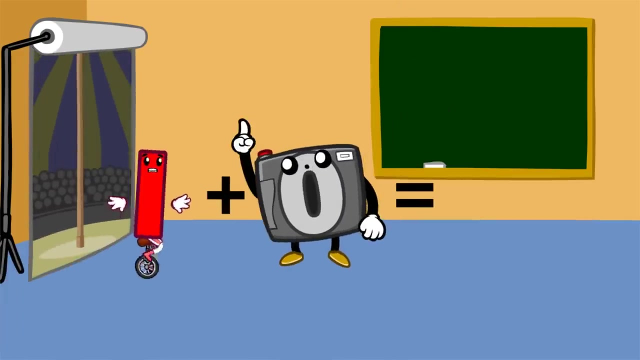 If you play the zero game when you add me, you stay the same. I'll take your picture. Just say cheese And don't forget to smile. please Watch this. If you play the zero game When you add me, you stay the same. 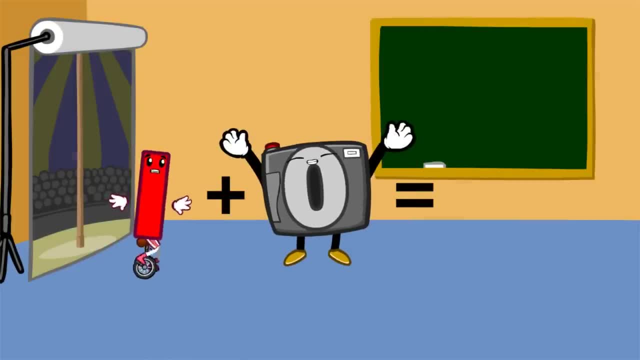 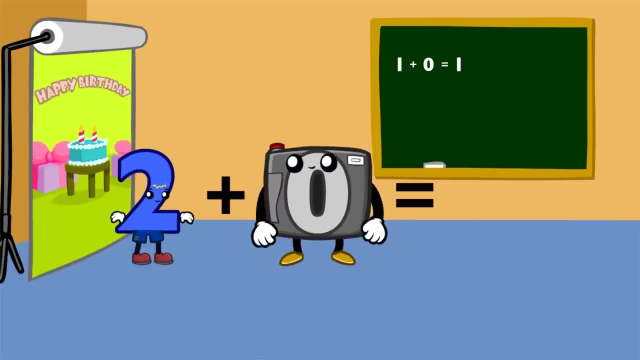 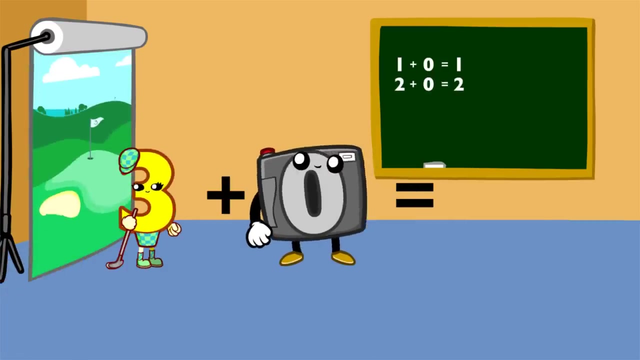 I'll take your picture. Just say cheese And don't forget to smile, please. One plus zero equals one. If you play the zero game, When you add me, you stay the same. Two plus zero equals two. I'll take your picture. Just say cheese And don't forget to smile, please. 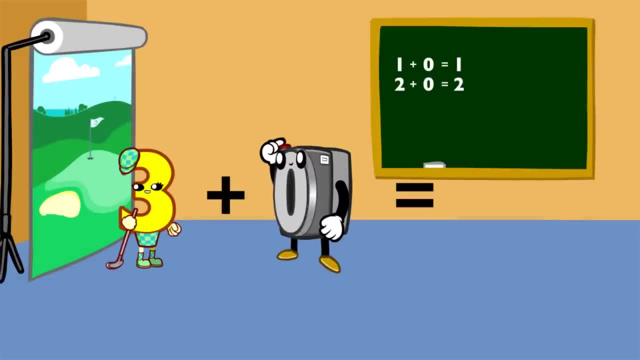 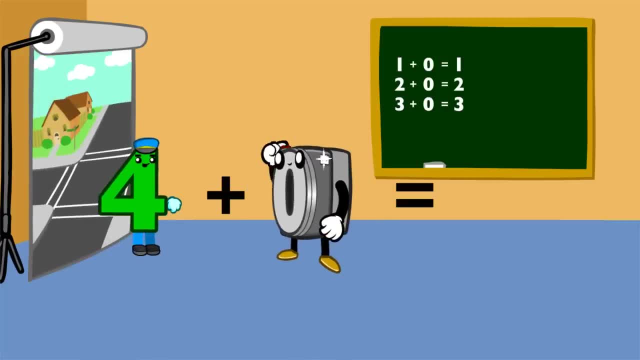 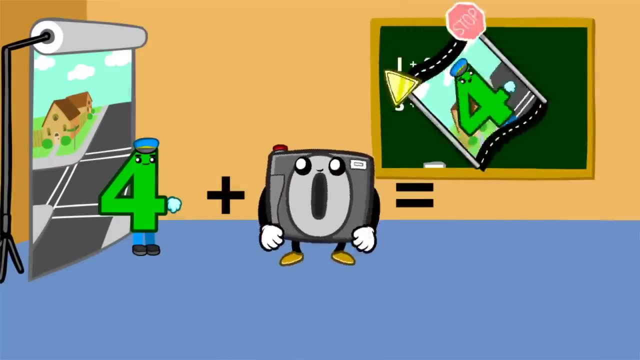 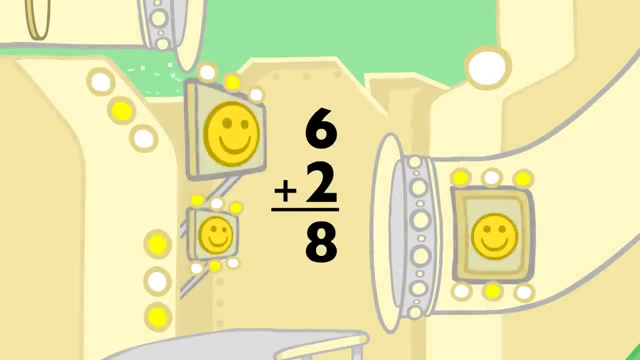 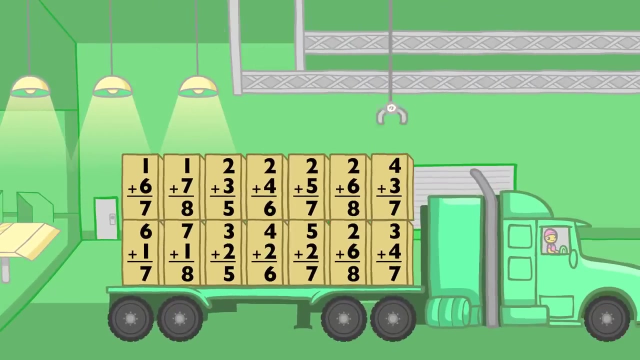 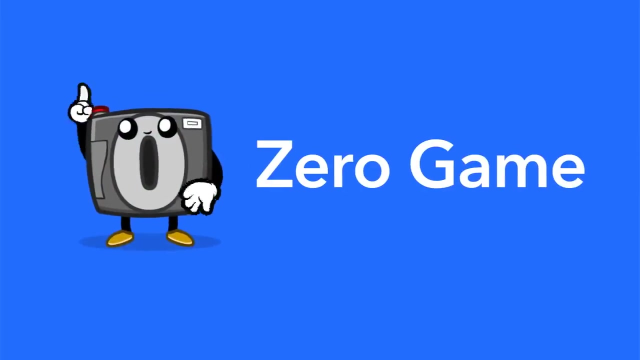 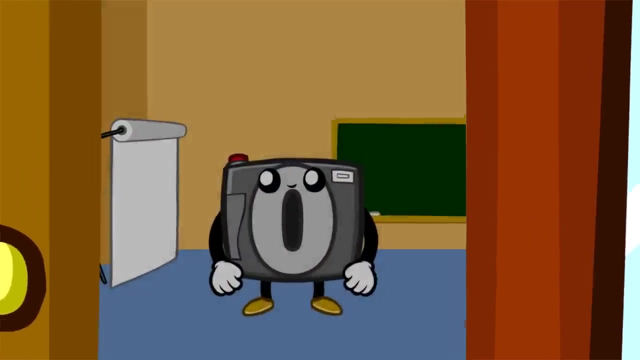 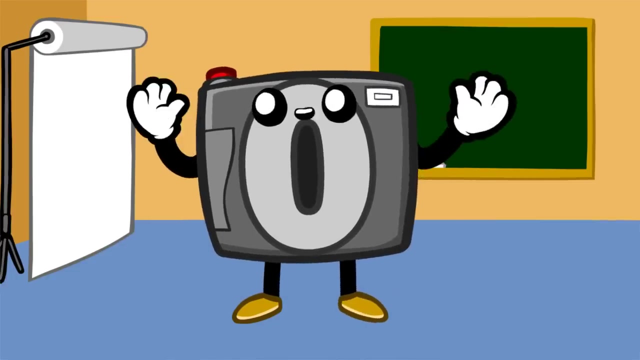 6 plus 2 equals 8. 3 plus 4 equals 7. 4 plus 3 equals 7. 3 plus 9 equals 8. If you play the zero game, When you add me, you stay the same. I'll take your picture, just say cheese. 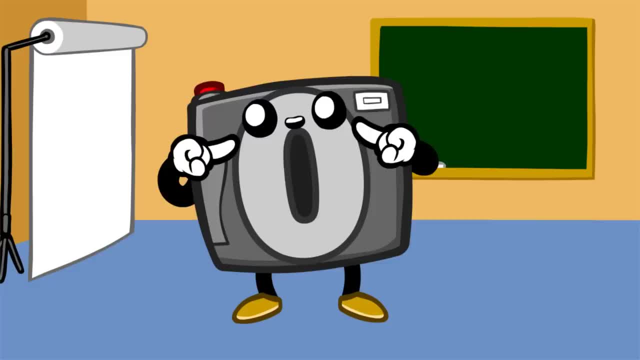 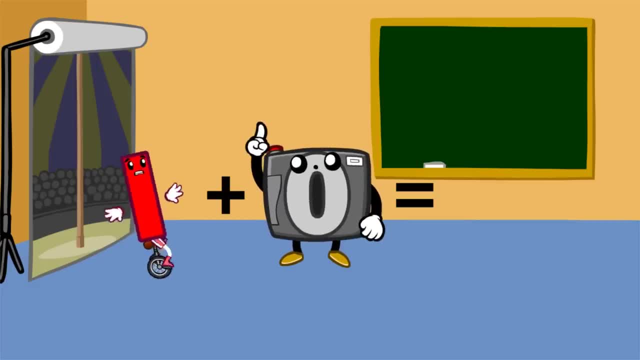 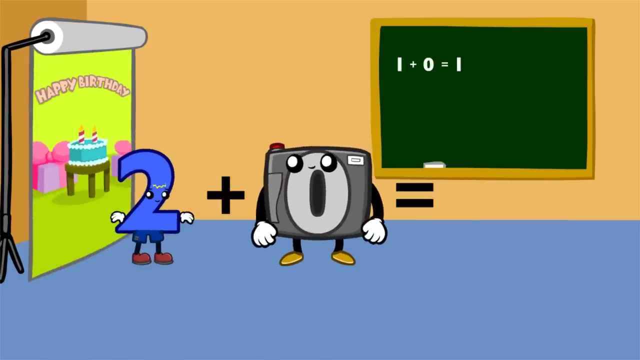 If you play the zero game when you add me, you stay the same. I'll take your picture. Just say cheese and don't forget to smile, please. One plus zero equals one. If you play the zero game when you add me, you stay the same. 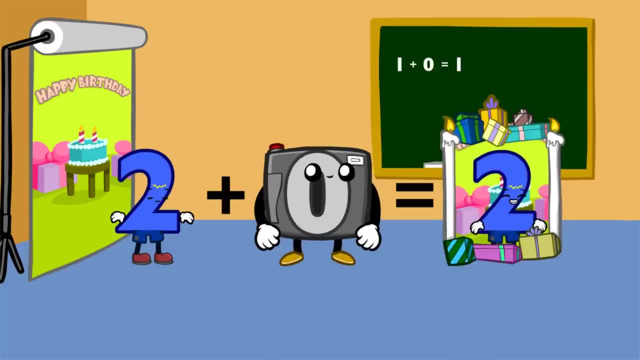 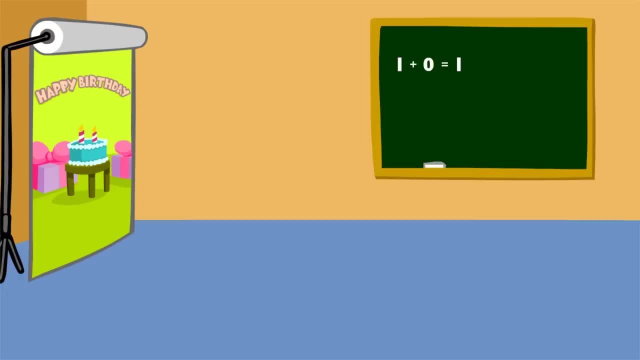 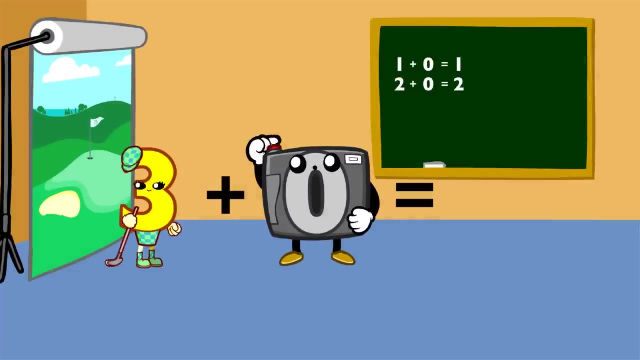 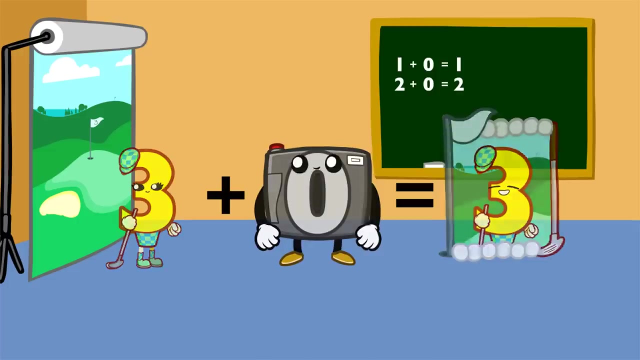 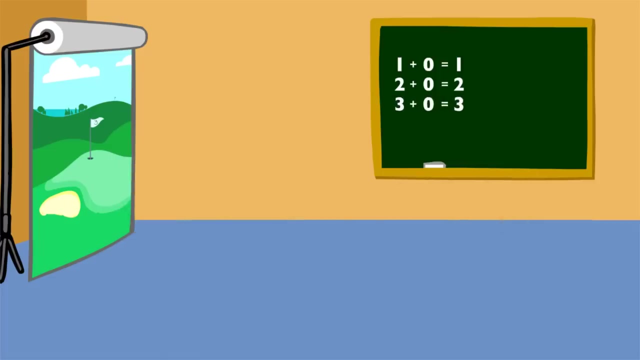 Two plus zero equals two. I'll take your picture. Just say cheese and don't forget to smile. please Wait a minute. Do you call that a smile? Let's try that again. Three plus zero equals three. Four plus zero equals star. 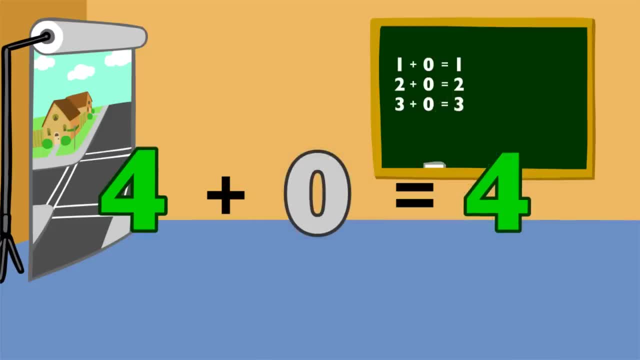 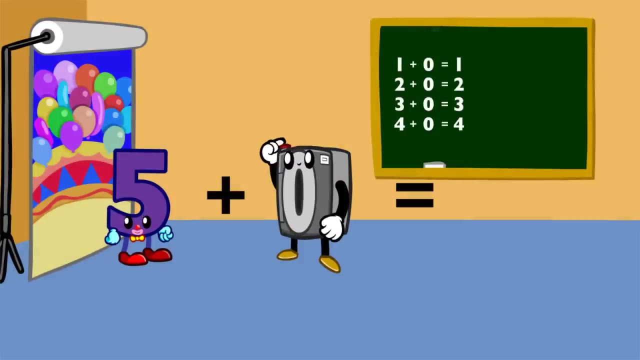 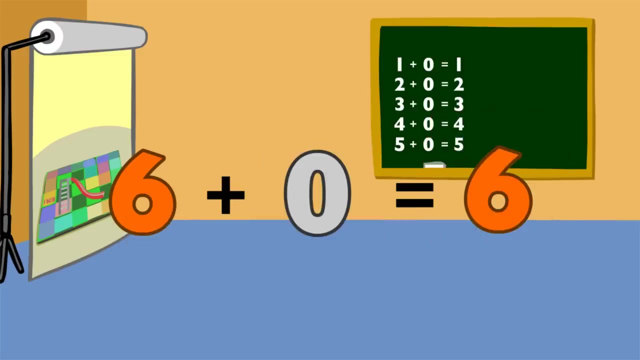 Three plus zero equals zero. Four plus zero equals four. Three plus zero equals one. If you play the zero game, when you stay the same, Just say cheese and don't forget to smile, please. Five plus zero equals five. Six plus zero equals six. 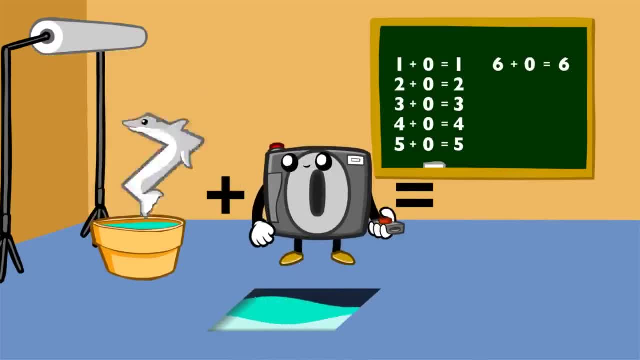 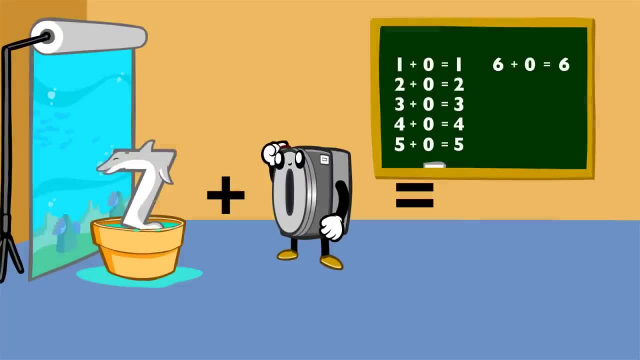 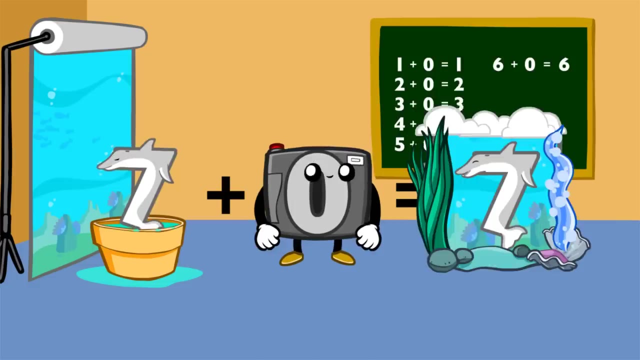 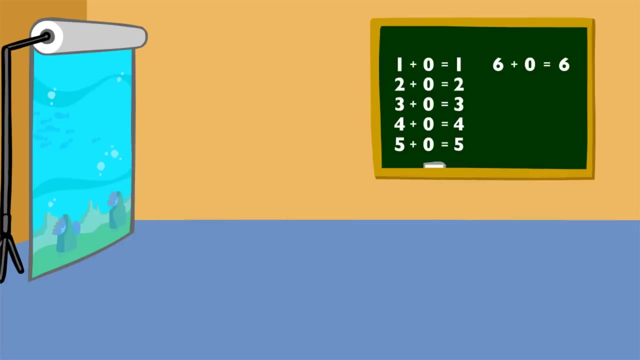 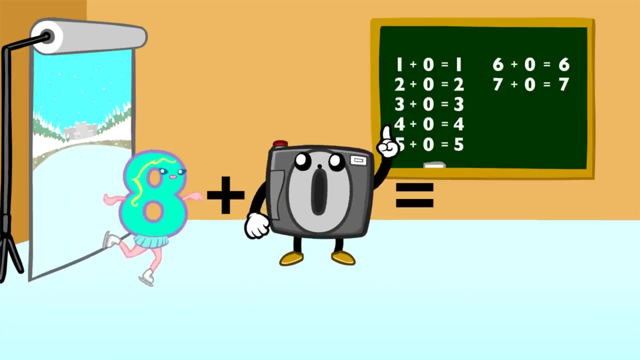 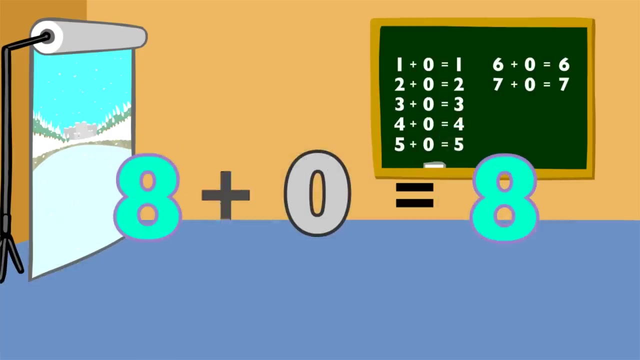 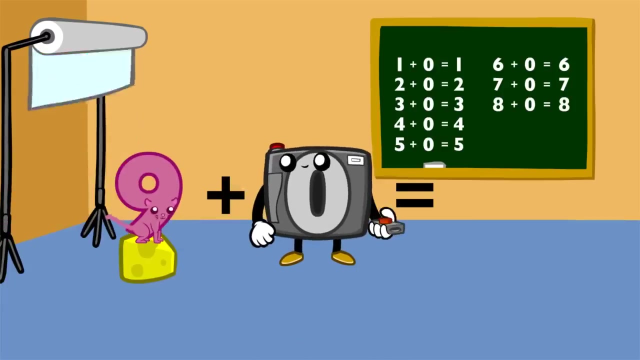 When you add me, you stay the same. Seven plus zero equals seven. And don't forget to smile, please. Eight plus zero equals eight. If you play the zero game, when you add me, you stay the same. I'll take your picture. just say cheese. 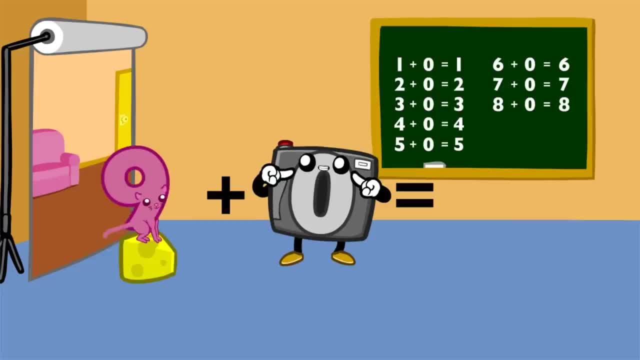 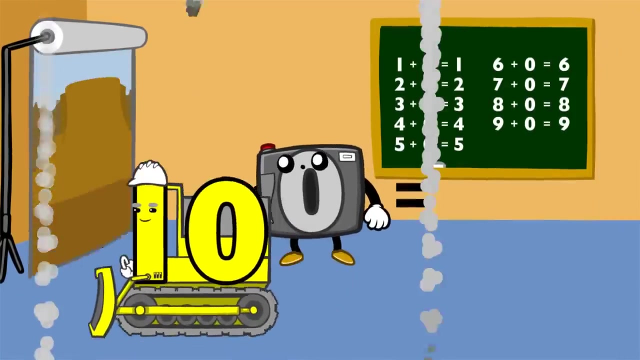 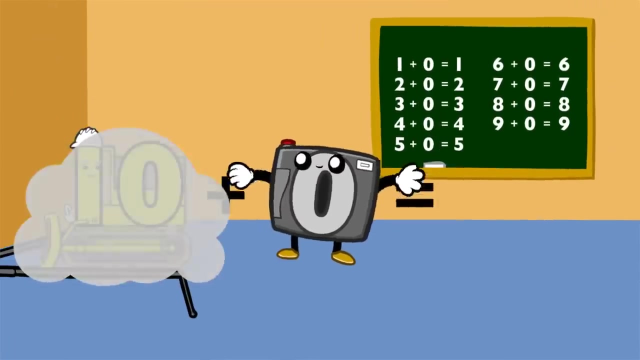 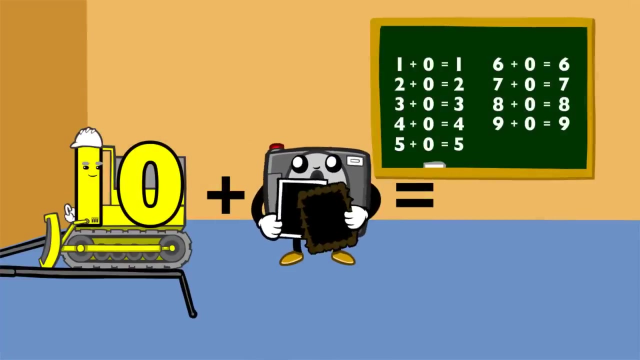 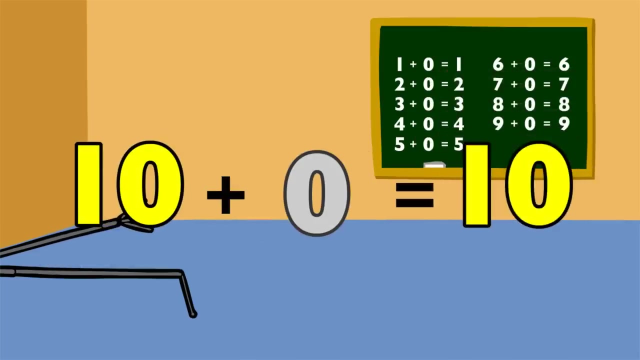 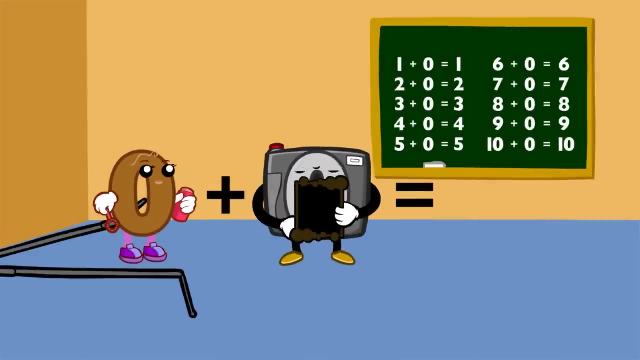 And don't forget to smile, please. Nine plus zero equals. Nine plus zero equals Nine. Ten plus zero equals ten. Heads are up, Children are playing telly with their greatest energy. Nine plus zero equals eight. I knew you could do it. 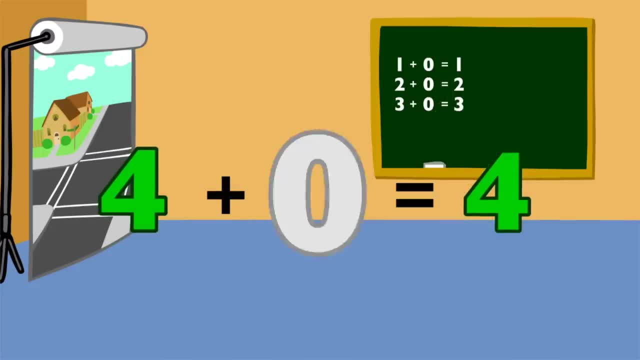 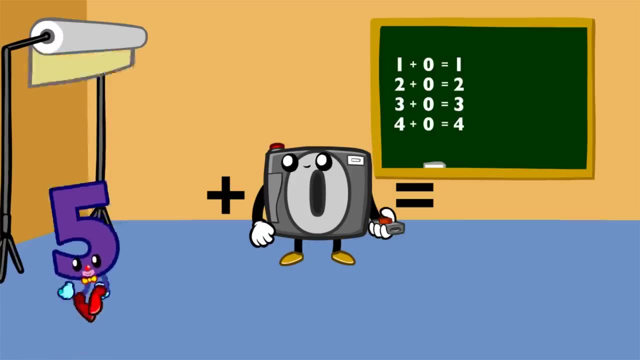 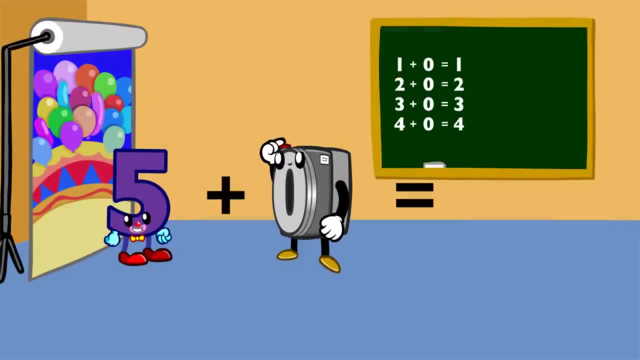 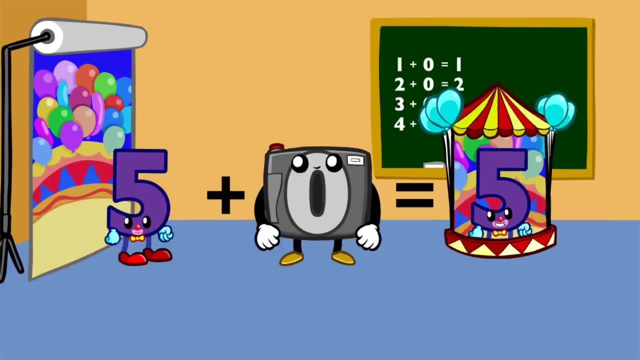 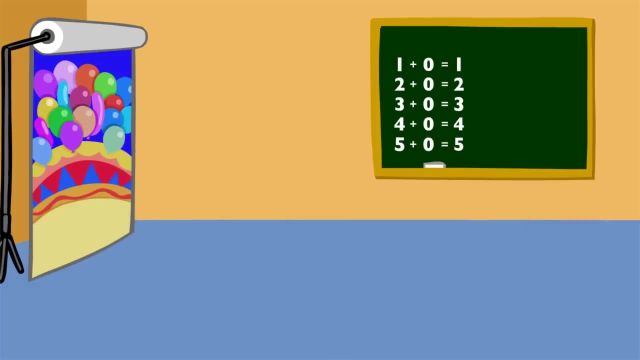 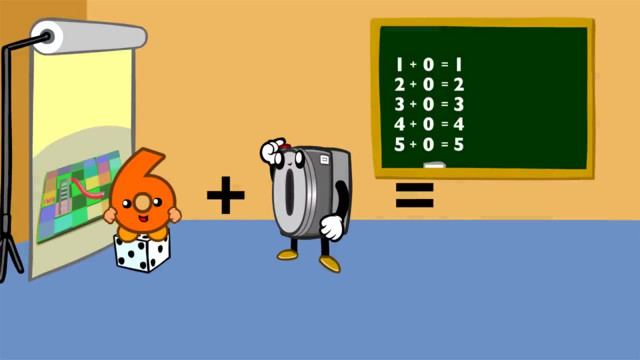 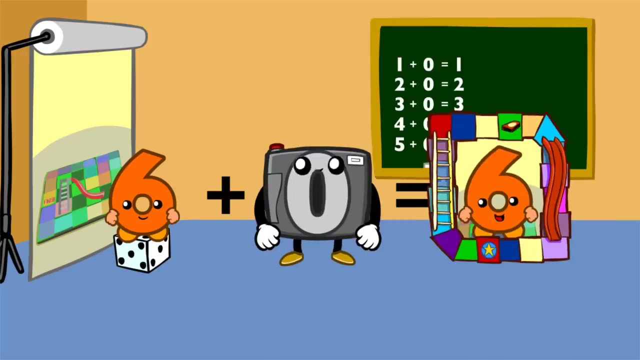 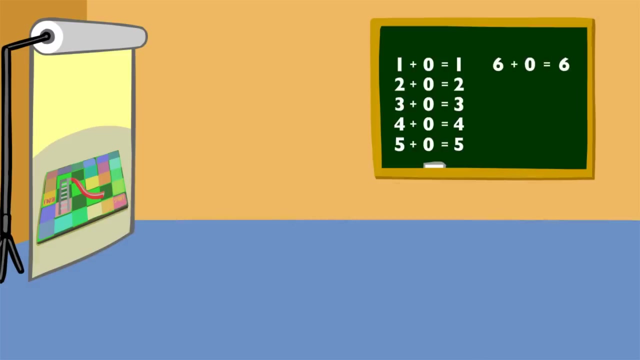 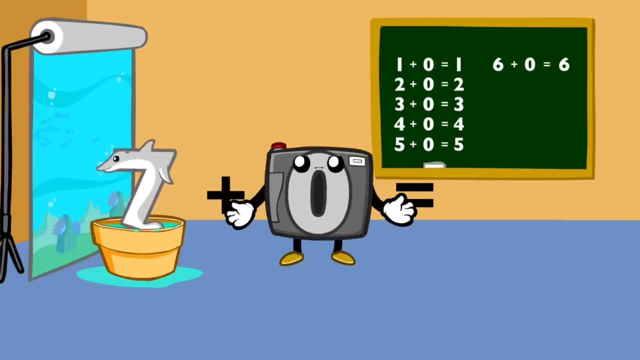 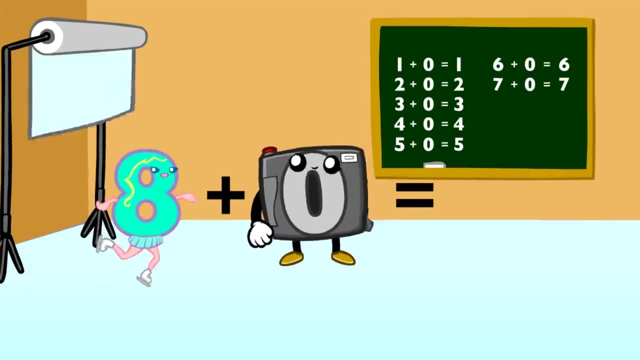 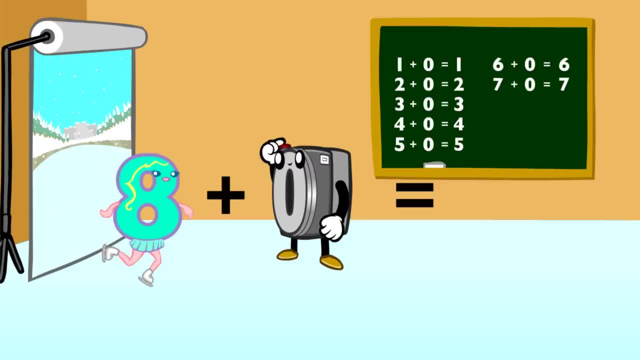 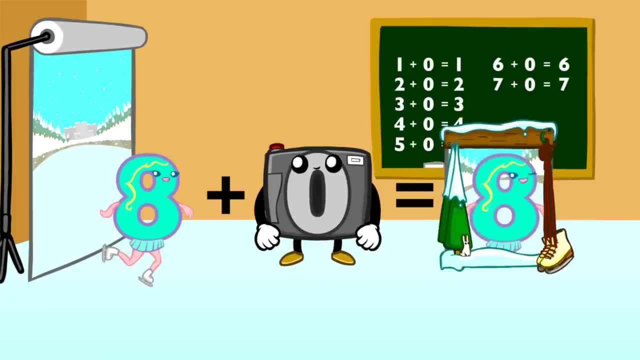 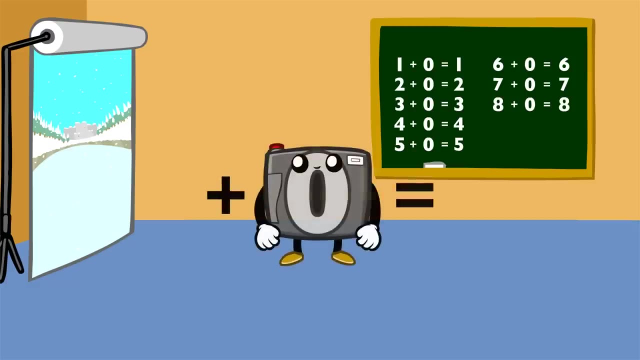 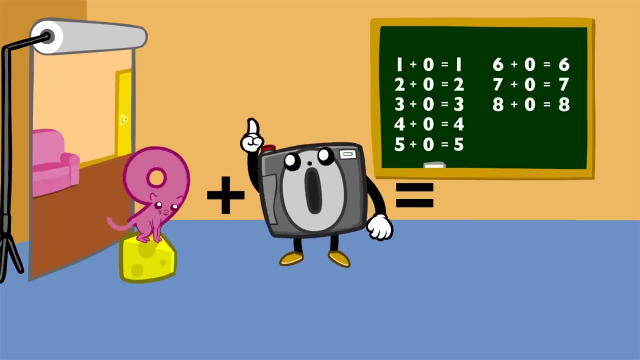 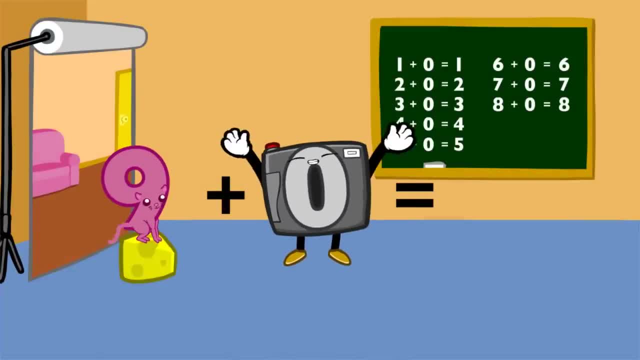 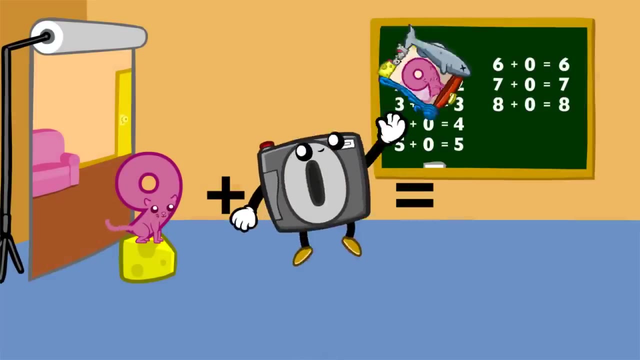 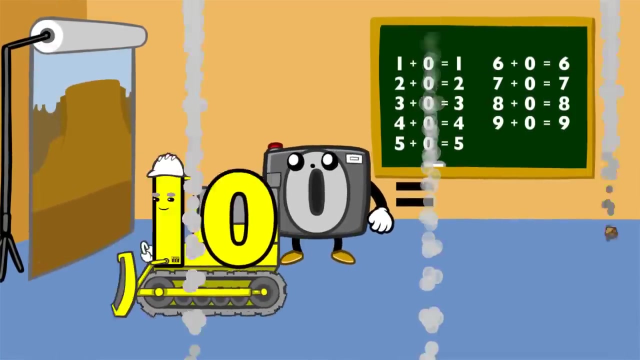 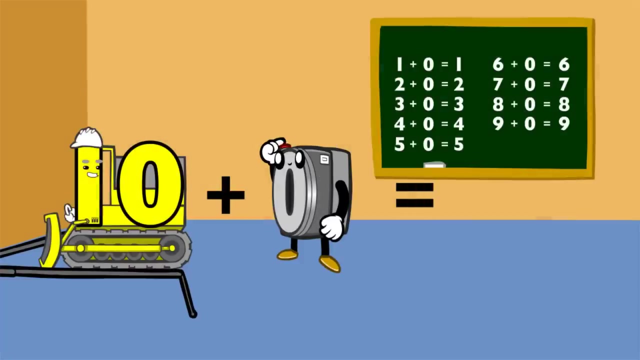 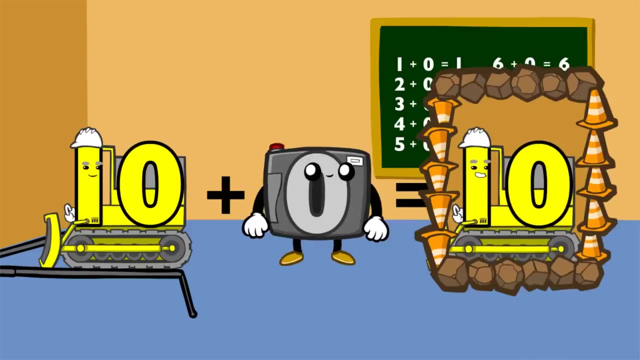 I'll tell you why. I'll tell you why. I'll take your picture. just say cheese And don't forget to smile, please. Nine plus zero equals nine, And don't forget to smile, please. And don't forget to smile, please. 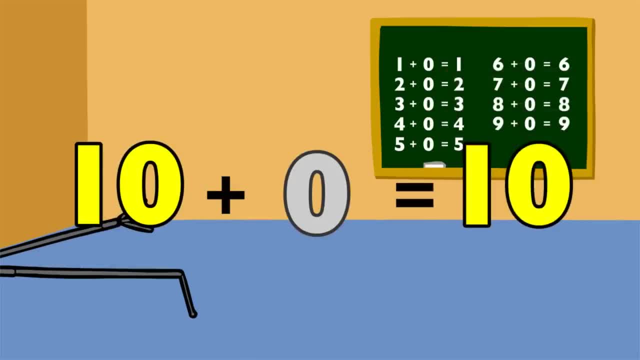 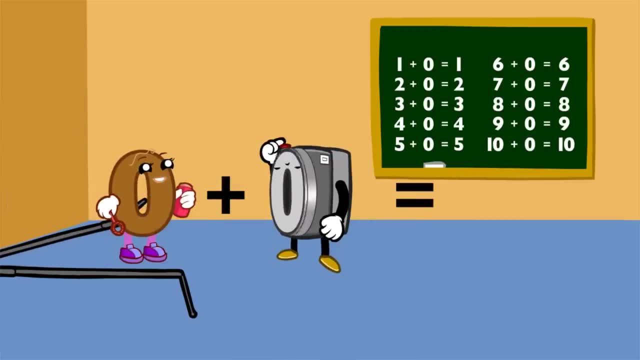 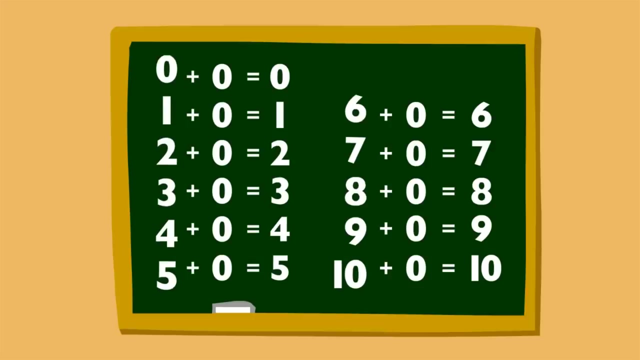 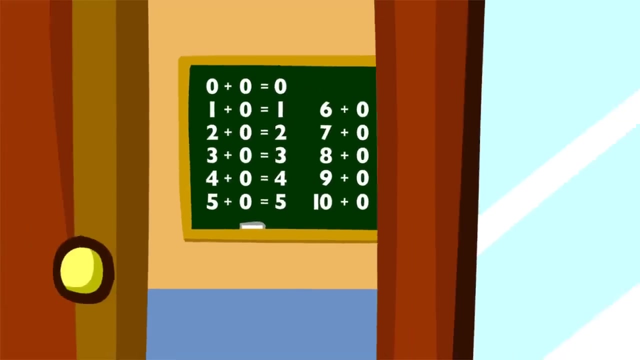 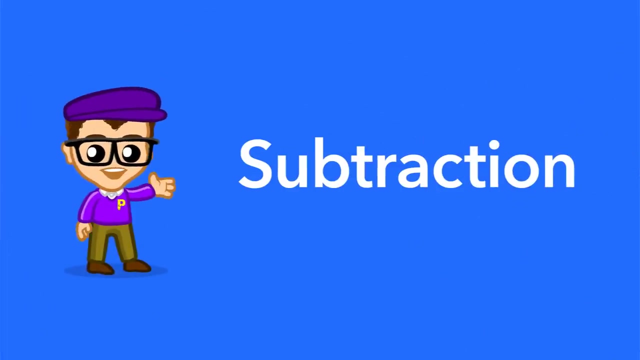 Ten plus zero equals ten. And don't forget to smile, please. And don't forget to smile, please. Zero plus zero equals zero. Any number plus zero equals itself. Now that you've learned the math facts, did you know you can use them for subtraction? 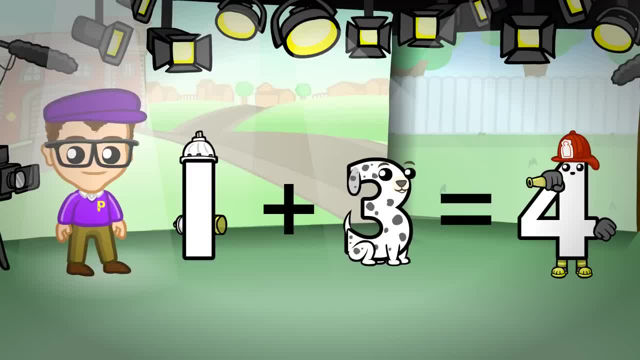 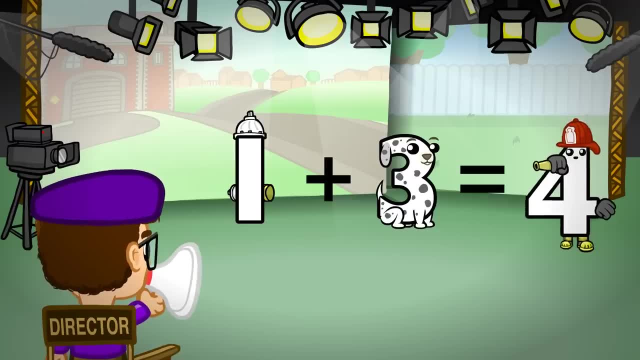 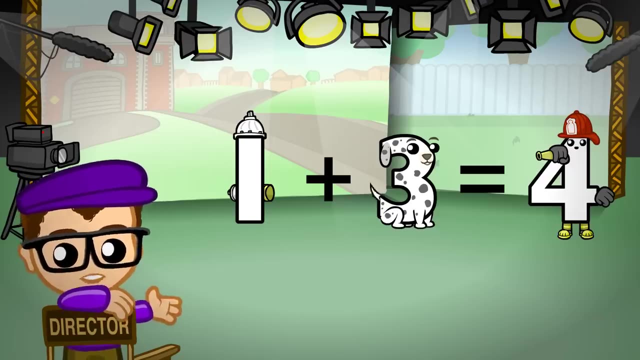 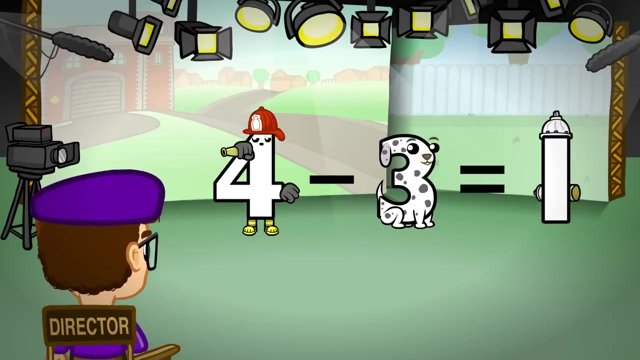 It's easy. I'll show you how. Would the largest number please step forward, Great. Now we just move the largest number to the beginning And action. Four minus three equals one, And four minus one equals three. Cut. 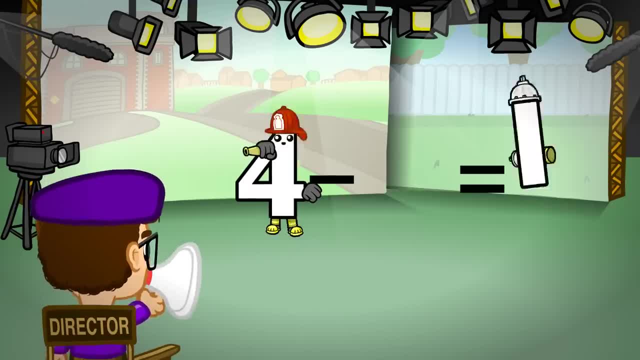 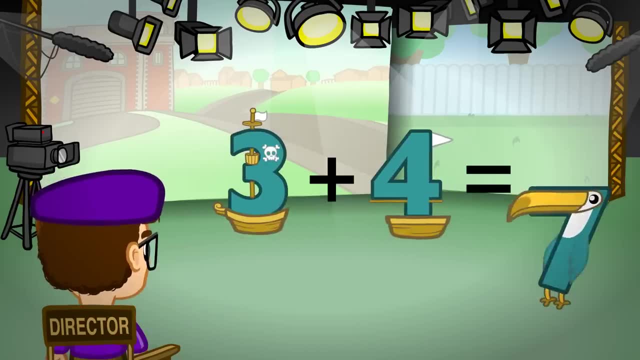 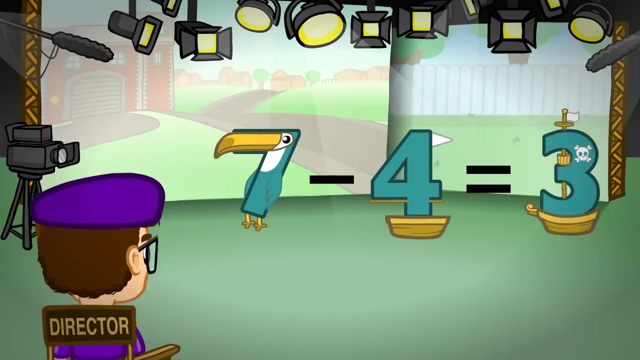 Next group. please Would three, four and seven take the stage. Would the largest number please step forward? Great, Okay, biggest number. Please move to the beginning. Seven minus four equals three, And seven minus three equals four, And seven minus three equals four. 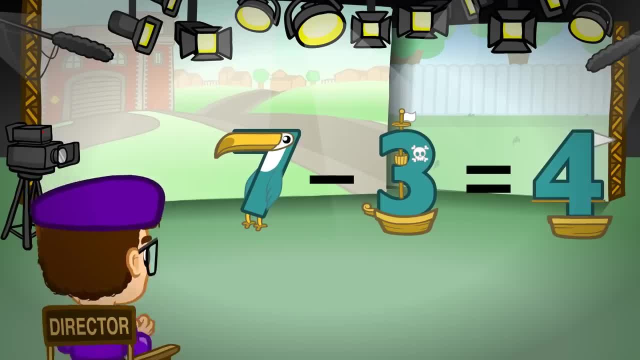 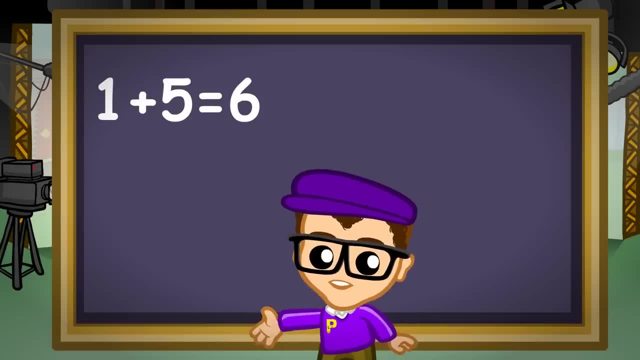 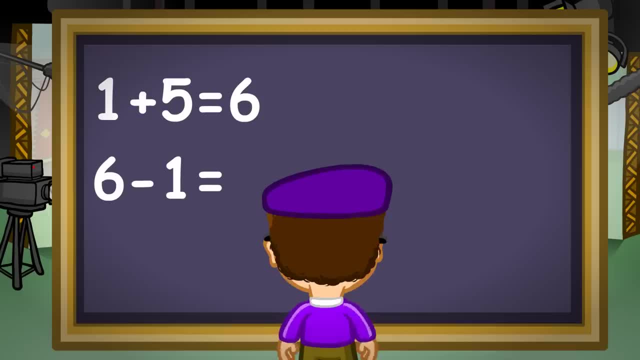 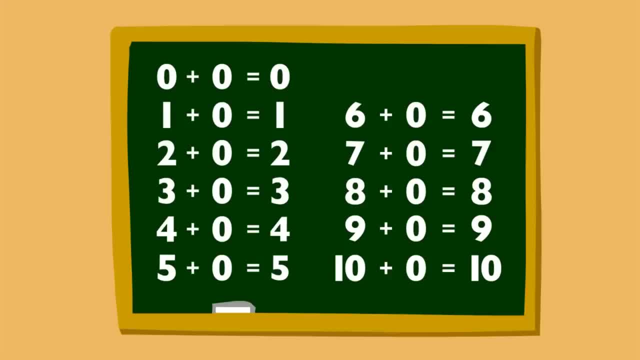 Ten and twelve are the pour treasure. Nine plus zero equals five. It's red and yellow. It's green and blue. It's blue and blue. It's green and blue. It's yellow and blue. It's blue and blue. It's green and blue. 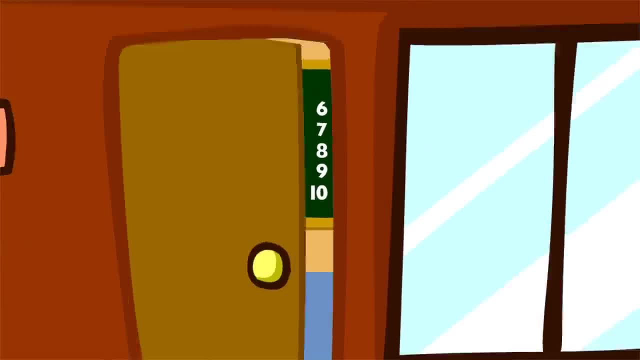 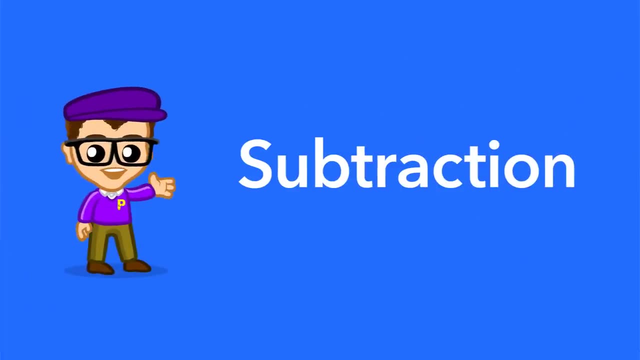 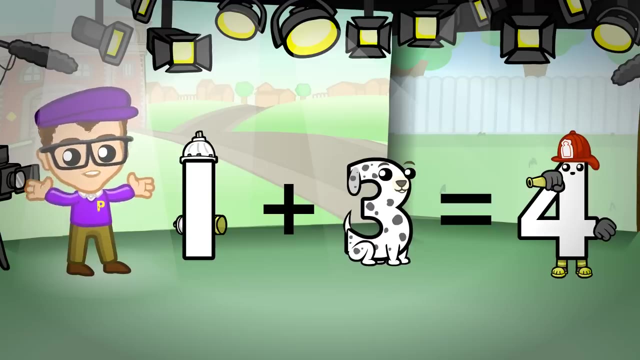 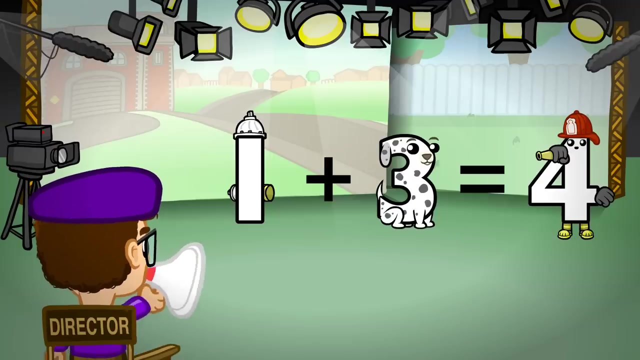 Now that you've learned the math facts, did you know you can use them for subtraction? It's easy. I'll show you how. With the largest number, please step forward. Great, Now we just move the largest number to the beginning. 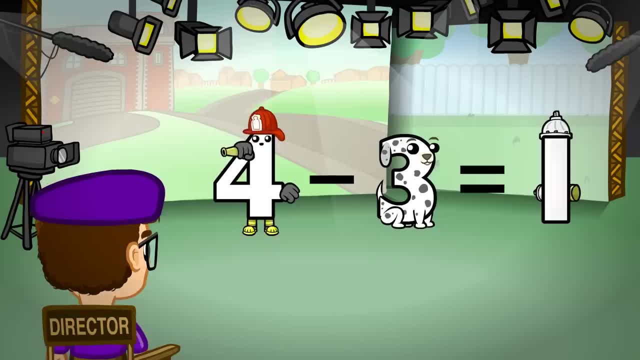 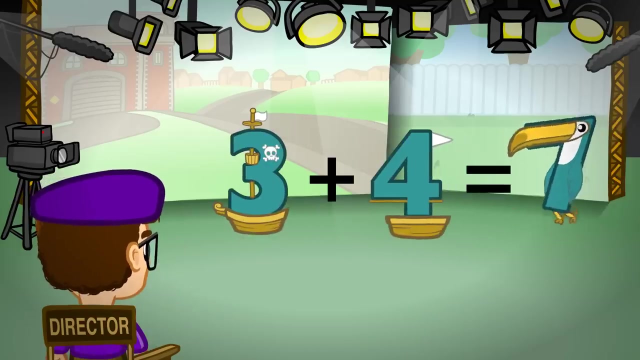 And action: Four minus three equals one And four minus one equals two And one equals three. Cut Next group. please Would three, four and seven take the stage With the largest number. please step forward. Great, Okay, biggest number. please move to the beginning. 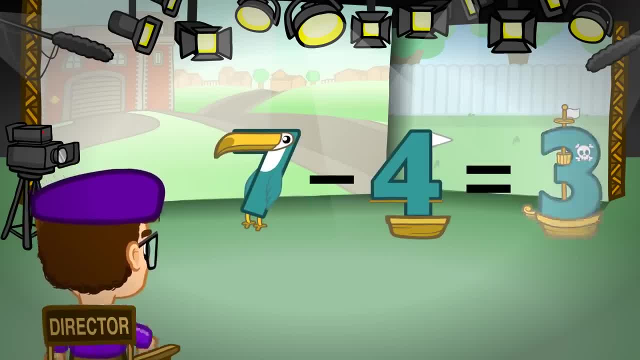 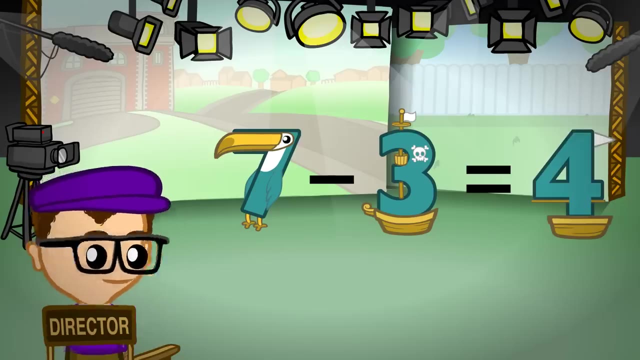 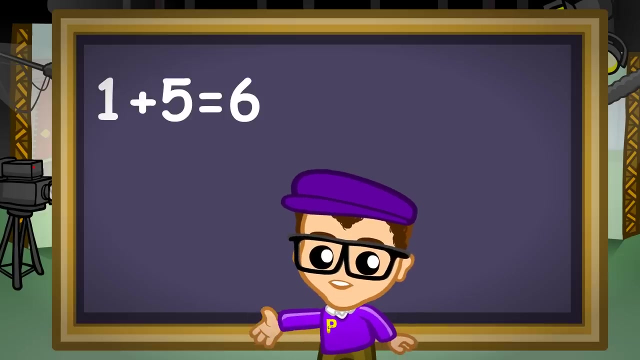 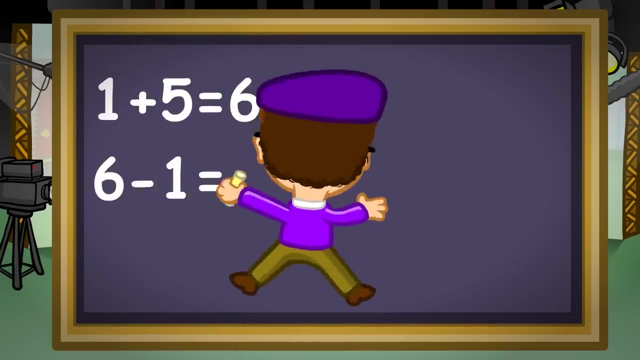 Seven minus four equals one, And action Four equals three, And seven minus three equals four. Now you try a few: One plus five equals six. One minus three equals zero. Four minus three equals one. No, Four plus five equals zero. 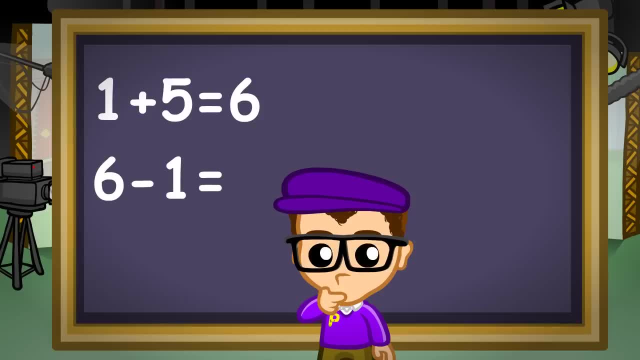 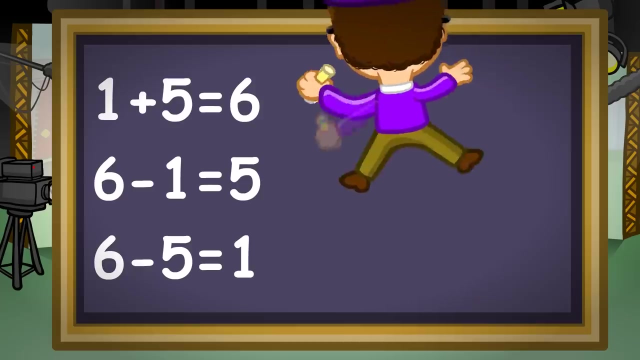 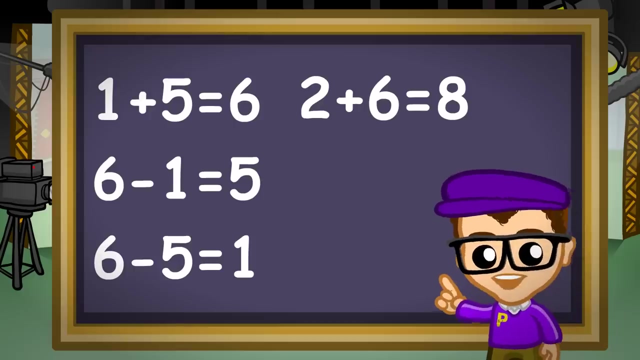 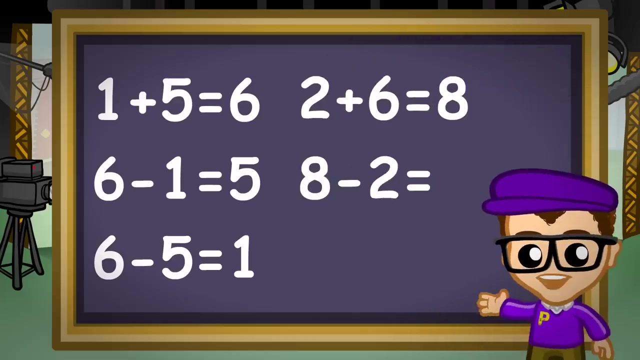 And seven minus three equals four, And seven minus three equals four. Five Right Five. And Six minus five equals One. That's right One. Let's try another. Two plus six equals eight. So eight minus two equals. 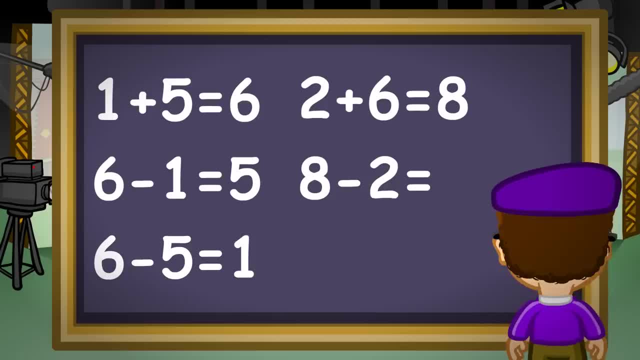 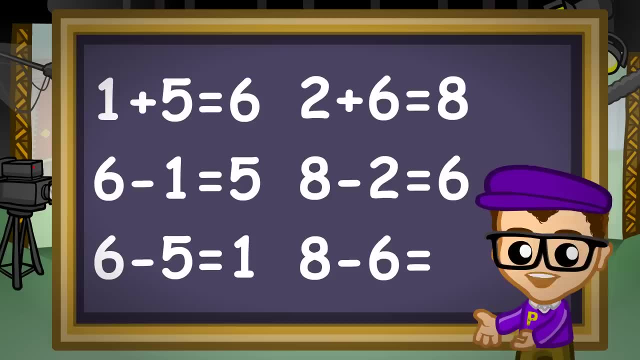 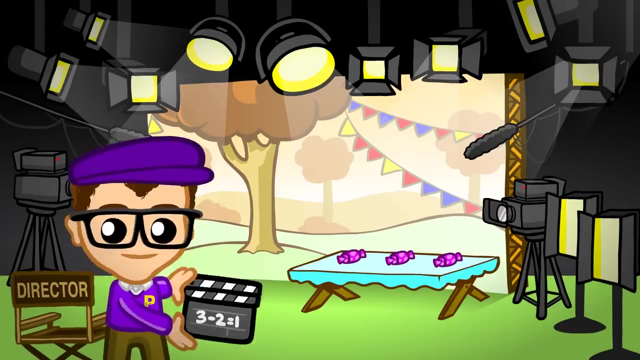 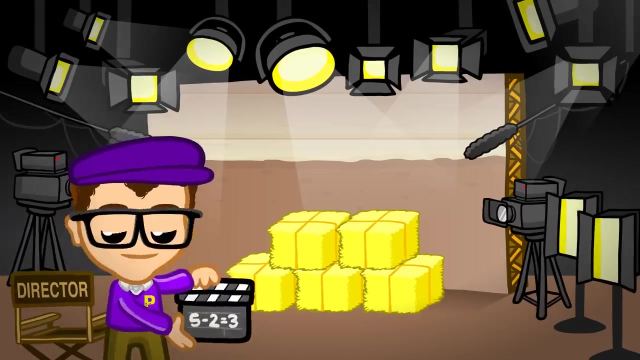 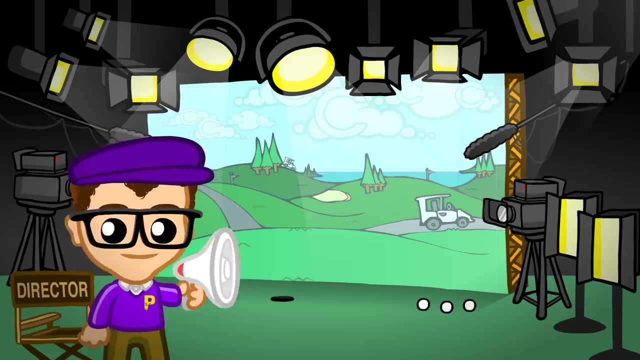 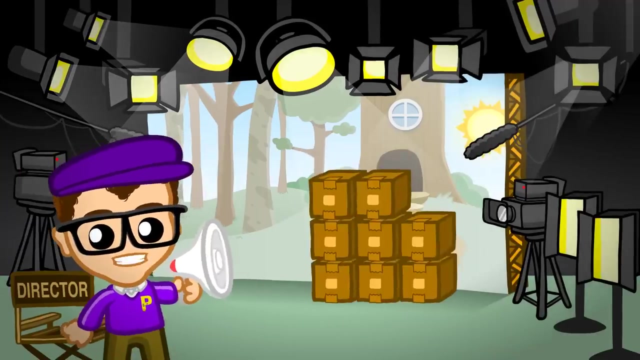 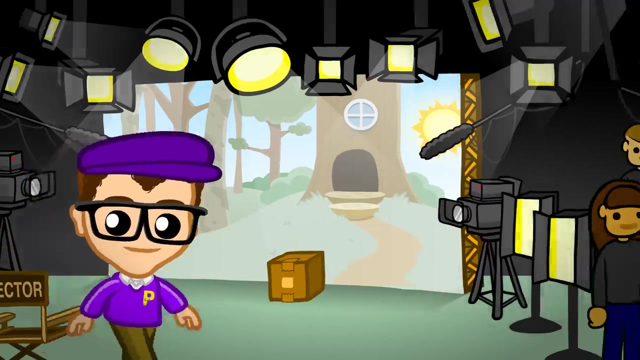 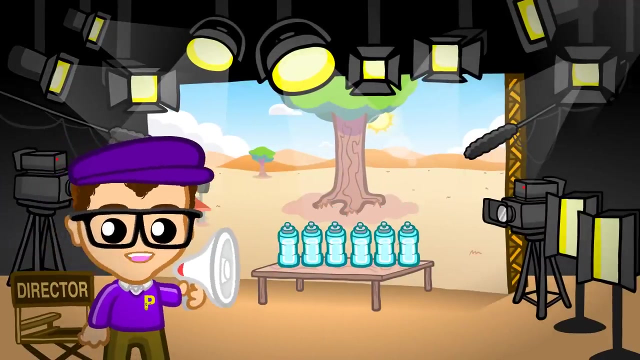 Six Right And Eight minus six equals Two Right. Three minus two equals one. Five minus two equals Three. Three minus three equals zero. Eight minus seven equals one One Right. Six minus three equals Three. And Ten minus zero equals Ten. Right. 8 minus 4 equals 4.. 7 minus 6 equals 1.. 4 minus 4 equals 0.. 4 minus 2 equals 2.. 2 minus 1 equals 1.. 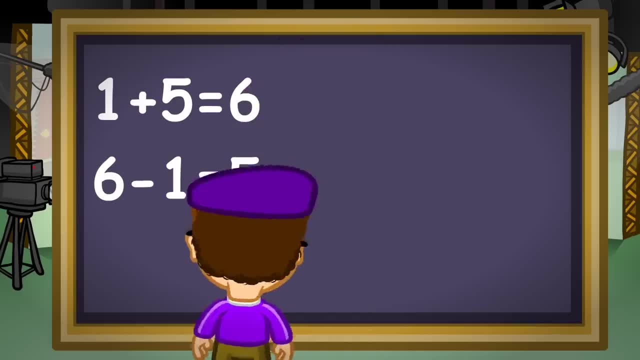 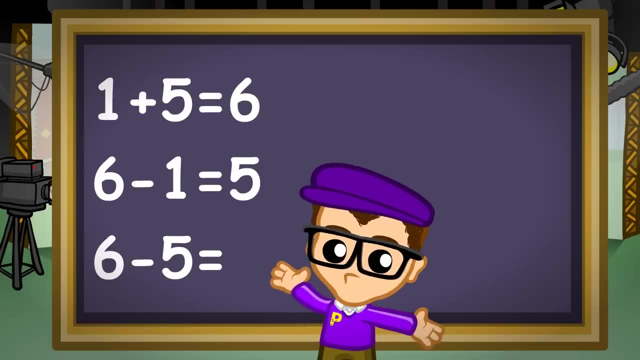 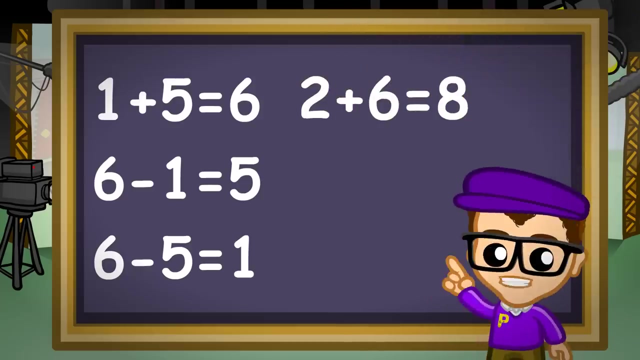 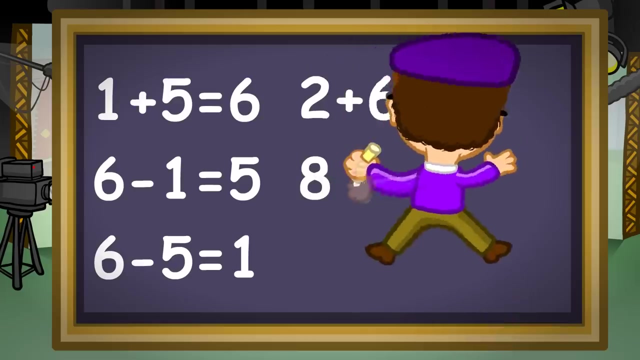 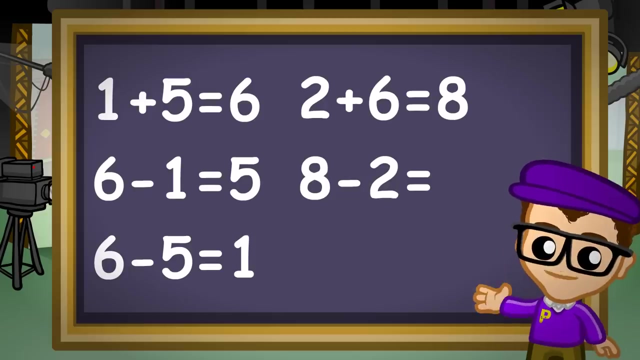 Now drop the cidade in the quarter. There we go. Six minus one equals Five- Right Five, That's right One. Let's try another. Two plus six equals eight. So eight minus two equals Six Right. 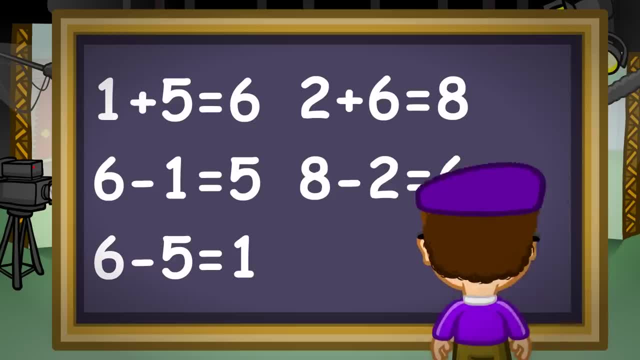 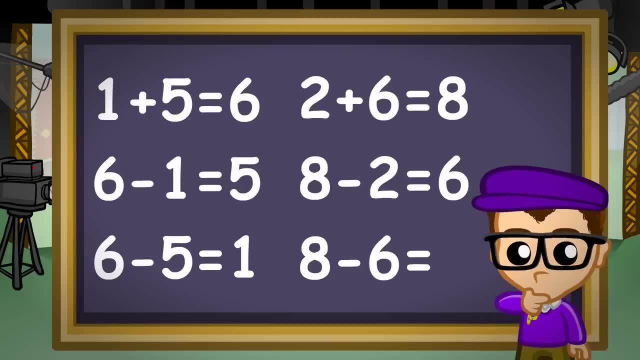 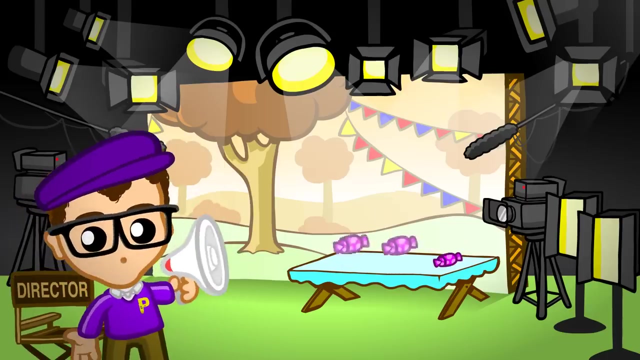 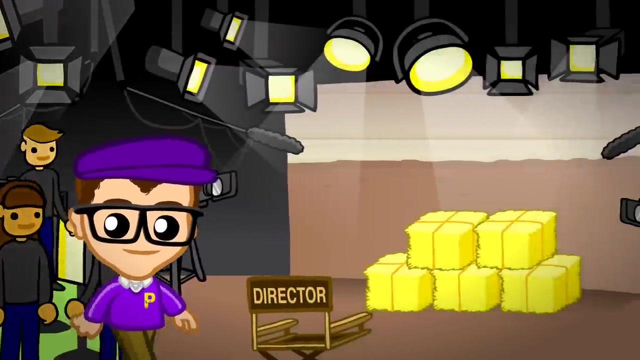 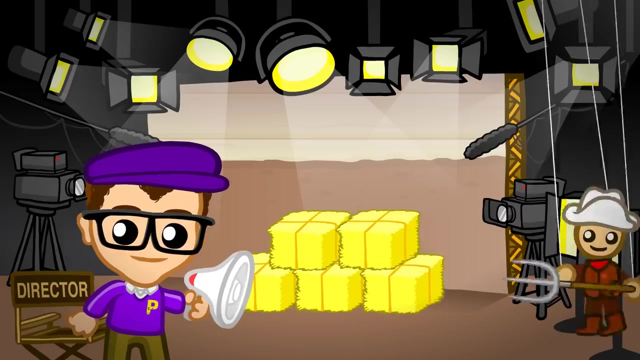 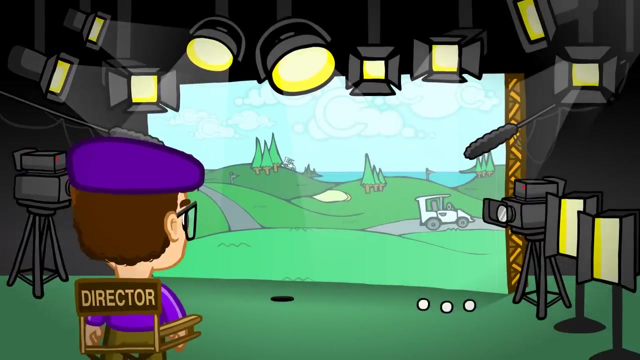 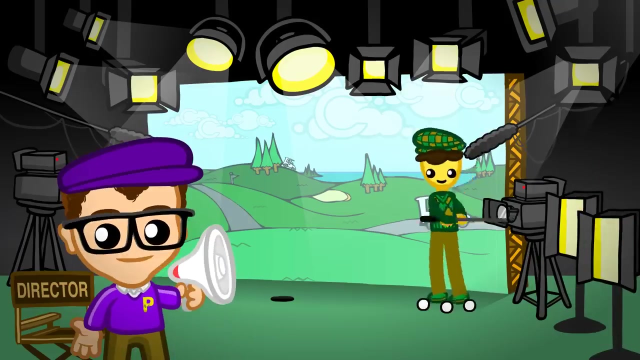 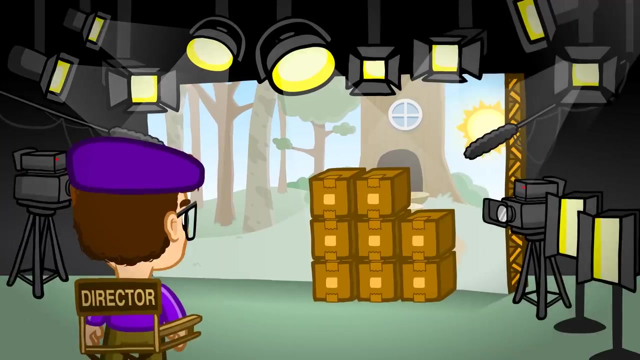 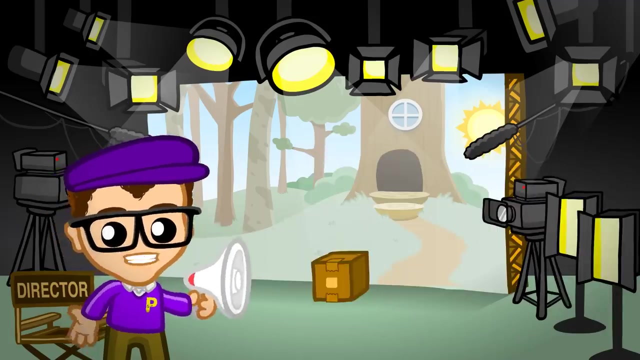 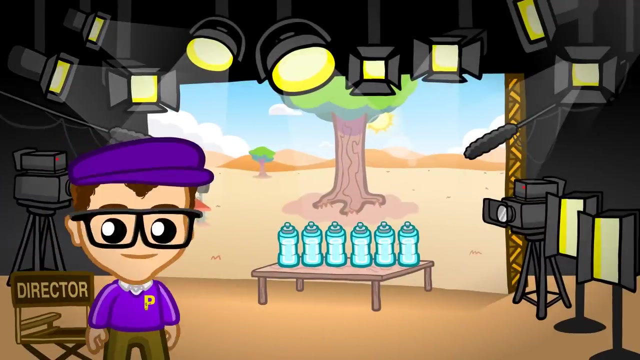 Two And eight minus six equals Two Right. Three minus two equals one Right. Five minus two equals three. Three minus three equals zero Right. Eight minus seven equals one. Six minus three equals three Right, Two Right. 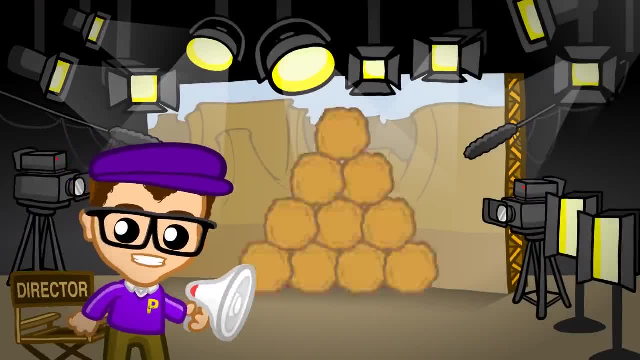 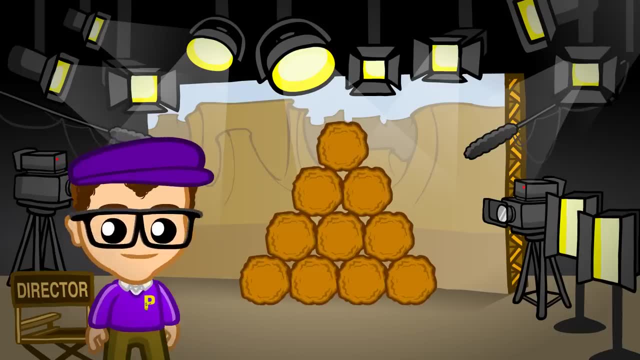 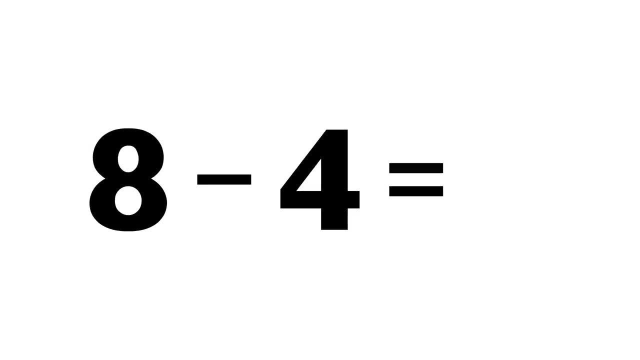 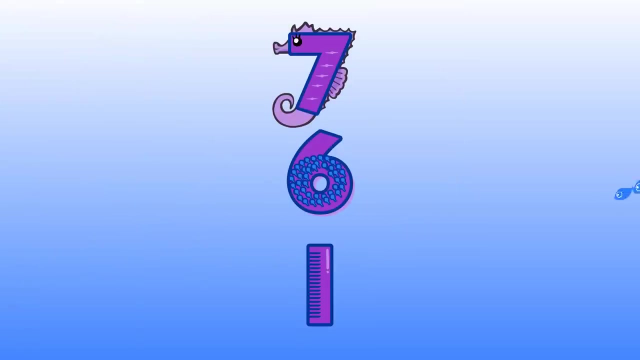 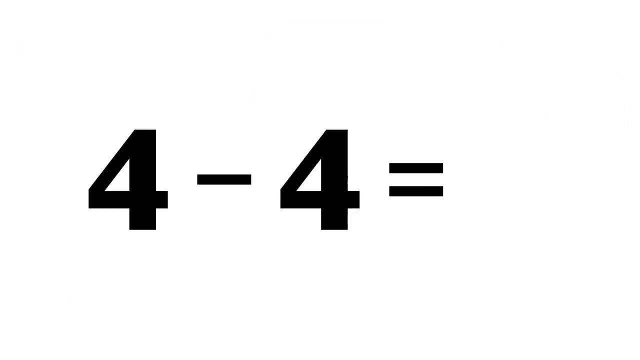 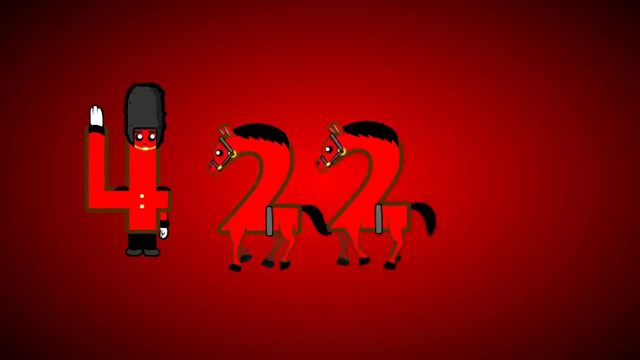 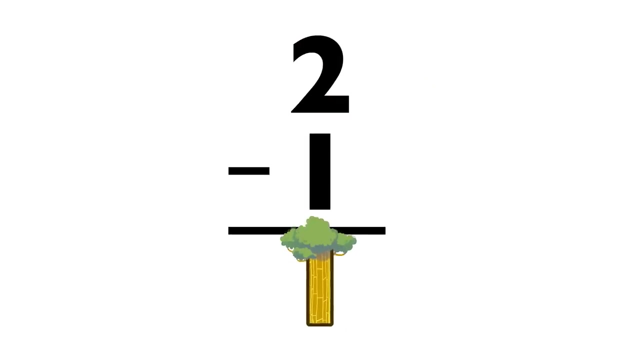 Two Right Two. Ten minus zero equals ten. Eight minus four equals four. Seven minus six equals one. Right Four minus four equals Zero. Four minus two equals Two. Two minus one equals One. One minus two equals two. 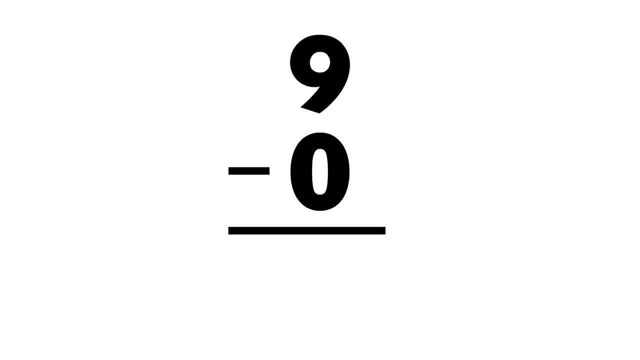 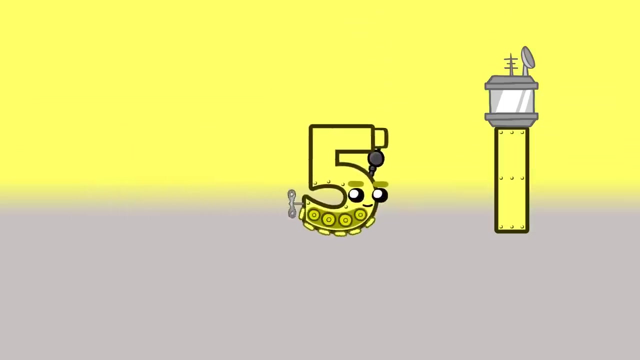 Two, Four, Two minus three equals half One, Two, Two. One Two Yeah Three. left goes to right Two, Yeah, Two, Two. Good job, Right One, Boom, Boom, Boom 3.. 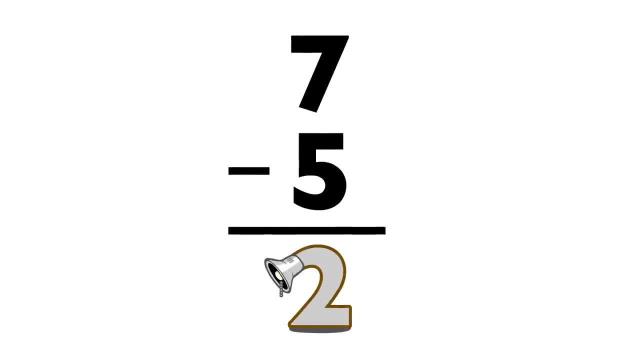 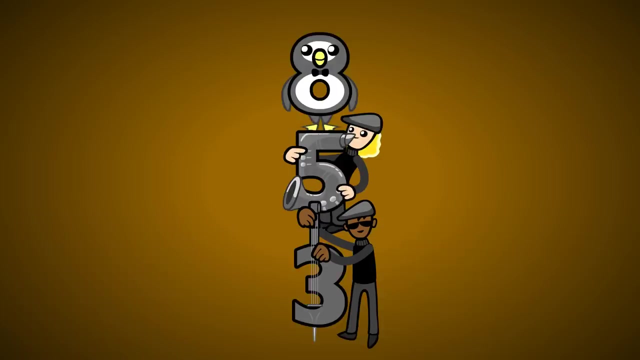 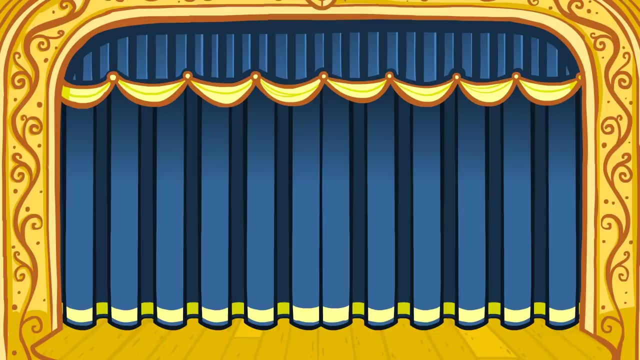 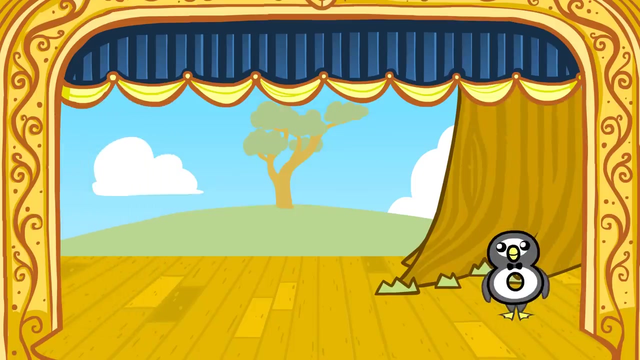 Four, No, No. Bark sorts. 6 minus 2 equals 4. 8 minus 5 equals 3. Ladies and gentlemen, please give a round of applause to Meet the Math Facts: 1 plus 1 equals 2. 1 plus 2 equals 3. 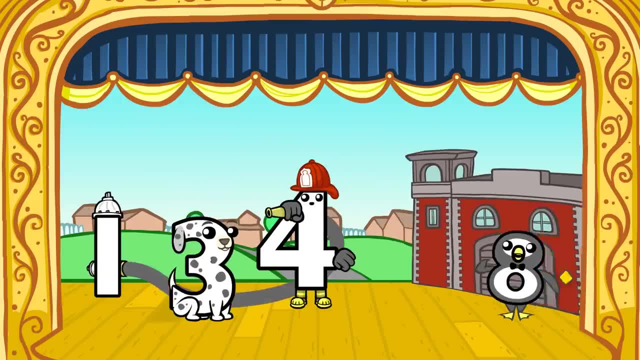 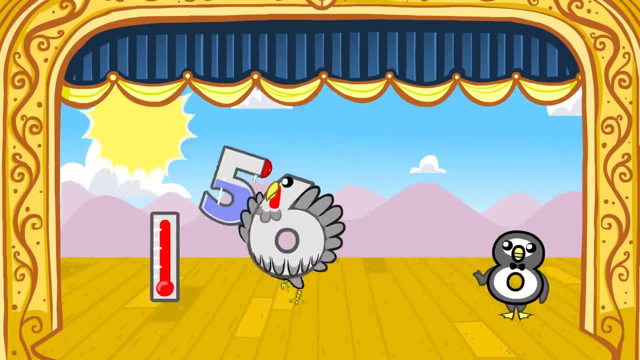 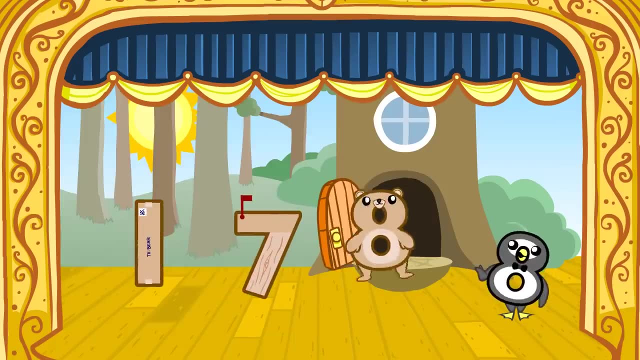 Whatever 1 plus 3 equals 4. 1 plus 4 equals 5. 1 plus 5 equals 6. Whatever 1 plus 6 equals 7. 1 plus 5 equals 6. 1 plus 5 equals 6. 1 plus 7 equals 8. 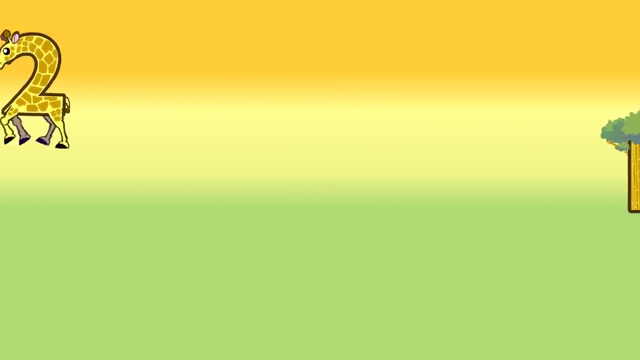 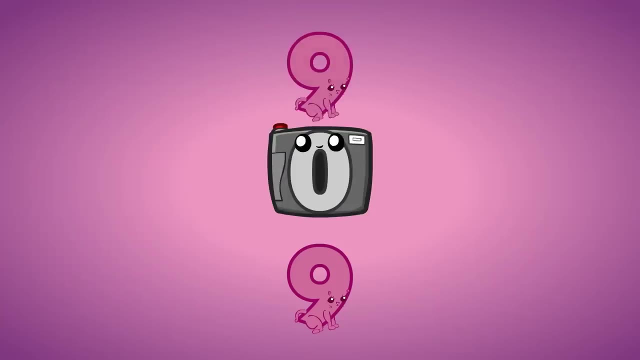 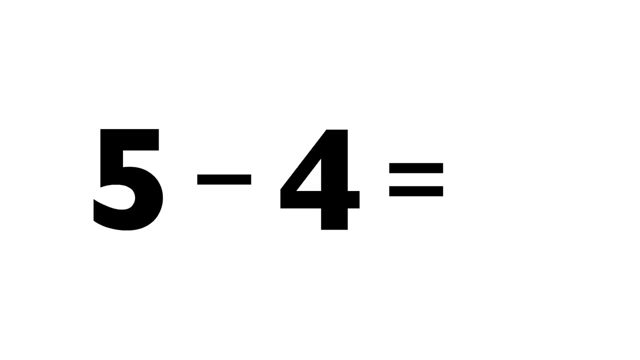 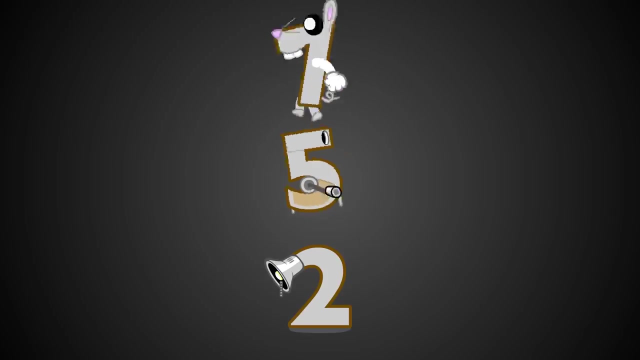 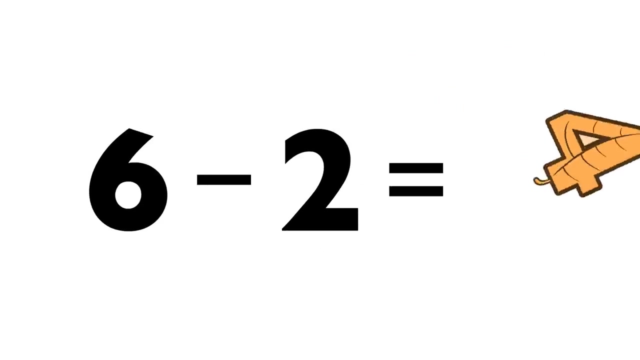 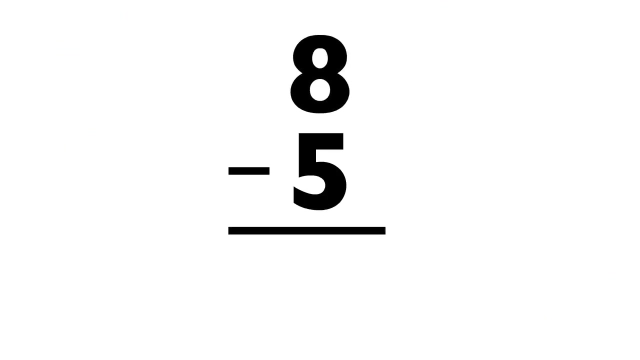 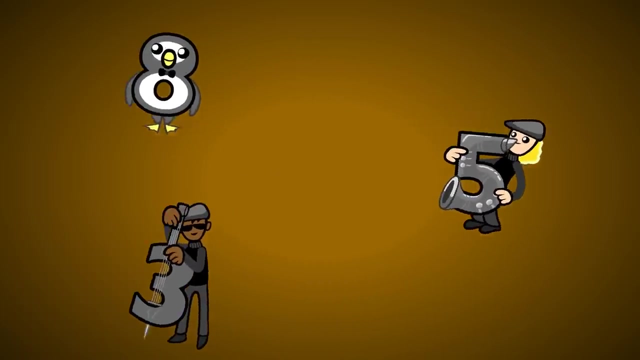 9 minus 0: equals 9.. 5 minus 4 equals 1.. 7 minus 5 equals 2.. 6 minus 2 equals 4.. 8 minus 5 equals 3.. Ladies and gentlemen, please give a round of applause to. 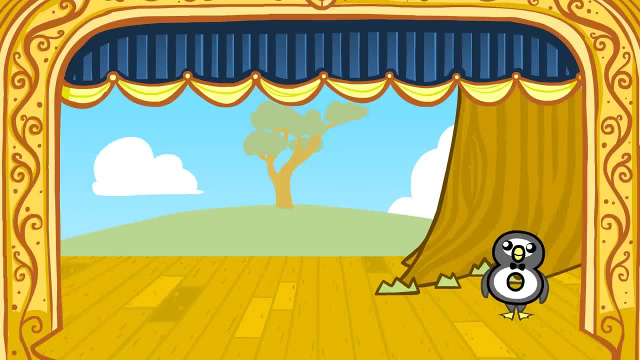 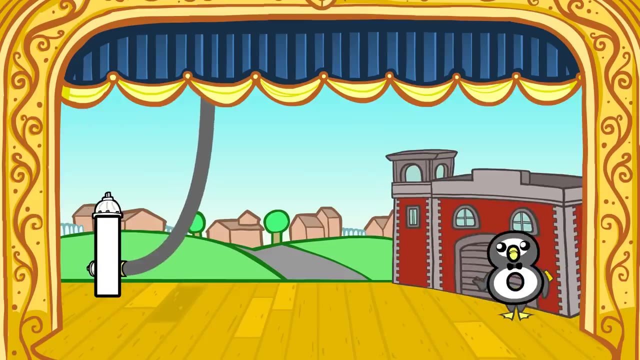 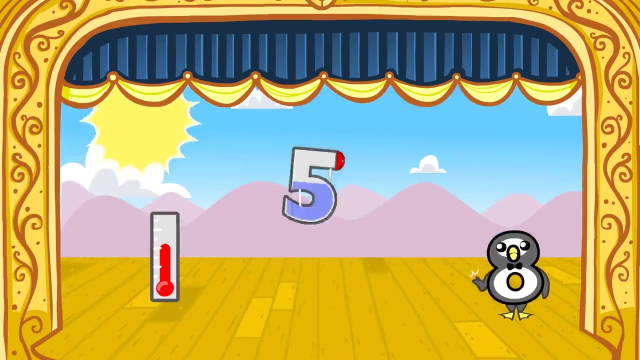 Meet the Math Facts: 1 plus 1 equals, 2.. 1 plus 2 equals, 3.. Whatever, 1 plus 3 equals 4.. 1 plus 4 equals, 5.. 1 plus 5 equals 6.. 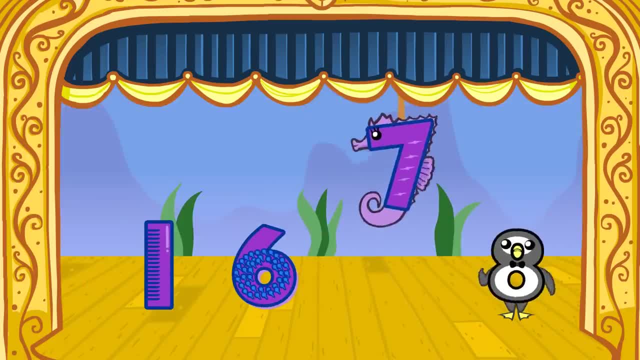 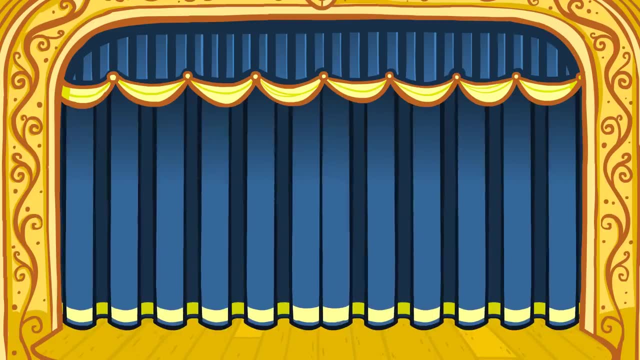 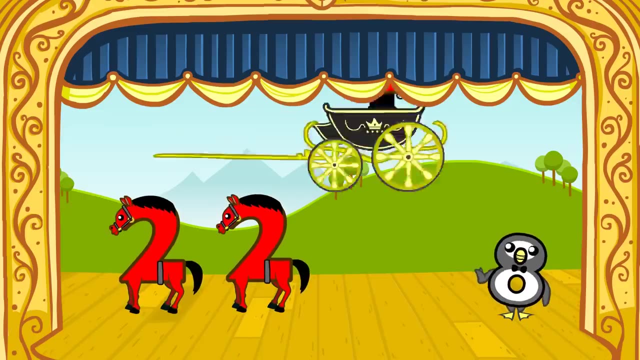 Whatever, 1 plus 6 equals 7.. 1 plus 7 equals 8!. And now let's start with 2.. 2 plus 1 equals 3.. 2 plus 2 equals 4.. 2 plus 3 equals 5.. 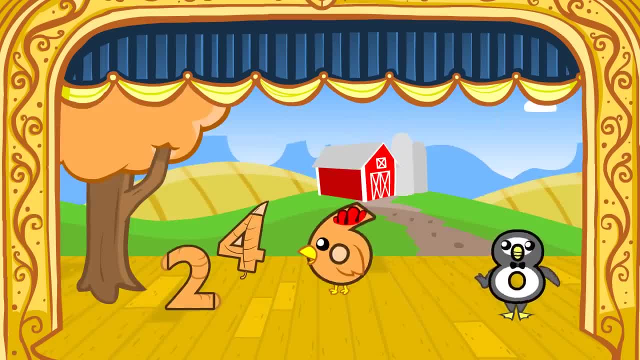 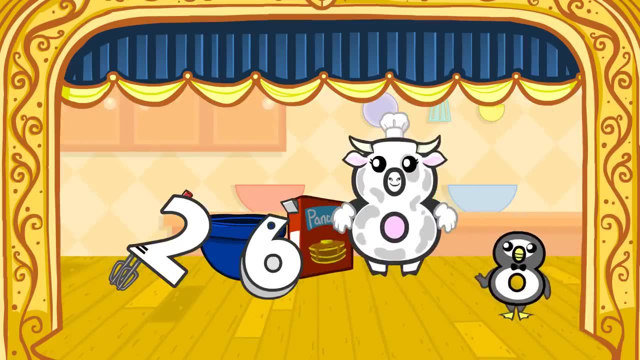 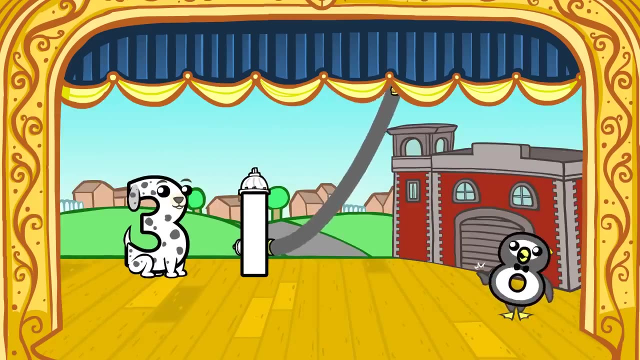 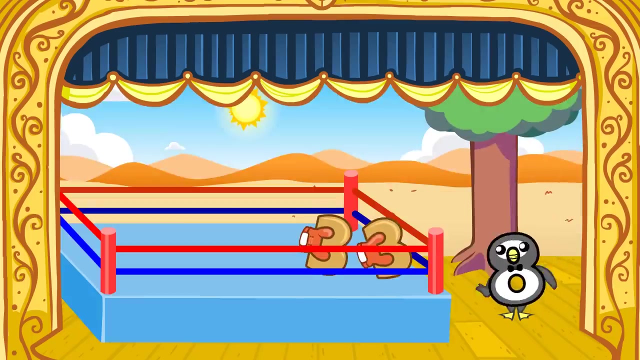 2 plus 4 equals 6.. 2 plus 5 equals 7.. 2 plus 6 equals 8.. Now let's move on to three. Three plus one equals four. Three plus two equals five. Three plus three equals six. 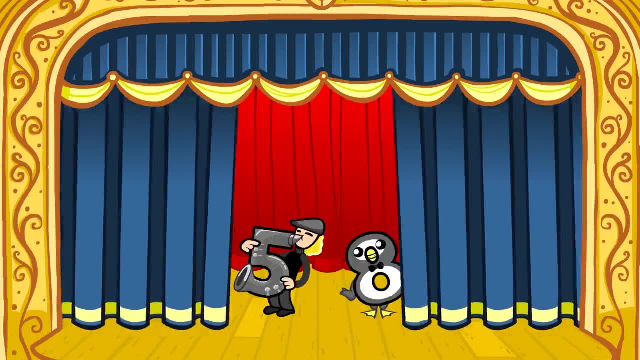 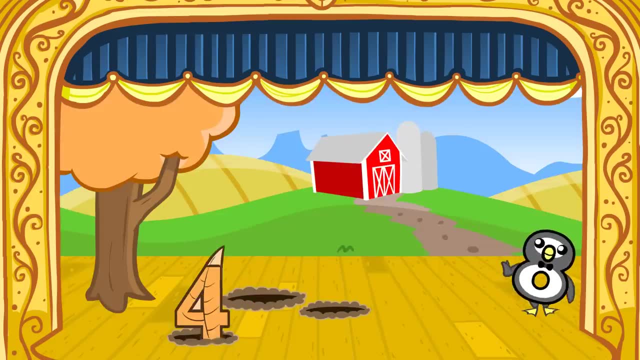 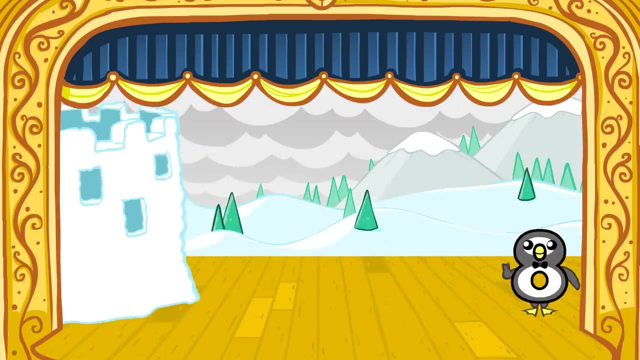 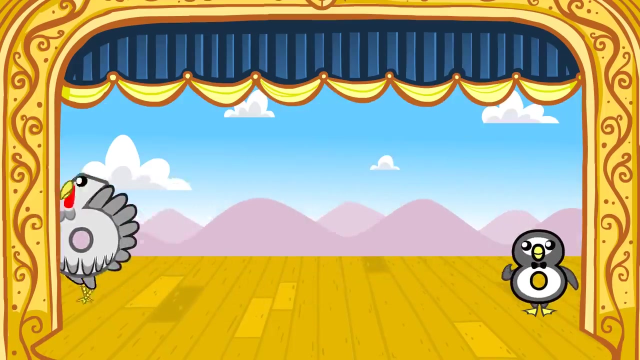 Plus four equals seven. Three plus five equals eight. Four plus one equals five. Four plus two equals six. Four plus three equals seven. Four plus four equals eight. Five plus one equals six. Five plus two equals seven. Five plus three equals eight. 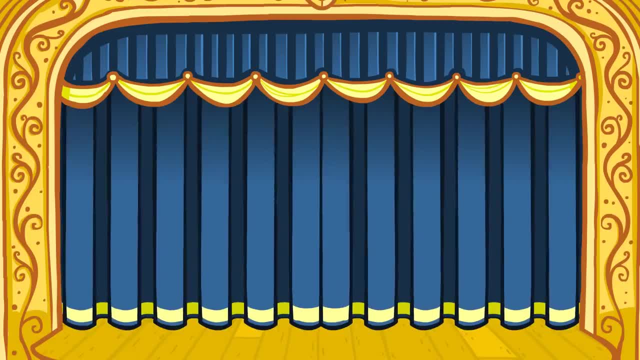 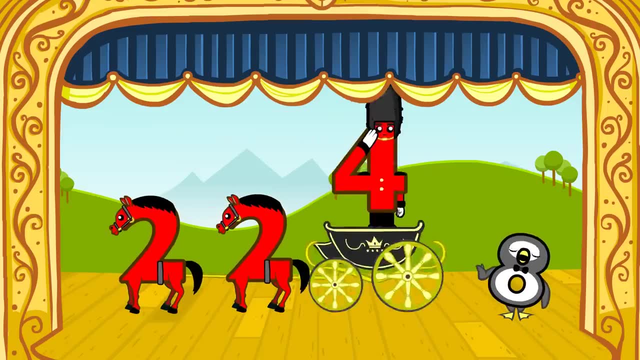 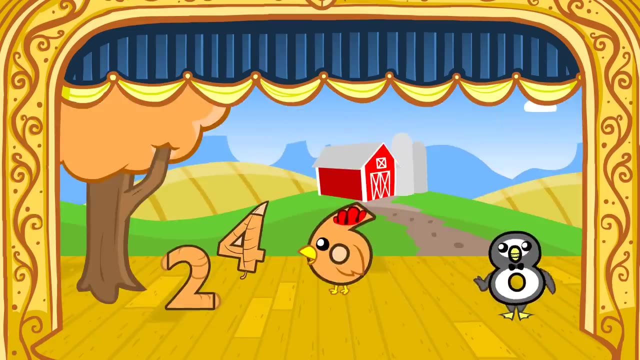 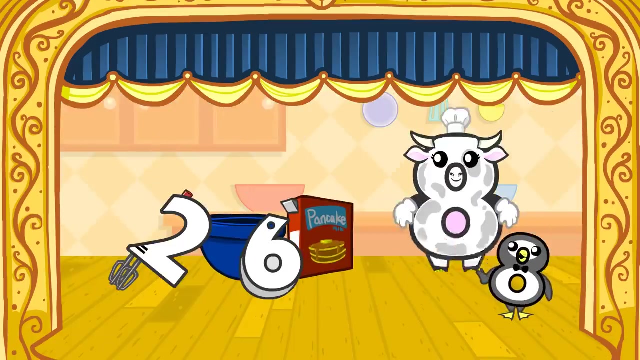 And now let's start with 2. 2 plus 1 equals 3. 2 plus 2 equals 4. 2 plus 3 equals 5. 2 plus 4 equals 6. 2 plus 5 equals 7. 2 plus 6 equals 8. 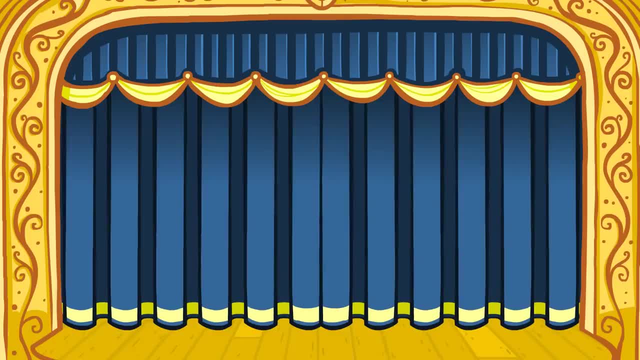 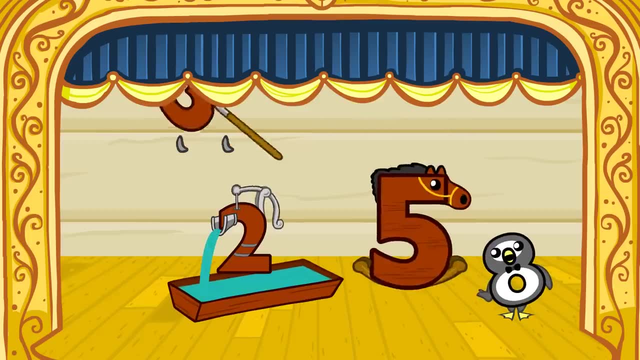 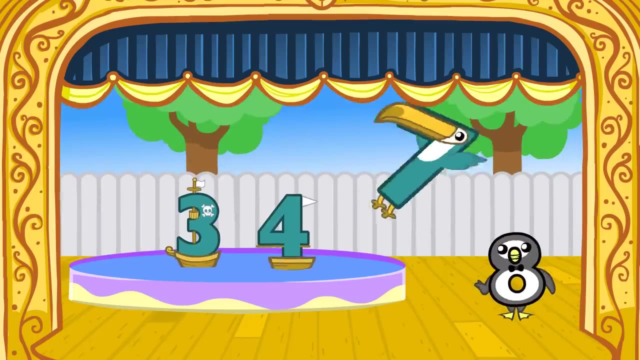 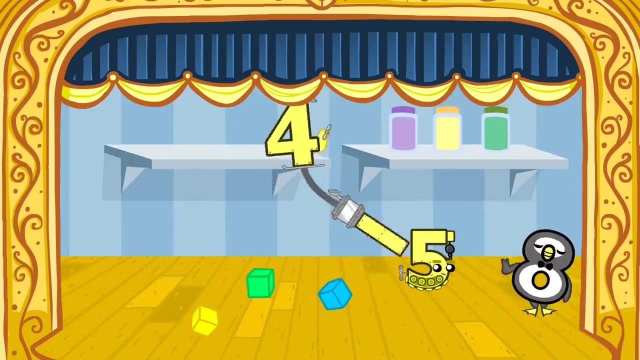 Now let's move on to the next one: 3 plus 1 equals 4. 3 plus 2 equals 5. 3 plus 3 equals 6. 3 plus 4 equals 7. 3 plus 5 equals 8. 4 plus 1 equals 5. 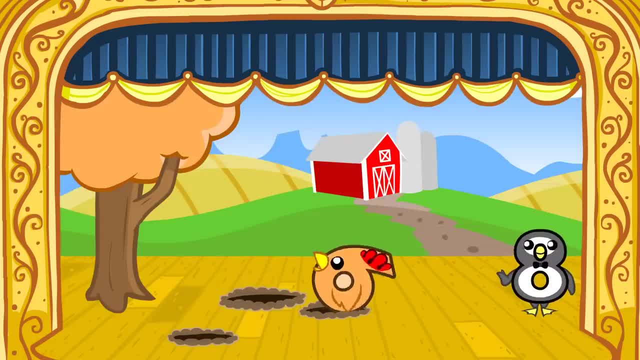 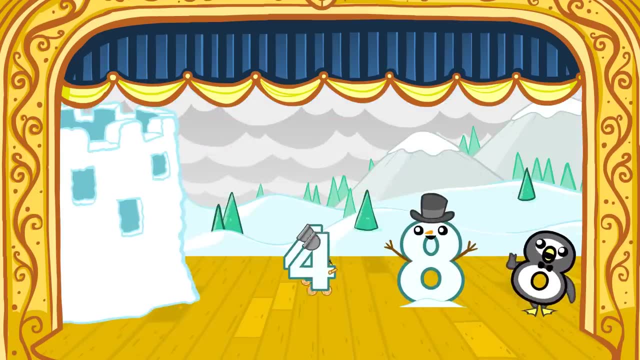 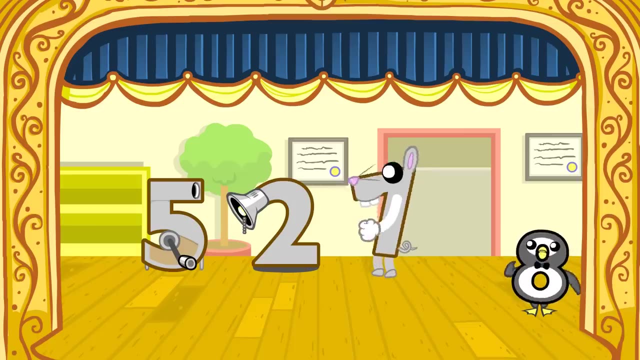 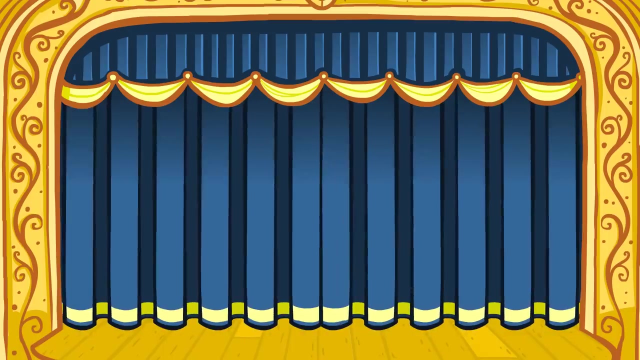 4 plus 2 equals 6. 4 plus 3 equals 7. 4 plus 4 equals 8. 5 plus 1 equals 6. 5 plus 2 equals 7. 5 plus 3 equals 7. Now let's start with 6. 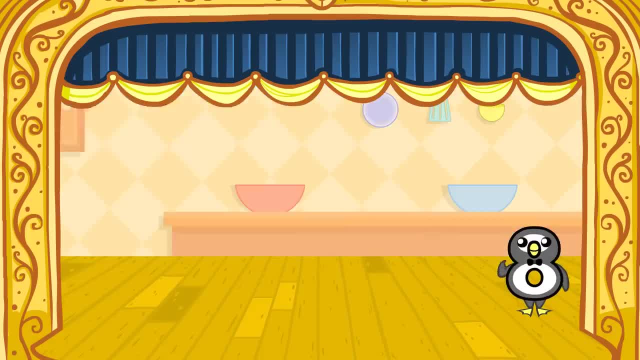 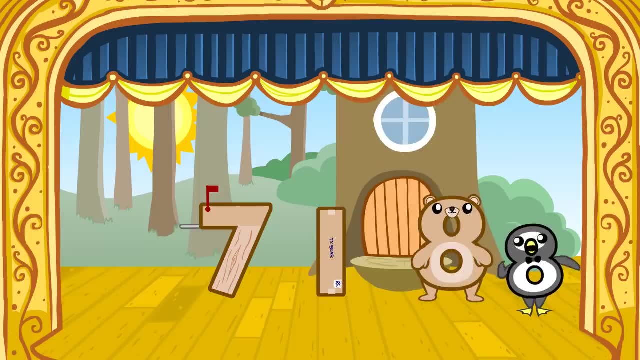 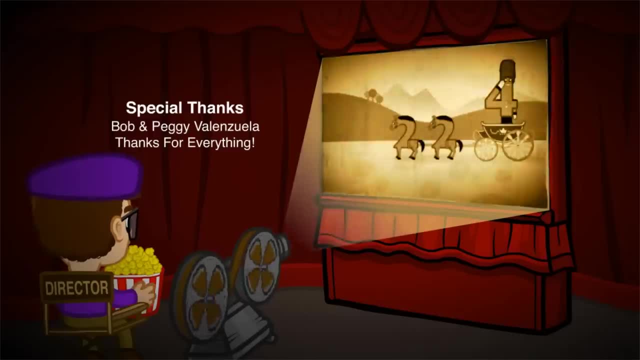